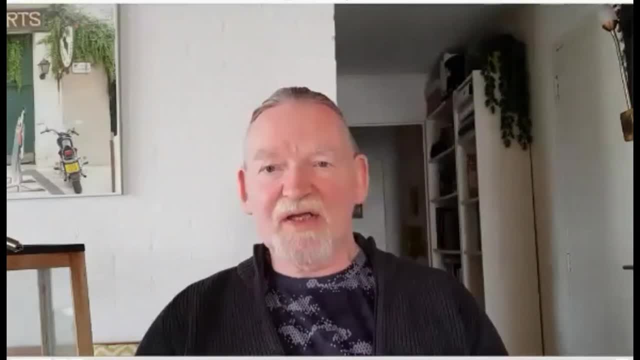 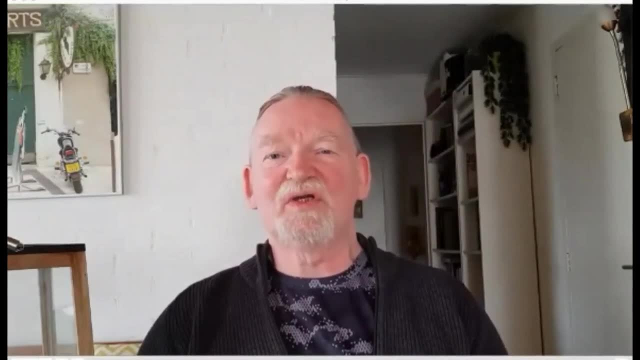 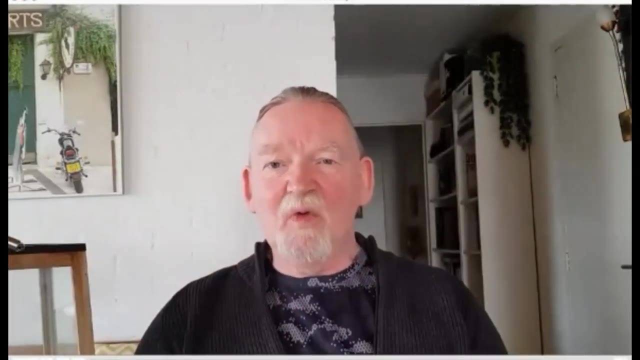 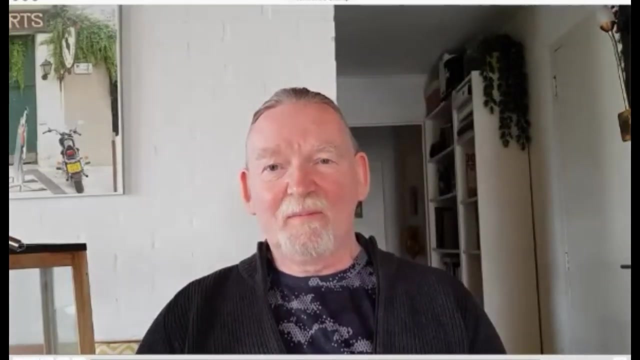 But we seem to be able to organize in real life events. this year, If all goes well, we expect to have the first real event, as in people meeting people, somewhere in June. Let's hope and pray we will be successful. Now then For the general overview of the chapter. 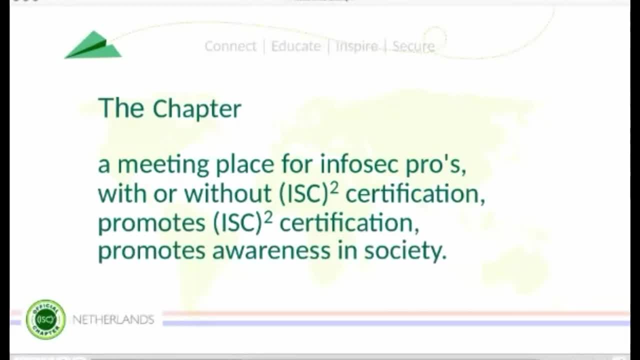 The Dutch chapter has been a meeting place for information security professionals for about five years now. We welcome people with or without IC2 certification. We try to promote awareness of information security in society, But we also try to promote IC2 certification. So for those of you that aren't certified yet, ask for help. 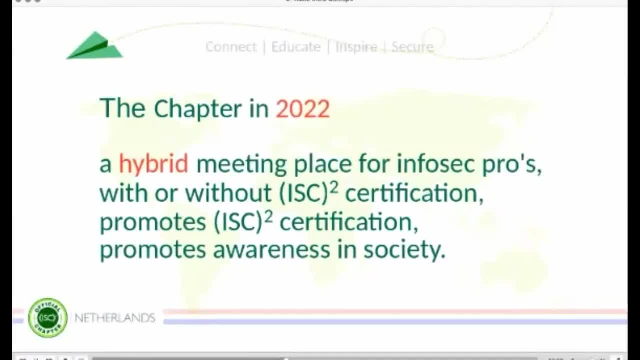 We will try to help you as best as we can. The pandemic: The pandemic has forced us into virtualization last year. However, these virtual events also have their advantages. Hence the board has decided to continue the virtual events, combined with, of course, as soon as possible in real life events. 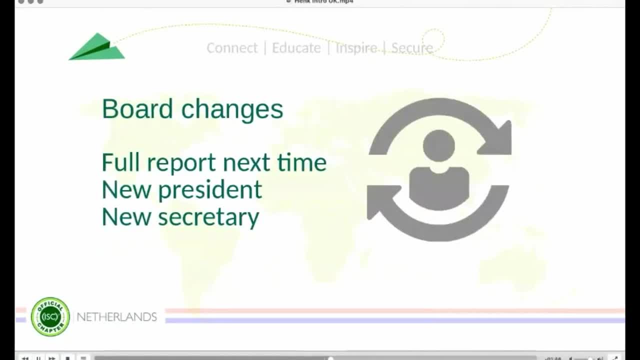 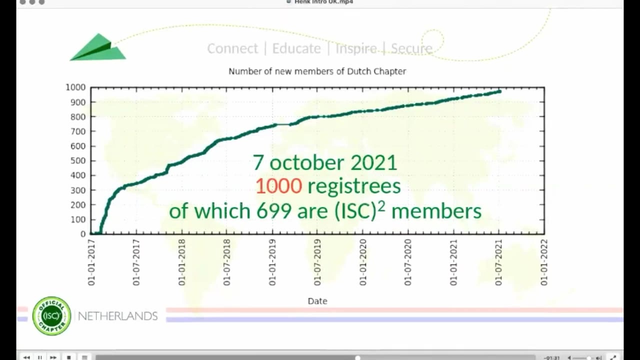 2022 will also bring us some board changes. We will have a new president and we will have a new secretary. A full report will be made next time. I am very happy to report that the chapter is still growing. Last time I reported 1,000 registries. 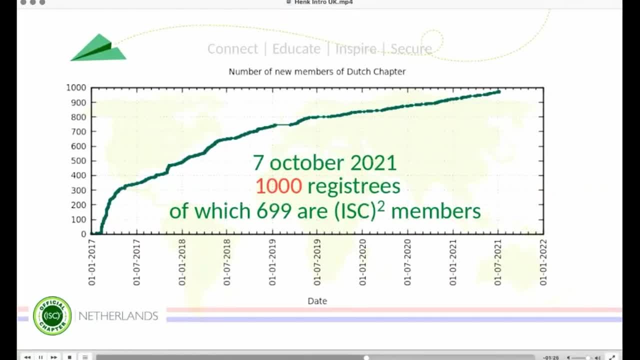 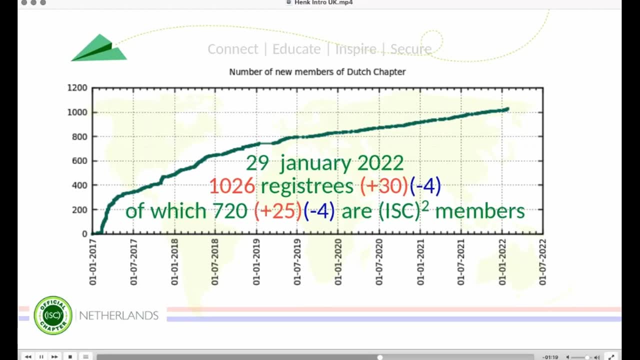 Now I can report that we have grown again. We are now with 1,026 registries, 30 more than last time. In case you may wonder how it is that we have a growth of 30 people and only 26 more registries, 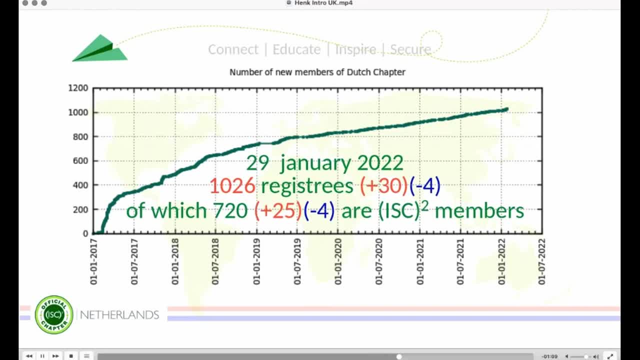 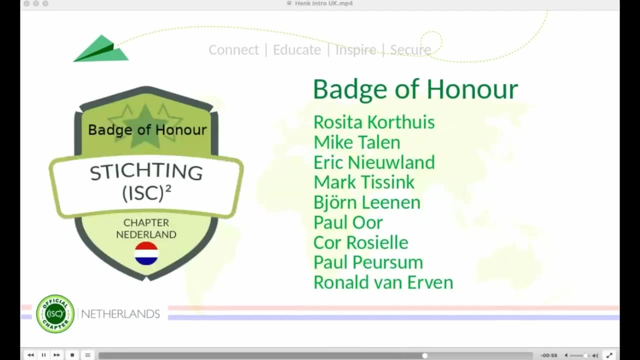 Well, People also leave the chapter, For example because they are retired. I am also very happy to report that most of our registries are IC2 members, so fully certified. The following members wear the badge of honor: Rosita Korthuis. 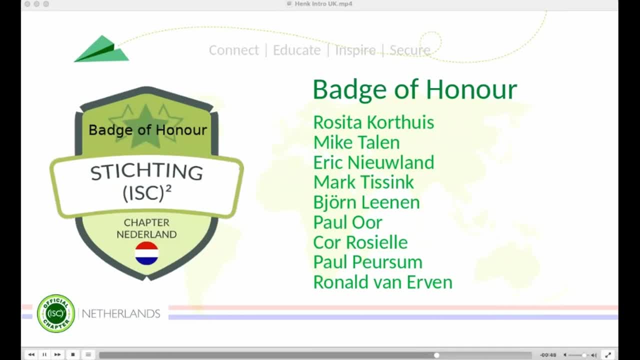 Mike Talen, Erik Nieuwland, Mark Tissink, Björn Leenen, Paul Oor Coro, Gelle Paul Peursum And Ronald van Erven. Thank you very much for your contributions. We would like to thank our friends and sponsors. 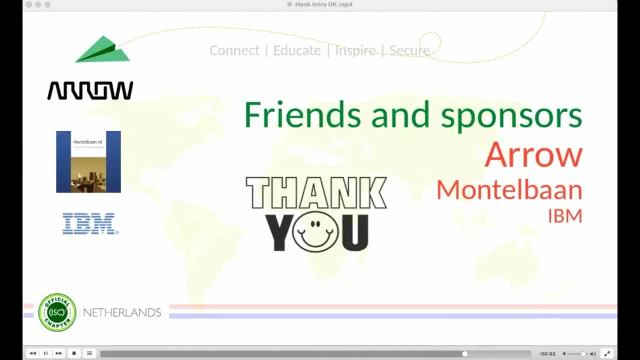 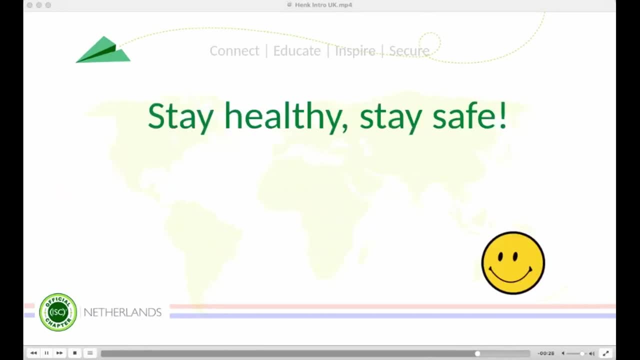 Arrow, Montalban and IBM. We would also like to thank Zoom for sponsoring today's event. Society seems to resume its normal course again. However, please stay healthy, stay safe. We aren't there yet. Head now for tonight's program. 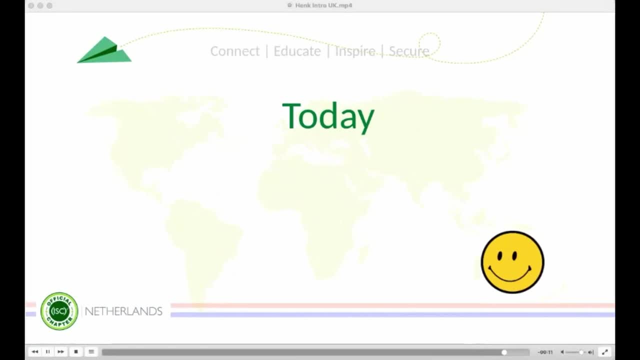 We have two excellent speakers. We have two excellent speakers that will tell you many interesting things about software development and software security. I hope you will have a nice evening And I'm looking forward to seeing you again this year. Thank you very much. 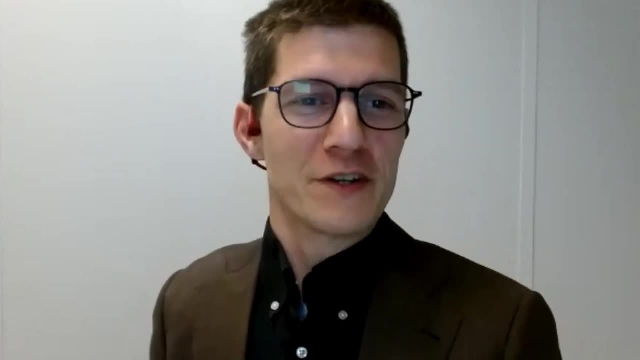 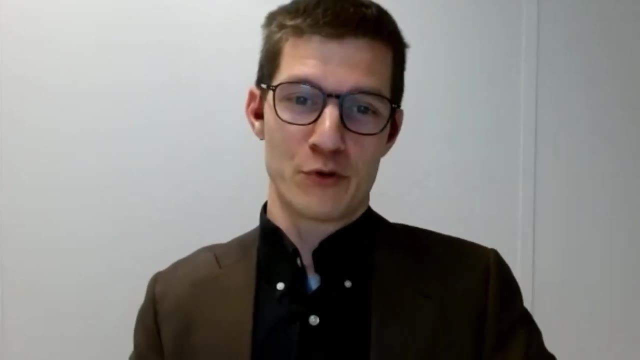 Bye, bye. Thank you, Henk, or virtual Henk, for this introduction, And I'm still humbly amazed to hear that we are growing with such large numbers, And I hope too to meet you in person rather sooner than later. 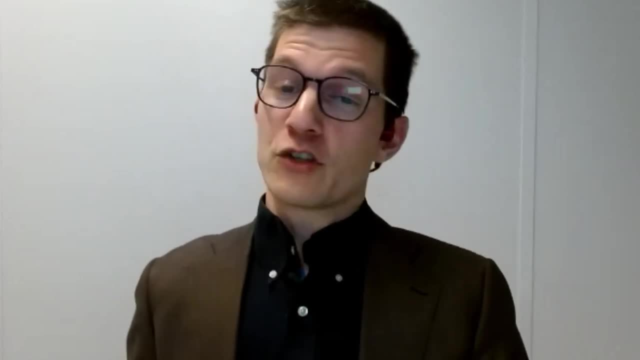 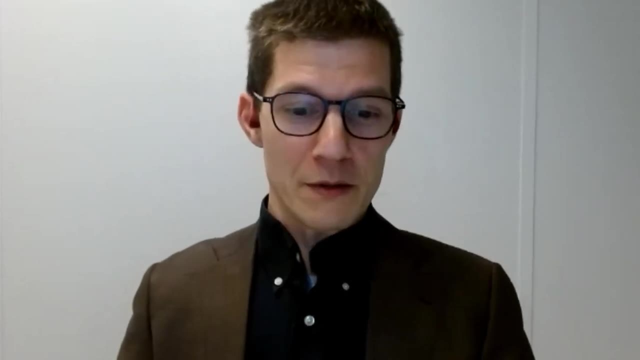 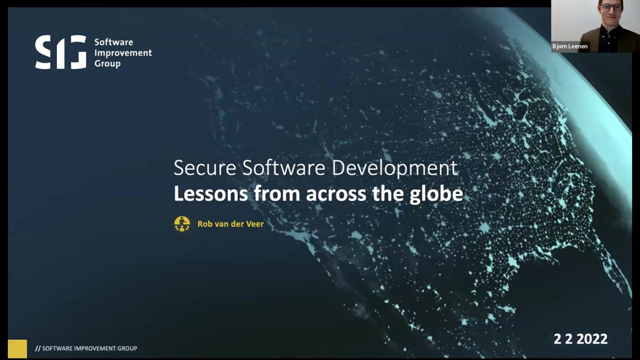 So the first speaker of tonight is Rob van der Veer, And the subject of his presentation is secure software development lessons from across the globe. Rob, would you be please so kind to turn on your webcam and audio and take the stage and share your presentation. 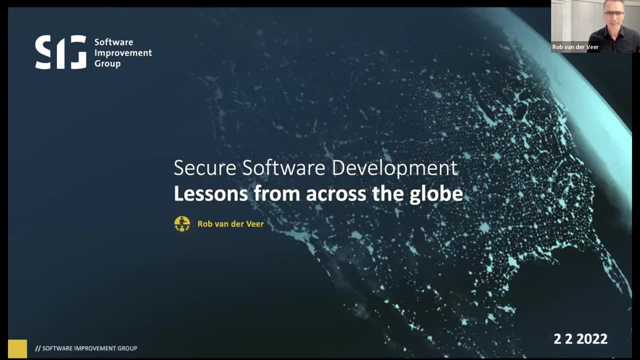 Yes, I should be live and visible. Thank you. First of all, a message to Brenda, who I know very well as we've worked closely together. Congratulations to becoming president. Congratulations to becoming president, I'm sure it will be a success. 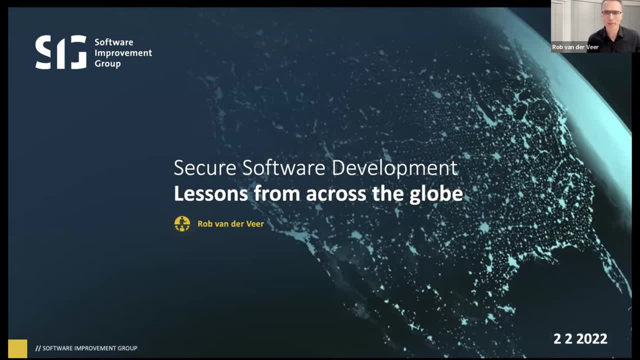 And thank you, IC Square, for having Martin and me here today to talk about secure software development. In this session. I would like to share with you some experiences while working with clients and doing research, And first I will go into the story of how software security typically evolves in organizations in order to highlight some of the pitfalls and how to deal with them. 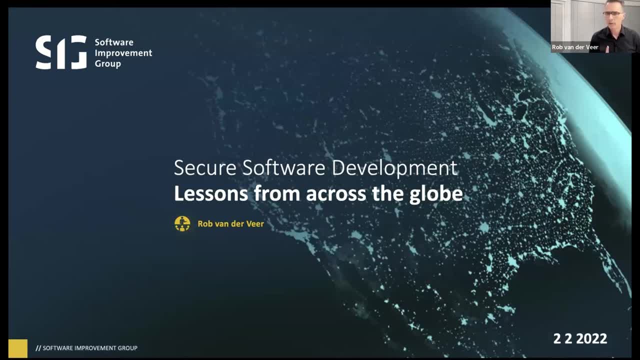 And you will see that it is actually a love story, by the way. Then I will discuss the most important lessons as building blocks for success. After that, Martin will take over, followed by room for questions with Martin and me. You ready? 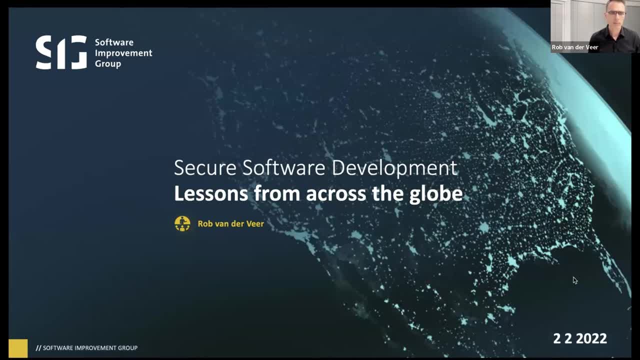 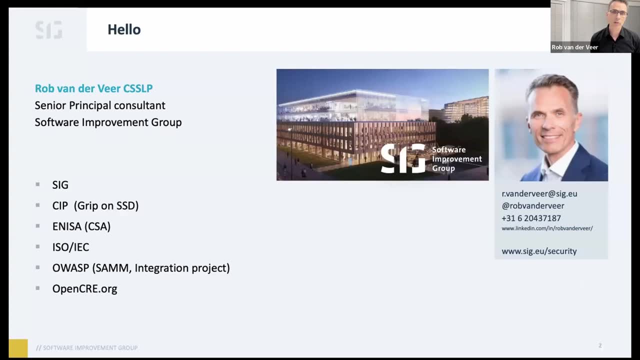 Let's go First. let's start with a little introduction. Hello, I'm Rob. I like to build bridges. I do this in organizations and in the fields of security and artificial intelligence. I work for a software improvement group, SIG. 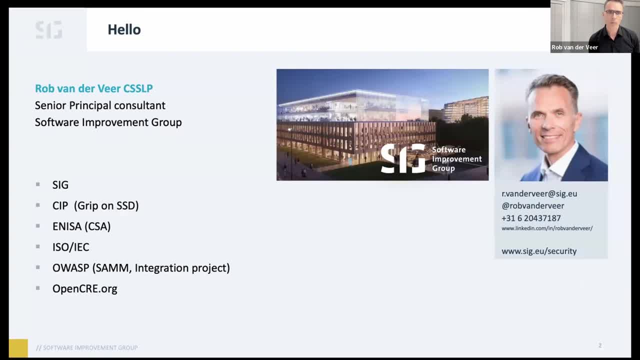 Where I started the security practice about nine years ago. If you don't know us, SIG measures software quality, maintainability, security, privacy and more to help organizations to get software right. We advise them, We guide them And, if they want, we can provide our platform to analyze and control software quality. 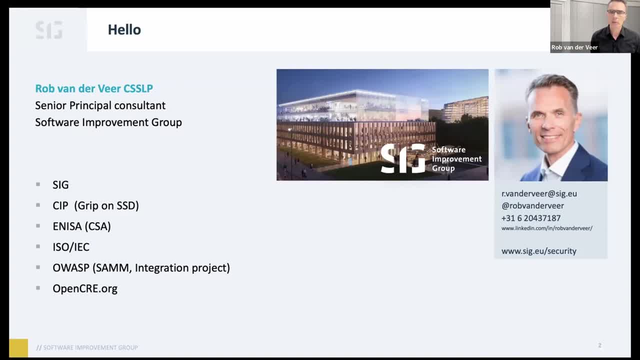 Apart from SIG, I'm also involved in several initiatives to help grow these fields. I'm the chairman of the Groupon secure software development staff. I advise the European Commission. I'm an active contributor to standards at ISO and work for OWASP, part of SAM, co-leader of the integration project at OWASP and founding father of opensiriorg. 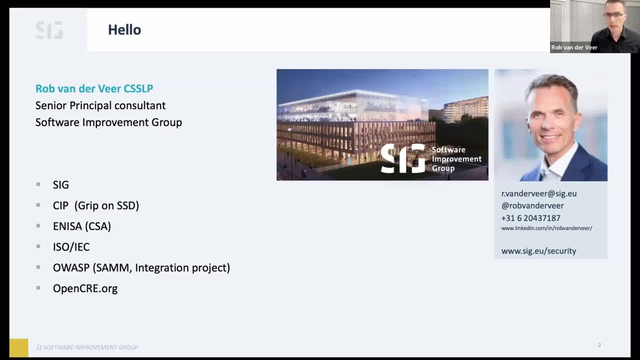 Now you may wonder why I do all these things, And the answer is simple: I'd like to earn CPE credits, of course, for my CSSLP. So let's go and have a look at the phases organizations go through with secure software development. 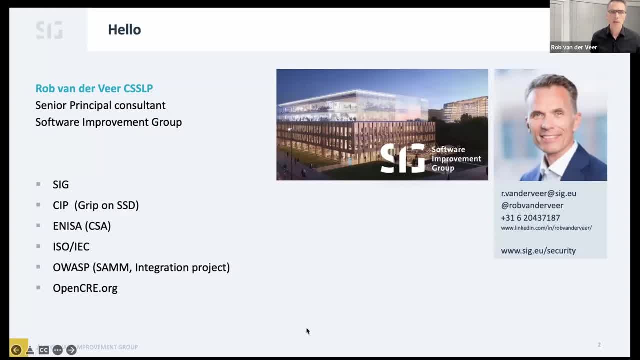 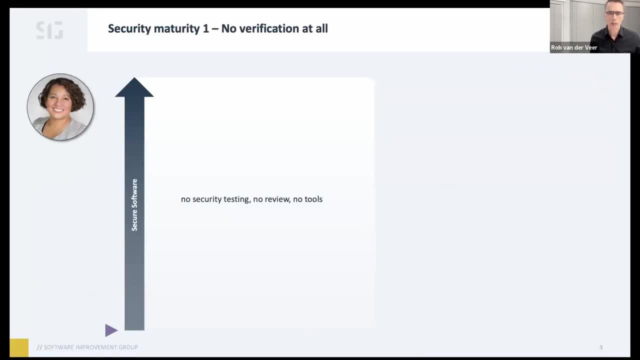 It's the story that starts with security. I'm the development manager, Elizabeth. In the beginning there was nothing. This is security maturity, stage one. Elizabeth is building software and basically just hopes that it's secure, But she doesn't know. 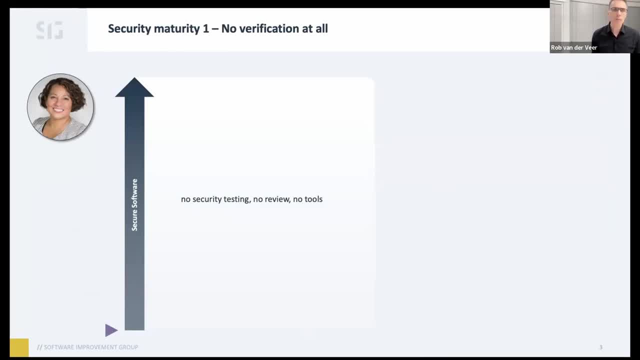 There is no security testing, no review, no tools. And then one day a man comes along called Darcy- Hello, Mr Darcy. And when their eyes lock, Darcy blushes and Elizabeth's heart skips a beat. Then, in a strict voice, he suddenly tells Elizabeth that there has been a scary data bridge. 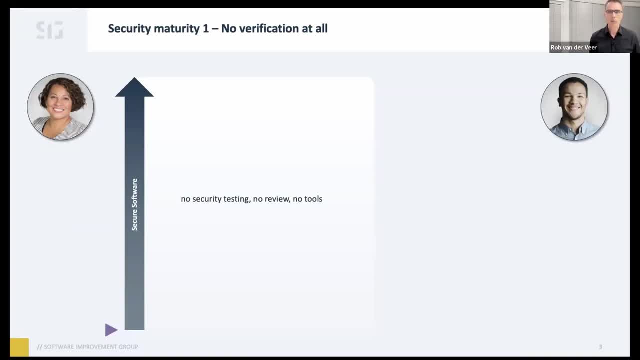 And from now on, security needs to be tested, Which brings them to maturity, stage two. They start testing, They look for some tools together to do network scanning and some automated testing of the application, And they quickly find that it's a good idea to have actual hackers try to break into their system. 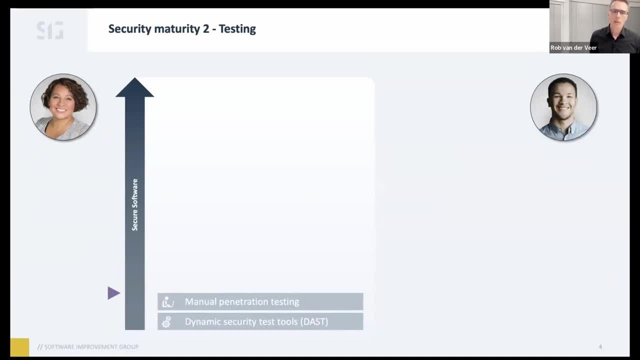 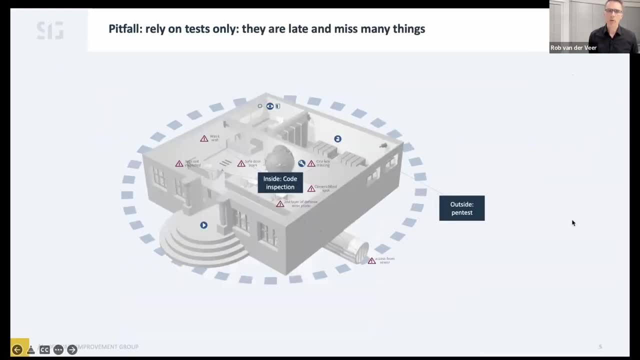 We call this manual penetration testing mostly, And this provides them with some good insights. Definitely, However, over time they learn it is a pitfall to rely on tests. only Pen tests are useful, But they can only be done very late in the development phase. 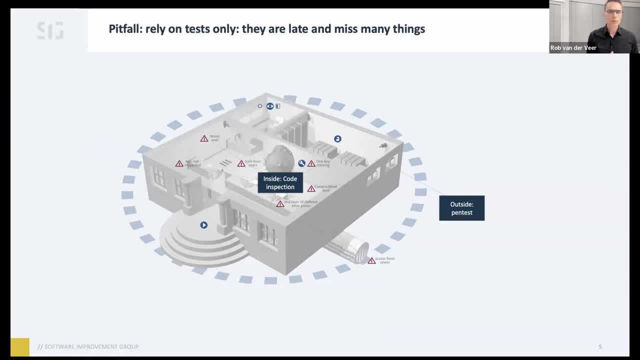 And they only find part of the issues. Here you see a computer system visualized as a bank building. Penetration testing is about trying to get in from the outside, But because you're not investigating the inside, you can miss a lot of things. 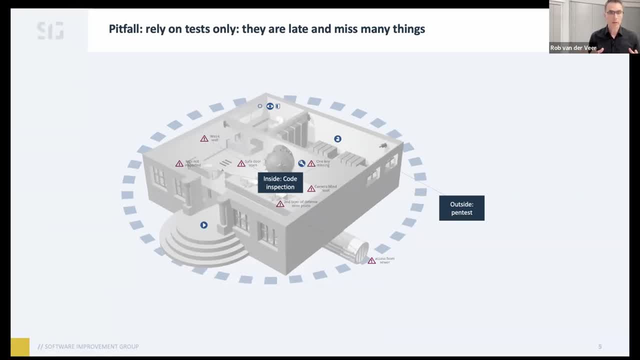 For example, That the safe door is actually open Or that passwords are stored unencrypted Because you can't break into the system. now. you don't see these issues, But the best thing to do is to assume that at some point people will break in. 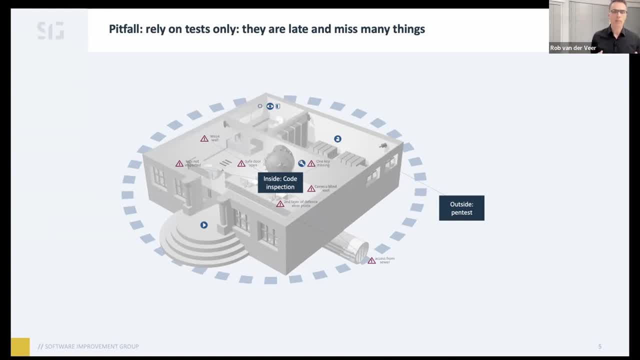 And that's when you need security to be really built in your system. So pen testing is useful, But we also need to realize that you can't see everything And also that you can't try everything. A pen test is a time box in which hackers try different things to break in. 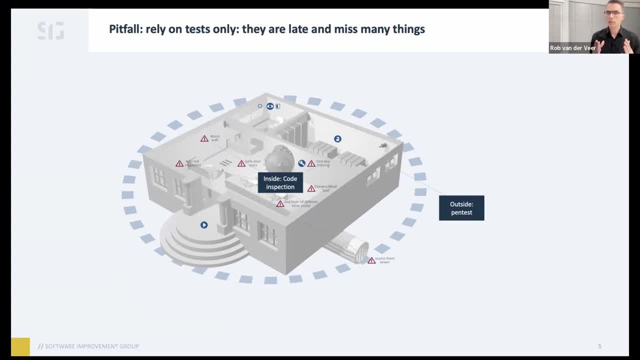 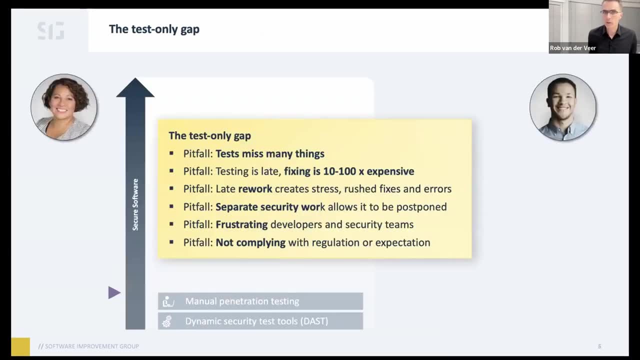 And when the time is up, they have not run out of options, Just out of time. So Elizabeth and Darcy have a problem now that I call the test-only gap. First of all, like I said, tests miss many things. Personal data leaks. 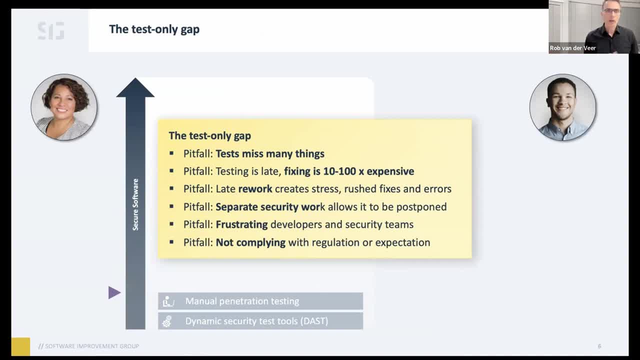 Sent unprotected to another system. Logging is missing, All stuff under the hood. that is wrong and presents a weakness. But there's more: Because it's late these tests, Elizabeth needs to fix the found issues once the system is already done, And it's a lot of rework. 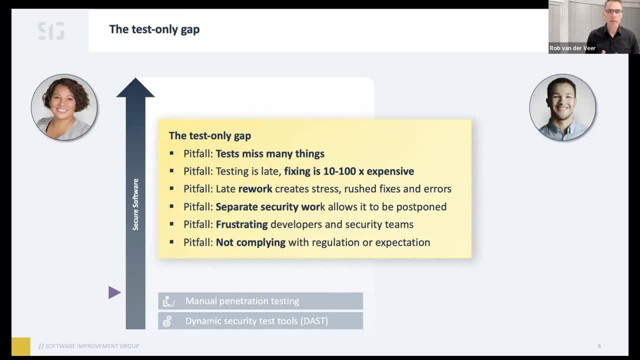 She has to change all locations where database queries were built to prevent SQL injection. Her boss is not happy Because that rework is typically expensive. Why didn't she do it right in the first place? Now Elizabeth is stressed because she needs to release. 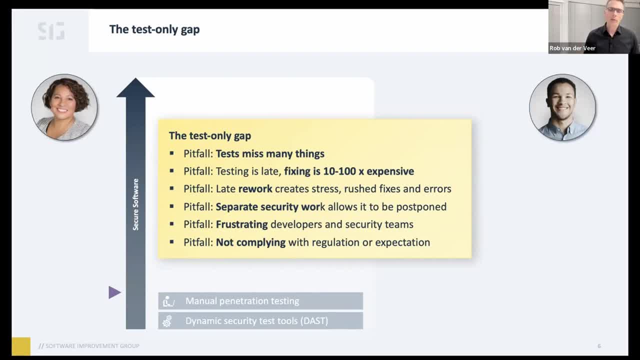 So she rushes the fixes as best as she can And unfortunately makes some mistakes along the way And also part of the work is postponed for later. The result is that the software is not secure. Too much effort is spent. Both Darcy and Elizabeth are frustrated. 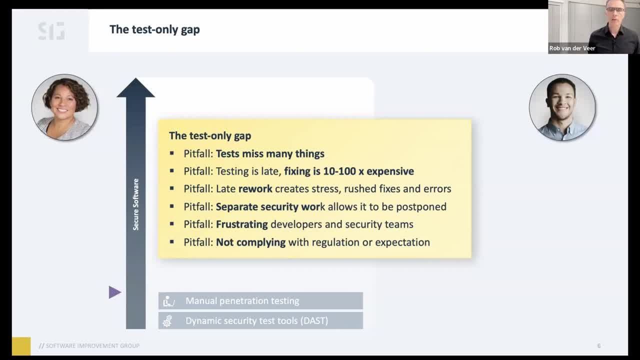 They realize they need to get it right at the start, And this is a growing realization, Not just with developers, but in the market. We definitely see this. You are increasingly expected to build security in from the start, Called security by design sometimes. 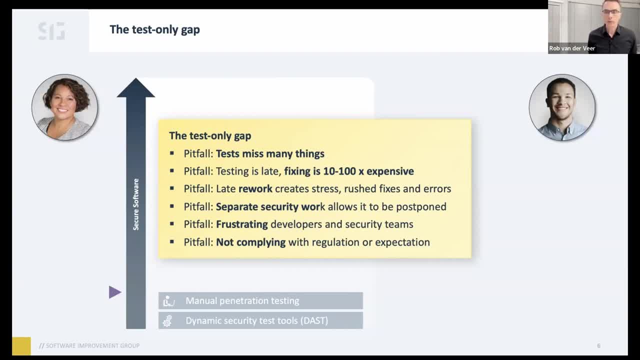 Shifting left, And this is a big problem. We have a lot of regulations that require it: The GDPR, for example, The bio government security standard in the Netherlands, The payment card industry security standard. And if you don't, you are going to pay a larger price if a breach reveals the engineering was bad. 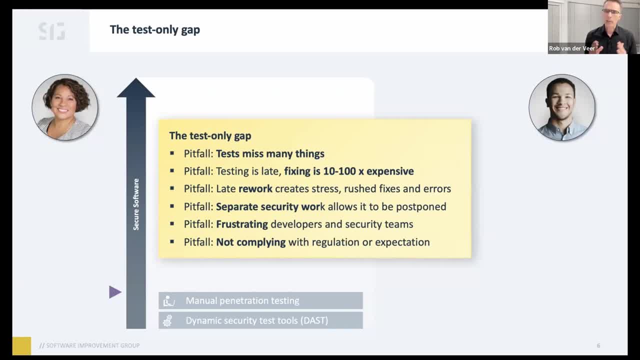 Look at Zoom. The reason that they faced so much criticism is not, per se, the fact that there were security issues. It's the severity of those issues And the negligence of the development teams In the meantime. by the way, There is a lot of work that needs to be done. 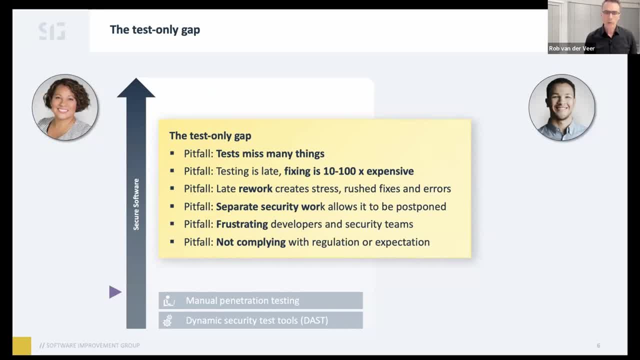 So Elizabeth and Darcy have more than enough reasons to work closer together to build security in for shifting left, Starting early and seriously with security in the software development process. It's today's best practice and increasingly regarded as duty of care. But how do you make it work? 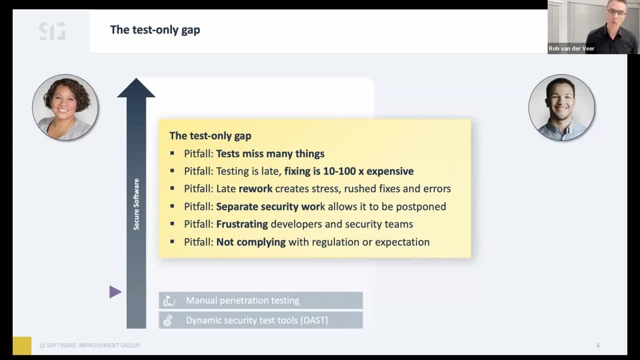 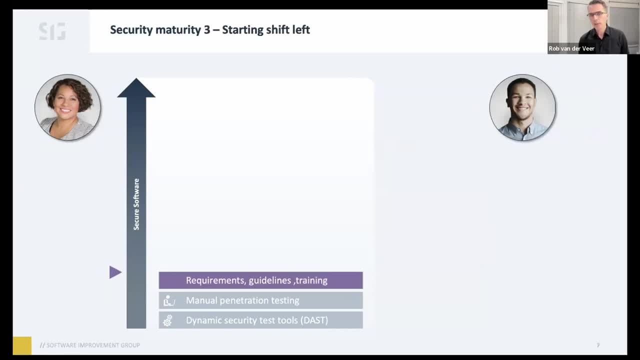 Spoiler. it's not easy. It's just like with love: We all need it, but it's never easy. It leads us to maturity, stage three. They start building security in Great. How to start? Well, Darcy came up with an idea. 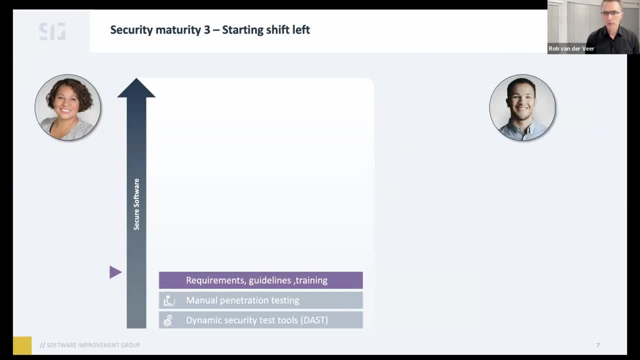 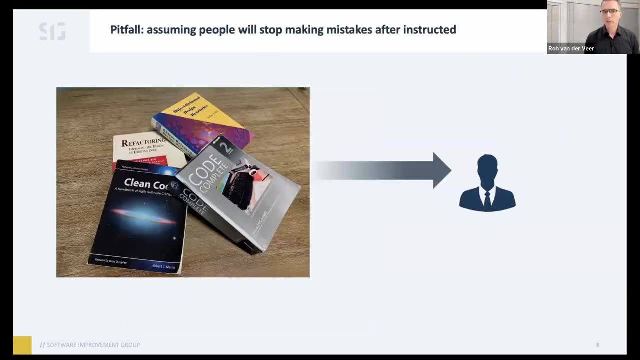 He presents Elizabeth with long lists of security requirements, Some books with coding guidelines And some training for the developers. Elizabeth appreciates the idea. However, after some time, developers are still making mistakes. They got the books on their desks And Darcy put 400 security criteria on the wiki. 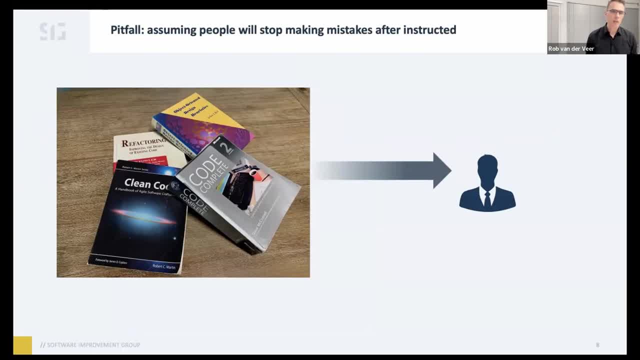 A lot of work, But they still make mistakes, Turns out there's too much to remember, And they're only human, of course. But Darcy has an idea. He proposes to start applying threat modeling. Let Elizabeth discuss with her team what could go wrong. 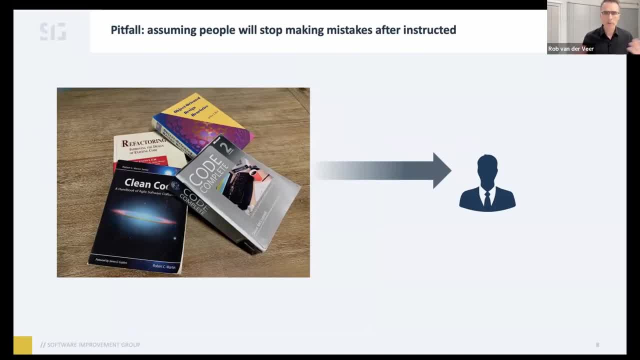 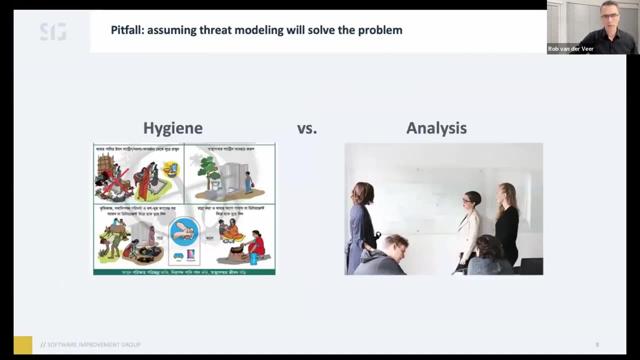 With a whiteboard in a room, Think about things that could happen, Threats to their system, Looking at the architecture, And then decide what to do against it. That will create the right requirements automatically. It sounds nice. However, Elizabeth notices that she and her team come up with some useful threats. 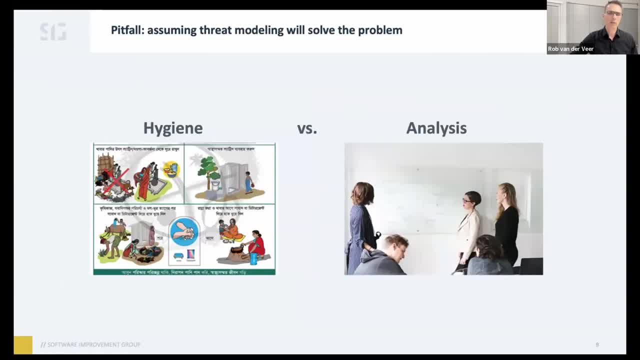 But Darcy finds they miss a lot of the issues. And then when Darcy joins the threat modeling session to see how it's going And to show them how it's done, He notices that even he misses a number, Even he misses a number of important things. 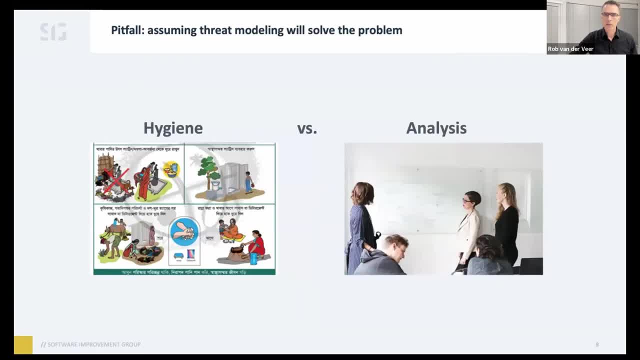 They conclude that threat modeling is useful for the team to understand the security of the system better And it can help to identify some additional requirements, But for the most part the hygiene approach is more effective, And with hygiene approach I mean the long list of requirements, of things that you need to do to gain secure software. 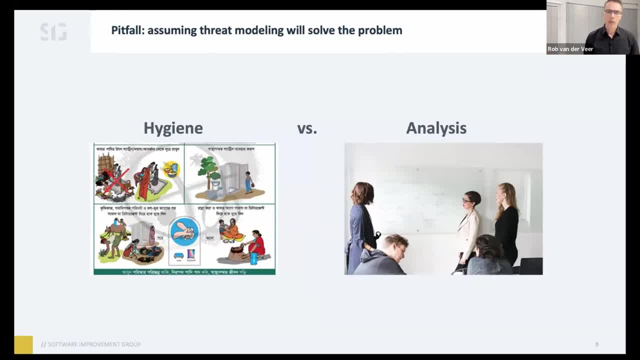 Like wash your hands before you eat food. So people are not perfect And neither is threat modeling. Slightly disillusioned, Darcy and Elizabeth conclude that the work of the teams need to be checked while they are developing, So during developing. 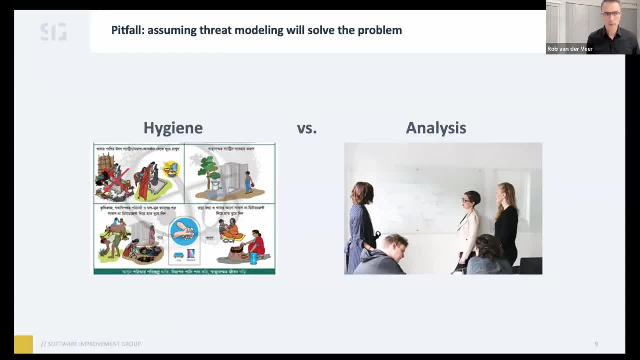 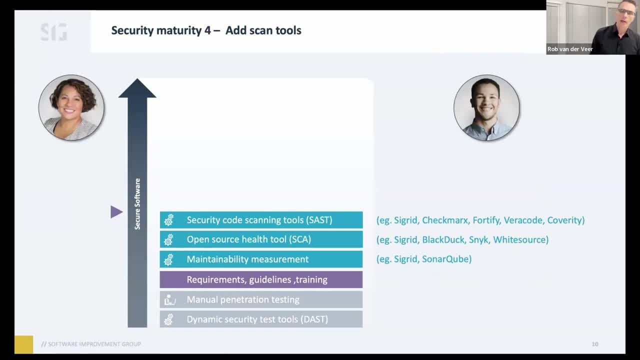 The feedback loop Which brings them to the next maturity stage, Maturity 4.. They download and buy some tools to scan the code And to detect weaknesses as developers introduce them. Some tools for maintenance, Tools for maintainability, To measure code quality. 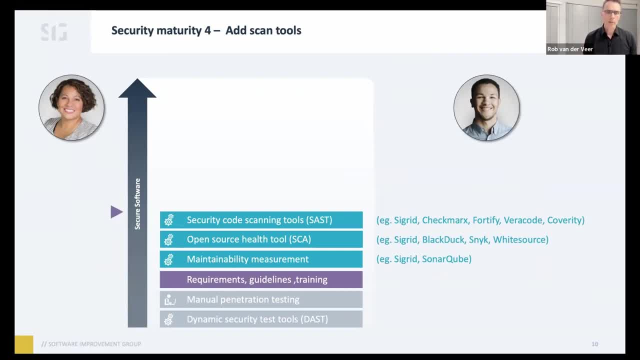 Because complexity is actually one of the main enemies of security Tools to scan for open source vulnerabilities. Mostly they are called software composition analysis tools- Well, at least the analysts call them that way. Sometimes you see them called dependency management tools. It has to do with the software bill of material. 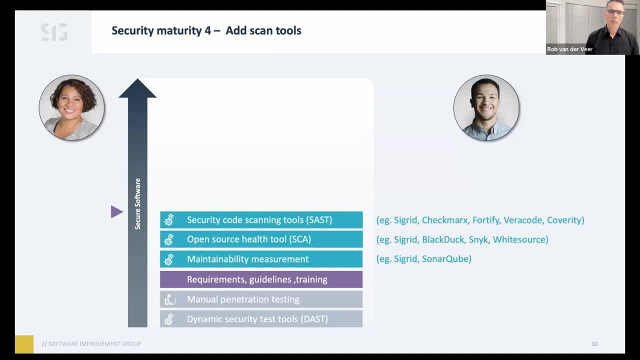 The famous SBOM, And, of course, Medical analysis of code tools, Also called SAST tools, Maybe different ones for different technologies. But then they have the tools, They are installed, But Elizabeth's team is a bit hesitant to start using them. 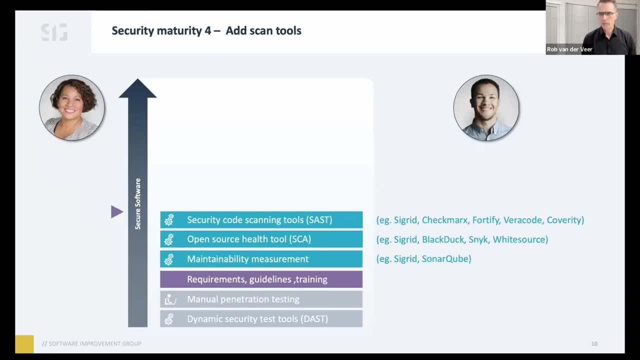 And they are somewhat overwhelmed by all the output that comes out of it. Some first efforts show that there were useful findings, But Elizabeth and Darcy are really struggling to make it really work in practice. Adoption seems to fail. Having tools is one thing. 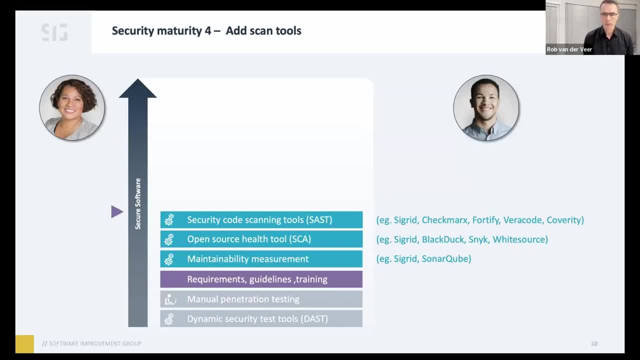 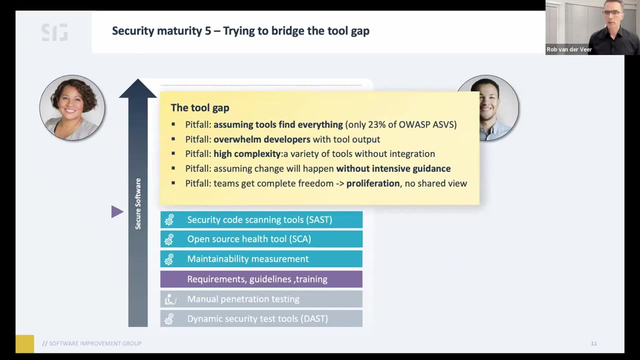 Making people use them effectively is another. They suffer from the so-called tool gap, Which brings them to maturity stage 5.. You see, the tools are nice, But they miss a large part of the weaknesses, Just like pen tests do, For example. 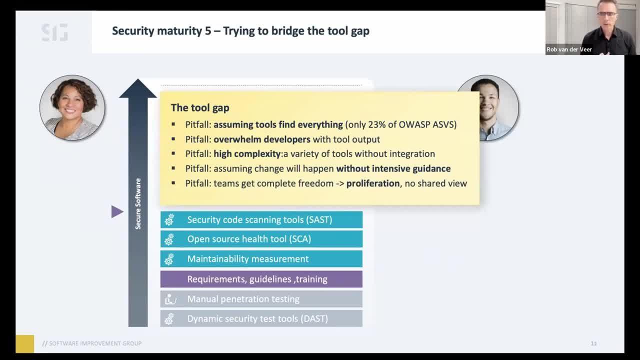 Many of you probably know the OWASP ASVS stack. It's basically a long list, Quite comprehensive, Of checks for secure software. It turns out that only 23% of these checks are checkable with tools only, So tools, for example, cannot see what is not there. 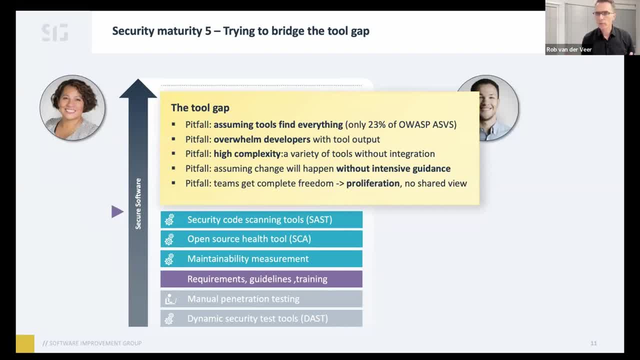 And the fact that something is not there is often the problem: Missing authorization, Validation, Logging, Encryption. Also, it's hard for tools to interpret business logic If I ask, for example, For somebody's password And then check it. 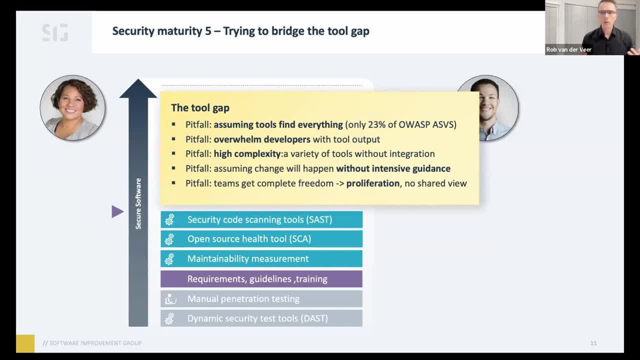 But even if it's wrong, I still let. users in A tool will not detect that And these tools will warn you for SQL injection risks If they believe there is no validation of user input. But they're not sure, Which means the tools can provide hints. 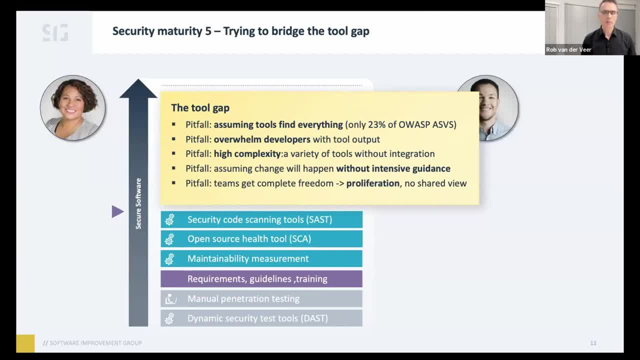 But Elizabeth and her team still need to analyze many of the findings manually. And then there's the issue that there are multiple tools That Elizabeth and her team need to learn how to use, And they all have different reports and interfaces And they need help with that. 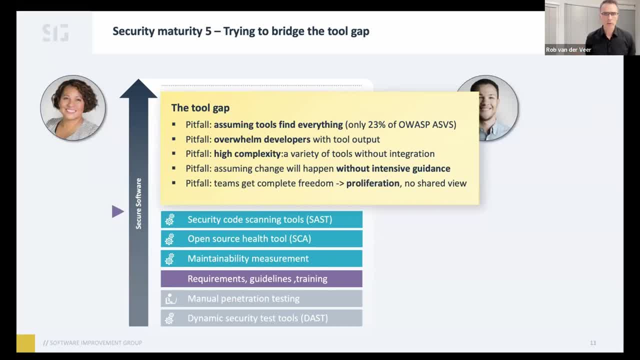 And also help with trying to make it work in your organization, Trying to get people aligned, Trying to get the right knowledge, And what these tools cannot offer, obviously, is some coaching and organization guidance, And then, to make matters worse, If you have multiple teams, 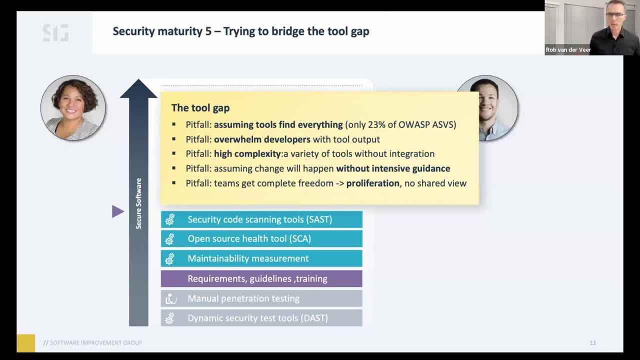 And you give them complete autonomy And freedom To decide what tools to use And how they're going to use it, It will lead to proliferation And fragmentation of choices. There are different approaches, Different tools And different workflow, So team autonomy is very important. 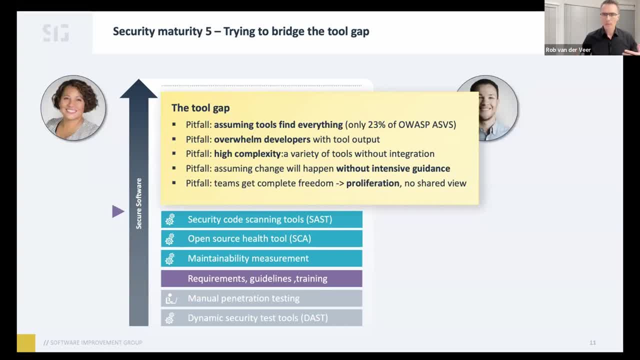 But when you go too far, You basically increase all these problems that have just gone through. And this stage is where we find most organizations. Most organizations are in, They got the tools And they're facing these very tough problems. And if you do it wrong in a first attempt, 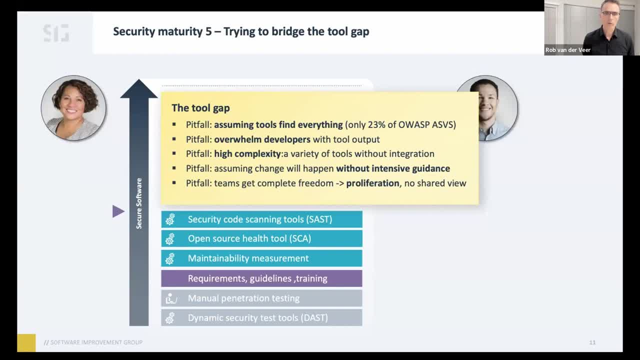 It will only get more difficult to get everybody along. So first time right is your best bet, And that even makes it more difficult. I know very little organizations that have bridged these gaps Completely by themselves. If you've done so, perhaps with some help. 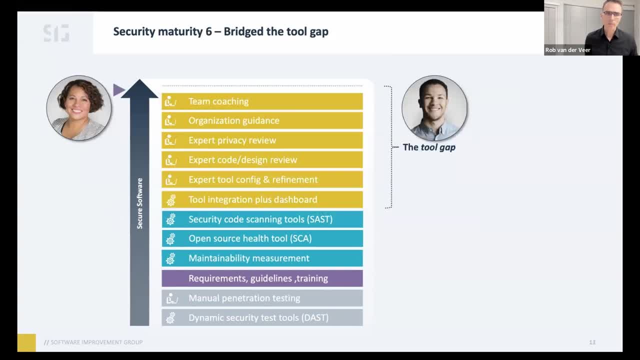 You reach maturity six And what this means is that you've bridged the tool gap. You solved all these problems that I just discussed. You integrate the results from the tools in a single point of truth For developers and for stakeholders. This single pain is really important to have actually a shared view of what findings are. 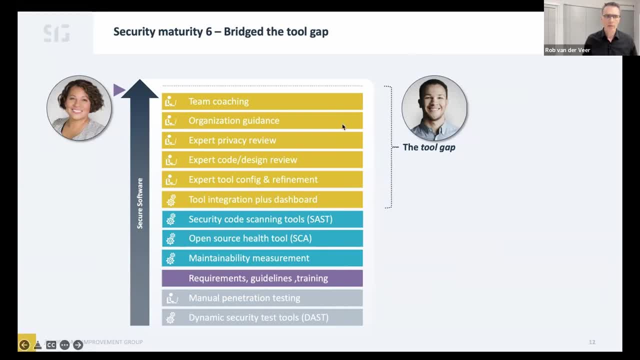 And what their status is. Then you have experts helping you With tool configuration And interpretation of the findings: Prioritizing them, Filtering them, Explaining them. Teams typically need help with that, Especially in the beginning. Then you have experts doing code and design review. 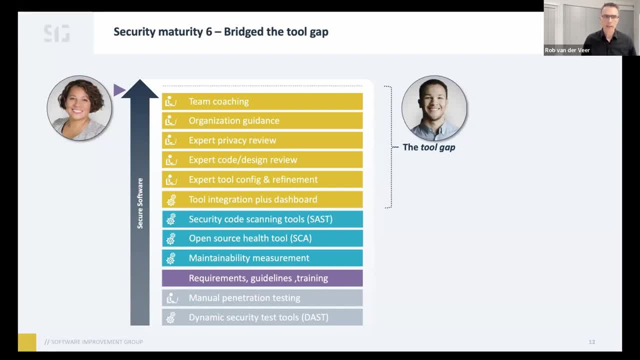 Or at least supporting that with their expertise And ideally also privacy by design reviews. And then you also need experts providing guidance to developers, Providing guidance to the organization And making this change And coaching the teams on building security in This whole stack of things requires a lot from these experts. 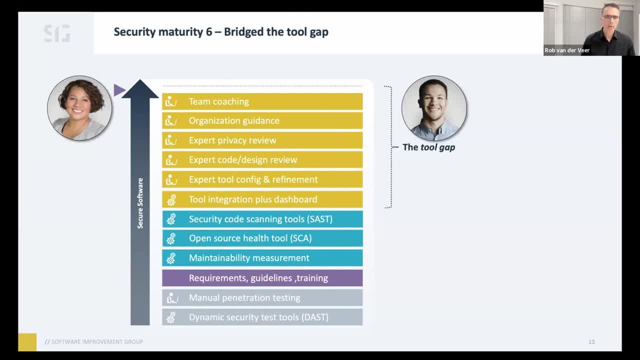 Security knowledge Tool, mastery, Coaching abilities, Organization sensitivity, Technology insight, Code review ability, Programming expertise, Management, consultancy capabilities. And they need to be culture changers And have the right And soft skills. Such experts are hard to find. 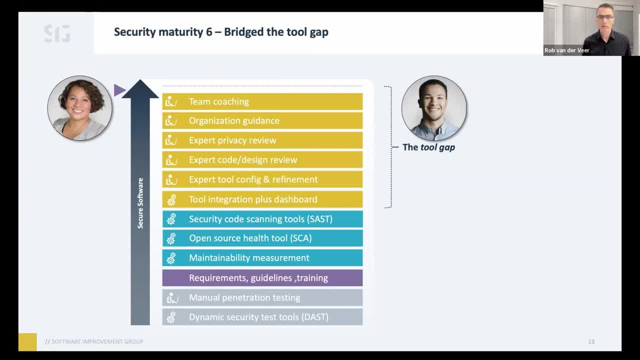 And hard to keep. And there you have it: The sheer number of things that you need to get right And their complexity. They highlight the key problem, As far as I'm concerned, in today's secure software development. The key problem is the underestimation of how much work it is to get it right. 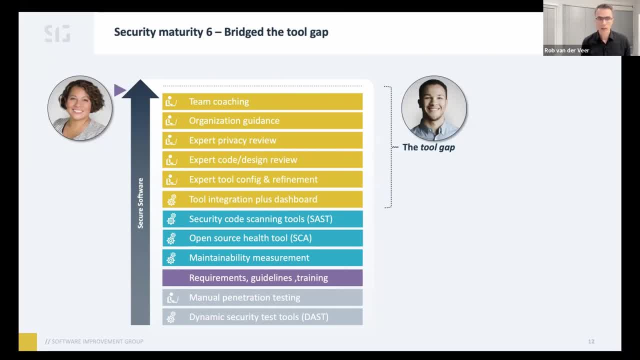 Let alone first time right. Secure software development is not a matter of buying some books, Getting treated for it, getting training and get some tools. It's an organizational change program that requires investing attention, time and money, And then it can be done so that Elisabeth. 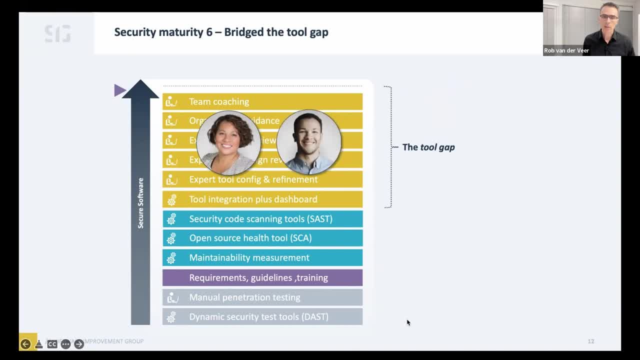 and Darcy can work closely together and live happily after after. Well, what is it exactly that Elisabeth and Darcy need to get right? Let me take you through some great lessons learned- key building blocks of successful, secure software development. Starting with, everybody should own the problem. 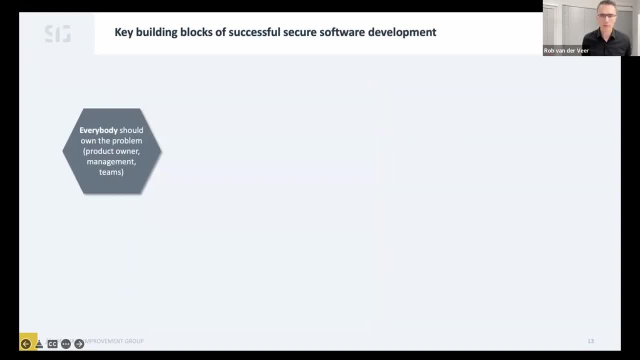 That's the basics. If you don't have that, you're going to have a really hard time. Organization buy-in is key And there are some tricks to achieve it, And I would say: never waste a good crisis, security breaches, incidents. they really help to gain traction. I'm not saying 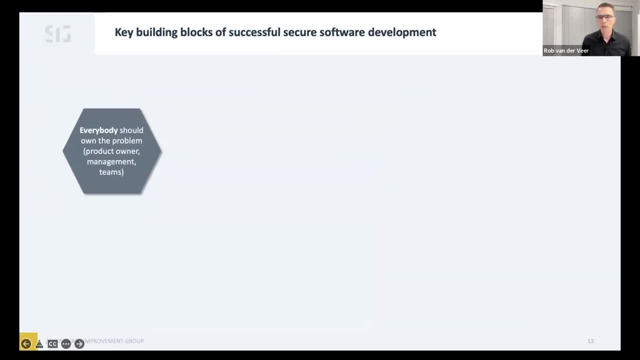 it's a good thing, but it's a good thing, And it's a good thing, And it's a good thing, but it's should create them. I should say that you should embrace them in the sense that, of course, deal. 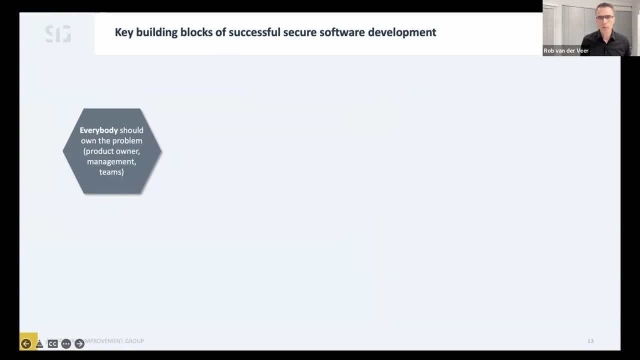 with them and then use them to gain traction with the importance of security. You can also do a software inspection on one of the systems to provide some evidence of weaknesses in the software. Really demonstrate the things that are wrong and the blind spot in the organization That. 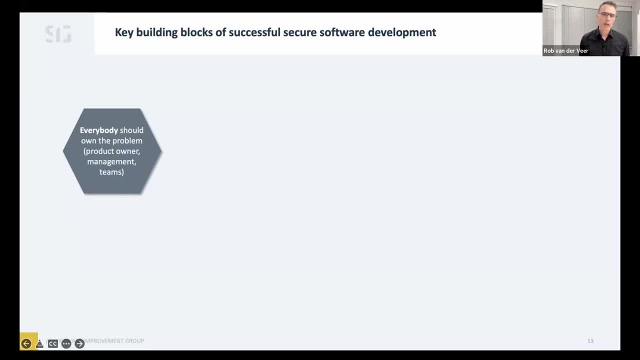 creates incentive. Another way to get started is to perform a base measurement, not of the security in the software but of the security in the organization, The processes that are in place, and compare that to some framework. I like, for example, the OWASP SAM initiative. 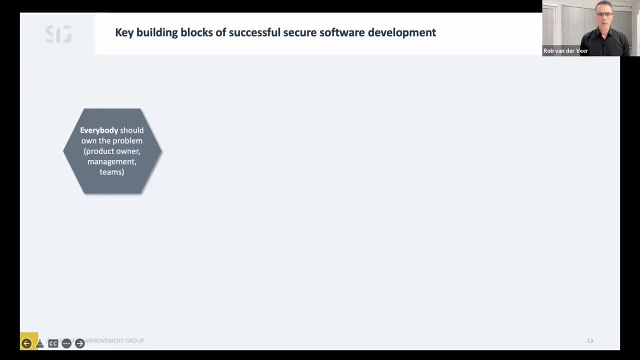 S-A-M-M, which provides an overview, a framework of processes, of controls, process controls basically, and their maturity levels, And you also get, with OWASP SAM, some tools to do self-assessment and to see where you are and what steps you need. 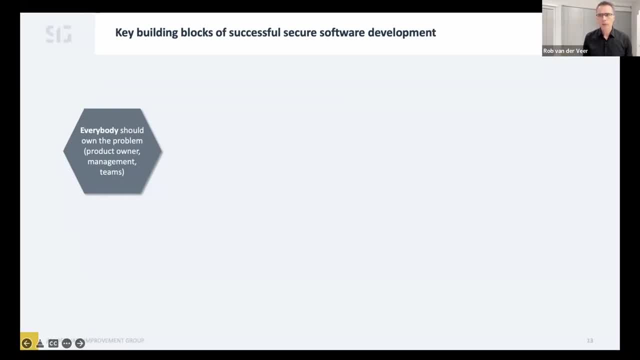 to take in order to improve And doing such a base measurement can highlight that a lot of work needs to be done in order to attain some level of appropriate control of security. Another organization aspect is that security experts and developers. they will need to collaborate. 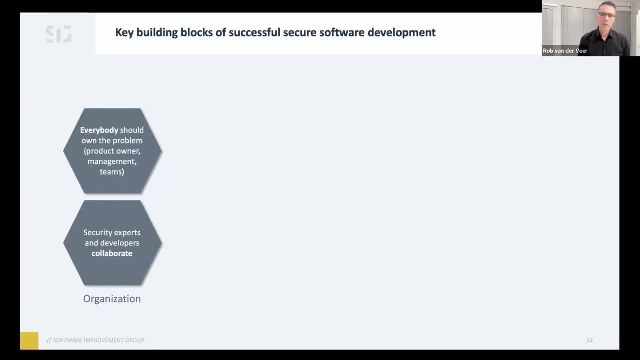 Well, just like Elizabethan Darcy did in the end, A good way to facilitate this is to put them together in a room, for example, when development work is prepared, instead of only discussing tests after the fact. Security teams will transform from quality gate to coaches of development. 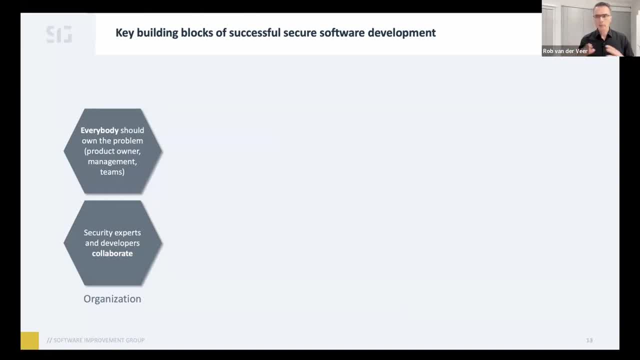 teams almost automatically as the organization goes through the maturity stages that we just discussed. Another good way to create awareness in an organization, to increase that sense of ownership, is tailored training. Provide teams, and not just development teams, but also involving product owners, for example, or architects. Provide them with training that is relevant for 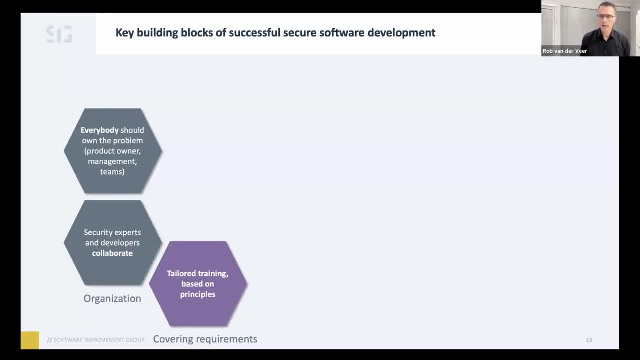 their context, their domain and their technology stack, not just a generic training. This will help them to start covering some of the challenges that they face in the future. This will help them to start covering some of the challenges that they face in the future. Another good way to create awareness. 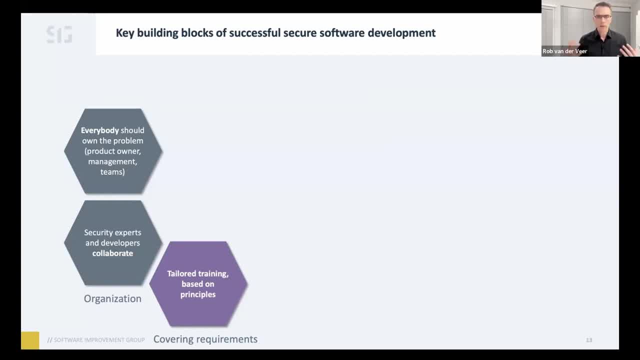 covering security requirements. It's actually one way to prepare them, share the principles with them that they need in covering these requirements And to further cover requirements. you want as many of them dealt with by the building blocks that you have: the frameworks, the libraries, the enterprise architecture. 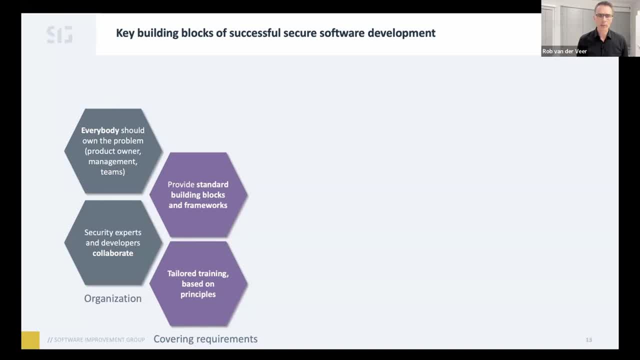 You want to take care of as much of the security issues by providing these, because it strongly reduces the number of requirements that the development teams need to take into account. And talking about taking into account, what remains are requirements that need to be applied, And the trick is to make them as situational as possible. 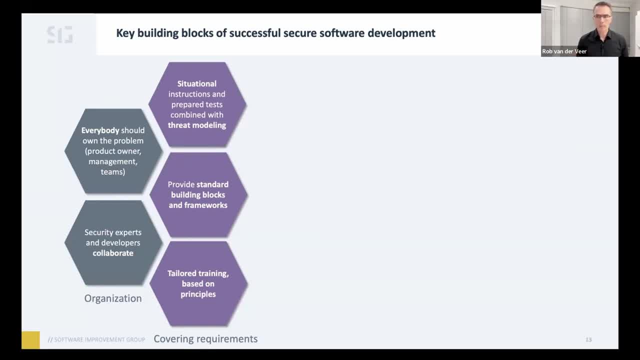 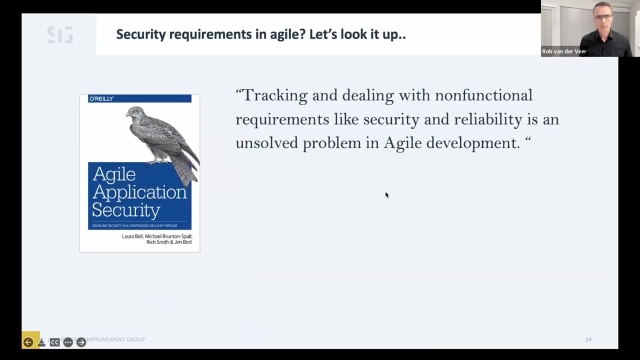 And to have tests ready and prepared so they can be quickly deployed. This is the only way to make secure software development work and be part of the structure, the development flow. Really important. Let's have a look at how that can work. First, I try to look it up. This is one of the most popular books on the topic of agile. 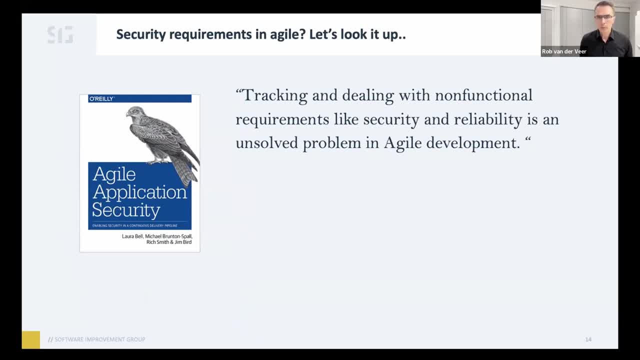 application security. What do the books say Well about security requirements? it basically says we don't know. This problem has not been solved yet, which is interesting. If you're doing stuff in this area- and we're doing a lot of this- it's actually bleeding edge. 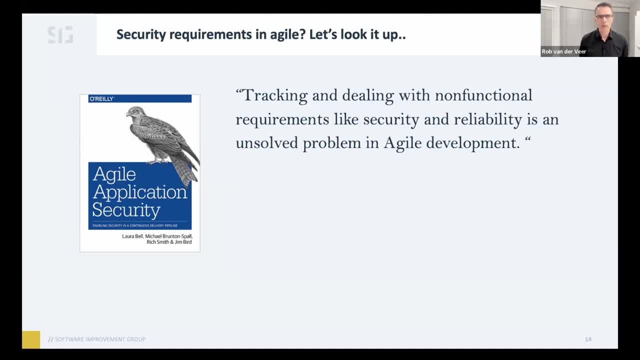 The thing that sounds so simple, just following a set of requirements, it's actually quite difficult to make happen in reality. There's so much for looking it up. There is some guidance available as part of the agile guidance of OWASP, SAM, and I have a link for you later on. 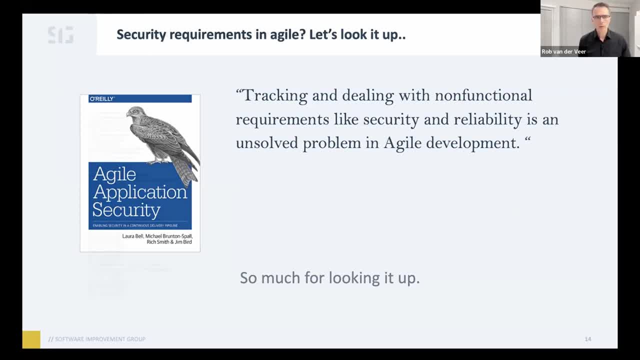 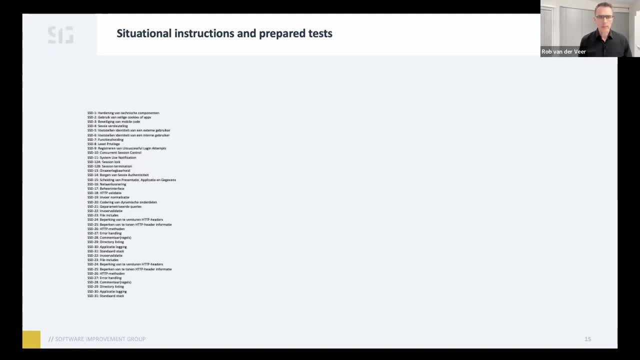 And regarding the requirements, it follows these ideas. There's a list of requirements that you want to apply. The key is to minimize the daily instructions that developers need to work with and to let as many as possible depend on the type of task they are working on. That's what situational means in this. 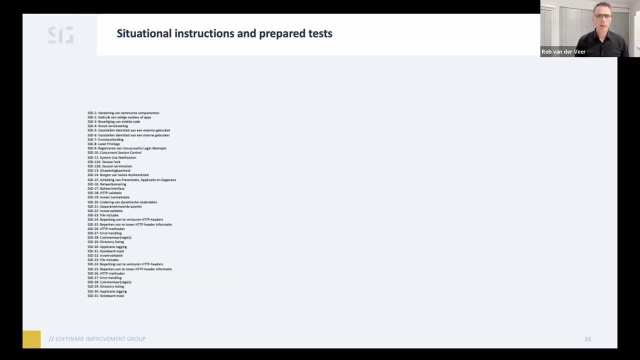 case. Only then such a list can be effective, because no one can learn this by heart and apply this consistently. And this is because, unlike functional requirements, security requirements are cross-cutting concerns In many cases. you need to constantly think about them, whereas a functional requirement 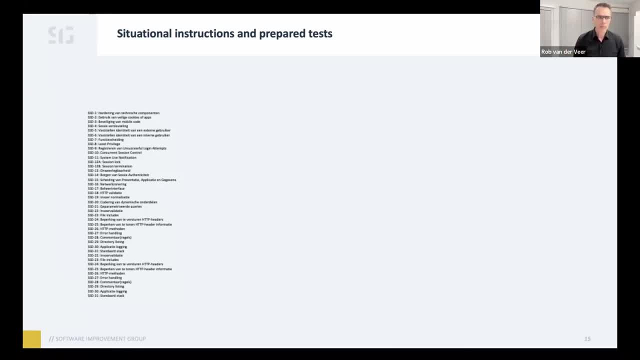 you can go one by one and cover them. Non-functional requirements, like many security requirements, are things that you need to take into account constantly, And that's the whole difficulty. So you see the long list of requirements, But you can do a couple of things. You can first remove a few as they're not applicable to the team. 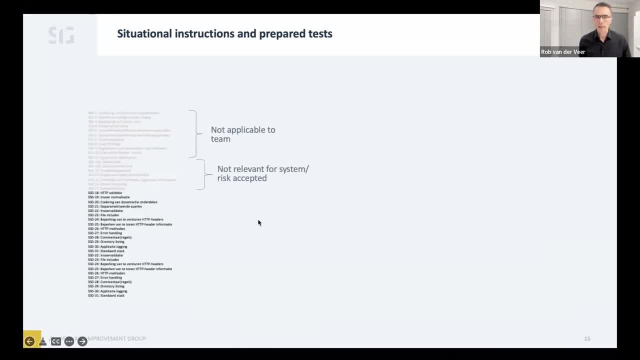 Then you can remove some more that are not relevant for the application, And even more, like I said, done by the framework, done by the building blocks that you provide. So the only thing you need to take care of is that the development teams are actually using those frameworks and building blocks. 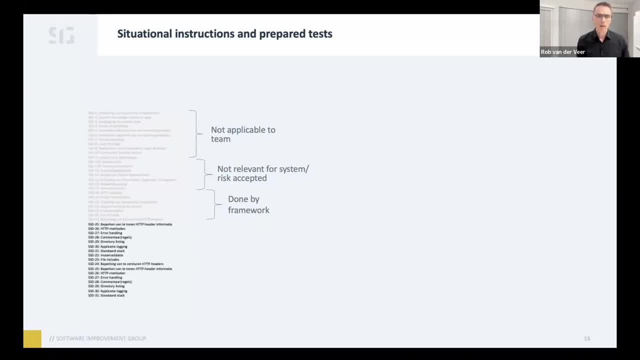 So that's something that you need to test for. Next are requirements that are what you can call story-specific, So they are dependent on the type of work that you do. For example, you're going to work with XML input, Then there's a set of requirements that you need to take into account because of that. 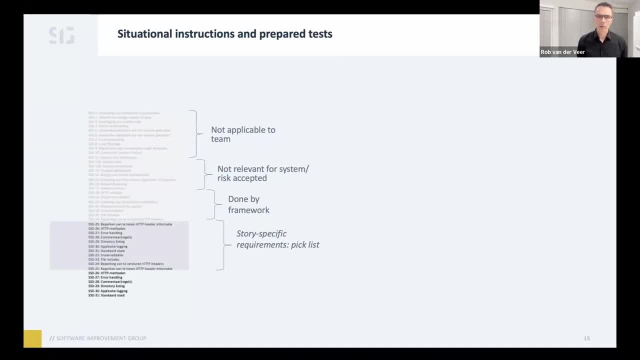 Or file uploads, Or you're going to output data, And we call these triggers, And these triggers help you select the right requirements, depending on your story, the thing that you will be working on And what it provides. the requirement is a set of instructions that are written in the language that's helpful for development teams. 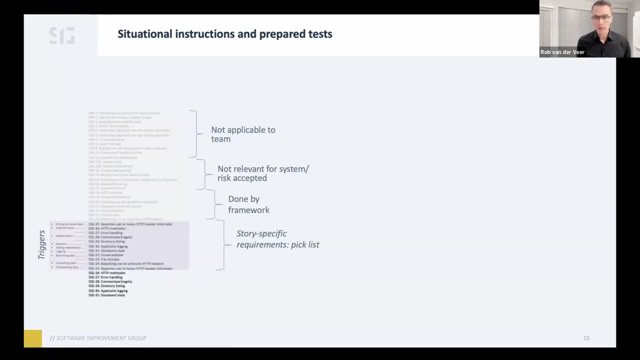 And not just instructions but also some tests, And they work as acceptance criteria for the story. So the nice thing is, because you're building something that has XML input, you're getting the appropriate instructions, but you're also getting the tests that go along with it, that, as an organization, you've prepared. 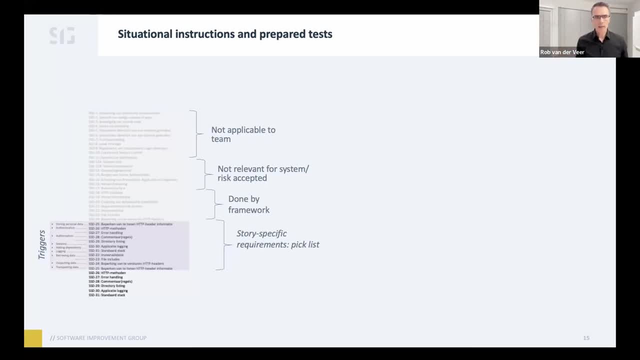 And they become part of the acceptance criteria. So, automatically, security becomes part of your development and testing flow. The requirements that remain- they are generic requirements. You want this list, of course, to be as small as possible, because they have to be applied constantly. 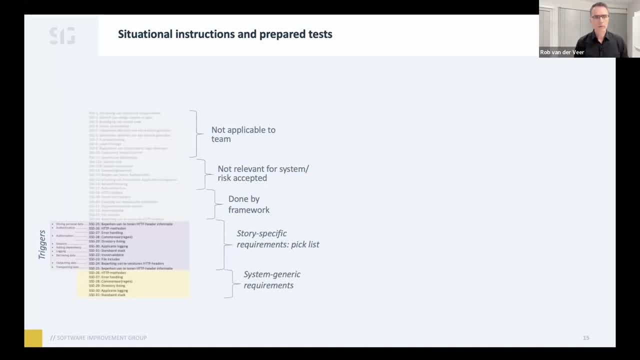 And you also want these generic requirements to be really testable, preferably because you don't want any of these to slip between the cracks. They represent instructions that developers really need to master and test, that always need to be performed as part of 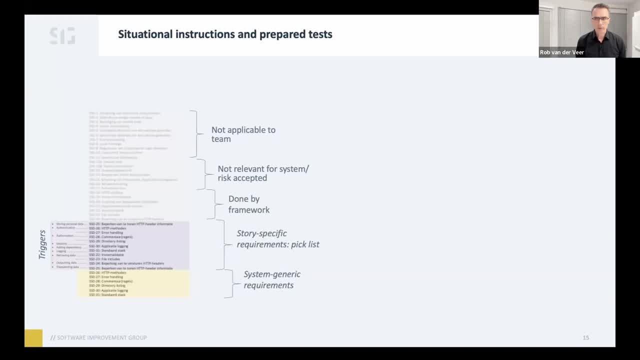 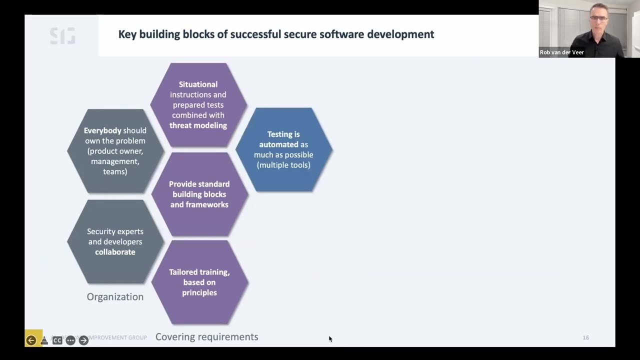 and I'm bringing in Scrum Agile again. definition of done. That's the way how you want to go about the system: generic requirements After requirements. of course you want to automate that testing as much as possible, But as said tools are not going to cut it, 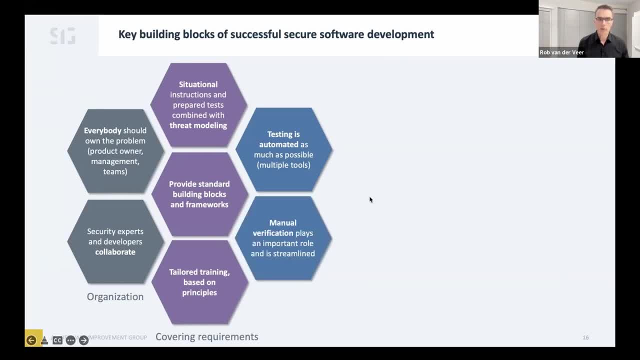 So there needs to be good attention for code review and manual verification, And you want to do that manual verification in a streamlined fashion because you have to do it all the time, For example, by having clear checklists with every requirement. Now the pick list, the triggers that I discussed. 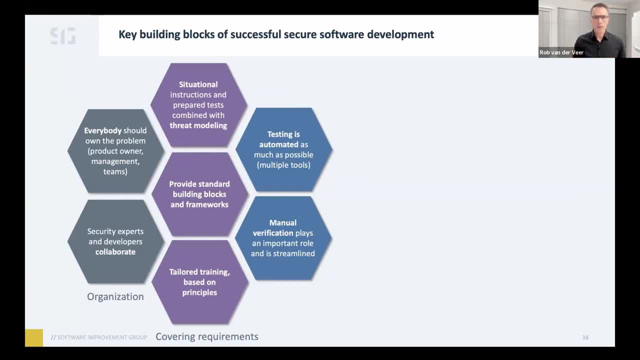 that bring you the really specific requirements, the instructions and the tests. The tests include checklists for code reviewers, So part of the acceptance criteria is a checklist of things that need to be checked through code review, So you don't have to code review the entire application. 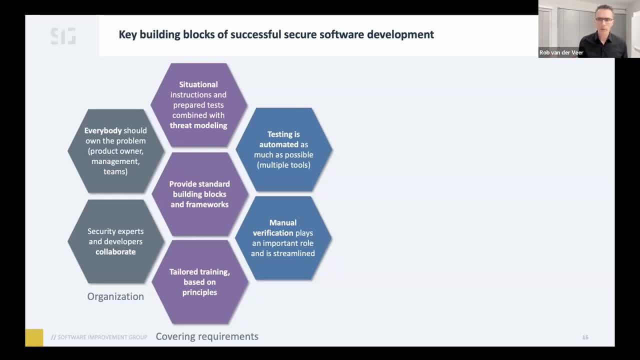 before you build or before you release. You do it as part of the story And the great thing is, because you make it part of the flow, security doesn't become this thing that you need to plan And this thing that you can postpone. 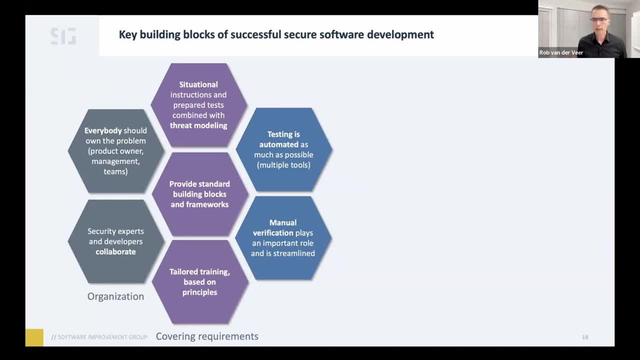 it becomes part of your hygiene, Just like testing has become part of your hygiene. And nobody- well, mostly nobody- is questioning the added value of testing and wants you to demonstrate the business case. It's just part of the duty of care And you see the same transition that testing made. 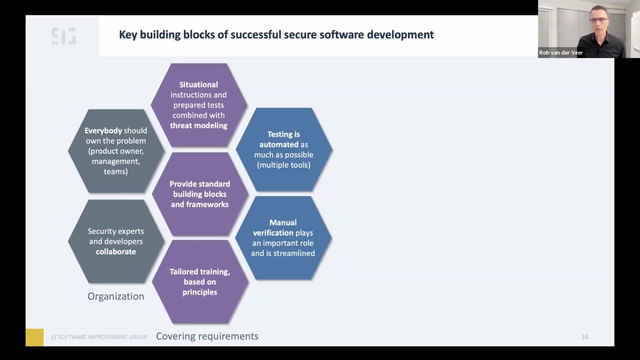 from being something that people scratch their heads about and wonder: is this worth it And what are the benefits to just being part of professional software development? Because you're shifting left with security. there's another opportunity because you can use the same facilities that you build. 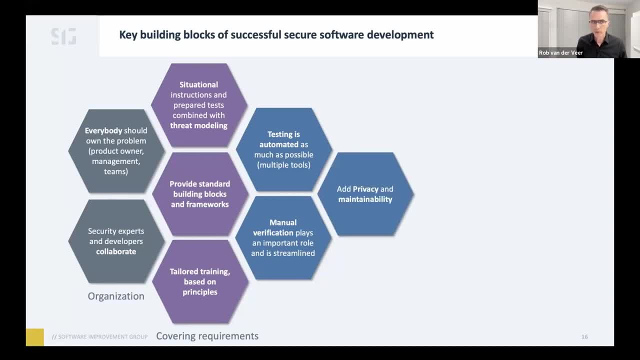 to measure other software quality aspects, like privacy, but also maintainability. These are things that are hard to tell from the outside, but you have a system so you need to measure them. You need to find out about them in the code and by doing automated testing. 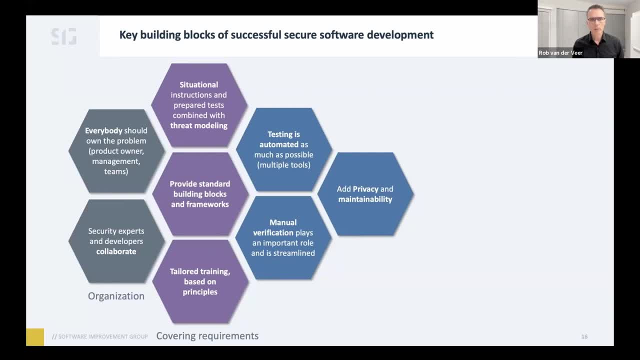 But you can build on the same things: the awareness, the collaboration, the requirements, the tools, the testing, part of your whole flow. You can add these other software qualities in one approach And this is the winning approach: not just a security tool, but a tool. and the old services. 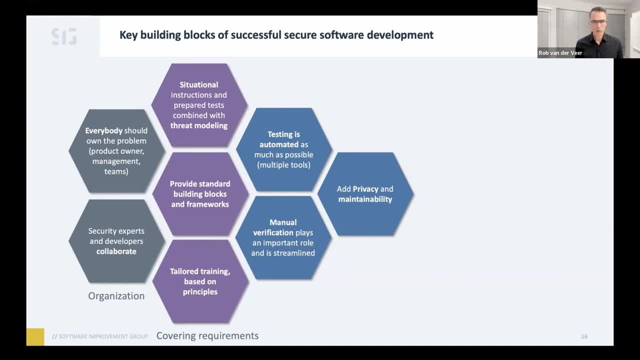 and advisory around it. that covers software quality, non-functional quality in general. So these tools and these reviews, they result in findings and you need to collect and track them somehow. What you preferably need to do with this is to create a single glass pane to integrate them. 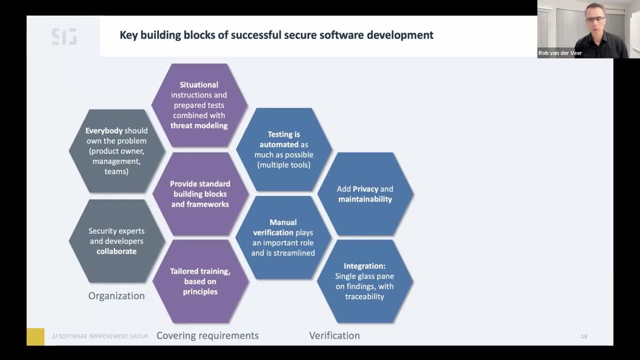 Otherwise, it will be very hard to track what things to do for teams. There are multiple tools. there's multiple tools involved, there's code review involved, there's dependency checking. It's a whole list of findings and they're coming from everywhere. 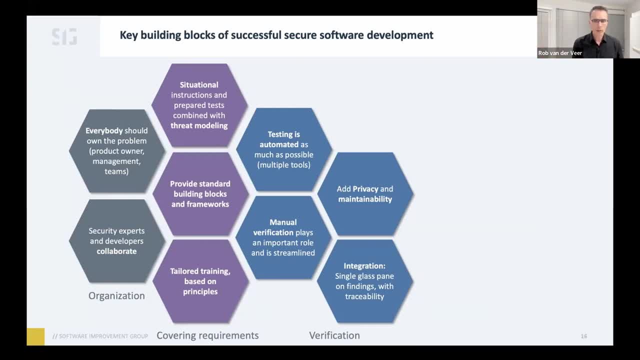 You want to bring them together and share them with development teams, but also with architects, with decision makers, product owners, CIOs, integrating these tools and combining their outcomes And, as I said, making the change in the organization and learning to use these tools and to follow up the findings. 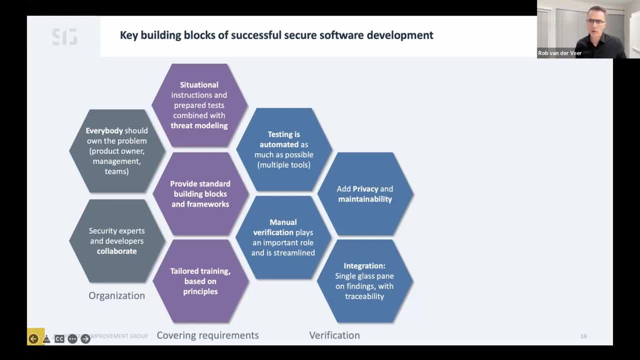 is not easy. It will not happen by itself unless you provide intensive help and guidance, Which should include exchanging knowledge between teams so they can learn from each other. What we found what works really well is to create community of practices, So within an organization that has multiple development teams, 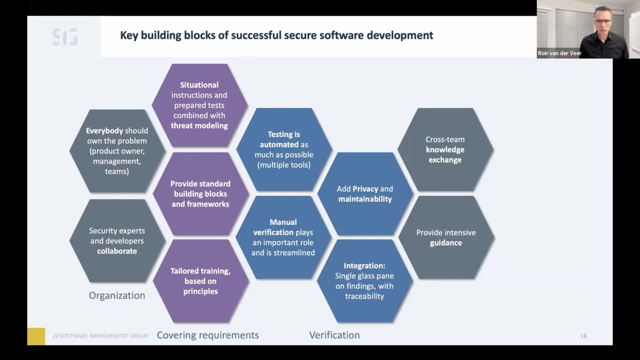 create a community of practice or a guild or special interest group, whatever you call it. it's a group that shares knowledge. group that takes the responsibility for security. That's a pitfall. No, it's a group that exchanges knowledge between the teams and shares best practices. 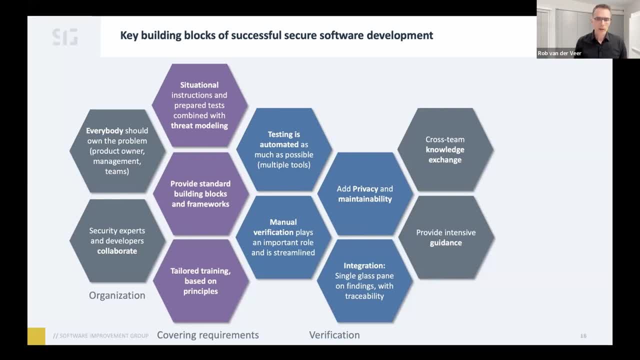 It's really helpful to amplify awareness in an organization. So there you have it: the key building blocks that allow you to build security in while you are developing. But what about all that code that you wrote in the past Without all this attention? 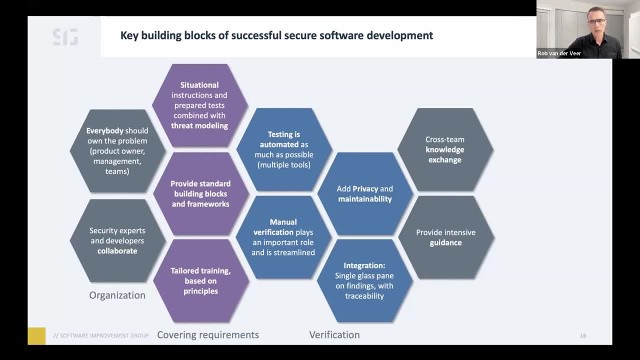 you wrote it without all these tools, without the awareness. did you get it right? It's basically the face that Elizabeth was in in awareness stages one and two. It is a pitfall to only put effort in secure development for new systems and ignoring the older ones. 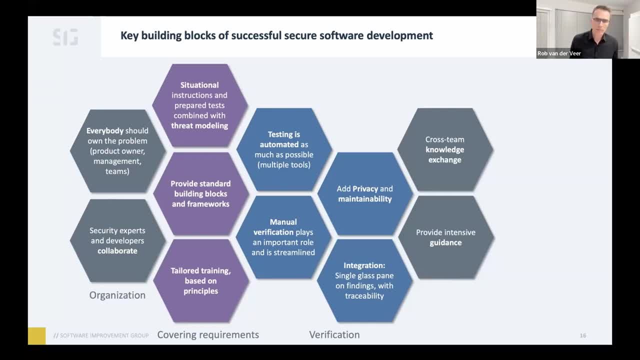 Typically, you have a lot of code that has never been checked. well, There's no need to program these systems all over again, of course, But there is an opportunity to have a close look at these systems now that you have the awareness, the collaboration, the requirements and the test approach. 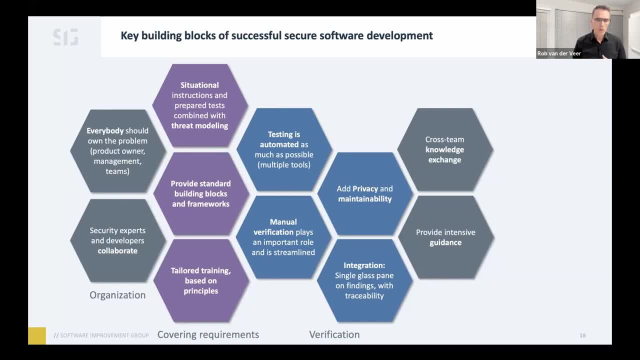 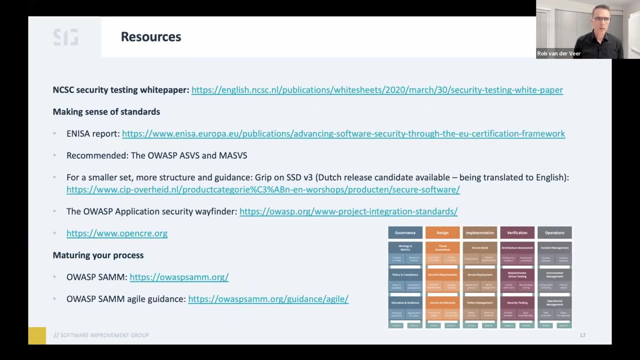 No need to put your head in the sand. Well voila. these are my key building blocks for you today, And before we wrap up, let me take you through some useful resources first. First of all, the security testing white paper. 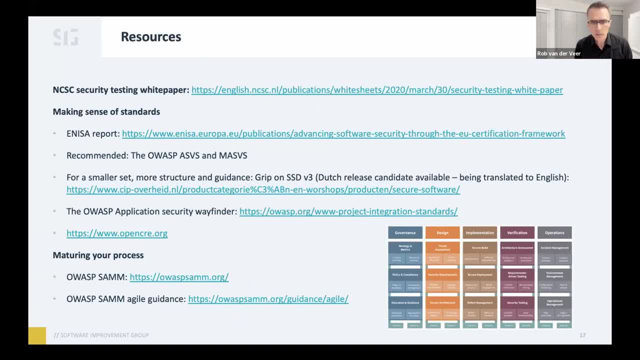 I think it's now. Oh, it's two years old, March 2020.. I was one of the co-authors. It's a really nice overview- It's available in Dutch and in English- of the different testing approaches there are. 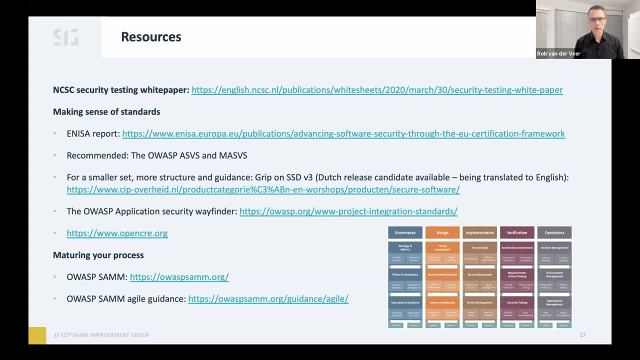 the penetration testing, the code review, the vulnerability scanning, the fuzzing. It's just very helpful to get insight into what the different test approaches are for secure software development. Then there's an ANISA report. There's an ANISA report. 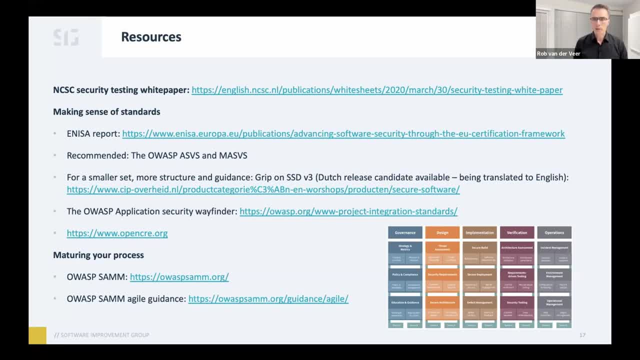 There's an ANISA report called Advancing Software Security through the EU Certification Framework. It's basically an overview of the state of the art of security standards, their issues and how we should go about this. It's just, I think, a general, nice overview. 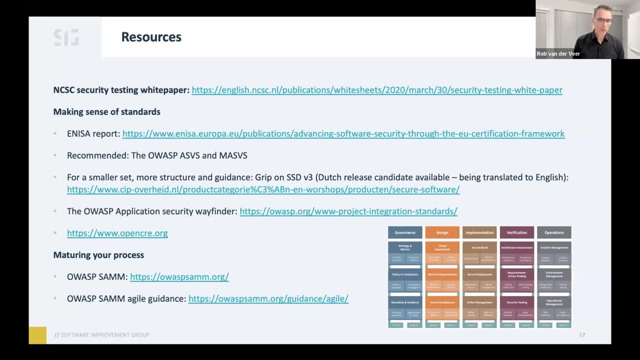 of the state of the art, Then I recommend you to have a look, if you haven't done so already- the OWASP, ASVS- a long list, comprehensive list of useful checks- And the MACVS for mobile applications, And if you're looking for a smaller set, 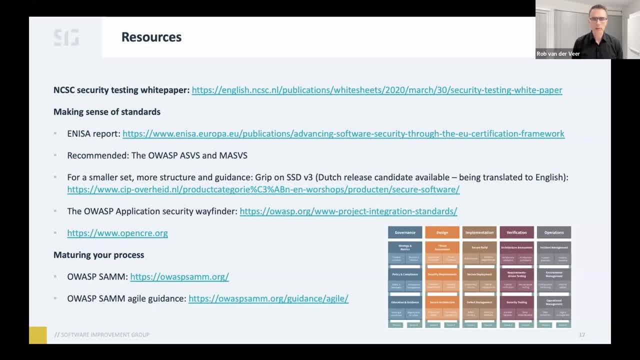 that's more structured and provides some guidance easier to grasp. there's GRIP on Secure Software Development. It's a Dutch government standard. There's a Dutch release candidate available and it's being translated to English. Actually, it's gone live. 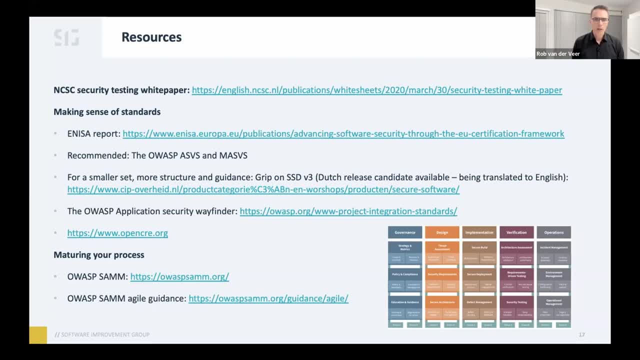 so it's no longer a release candidate anymore. Then there's the OWASP Application Security Wayfinder- I will show it to you in the next slide. And there's opensiriorg, on which I also have a slide, So more on that later. 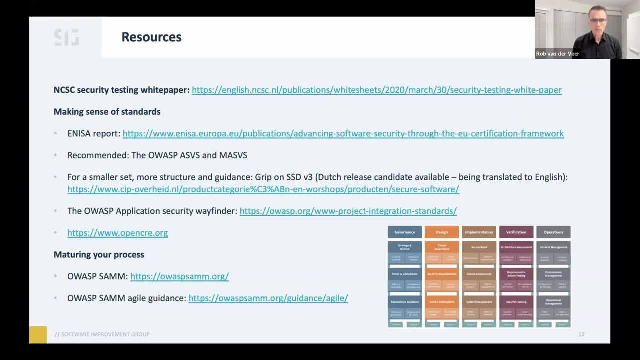 So to wrap up this slide, maturing your process, you can do with OWASP SUM- Very helpful guidance there. The chart that you see is an overview of all the controls there are in SAM And there is SAM Agile Guidance And it contains the story with the requirements. 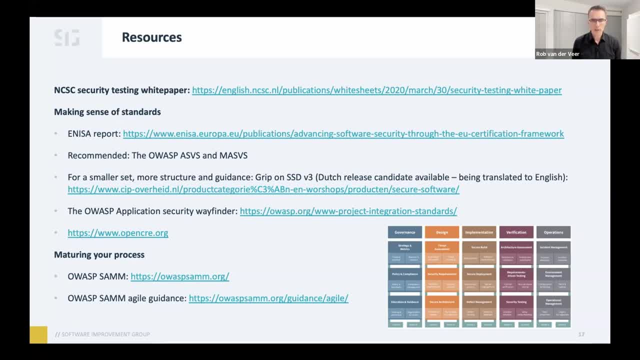 and keeping them really tailored to the stories that you're writing, and lists a number of pitfalls and issues that you have while applying secure software development in an Agile environment, And I'd like So. this slide will be shared with you later, but I think I can. 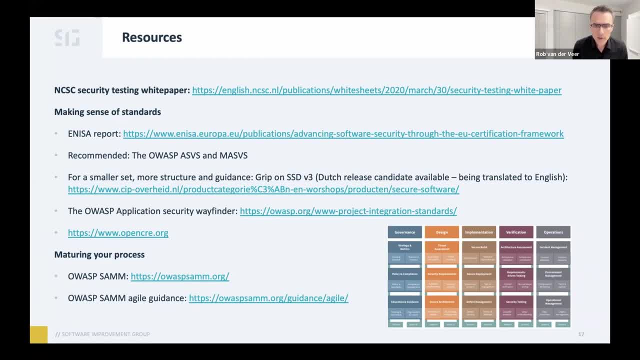 Use the chat to put this information in. Let me see if that works So you can have a look in your own time. I think that works. Cool. It was in chat, Rob. I just wanted to add that to you. Brilliant. 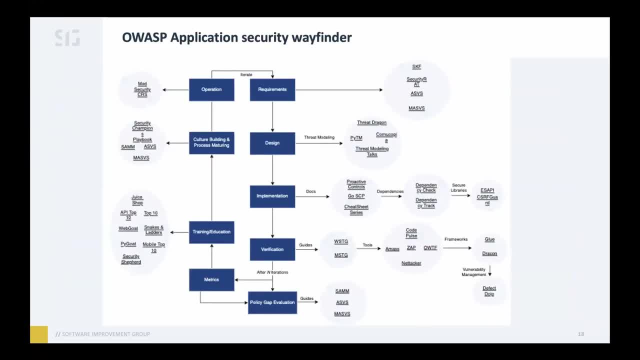 Yeah, So wrapping up, the OWASP Application Security Wayfinder that can be found on the link on the previous page And in the chat now duplicates. It is an overview of the key OWASP project. Really helpful to find your way. 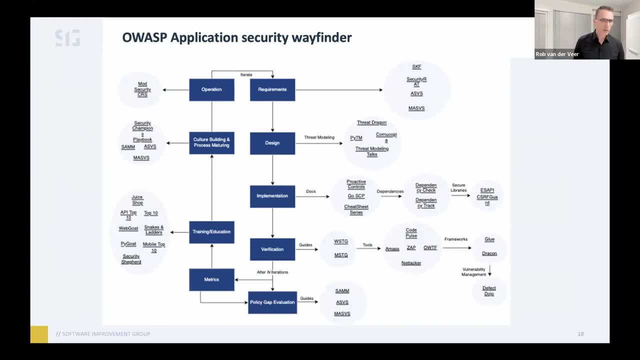 into all the nice standard and resources and tooling that's available by OWASP. It's interactive, So if you go to that URL you can click on these projects and they're nicely grouped by their role in the development lifecycle and their type. 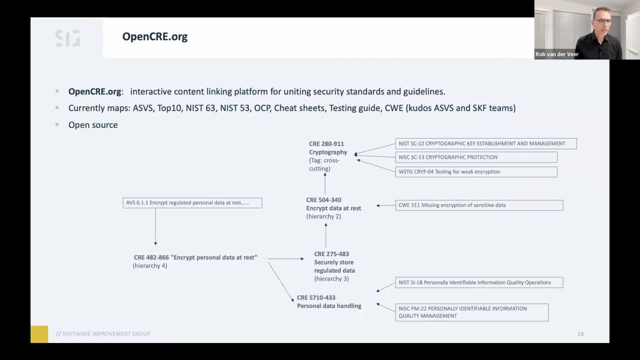 Next is opensiriorg. OpenSiriorg. It is an interactive content linking platform meant to unite security standard and guidelines. We found that the landscape of security standards is really difficult. It's complex, it's fragmented. There's a lot of different standards available. 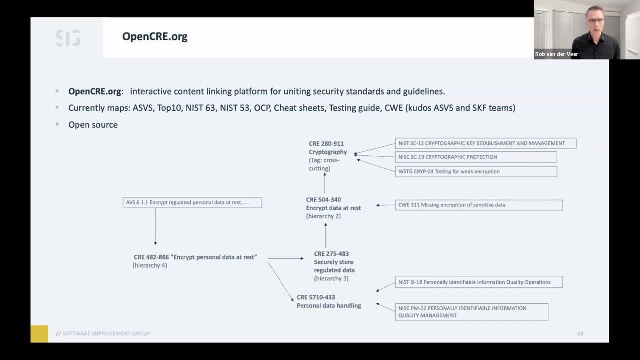 and it's hard to find the right material. And it's hard also to connect when you talk about compliance And it's hard if you have a certain check to find. if you fail that check how you should fix it, to get code examples: 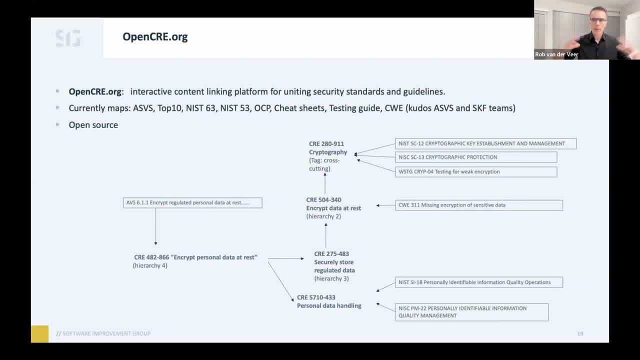 to get explanation of the corresponding threats. So basically actually everything is linked together and organizations that make standards try to link, but these links often break over time. It's hard to update them And we try to solve this problem with OpenSiri. 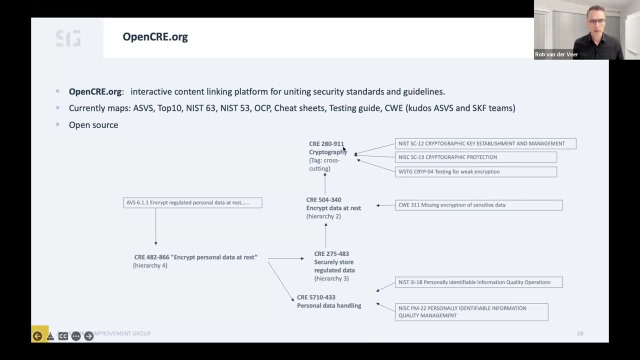 So OpenSiri contains a semantic web basically connecting a number of topics. So encrypting personal data at rest is connected to securely storing data and also the personal data handling which is then linked to a number of NIST documents. But secure storing regulated data is again. 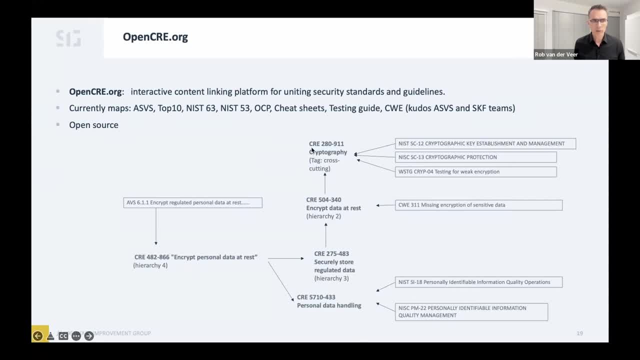 connected to encrypting data at rest, which is connected to cryptography. So using OpenSiri, you can go from one specific standard entry or one specific topic to everything that's connected and all the resources that are available in the world on these different topics. 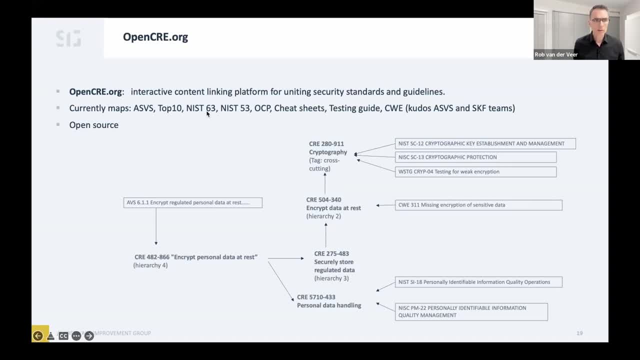 And we've now mapped ASVS top 10, NIST 63,, 53, proactive controls, cheat sheets, testing guide, CWE, And I'd like to give kudos to the ACS teams and the SCF teams. It's very helpful for linking. 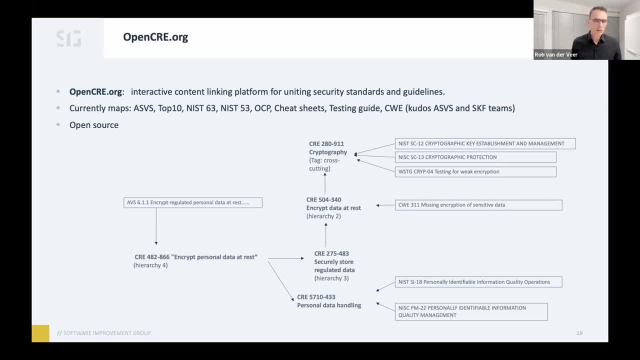 but it's also very helpful to find your way, And the nice innovation here is that it's self-maintaining. So standards have links to these topics. And because they're self-maintaining, standards have links to these topics And because they're self-maintaining, 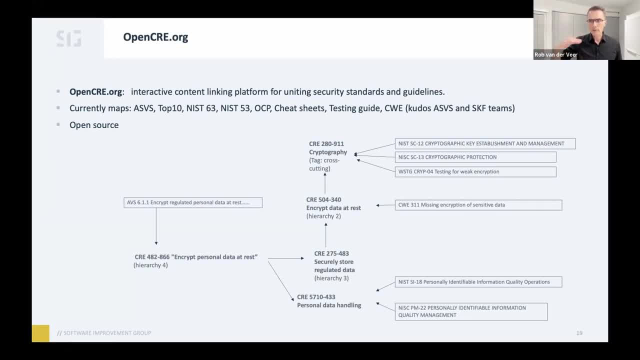 standards have links to these topics And because we scan these standards, the mapping is automatically maintained if the standard moves to another location or gets rearranged. So it's quite sustainable. And that concludes my story. Thank you very much for your attention. 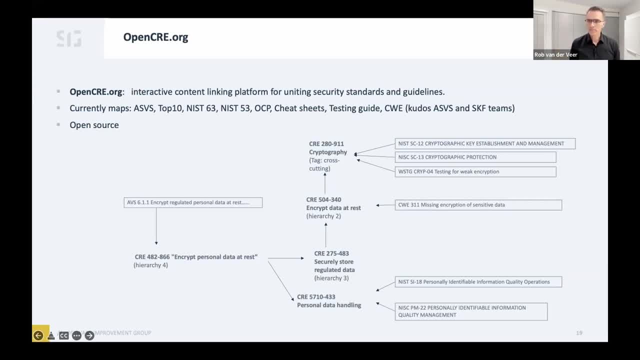 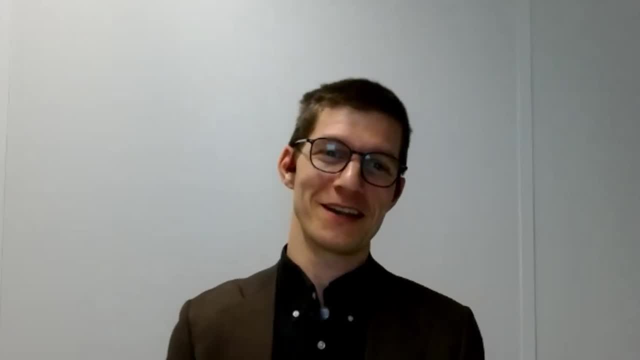 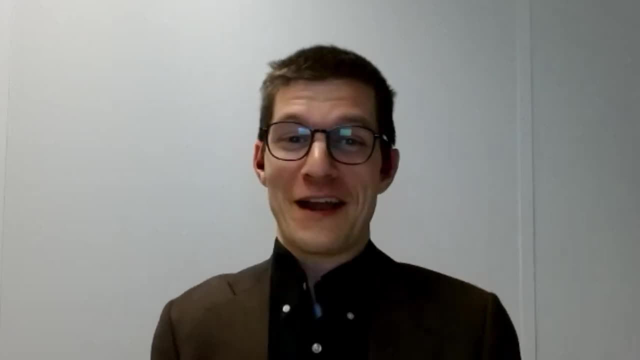 And I'd like to give the floor back to Bjorn. Yes, Thank you, Rob, for this great presentation and what a pile of information already and only 45 minutes into this event. I surely hope that Elizabeth and Darcy are now both better educated. 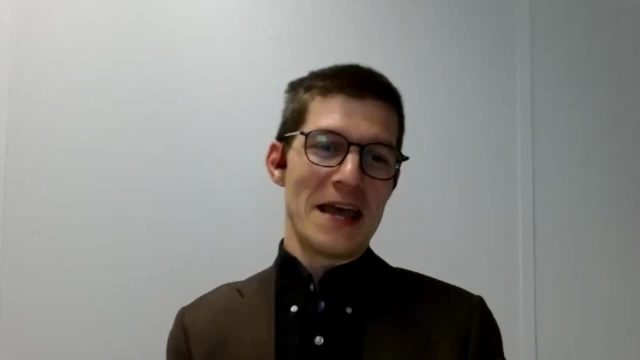 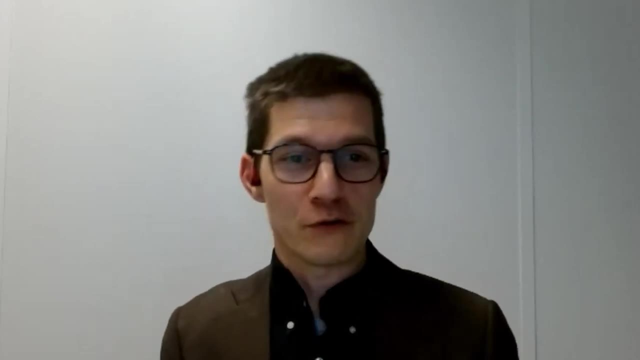 and they're living happily ever after. That's what I heard from your story. Now I hope our audience also learned the same things here. I learned a lot about what is needed to successfully build secure software. how does it fit agile, how to change the mindset, requirements, privacy. 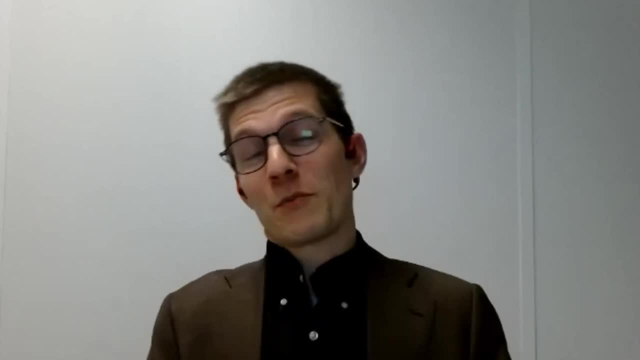 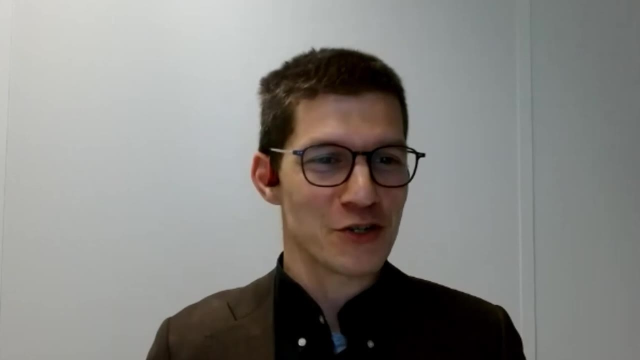 what have you? So just know that we will have a couple of questions for you after Martin's presentation, because Q&A is filling up and the chat is filling up. I'm trying to keep up with all the questions And, having said that, 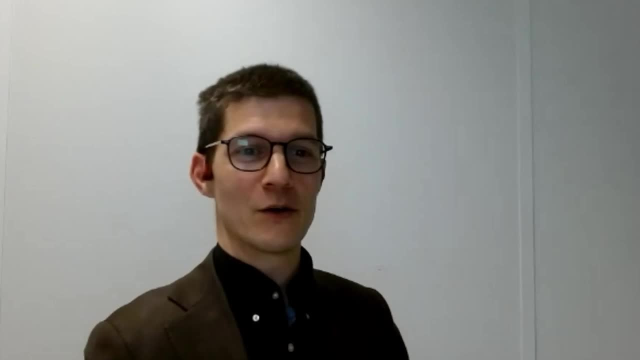 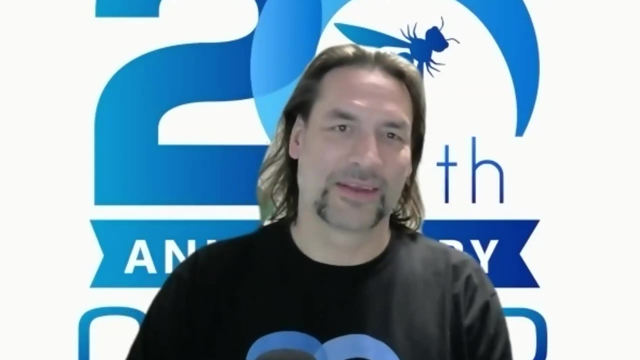 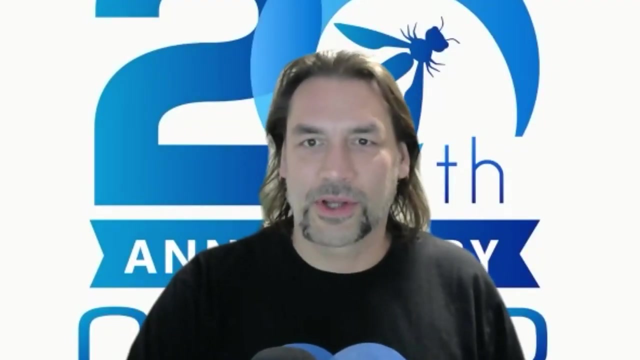 we are looking at the next speaker's presentation. Martin, would you be please so kind to turn on your webcam and your mic And Martin will introduce himself and his presentation Now. we'll be back later. Yeah, So let me share my screen. 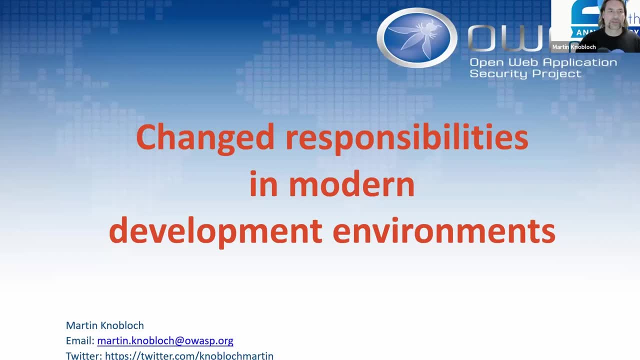 Okay, so now you should be able to see my screen. It's always very interesting How it works with Zoom meetings. Yes, Okay, Yeah, Victoria question. So yeah, we also hopes great presentation. So next step for me is when you have this building. 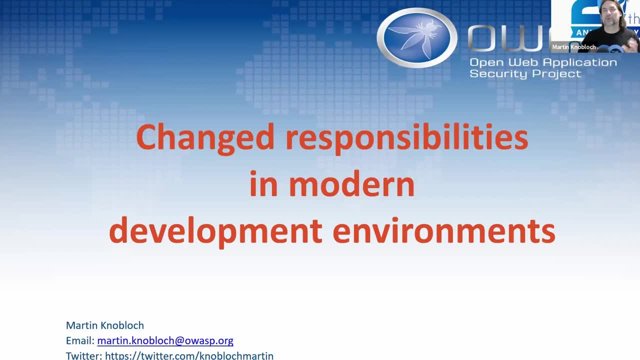 wasn't going. there actually is, then. so what is the responsibility? So everybody knows this software development and everybody who does security thinks they are in security And so, therefore, they do security. and I dare to challenge this: Who am I? Those who don't know me. 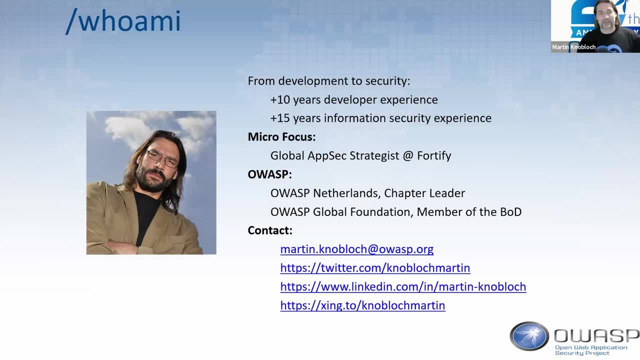 Yeah, I was a software developer, a self-trained developer, back in the previous century, in the 1900s and the 2000s and 21st century. of course, I'm not that old, I come to security, but before I was developer. 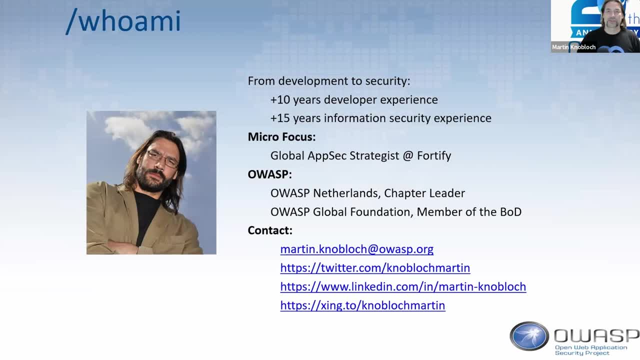 I was actually in a production area. I was a mechanic for injection welding machines And I looked into PLC programming And this is very physical: more security, action, more safety and knowledge. I went into software development and was wondering why there are things are possible. 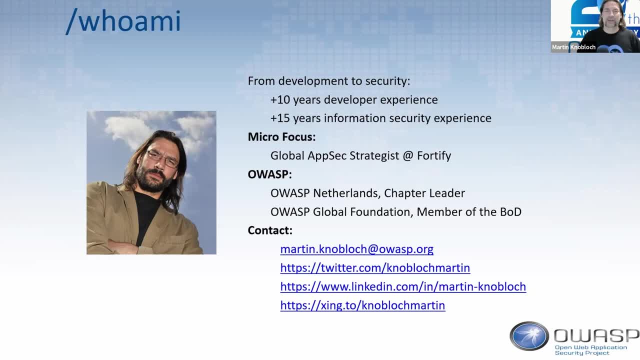 where in the production area it would not be possible. And back then in the internet was new in the late nineties, They said, oh no, we will do that. I was like really, And you all know, when you don't work from home. 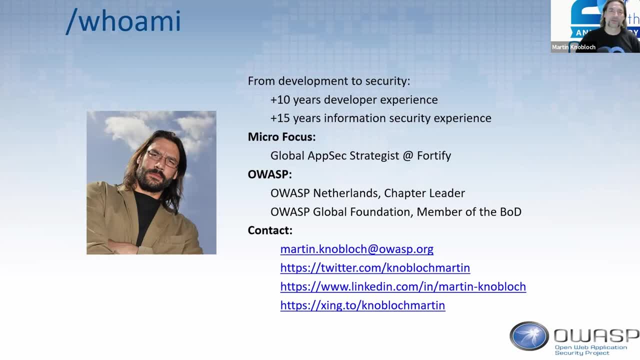 and you in the past. when we talk about work, what crazy people sometimes do in a physical world do not be secure. Actually, they're there in other people's life And now in the internet. then we thought everybody would behave right. 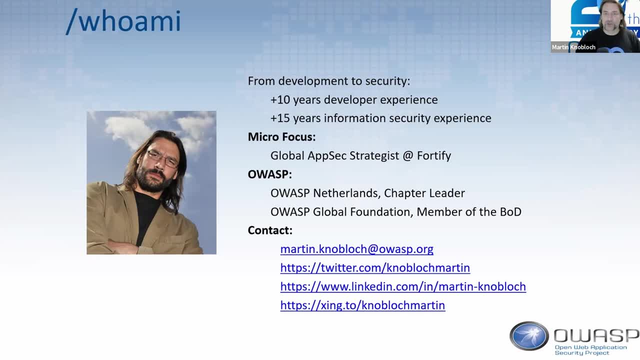 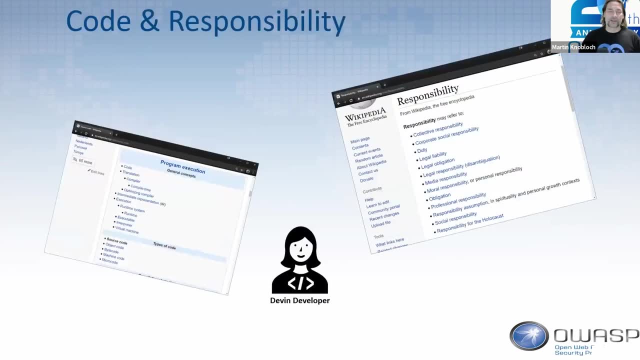 A big failure, as we know now. So enough about myself. I do a lot of stuff for OWASP. The next thing is more important, like the presentation, And for this let's start as a responsible change: responsibilities in the software development. 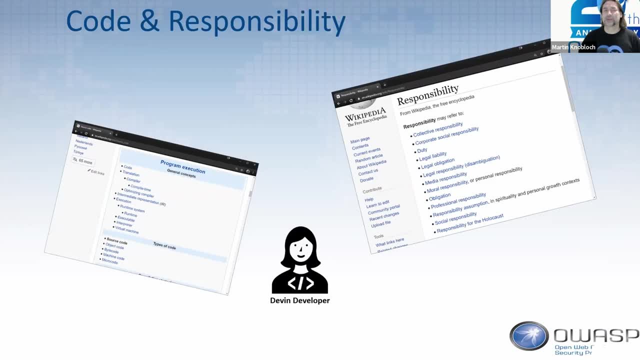 life cycle is what is code? And this changed a lot, And I know that a lot of people are about software development- are like: source code is everything. It's just syntax and the grammar and everything. Forget about it. Currently, these days, the modern software developers 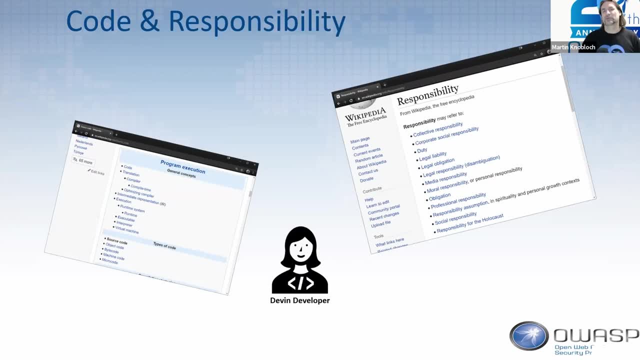 these days, whatever they can check in your source code repository, your GitHub lab, whatever they will consider it to be source code, That includes the configuration files for your infrastructure service, your Terraforms, your Azure, your, whatever you have, your Helm chart. 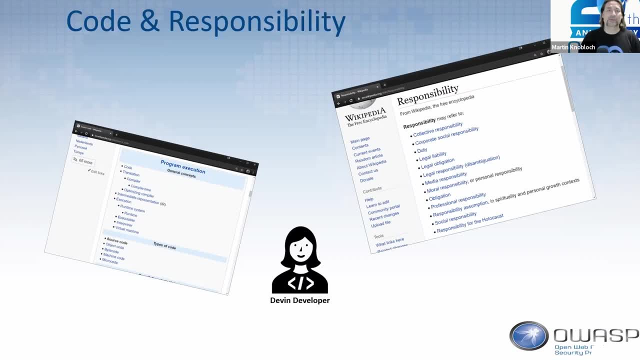 They consider a source code. Therefore they expect when it's scanned for security, there's the source code, It's whatever they set up. We have been also scanned and validated for security And the responsibility is another thing. In the past I saw a lot of security specialists. 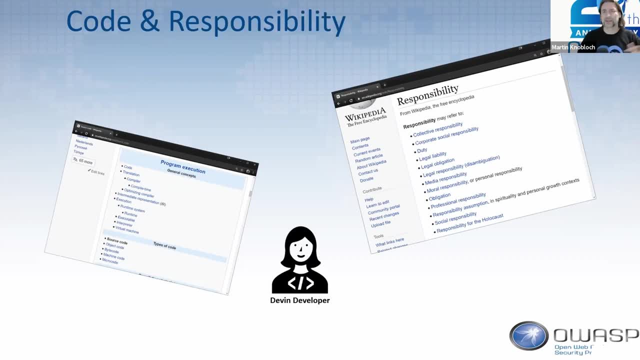 that said, oh, I did software development. I can do a good job. I did it in my university times. But there's a big difference writing software for your hobby project, for when you're doing your IT master's or whatever degree, or you write software 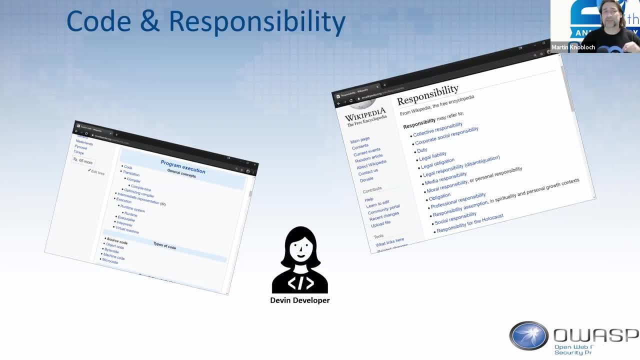 for an enterprise, And that's awesome. It means that this 25-year-old- I always jokingly say senior, full-stack developer when they're like: oh, I'm senior, I have done two projects or three years of software development, that you are not senior. 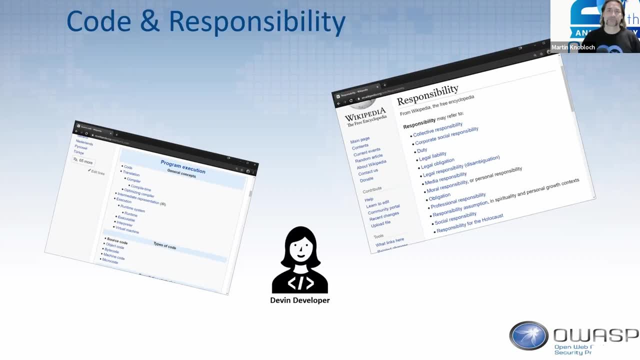 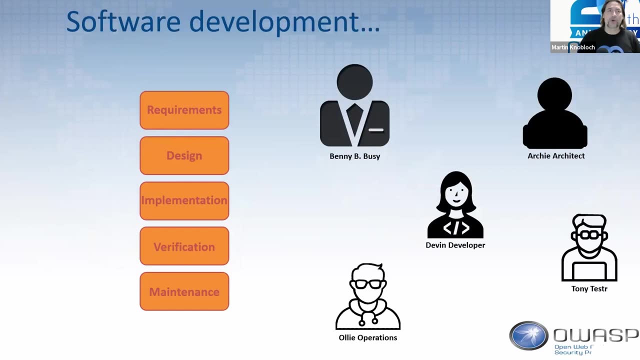 if you have not suffered from the consequence of your own choices. But let's go back into history. I truly believe you only do things really well and right the moment when you understand why you're doing it. And software development actually didn't change a lot. 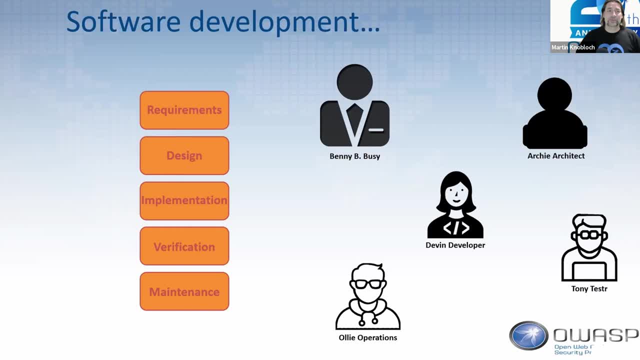 the previous years, We always had some requirements. Yes, we build software not just for fun. It has to do something And there must be a design how we do it And so providing implementation, the verification, and at least we have to keep it alive. 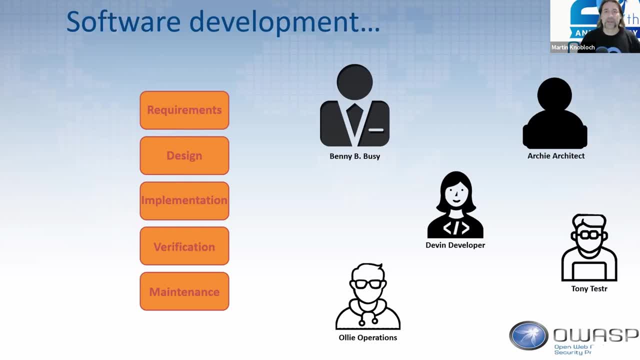 And also the roles didn't change a lot. We have the business people with the money, We have the architects And I remember early 2000s that we had a lot of architects: the information architect, the functional architect, technical architect, whatever architect. 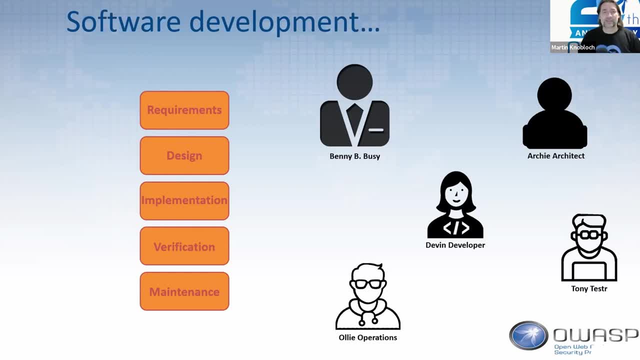 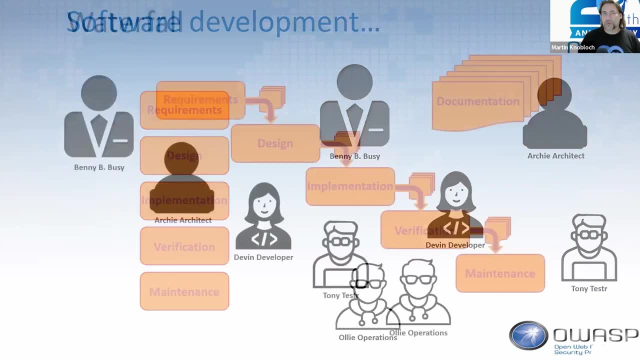 Then central, then somebody has to write a code, Somebody has to test it, And then operation gets it and has to maintain it. So we needed a process for this, And a lot of people recall the times when Waterfall was hot, And people nowadays bash Waterfall. 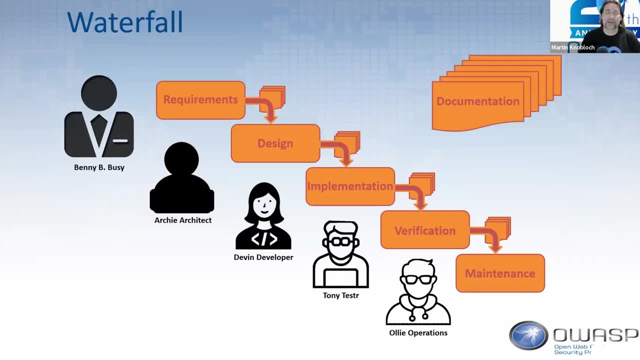 But it's not bad. At least we have a process, And process means that we have a means to do something on a repeatedly way. When we repeat, we improve right. Of course, we all know the problems with Waterfall. 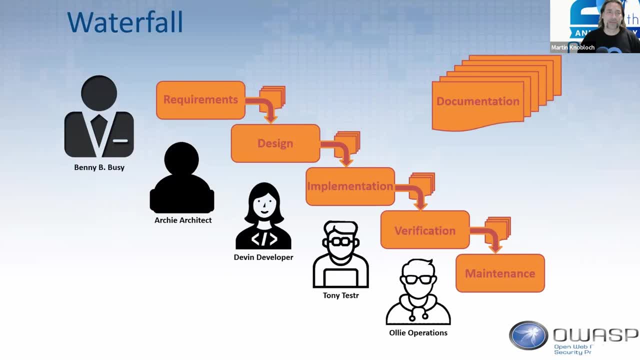 It got its name because it cascaded from one step of the process To the next one by just zipping down the documentation And there was no feedback loop. And they came in later because we tried to make Waterfall more agile. But yeah, when you have a question in verification. 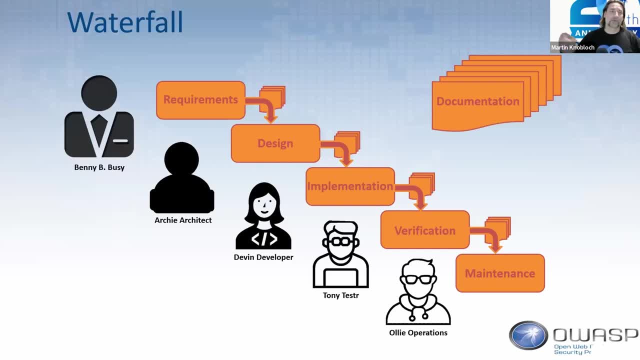 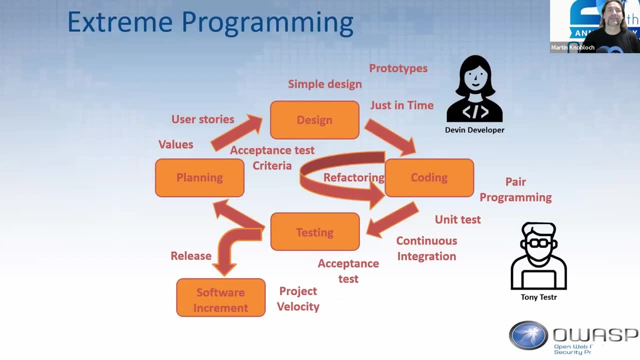 you couldn't go all the way back up to requirements because the team or functional analysts were already dissolved or worked for another customer right. So the big release came already in 1996.. Extreme programming 1996.. The first documentation about it. 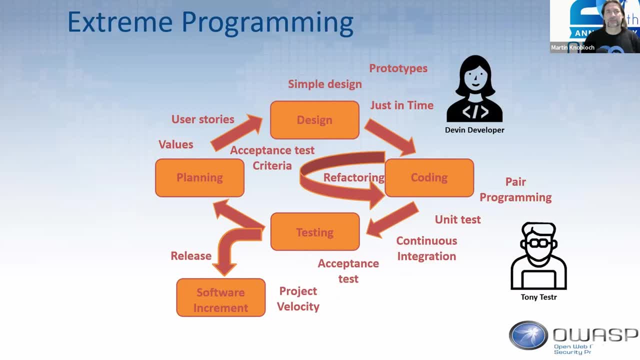 It came over to the Netherlands in 2001-ish- 2-ish- the first companies working with that- And it was great, And actually a lot of things we do these days in DevOps- whatever you want to call it- comes. 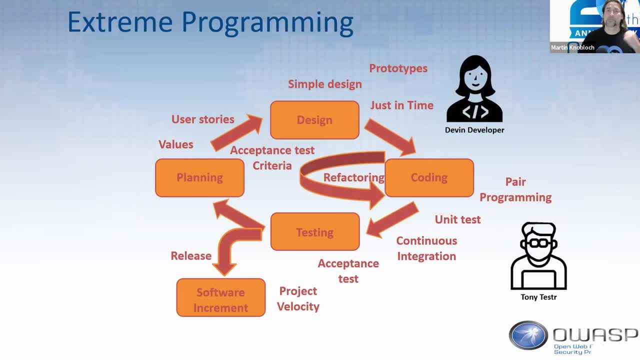 from the time of extreme programming. So the planning: we had a planning, design, coding, testing and keep it alive. The thing is we said, hey, we build for not the whole thing documentation wants. No, we will incrementally build it. 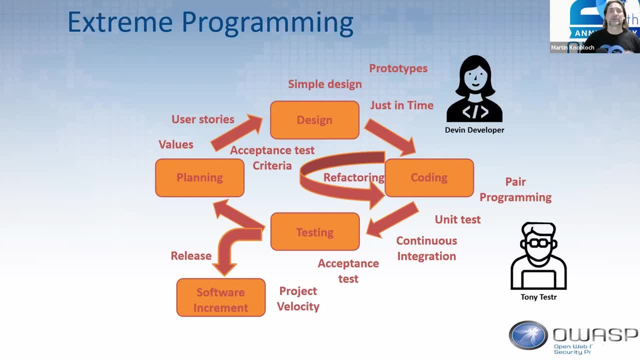 So it is development cycles, the sprints we call it. So we did a sprint, We did the user story, We had a set criteria. We keep the Kimball design, We prototyped stuff And everything in prototype has to be production-ready code. 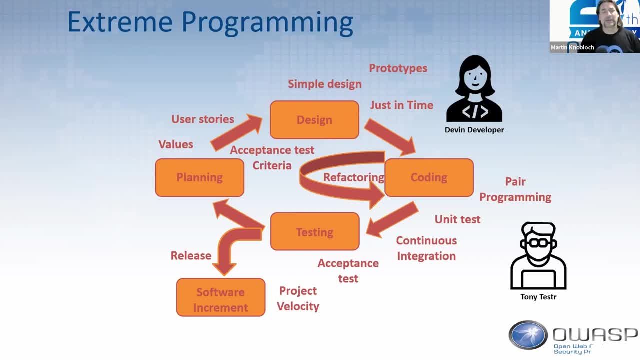 People can't forget that We did pair programming, different than in Waterfall, when our testers and developers were like two camps of fighting each other. Now they became our friends. So we did pair programming. We sat together at one keyboard. I hated it. 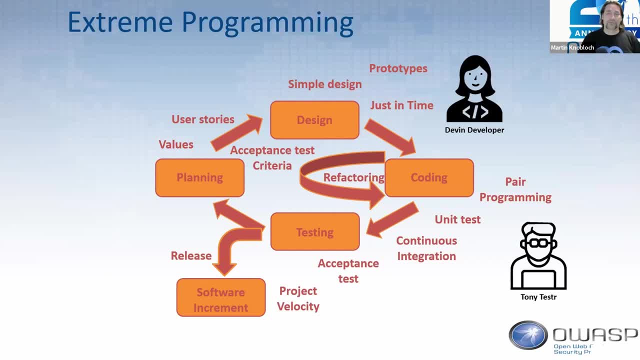 Nobody touched my keyboard. We do it. It's software, Because the tester understood the requirements and the developer was the one who could implement it. Test-driven development comes from that time- Perfect. So we built something happily, with the developers and the tester together. 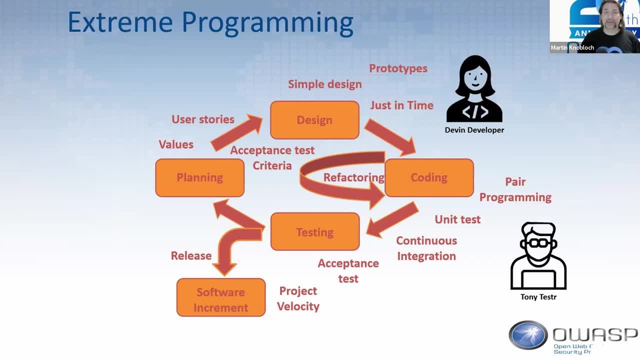 And then what We did releases right. We had acceptance tests, We had integration testing already up there And we had our demo And we released it to. yes to operations. And normally, where is operations? Yeah, in the basement. 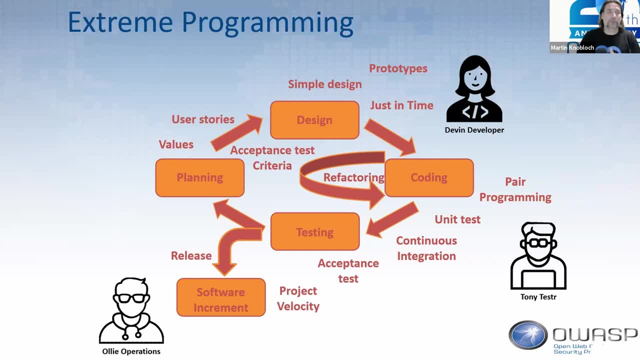 So they had this artifact And it was so shiny and great, It worked on my computer And then we dropped it to operations. They were like: what the heck is this? Yeah, And that's one of the pitfalls for extreme programming. 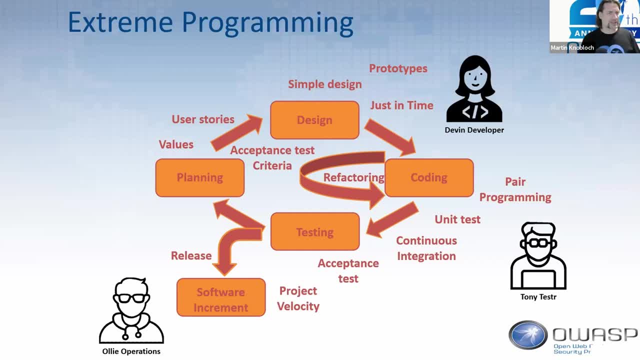 One is operations were not involved. That's really weird. We built something but we don't have on board who have to maintain it. Also, the architects were there, of course, But the business? there was no business alliance. And of course, with Agile we say, hey, fun. 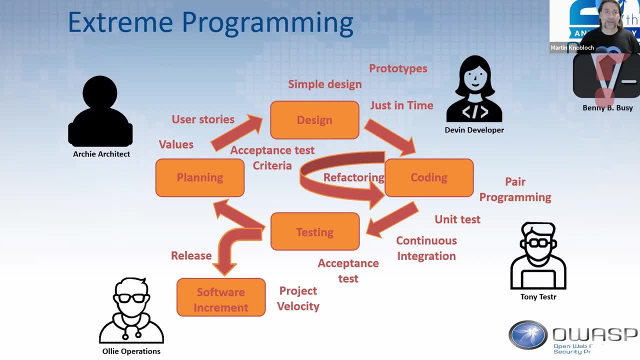 Time and money is solid And functionality is flexible. It's very hard to sell And a lot of people adopted extreme programming And said it's so cool And they just left out documentation. We have self-documenting source code- Not completely right. 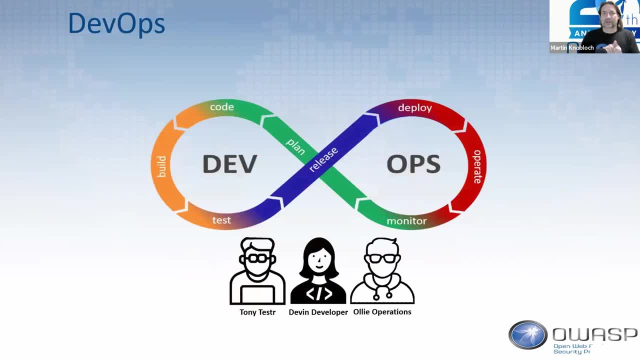 Anyhow, these days it's all about DevOps. Let's go there. DevOps is great. Everybody wants to do DevOps And we have to full stake Java developers. I love them. So how does it work? Let's look into DevOps. 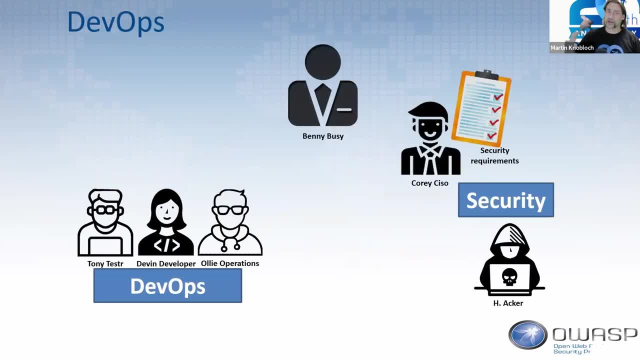 We have the cams right, We have security and development on top of the business, because they pay everybody, And we have two cams right. So the business has a need of functionality. So they assign some cool new feature or whole application. Ooh great. 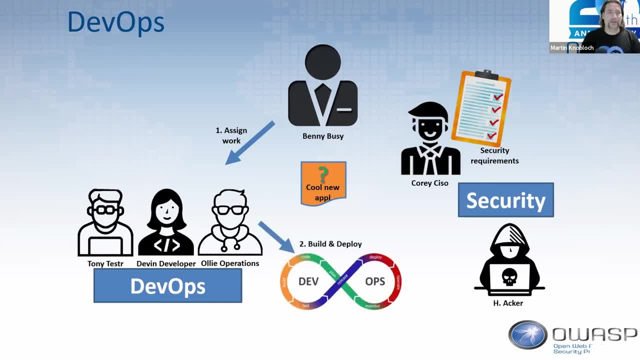 To the development team And they say: great, We have a DevOps, We can decide ourselves what technology is best, which target system. Because we have a DevOps, We are DevOps right, And they build and deploy this new cool feature. 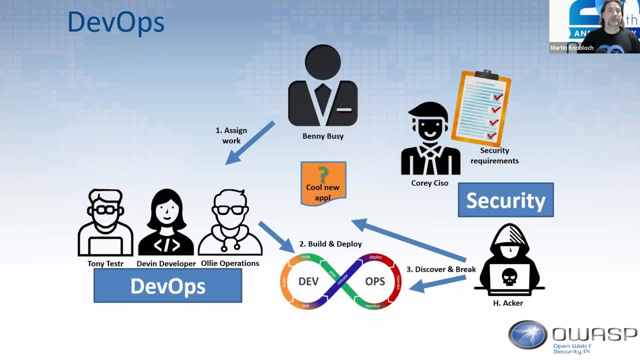 And then someday the security team finds out about it And they hire or have a hacker And they hack it And they break it, And then they will blame and shame. Hey Saiso, have you ever seen this in your security requirements? 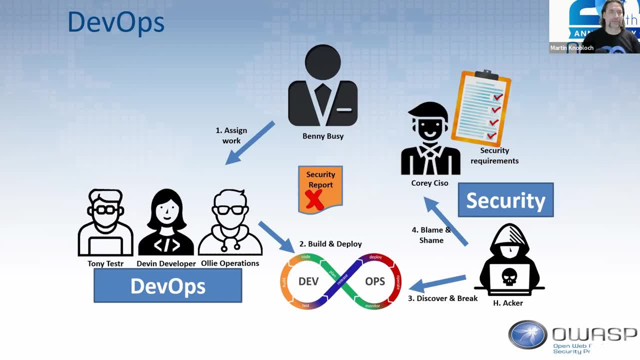 This tool is really, really bad. So it has a speedy, long, dreadful long security report And they blame and bash on the developers And death will be complete. And then they say, hey, we can't go live. This application has to be fixed first. 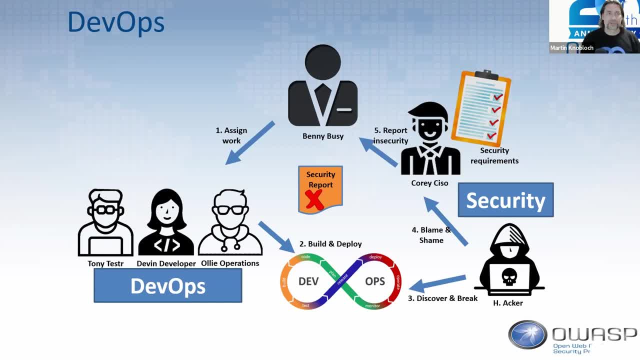 It's what Rob said earlier- Has to be fixed first. We have to go live next week. We have PR already there. Our competitors are there, So it costs us money. So business has no other chance than to accept the risk, right. 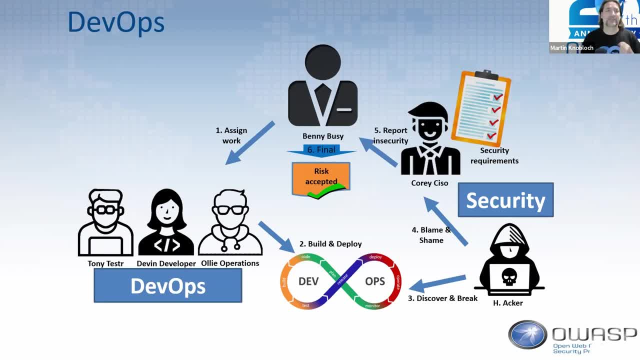 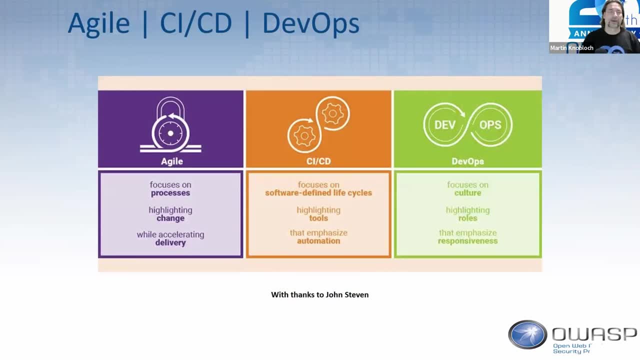 And that is the fail And that's the reason why I put DevOps on it. So that is the misinterpretation of DevOps. So of course we didn't do one giant leap. from extreme programming To DevOps is actually DevOps is a collection of things. 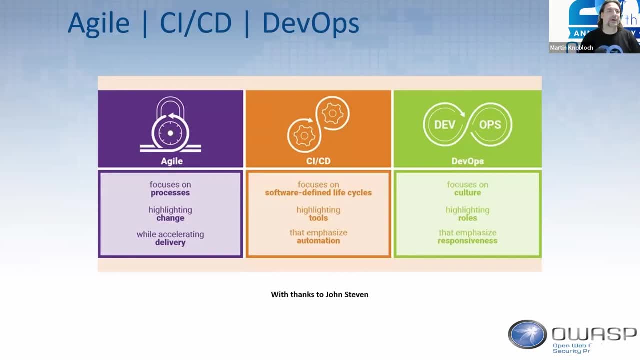 And they have been used for some people interchangeably wrongly, Because first we come from the extreme programming, We came to agile right, As I always said, something from: we had. the time and money is solid. We cannot spell it with that. 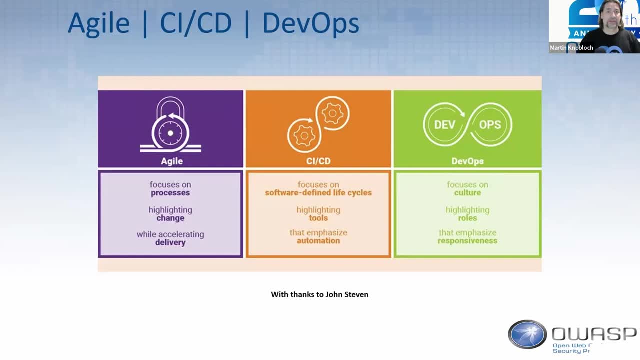 But the functionality we deliver can be changed right And we deliver on a basis. So you see, agile focus on the process And the change is highlighted. So we did it. We don't know what we need next year. What we had in the model, we chewed out an application. 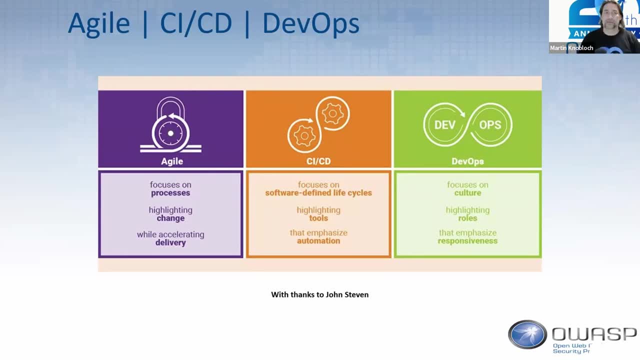 We spent six years on developing And then we delivered, seven years later, something the customer never needed in the first place. Now we're highlighting on changes. We purposely build something and will do it in development years and see if you go the right direction. 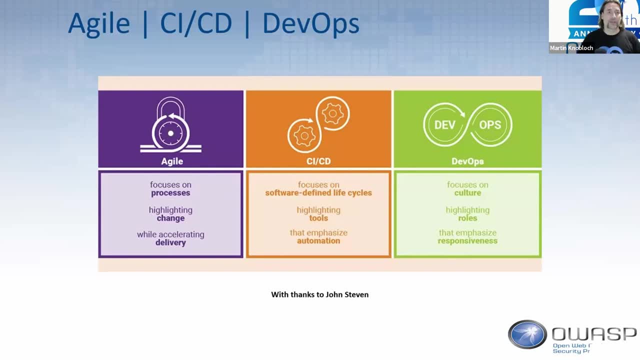 So we accelerated on delivery. Not one thing to wait for a moment, but small features continuously. And when you then deliver something continuously, then there's: hey, we need a continuous build And to eliminate everything we do by manual. we have human error abilities. 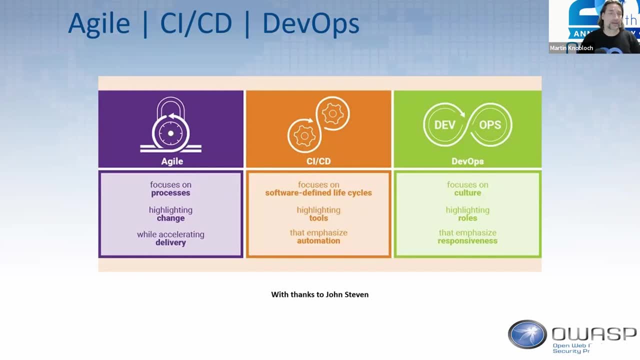 So we have to have some software-defined life. side Brings us to CICD And we're highlighting the tools. More tools are better And that's where we came from. extreme programming. Keep it simple. It's all so many bits, simply bits. 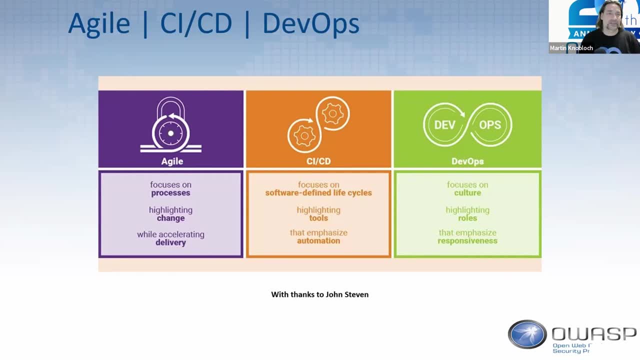 that it becomes complex to oversee. But the emphasis on CICD is out of reach. We're eliminating the human factor of human errors, the effect of human errors. And now then we came to DevOps. currently, DevOps is still for quite some time, it's not that new anymore. 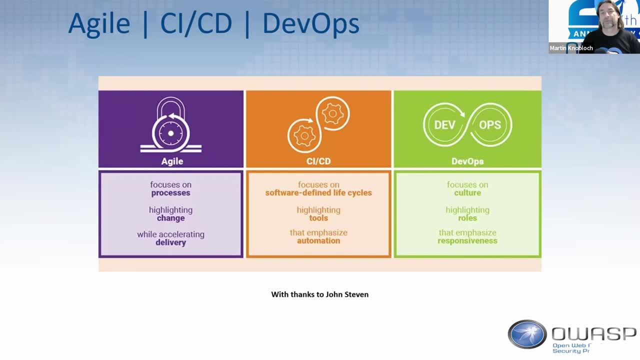 It's hot And it focuses on the culture And it's a big, big, big difference. It highlights on the roles. We have different roles Because, yes, an ops guy in DevOps is still an ops guy in the context of software. 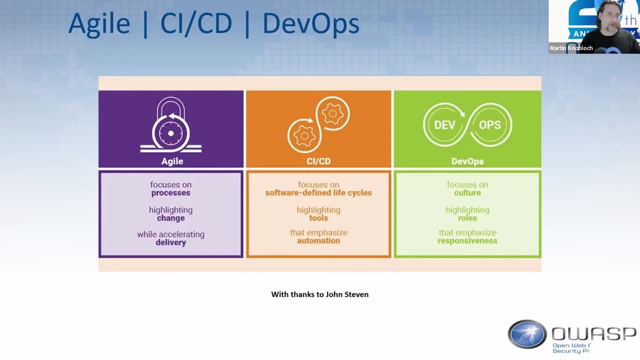 It's not somebody who walks around with a server in his hand Or the Azure network cable. No, in the software-defined environment they will configure the software-defined hardware. It's not a video operation, It's a software content And the full-stack developers are full-stack. 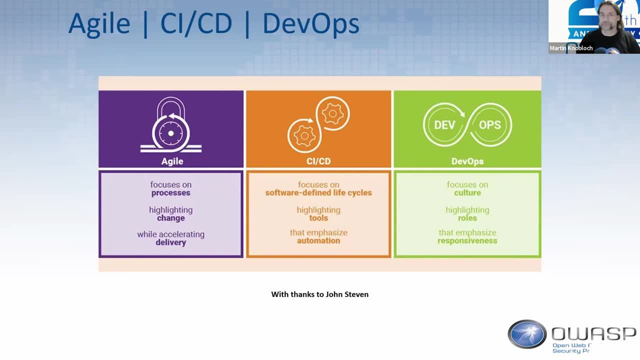 in the context of software development. Keep that in mind. That is important. So, that said, the emphasis is on responsiveness. Sounds maybe initially a bit the same. as for Azure, It's a bit different And I will go more in details on that later. 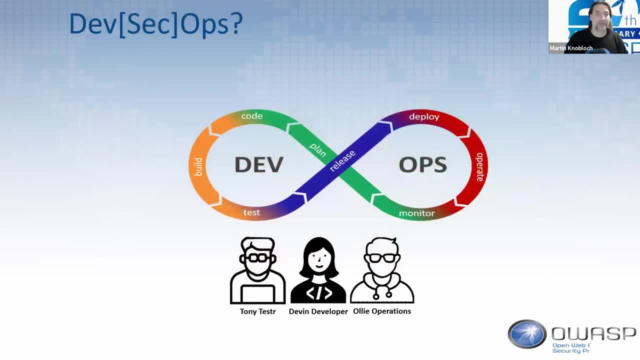 So now we come from DevOps to DevSecOps- And I put it in braces because I think it was one of the questions. Yes, the sec in DevSecOps should be temporary. It's only there to emphasize security And of course we want that. everybody is unknowingly able. 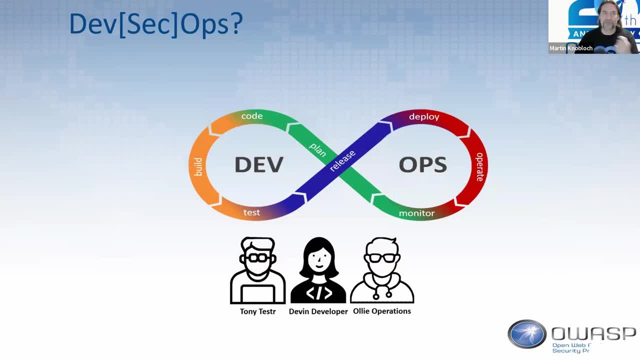 So we don't need to emphasize security. But when you go to emphasis on it then you say secOps. So it's DevOps. We have DevTestOps, We have the AzureOps and the whateverOps And IoTOps. 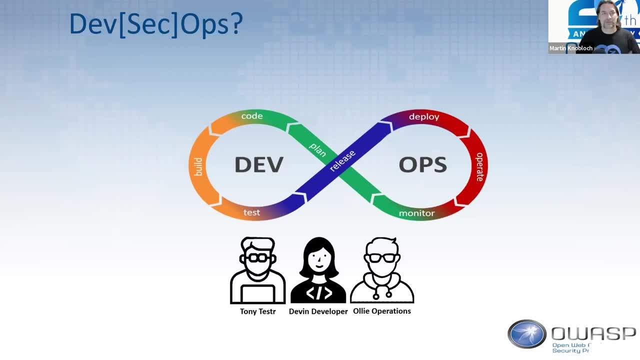 I talk about DevSecOps because I want to put the emphasis on security. So if somebody is DevOps, of course they are right. I know that a lot of purists say no, security is more important than software. But if there's no software, we don't need security. 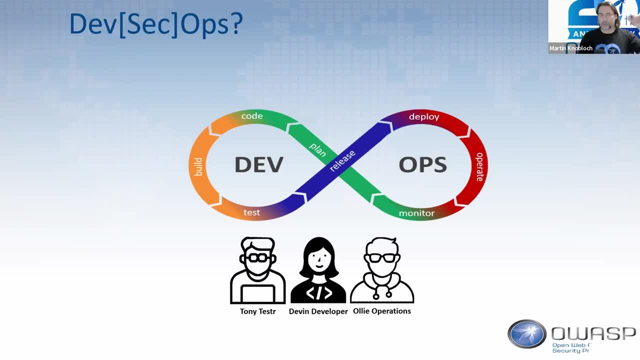 Anyhow. so what I see a lot of time when they implement it. so now we do DevSecOps is we have, hey, static code analysis. It means that actually we can look at a source code in a static way, because there's all the truth is in the source code. 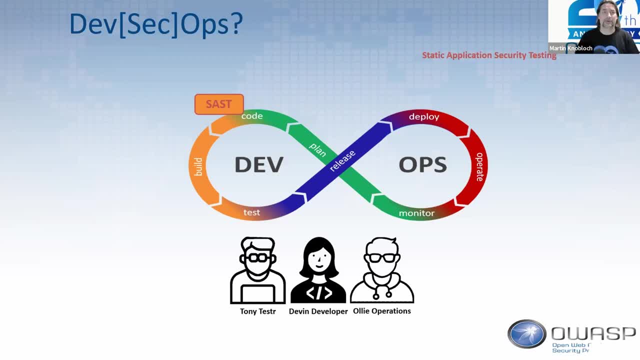 We can then see all that in it, So we can find any error. That's what people really believe. And the great thing on SaaS- the static application security test- is you can do it before you write one line of code, because you can already in your CIC pipeline. 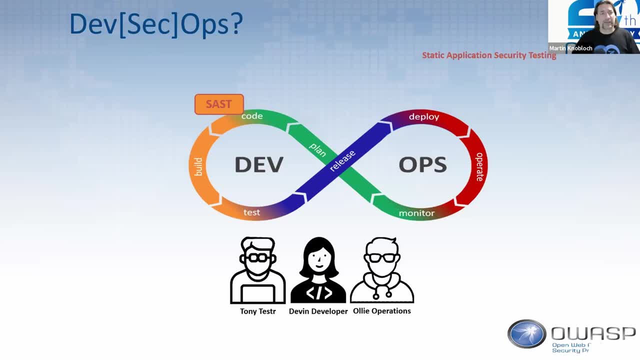 set it up that when you ever check in a file that it will be validated. There are different levels of depth of validation And people forget it. It's not just one size fits all, even for SaaS, because when I write code, I compare code writing with writing a book. 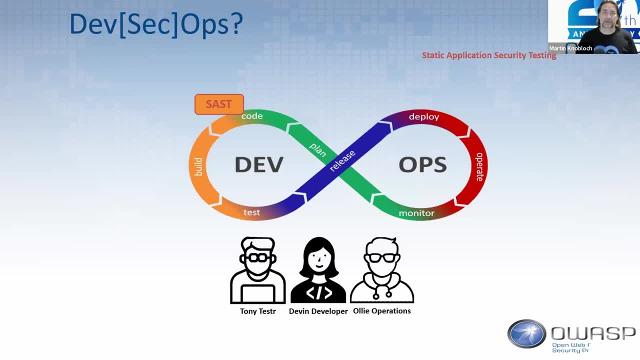 If I write a book, I write a story in my text editor. I don't want to write the whole story in the end. I look for grammar and spelling mistakes. I want them on time During my time that I write a story. let me know if there's a grammar fault. 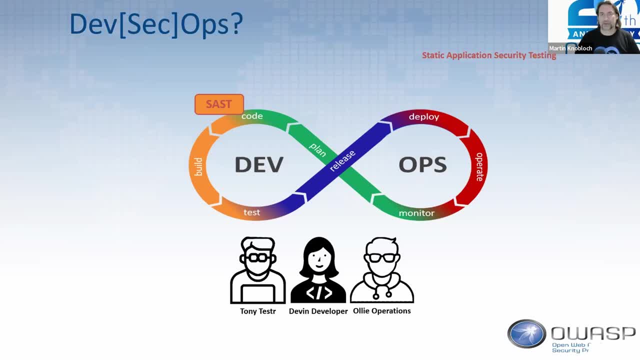 Let me know if I have misspelled them, because it takes too much time to fix it, So you can put it already in there in the IDE, in the editor that you're using- Sorry, in the IDE that you develop and use, because developers live in the IDE. 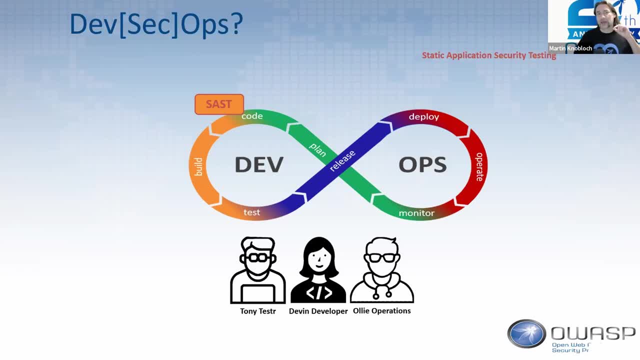 Everything outside of the IDE will not be used, So there will be early feedback, quick feedback, not a deep scan, but just. is my grammar correct? Do you use functions correctly? Have I fired level security? Very quick, instant feedback, right? 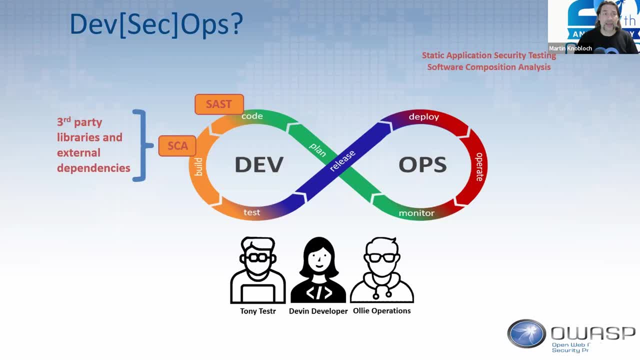 SaaS, Then you have SEA. It's a new hot thing. It's almost a thing. It was 2015 when they said: firstly, the unknown vulnerability in third-party libraries. Now it became hot and now we all who have lost their holidays. 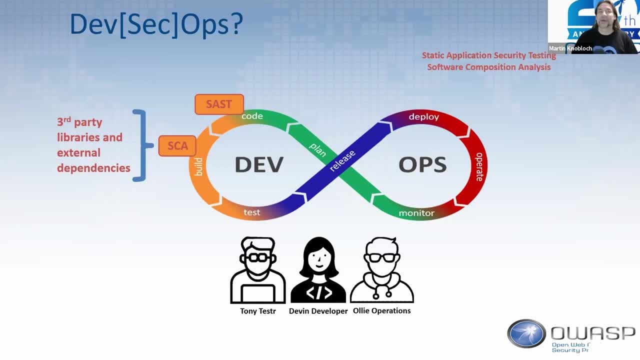 their Christmas holidays with log4shell or log4j, formerly known. Yes, our software is not these days 100% written by yourself. Even in my time when I was a developer so long ago, we didn't write everything ourselves mostly. 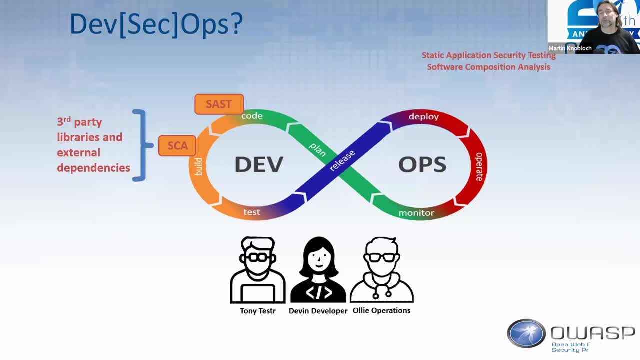 But even your framework, your library, your technology, you write the source code, You have PHP, Java, whatever, Ruby. It's a framework, It's somewhere, people have written it. So that's all your third-party libraries and you need to know about dependencies. 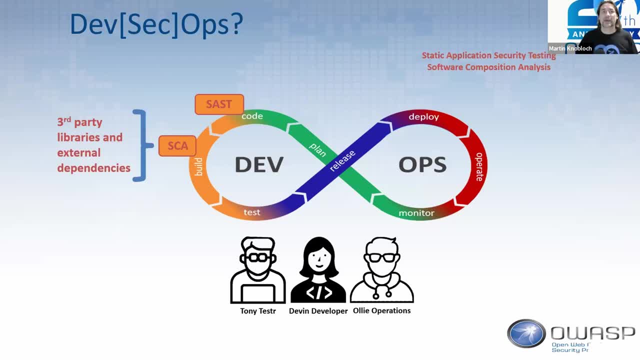 And there you have software composition analysis. It looks in all the bits and pieces that make your software, if there are any known vulnerabilities in there. And of course one thing is there is a vulnerability in there. The other thing is: is it relevant? 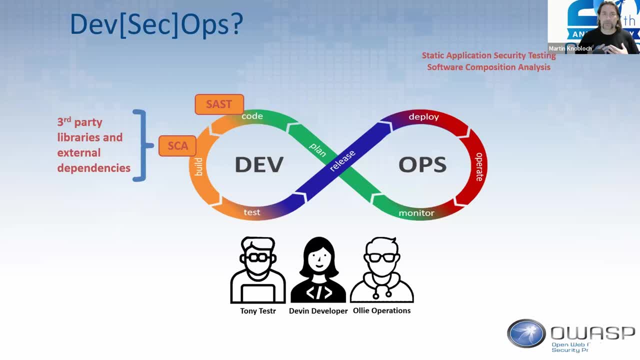 There can be a vulnerability in a third-party library. I don't care about, because I don't use this feature And in the past we said: no, you have to use the newest one and the best one, because otherwise it can be used later on. 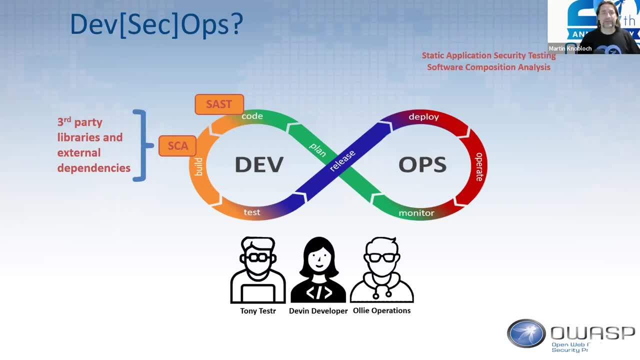 And then we saw for Heartbeats and yeah, the newest is always the best right, And we had to go a version back. So yes, to maintain SDA means that you look in what you call the. is this vulnerability even a problem on my software? 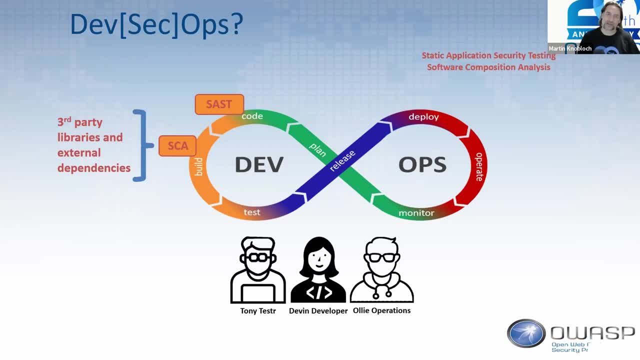 But sometimes you just have to say I can't, I don't want to risk it, and say I don't want to have a certain version. That's what we see with Lock4J. Some applications, they don't care. 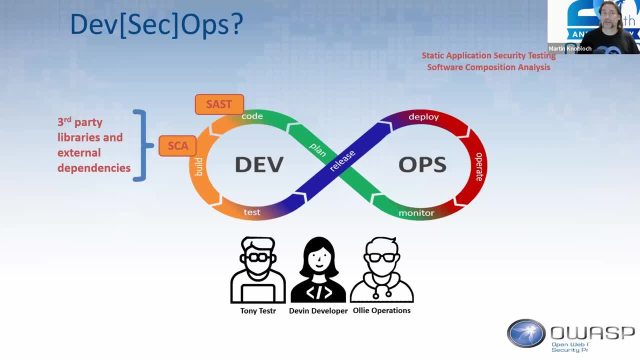 They have not a problem, because only when you use Lock4J correctly you don't have this problem. But then, yeah, do you want to risk this? It's a choice, right, It's always, risk is a choice. So after that you also can then have DAST. 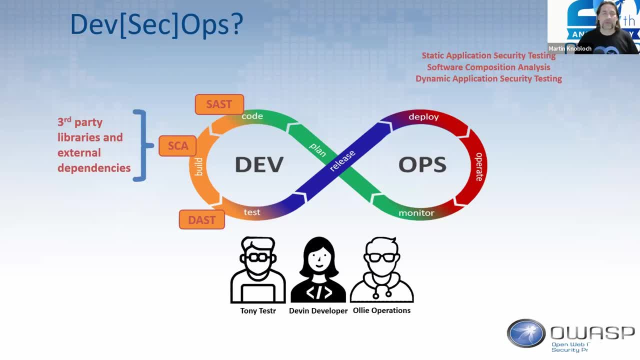 And it's the same thing. I heard people say: oh, the DAST we set up later when we have a test server or a production-like environment, Ridiculous. The moment you have a testing environment, you can set up your dynamic application security testing. 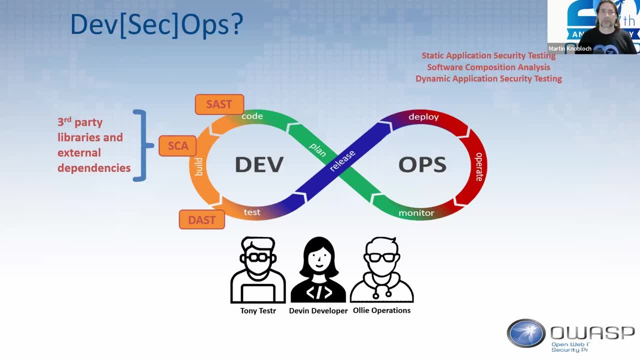 That means in the SAS I look at all the source code. In the DAST I look from the outside. So if a building and I can walk through everything in the blueprints, that will be your SAS When I can click the walls and tick on the windows. 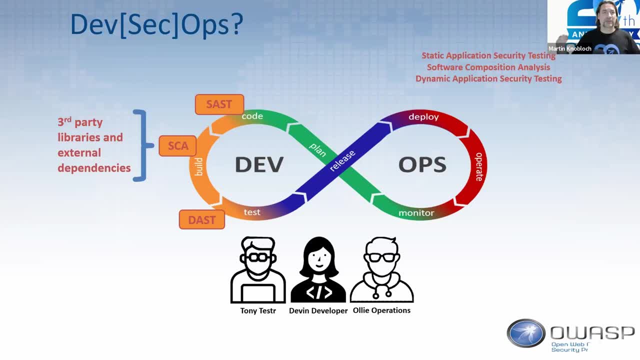 and the doors that will be your DAST. And the question is then, between this, all software knowledge in the SAS and this look from the outside DAST is: where can I link? How can I link the vulnerabilities I find in the one environment to the other? 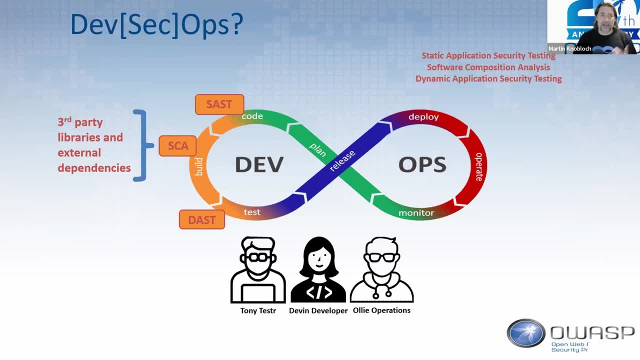 That's not easy. The other side is: when you have SAS, is the one better than the other, than DAST? No, You need both. When SAS, yes, we said there's all tools in there, but what is about the dynamic vulnerabilities? 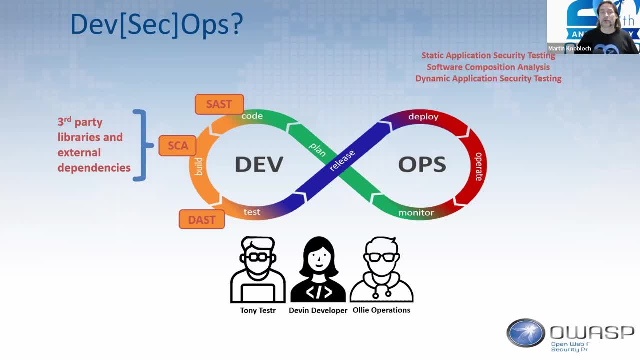 like cross-site scripting, cross-site request forgery, where some controls or mechanism measures are outside the source code. you can verify that, So you have to alert. but it's not relevant, It's not a false positive, It's an un-relevant finding whereby in DAST, for example, 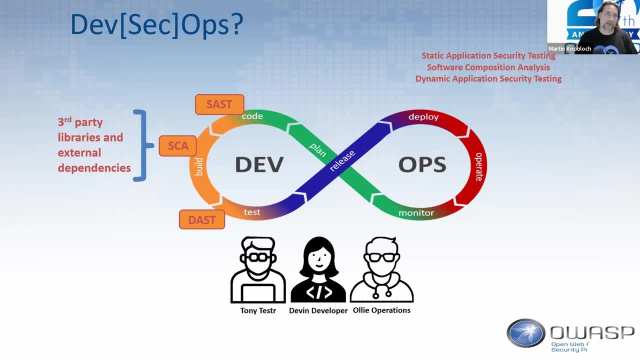 SQL injection. I cannot find it. Maybe I missed one path in the way how I can actually trigger SQL injection. I would miss it because I look from the outside and it's a black box for me. So you need both. you have the full visibility. 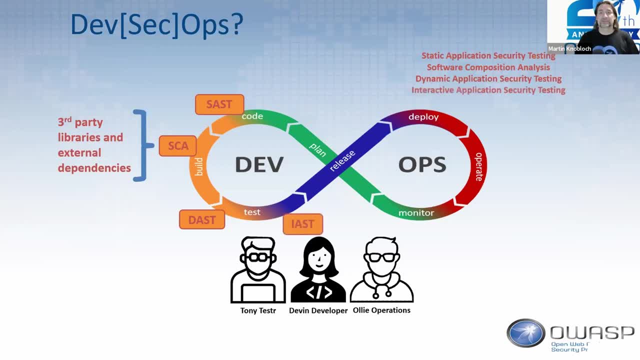 and the interaction. And then the next step would be an IS what is currently set to be hot- where you have an agent monitoring the virtual environment, where all happens. So you do your DAST testing and you measure your monitoring, your target moment: the virtual machine. 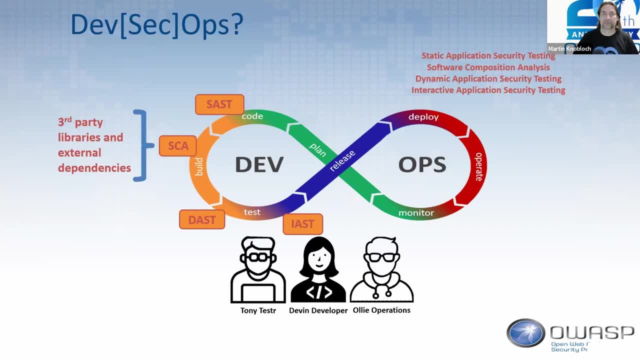 where your, for example, travel runs and what happens if it behaves correctly. right. So SAS static, SCA is the software composition analysis, DAST is dynamic application security testing and IS is the interactive, So you interact with the application monitor. yeah, 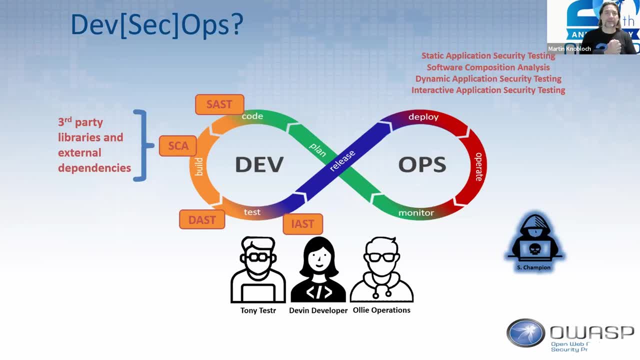 And, of course, we have now our security champion right, Because it's DevSecOps. We need a security champion. As I said, it's not the one who should fix all the security issues right Or just mark them as false positives. 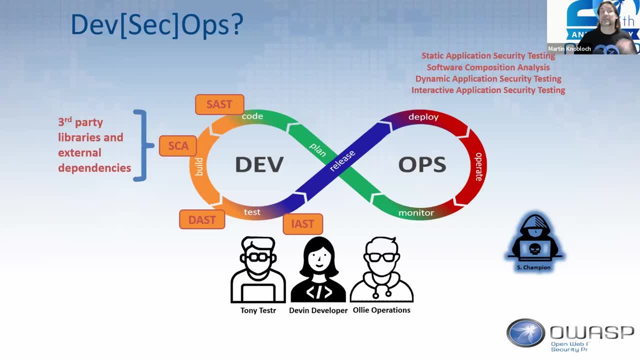 No, it's more than that and I want to go into that later on. But in the past was that: oh, you do all the security things and the rest can develop right. That somebody, yeah, so the shift left was shift, all those things you don't. 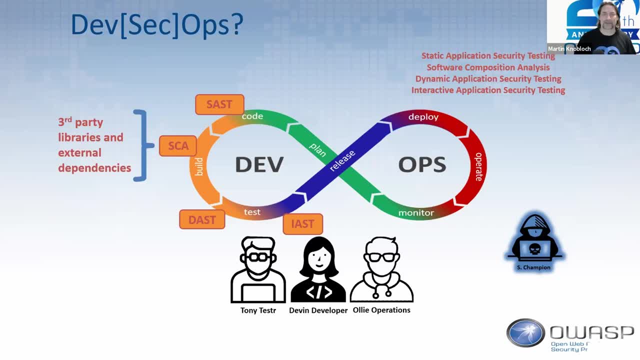 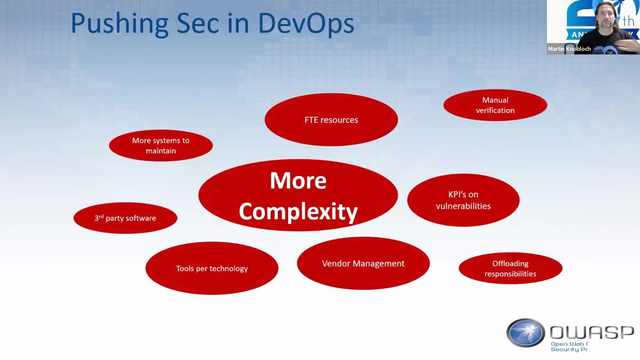 want to do as a security specialist off to the security champion. that will not work Because there are problems. There is a problem when you push left incorrectly when you're doing security. just push off to DevOps. Trust one is to add more complexity. 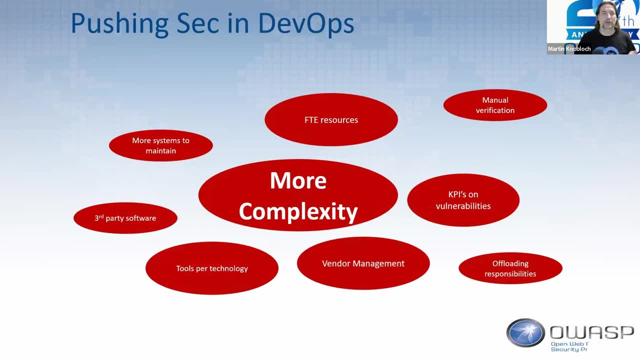 Security has abbreviations and namings the developer are not aware of, right. So the complexity of what is now a cross-site scripting, what is tag naming? I don't know how many people of you can explain stuff like that. What is the real problem now with the cross-site request? 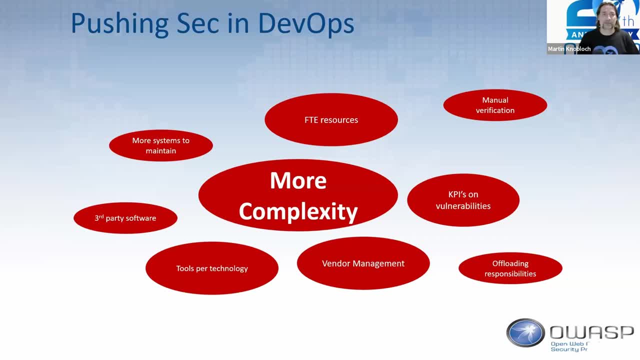 for tree and stuff like that. So it's the new complexity. you need to have knowledge and have training. So you need- then you have- more systems to maintain all the SaaS. DAST SCA IS tools. Somebody has to maintain it right. 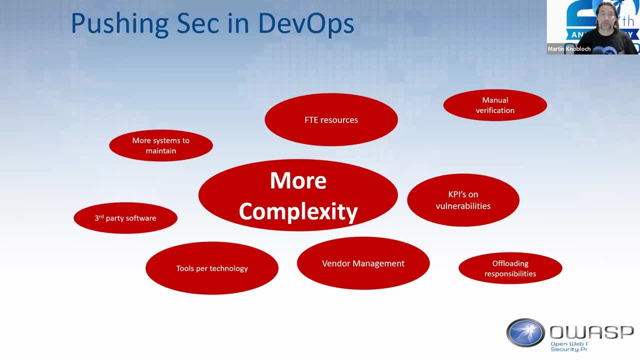 You need new software, new third party software. You have a tool pack technology. Maybe one offender is better for those and the other offender for others. You need both of them. both are not cheap, So you need vendor management And, of course, our security specialists. 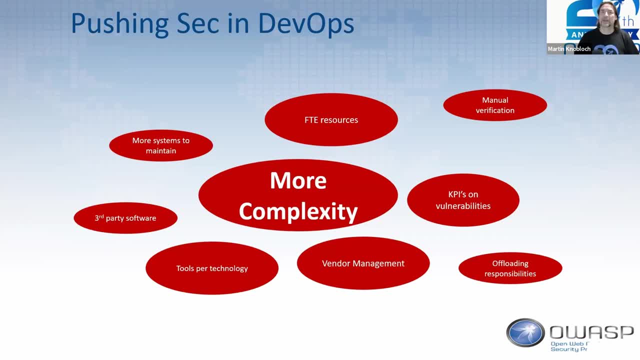 they get KPIs on finding vulnerabilities right. The more vulnerabilities you find in applications, the better you are, And when you are doing automated, you need a manual verification. That's the security champion, right? And of course, it was all about offloading. 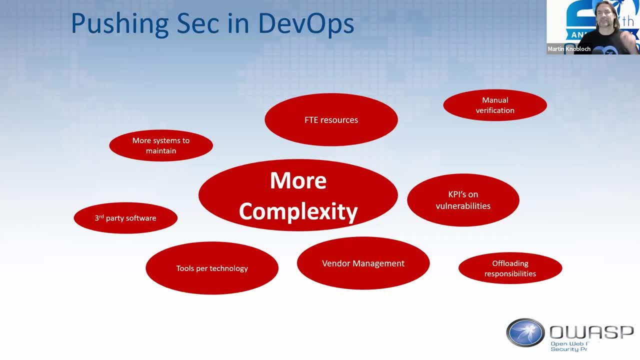 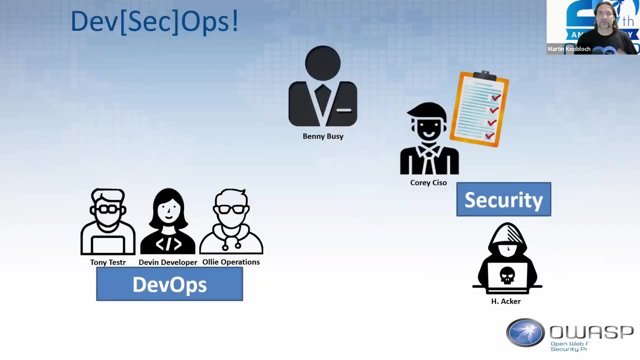 responsibilities to the security to the family. That's not how it should be right. Let me see what goes wrong in that. So one step is what you should do now. sorry, how to make it right. right to the positive side. 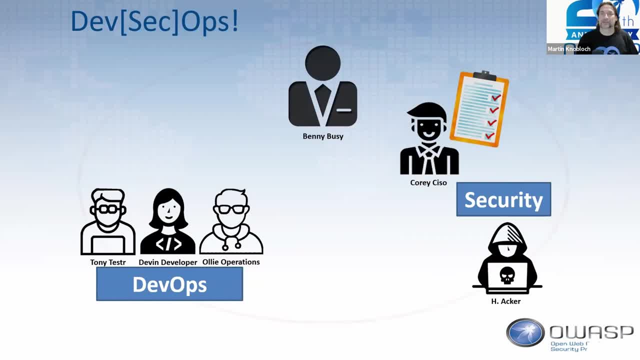 So how to do that? there it goes Again, our players. the first thing we have to understand it's everybody's responsibility. You cannot offload responsibility. When you have to share responsibility, you need also a shared truth. You need more. 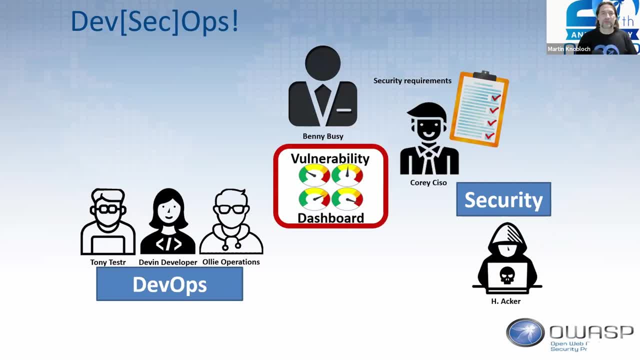 You need one dashboard. I remember times that it was very hard to explain, when you have one data set, that depending on what angle you look at, the data set get different results. These days, with data mining, data analytics, people should understand that. 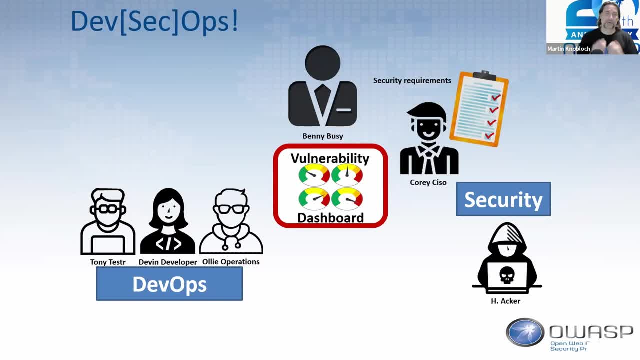 The same data. when I look at it, there's a different context of requests, of questions that get different results. So we have one data set where we keep all the results, one vulnerability dashboard right And there, when it's there already, 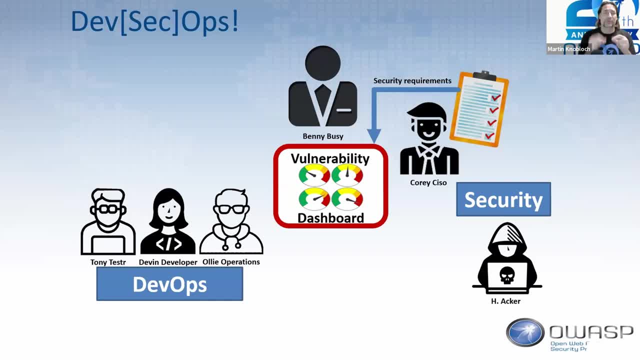 now our security requirements are unknown. We cannot put them in upfront, as Rob said. Then we can define our project that fits into this, depending on which requirement. Is it a desktop application? It's different than it's a SaaS service. 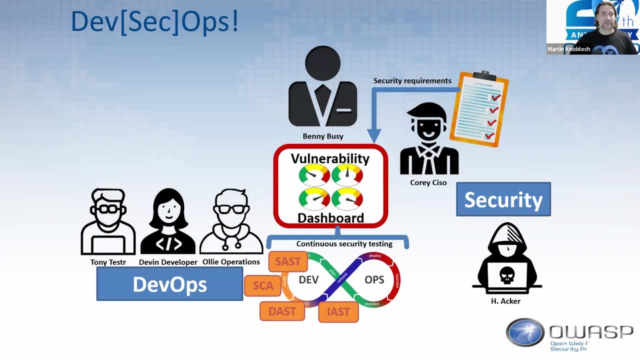 If it's an SQL database it's different than it's a mobile app, right? So system-specific requirements early already in the dashboard. So when I feed my security testing that's always in my testing When I send my testing pipeline into the dashboard. 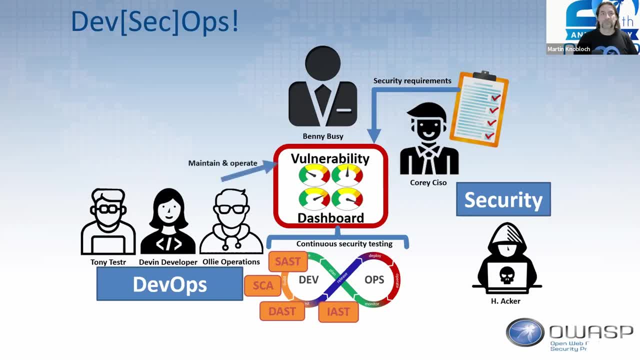 the requirements, match what you need And who maintains and operates the system. Many times, when it comes to where we have the security, they pay the license, so they hire the security group, so they maintain the server where this web application runs on the data security testing. 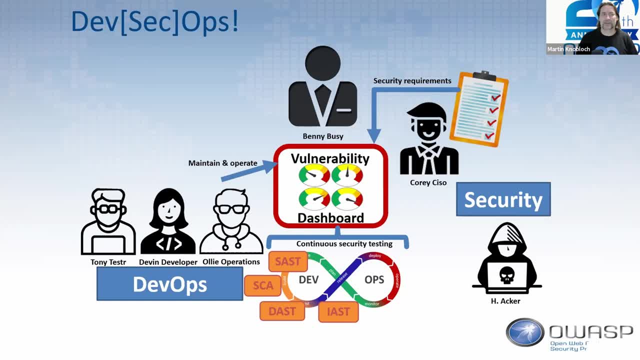 Security will able fit to maintain one system, an IT system. No, give it to developers, Because those tools I just said- SaaS, SaaS, SCA- are not security tools, They are developer tools. So give them to the developers. 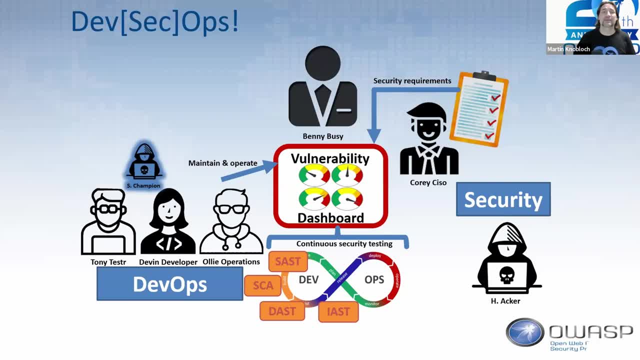 They know how to run the software when it's there, so they know how to integrate. Imagine: whatever you do, Somebody comes: Hey, here I have this cool tool and you have to link to that And after that comes out, be curious. 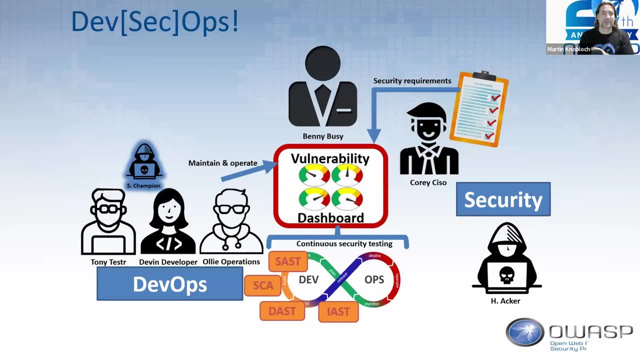 That will not work, So make it theirs. They can early adopt and integrate, And that's where the security champion comes in place, because it's the guilt, or whatever the tribe, of security aware developers. It's not a security person, it's a developer where you have security awareness. 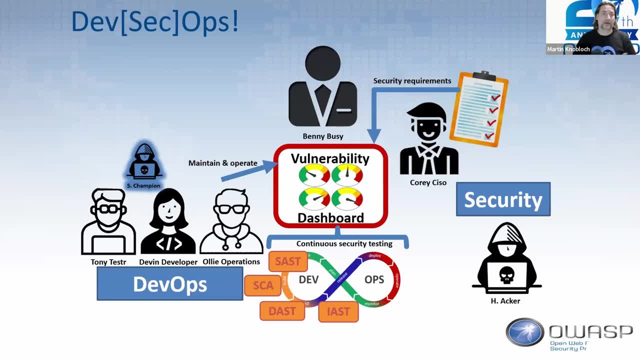 And they are those who maintain and operate the dashboard. from the technical perspective, They are responsible to integrate your build pipeline results, test results- to the building dashboard. Yeah, it also means that now penetration tester can do what they are made for right. 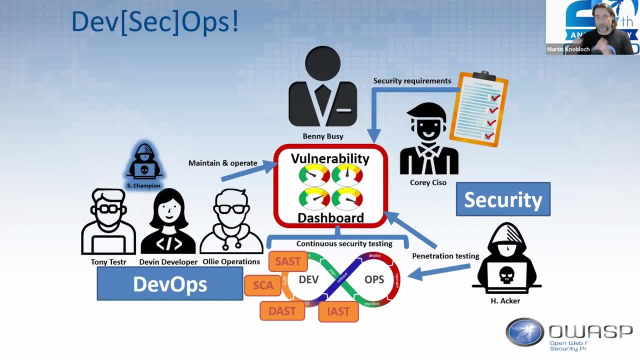 They're human so they can spend on find vulnerabilities, flaws, functional vulnerabilities that a tool cannot find, Not just a box. I don't want my security resource. it's not cheap to spend time on report cross-site scriptings, please. 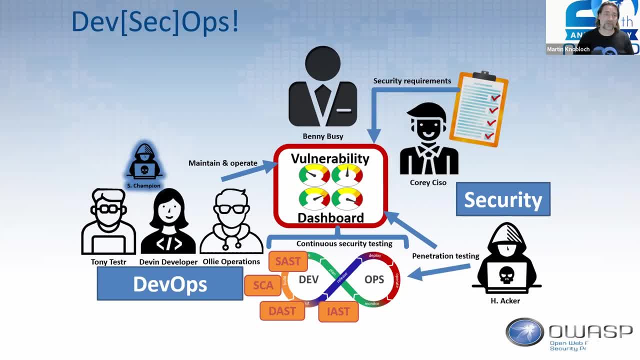 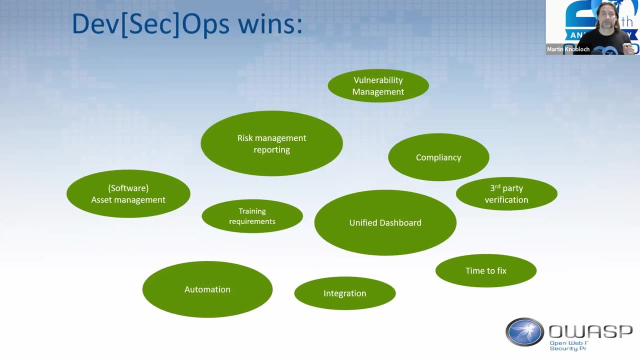 No, we have tools for that right, So we can increase the tools and increase the testability of our applications. So it's a shared responsibility for security over the teams. Now the benefits of this One is one unified dashboard, Maintain operate owned by the developers. 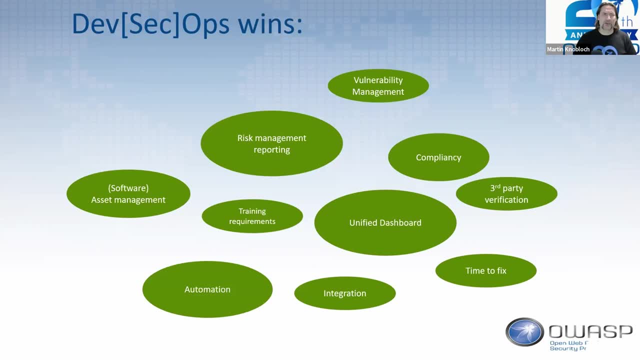 And that can go beyond, not a vulnerability management, this work. I don't want to see a pitch for how many projects I have and every project I can see. oh, they have 512 SQL checks. Oh, now they have only 560 SQL checks. 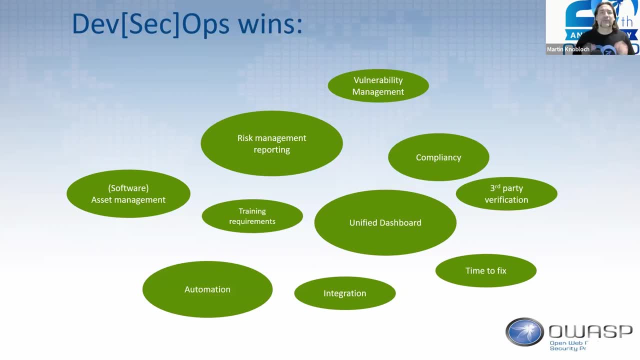 it must be better. No, I want to see the trends in my software, asset management Software. I want to see what software do I have Internally- it develop, but also my external software manage. Because when I was a security guy in my previous company, 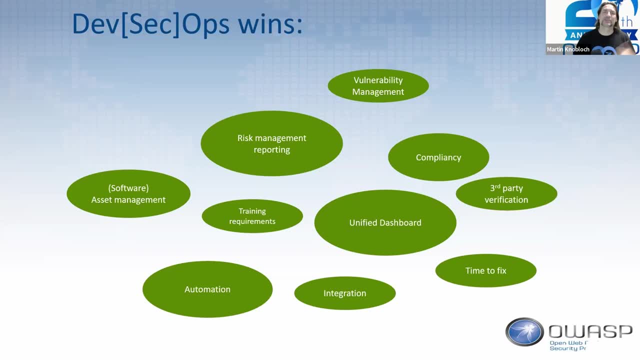 my biggest problem was not my internal software, it was 130 countries. we had HR systems. It's much more complex than my own software. it's a small bit of it. So vulnerability management yes, but software asset management is more important. 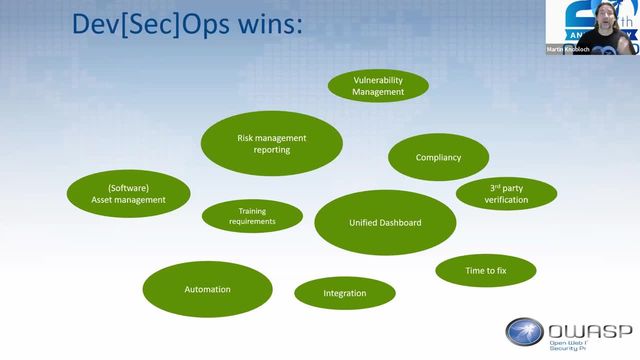 where I can actually do risk management and reporting, so I know what's going on. One unified dashboard to fulfill compliancy, And it also means that I exceed trends. I don't want to manage my company. I don't want to manage. 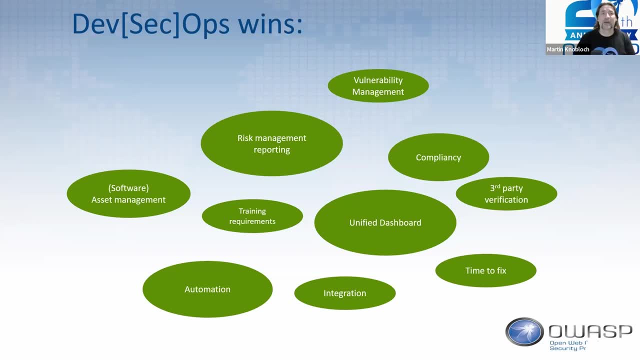 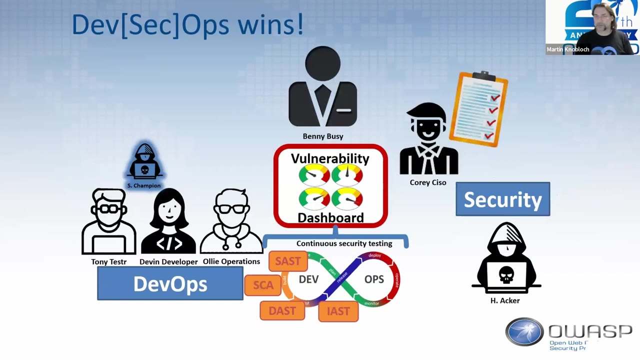 I can manage application projects by number of issues. I want to manage my software development practice by in security trends. Okay, What? how that will be then benefited? Let's go with this. It will benefit like this: They the moment it's integrated. 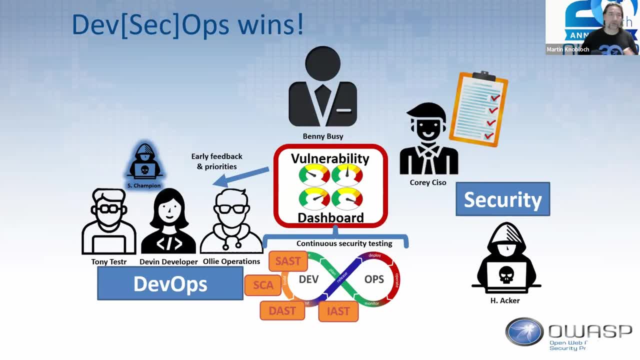 the development gets a feedback. So it's not after the first review, because in the past the security team was the ministry of no white, nothing against. oh, it must be security approved. And now it's the ministry of slow. 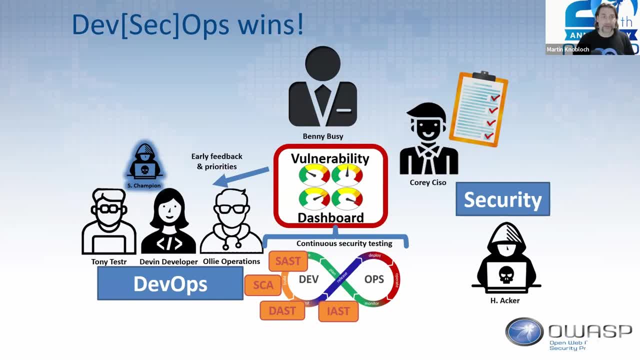 because you have to wait for three weeks or months- imagine that- and you have to security check. That doesn't work for an agile environment. right, I do something. I want feedback When you manage that, when you get early feedback. 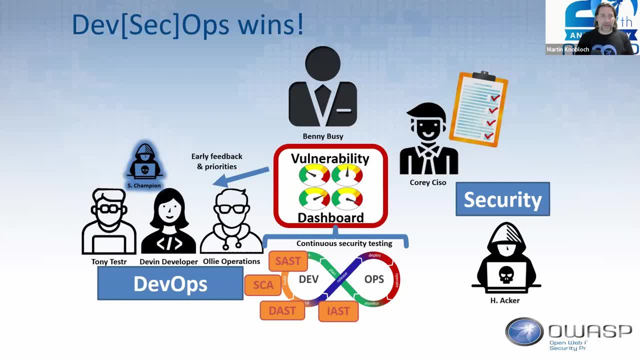 then I know what I have to fix. It's like I said: when I write a book I want to see when I type. I look up, oh, I can touch, type. so I don't type like this. I can type and see, oh, it's misspelled, and I fix it. 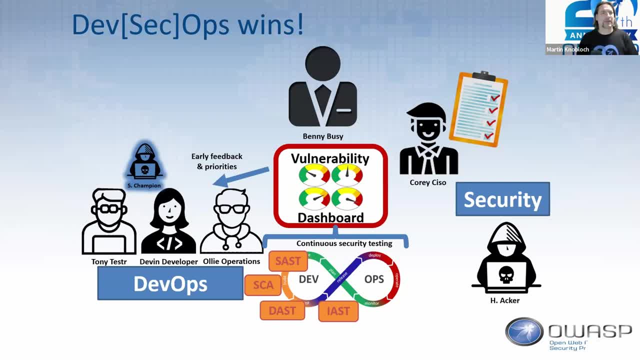 Maybe later on, or I can choose: oh, I fix it before I save it, or before the end of the day. I want to have the choice that I save it before it's pushed to the repository. The other side is the security team. 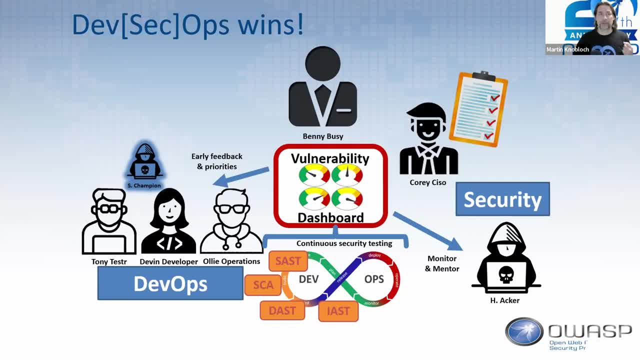 They now have the feedback that they can monitor, not on numbers but on trends. So when I see that a certain part of the teams have been raising in whatever, I can look what is the problem? So what are similarities? So I can say, hey, team one, four and 17 or whatever. 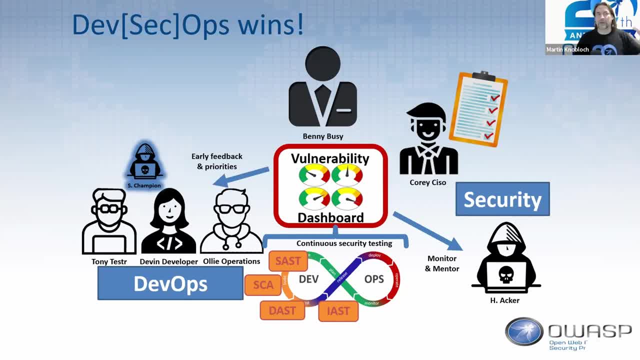 what cool name they have: security champions, you have an increase in this vulnerability. What changed? And then I maybe say, oh yeah, we had a new version update on our front-end template engine, So I can be at once say, hey, who else use technology? 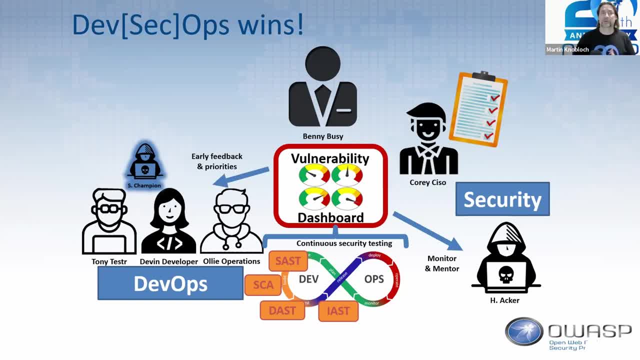 Who is about to update? Maybe wait with the update because I can now manage on trends and say let's see if I fixed the other one. We find a fix or a countermeasure for this security problem. Maybe I can wait for the next release of the template engine. 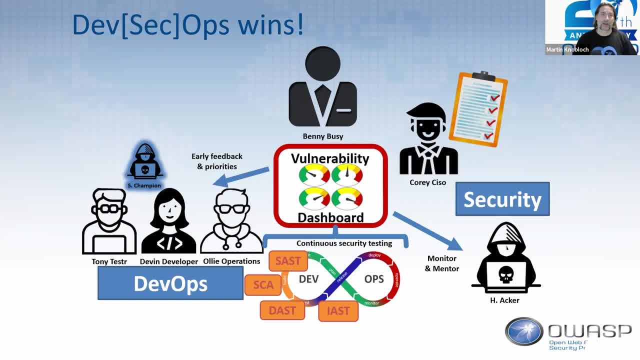 And so I can manage upfront before something goes wrong, and not by total numbers and give them like, ooh, you fixed three SQL injections, You are a good team. It doesn't work right. So monitor and mentor- That's also a change. response from the security people. 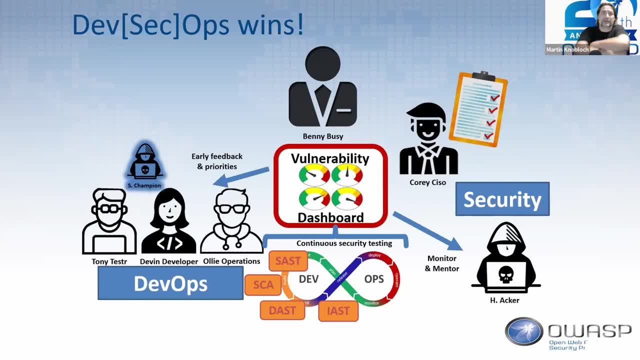 I have seen so many times that I come to developers and they say like I lean back and I'm like, oh, you're coming to do security. I told them: of course not, You're the security guy. They say yes, but do you really think that me? 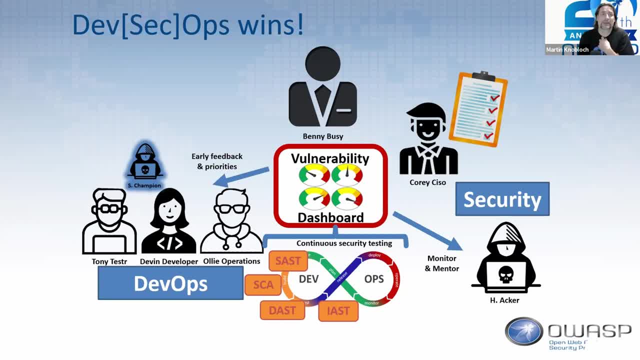 as one person can fix security of something you've built in months in a week. No, I can be the grower, I can be the teacher to show you how to make it more secure And actually when you have good developers. 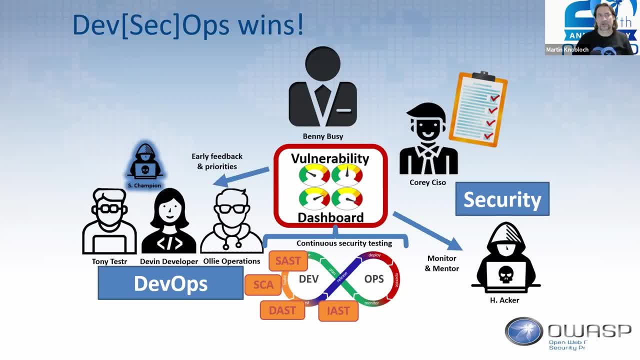 developers who care. many times they know what's wrong, but they haven't got the time or the means to fix it. When you talk to them and give them the ability, then suddenly it will improve. As I said, everything you are made responsible of. 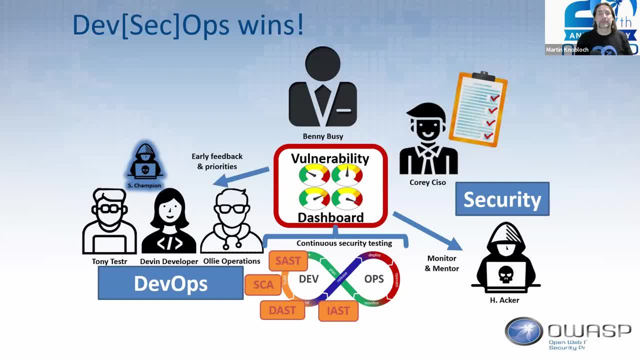 you do better. So the security team can monitor and mentor the development team. That means actually you have to speak with them. And the next thing is then for the CISO: he has control and strategy. If I see trends going up, that means 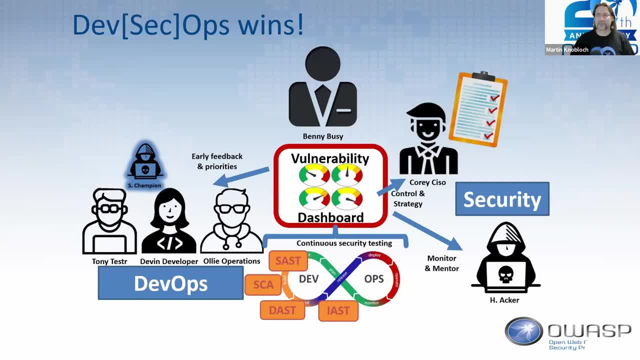 that I have a strategy to which training I need. It's not this, Oh man, Sorry. Mandatory one-week security training every year. that rips out the developers out of their context and their NET developer gets in security course teached by PHP. 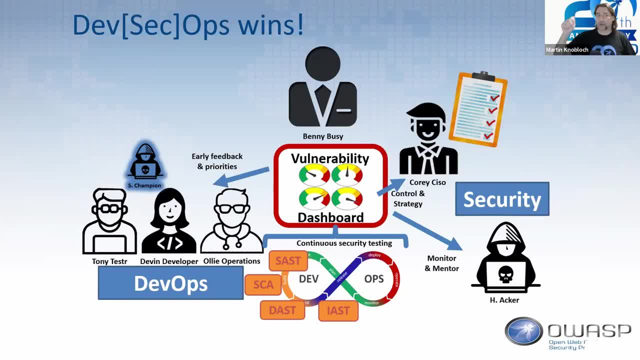 Totally senseless, useless waste of my time and money. but hey, I got my compliancy. Now I can look in what's going on in the trends and can give the right trainings to the right people. Say, hey, you write an application. 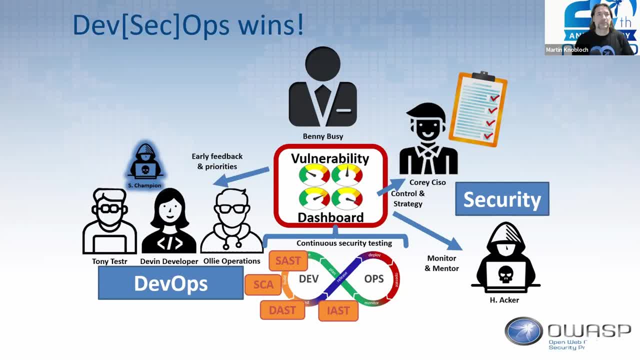 This is a backend application, but you use DB2.. Maybe there's a DB2 security training. Maybe it's a new Azure application. Hey, what's the latest Azure configuration security problems. Why should the DevOps team for the off-person of the teams? 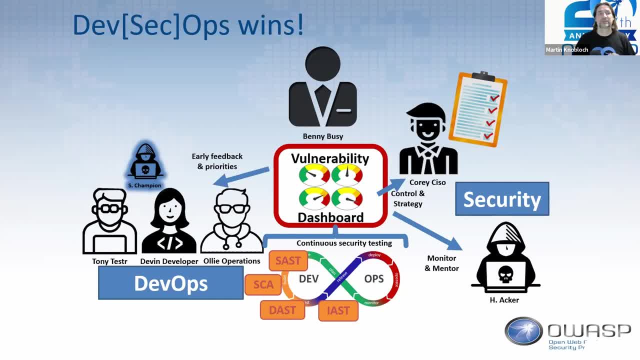 You can manage on trends, predict on trends So important, And of course it means for the reporting, for the business, that they can also see and prove that they're actually in control. They're not surprised So many times we have seen it because that's. 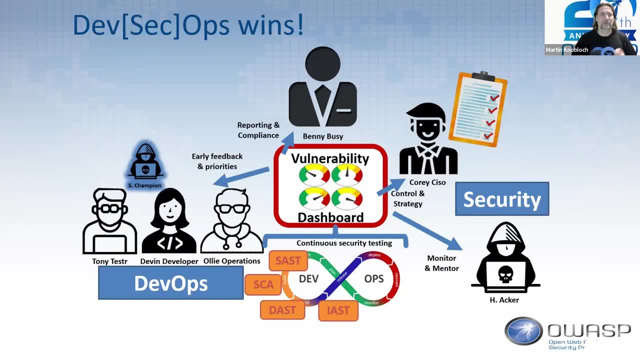 why they say you shouldn't do this, You shouldn't do that. And actually one is vulnerability dashboard. You want a software asset management overview. How many times we have not seen that we come somewhere and ask: how many applications do you have? 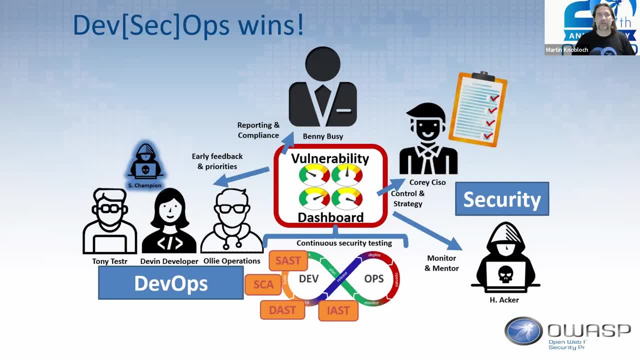 And you get a list that says 100 applications, 30 never been live, 30 don't exist anymore And the other 40, you have never made it to the list. When you have a dashboard, a living truth spread by all the teams together, 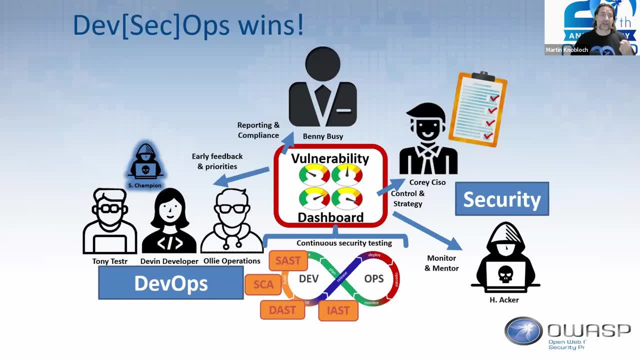 everybody's responsible and has his or her responsibility kept alive, then you can And also you can monitor. Monitor means that teams that do a good job, you let the reins fell a bit, They have more freedom, And those who try to cut the corners. 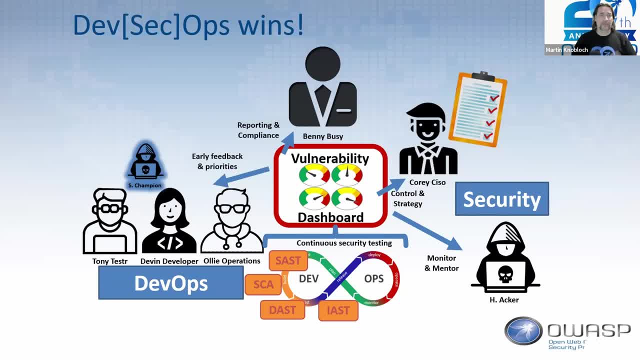 you can pull the reins. Cut the corners means like little kids, like developers are not different than little kids. You do something wrong. I hold you closer to myself. If you do right, you can go a bit further. That's how you teach them. Mentor right, Not punish. I have seen so. 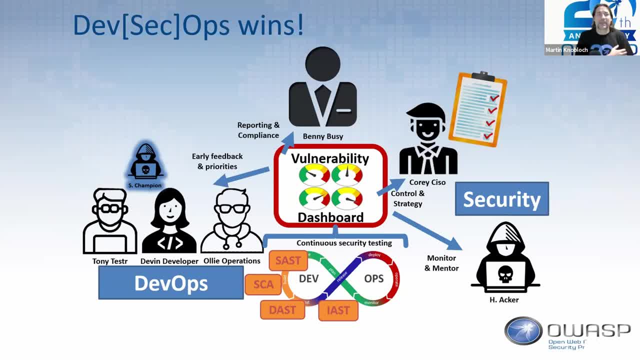 many times when I come somewhere I see a security guy. it's like being hit by the security stick. When I hit you every time on the same spot with the same stick, you see the stick already starts hurting. It means also a different responsibility for the 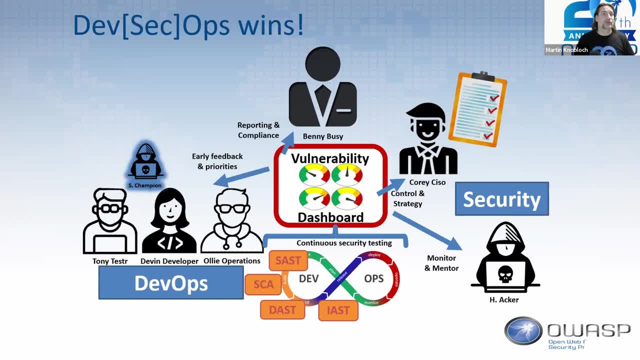 size of it, Because you know now the trends going on in technologies. you have to be prepared, but you also have to be listening to the security people. Maybe they talk to you. you have more time together, speaking and sharing. There's no, definitely this, homeworking times. it's really. 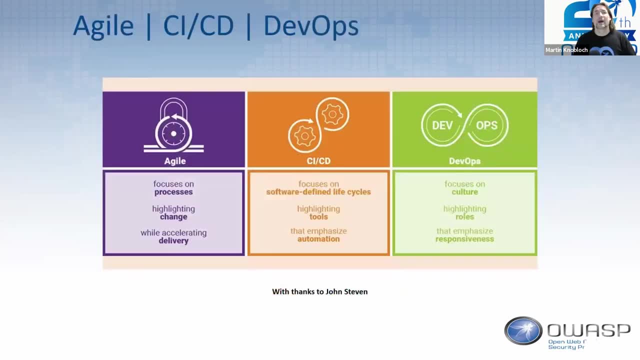 hard, but that's what we need Again, back. I always truly believe when you know what requirement is there, for what reason, it will help you better. We have seen it like. I think the best example here in the Netherlands is the A2.. In the time when it was the old A2, those who remember it. 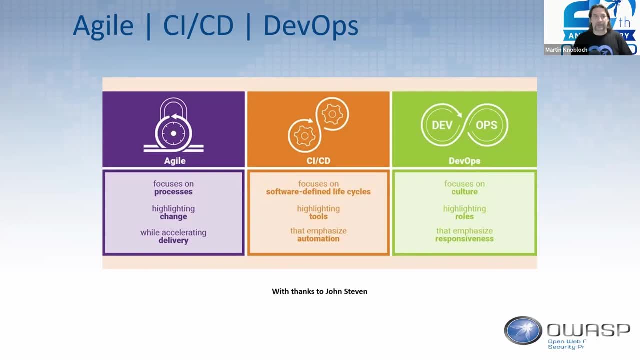 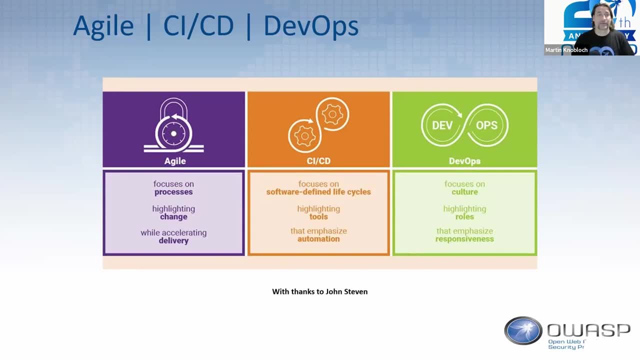 but then you have heavy rain. It's the Netherlands, there's a lot of rain, and then you get a five-lane highway with a better asphalt car, no aquabending anymore, and you can only do a 100. If I don't understand why that is, people will cut corners and then I 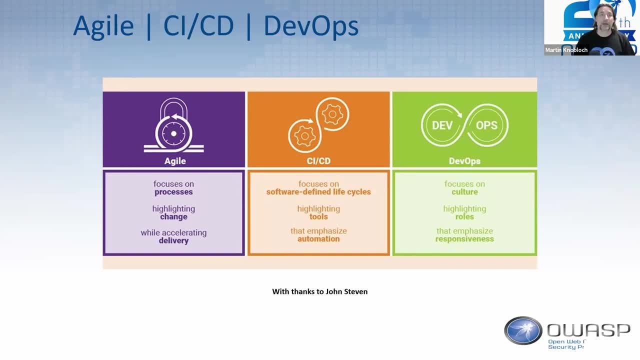 can try to put mess into alert when something goes wrong and can heavily fine them. Well, it's a solution. Yes, they will go slower for this monitored bit, but in between, on the end of that, people will then get rid of their frustration. So, when you teach them, understand them- yes, maybe it's inconvenient, maybe you just have to do something because, but if you explain them, 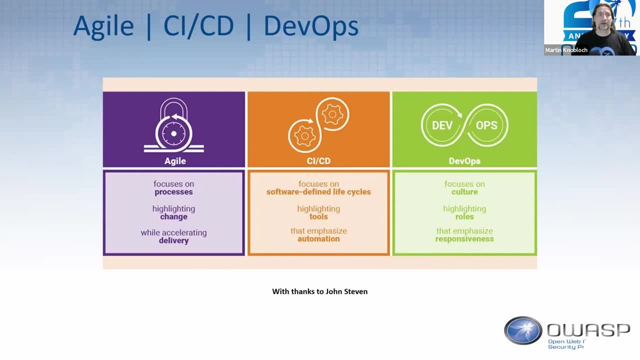 I'm a bank, for example. I have to do this so that we have also our surveillance easier. they will work together, Share your thoughts and responsibilities so they can help you and think with you right Again, action is about a process, Highlight of change, CICD, highlighting on tools, so eliminating the human error. That also means for security, freeing human resources to find actually the right stuff. 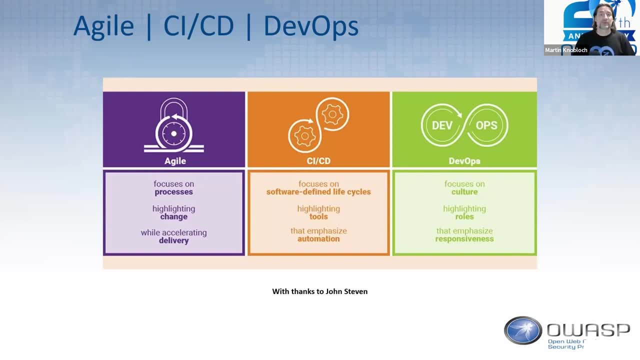 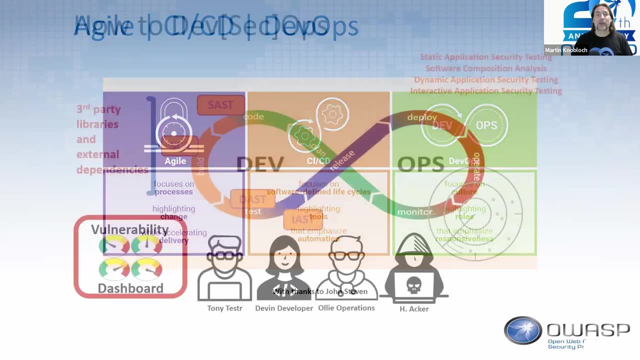 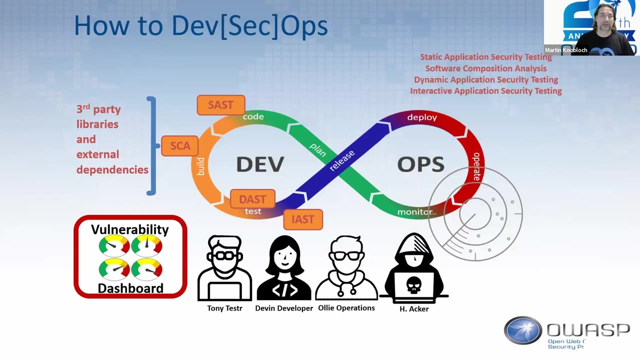 And not forgetting DevOps focus on the culture and it's highlighting on the roles and emphasis on responsibility, And that's a very important one, because when you have run something in this full DevOps environment, it's all the automation tool and your security people checking And you need also something that monitors the right environment right. We all know that the production-like environments- 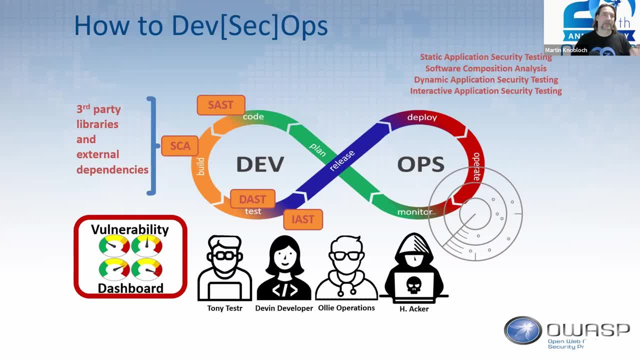 they are everything but production-like right. Most of the times they are kind of production-like. I have seen very funny flaws. that took us a lot of time just because the difference between the Linux Java environment and the Unix Java environment. It cost us like a week of. 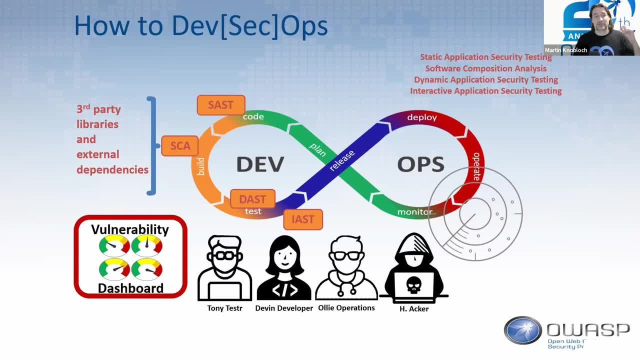 breaking our heads why something goes wrong. yeah, So you have to do security upfront to save money in the bank, but you don't forget the external security right, Your internal checks. That also means maybe something like your OSINT, your open source security intelligence. like: what do you scan, scan, refine about yourself from the outside? It's the list. you have right. It's absolutely valid. 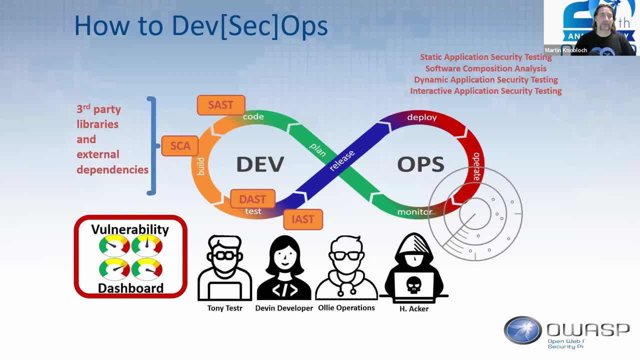 So the whole thing means that shared responsibility is everybody has to do something, but do actually get what you're good at. Security is not good at being the owner of an application or dashboard. maintain a dashboard, No, it's the development part. And they have the experience and the knowledge and the tools. By giving them the tools, they have the responsibility. 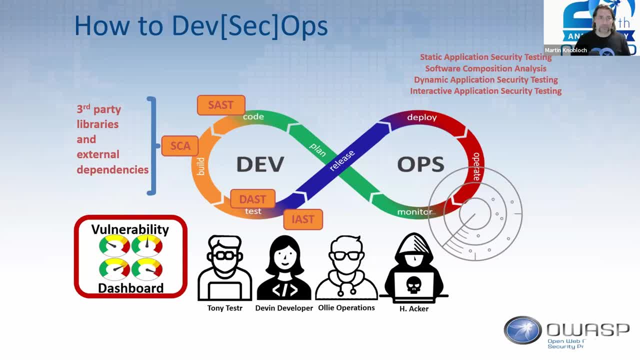 And the other side would be: you have the responsibility, so enable them, give them ability to live up to the responsibility. they have right. And of course, we are not living in a land with unicorns, far to the rainbows. so it's a process. 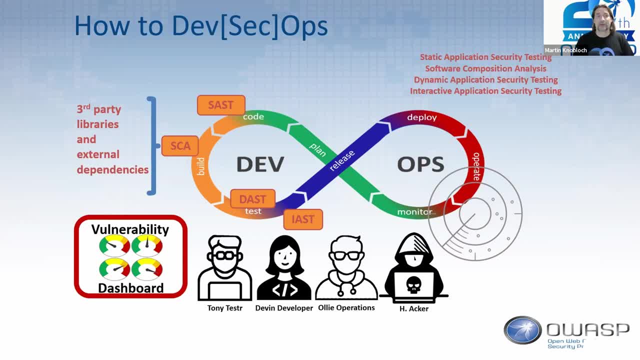 It's a process, a long process, and you start the process and change by listening to them and help them early, not come to the end and say no, definitely not holding them back. That was a bit quicker than I thought, but yeah. 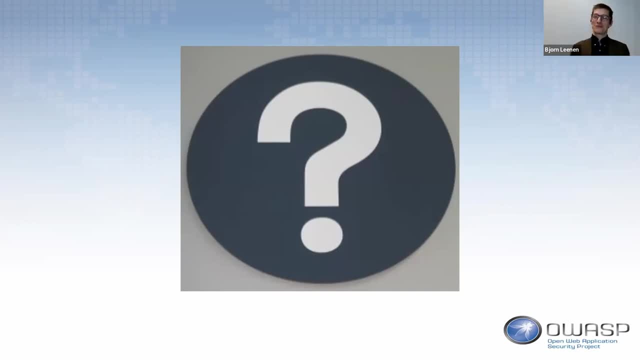 A bit quicker. Well, I applaud you for your long back. Thank you for your presentation, Martin. I liked a couple of these analogies that you made: the department of slow and all the personas that you use throughout your presentation. I mean that makes it easier to make things stick, also because it is describing a little bit of the role that each and every one of them has. 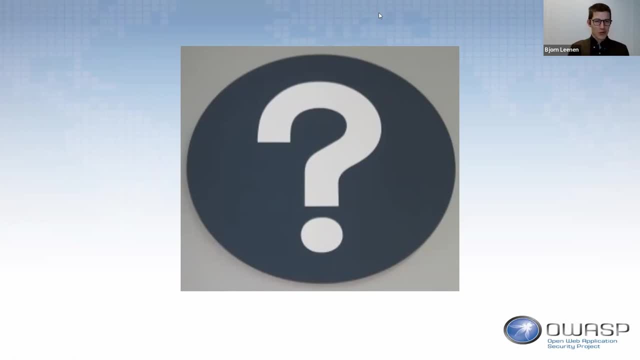 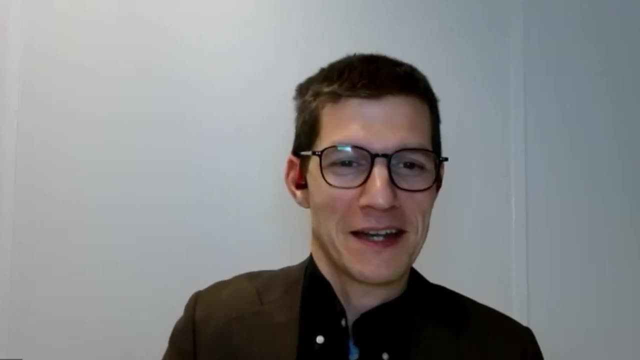 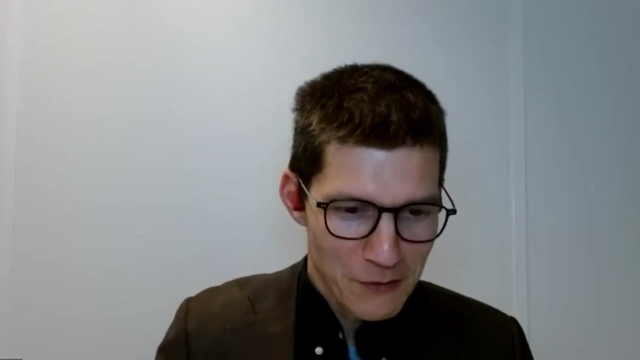 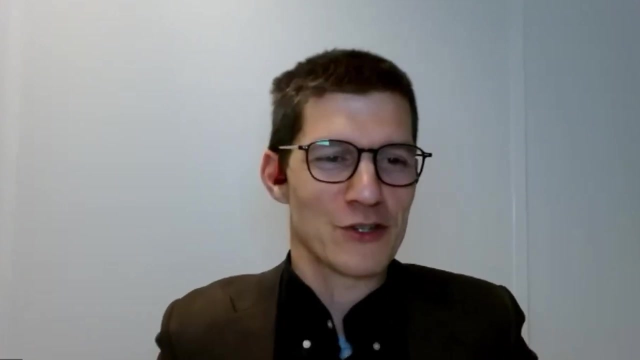 I see a lot of kudos and a lot of questions in chat and in Q&A, So I would like to ask Rob to also enable his webcam And his microphone. Wow, Thank you, Thank you, Thank you. Chet is going berserk here, so let me see if I can make a little bit of straight questions out of this. 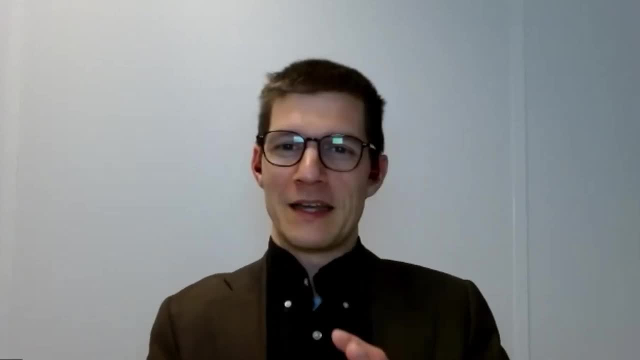 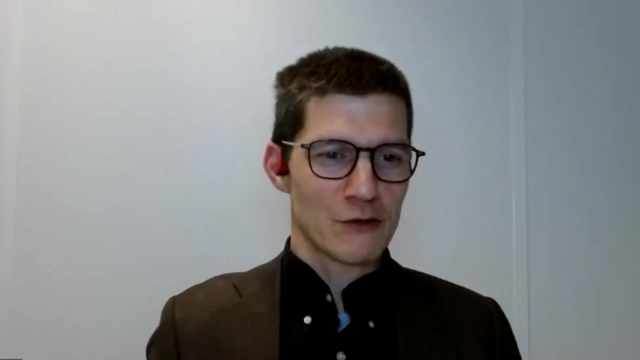 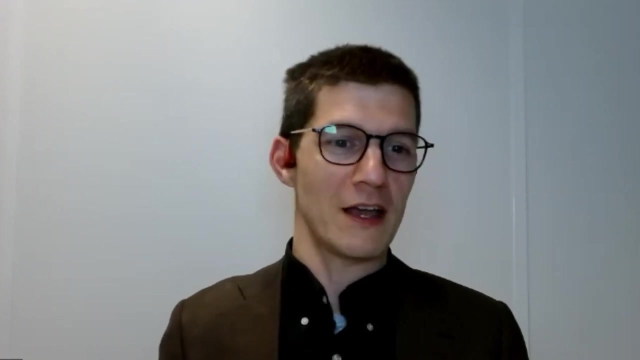 I copied a lot of them from chat earlier, Rob, I see a couple of questions that are specifically addressed to you, so let me start with those. I like your presenting it in the form of a maturity model. Can you share, as if you talk from a global, as you talk from a global experience in percentage? 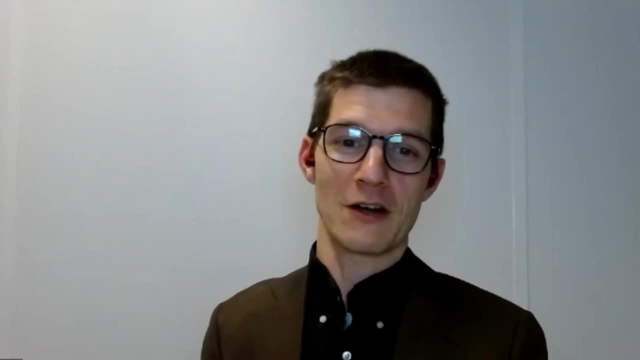 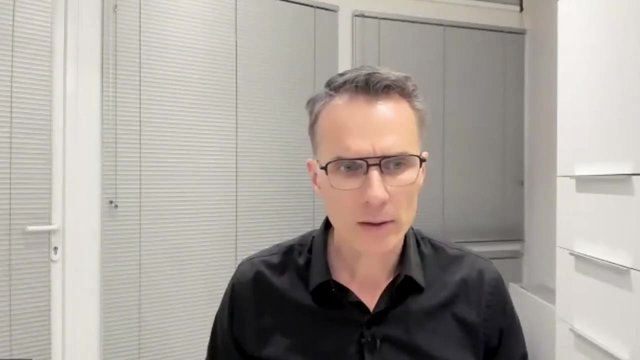 How many organizations are in level four and five and how many are at level two, three? Yes, I looked at that question and gave it some thought and I got an answer. Just pen testing at level two is 20%, So we're talking about number of organizations, right? 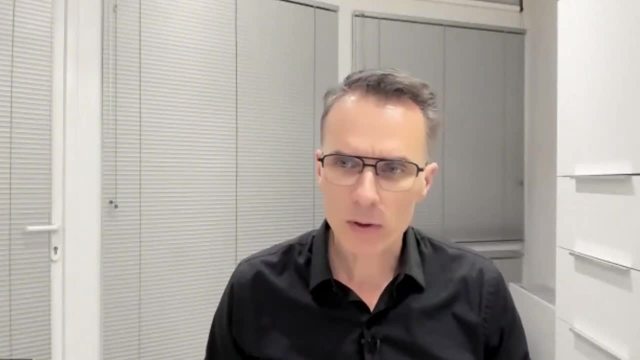 Then level three, having books and hoping that that's covered. That's 5%, really small. Then scan tools: only 25%. And then the big one, level five, trying to bridge that tool gap, So taking steps to make it easier and provide expertise. 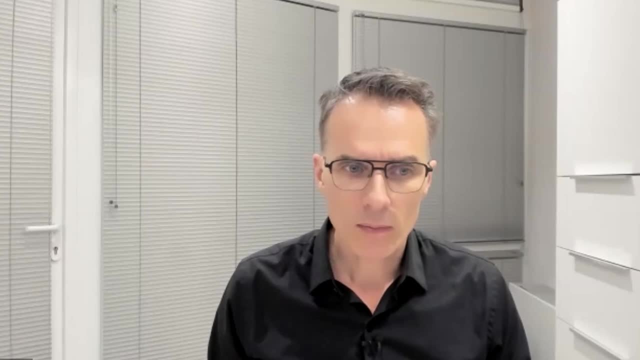 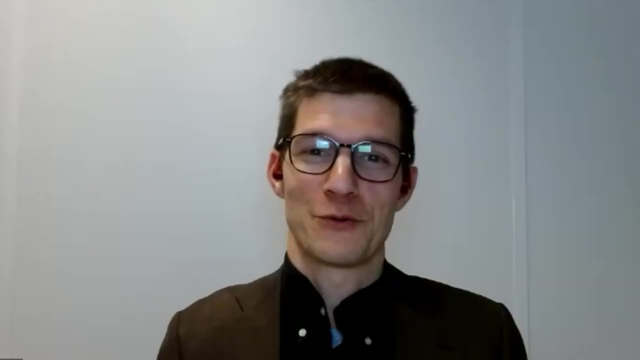 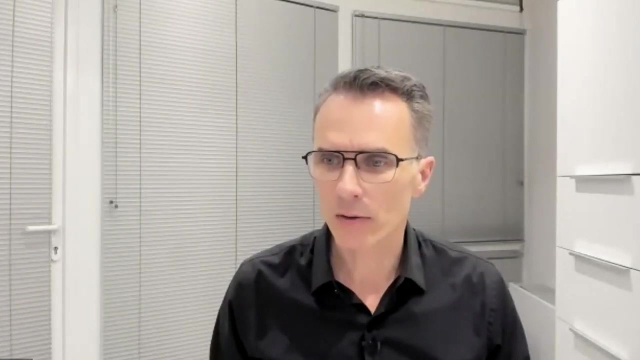 That's 45%. And level six, everything solves just 5%. Okay, so there's still work to do? for the majority of us, I think Yes, but it really is in the air. It's a theme for many organizations. 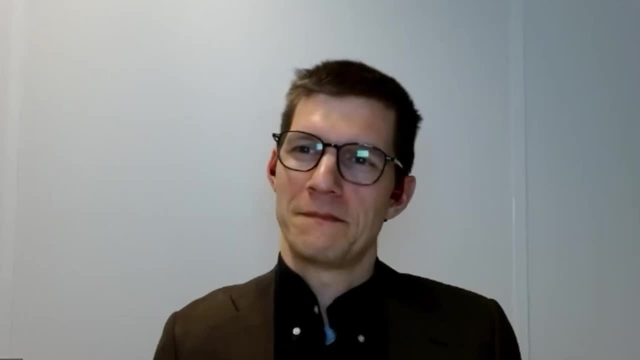 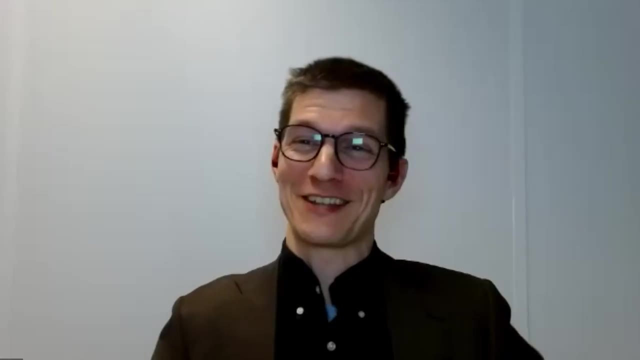 It's really buzzing. I would be interested when you say 25% have the tools, how many use them correctly? Oh yeah, Don't get me started. I think it's not only for software development. Let me buy a hammer. 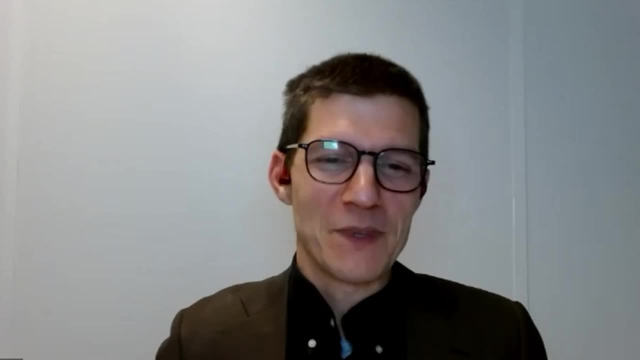 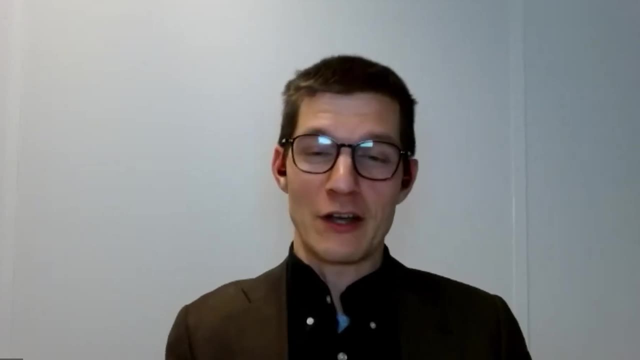 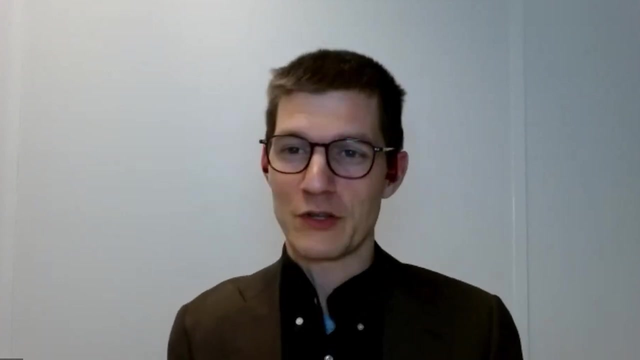 I'm a carpenter. Anyway, I think there are a couple of questions about slides in the recording of today. Let me do this in general: The slides will be shared on our website, And the video that we created out of this or that will be created out of this- sorry Zoom is slowly recording everything for us- will be posted on YouTube. 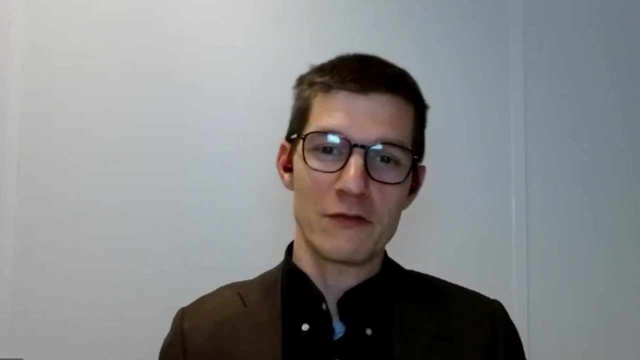 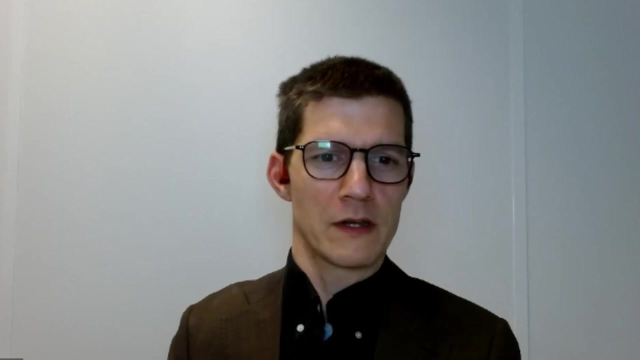 It does need some clipping off at the beginning, at the end, So give us a couple of days, but then it's online on YouTube. I see here, let me see this one is taken care of. I see one for Martin, Rob and or Martin. 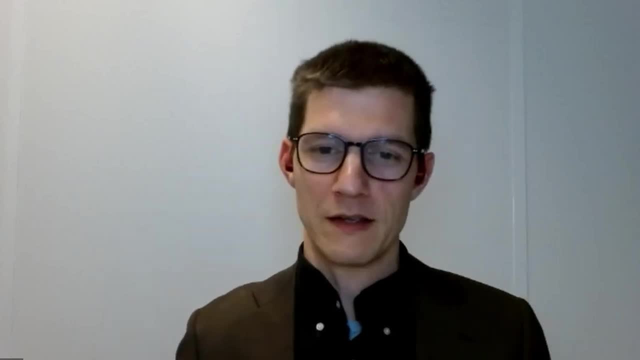 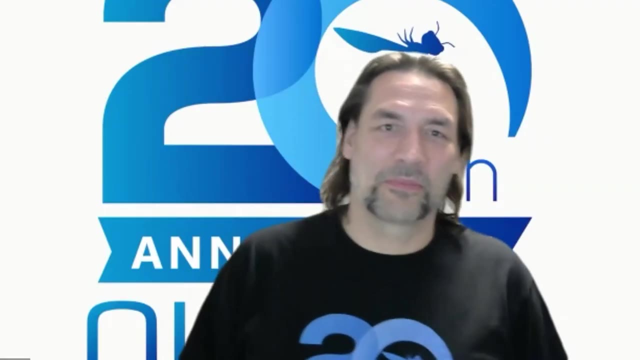 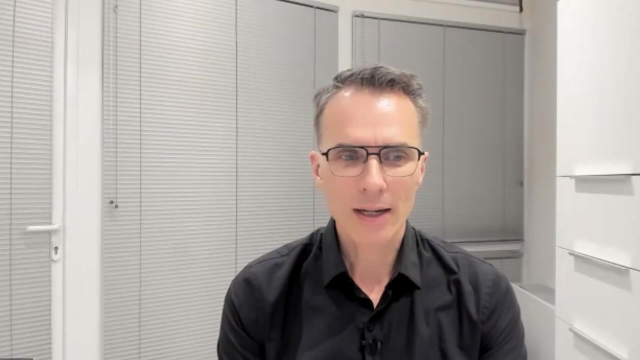 Do you have any opinions on the SAFE framework? And SAFE was written in a kind of strange way. Yeah, that's how you write it. Yeah, Rob or Martin, I can start. I can be really short. I like their community of practice approach. 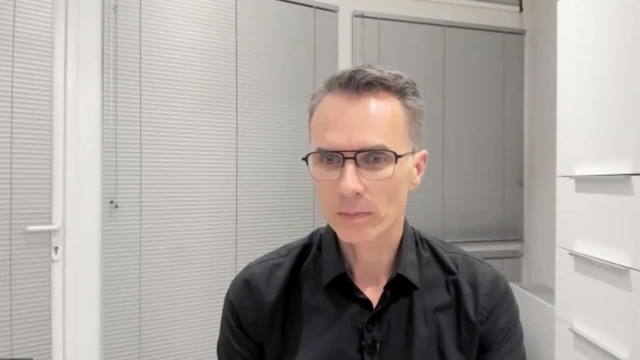 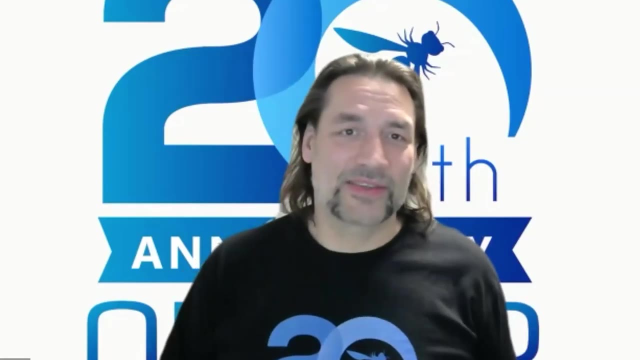 I apply it a lot. For the rest, I'm not an expert. Okay, Any thoughts on your end, Martin? Yeah, SAFE has always been kind of competing, of rejoining the, not with my nice words like cum collega. 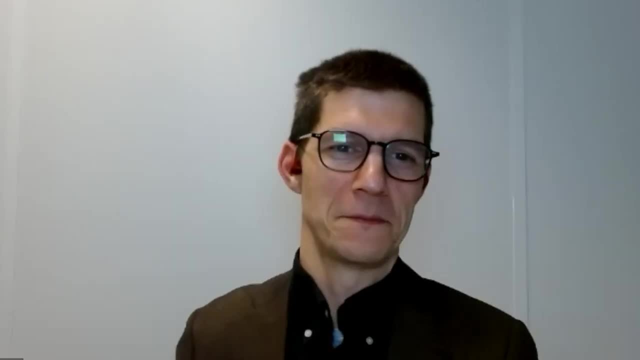 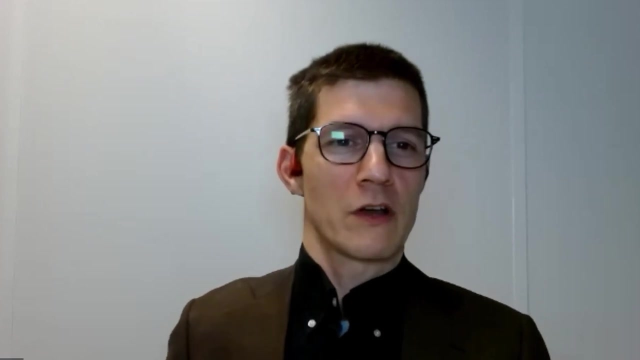 We are operating kind of the same field And we enable each other and work together, Awesome, Good. I hope that answers your question. Let me see, Because Mr Kumar or T Kumar asked: like payment card world has PCI DSS, Is there a worldwide standard of secure software development? 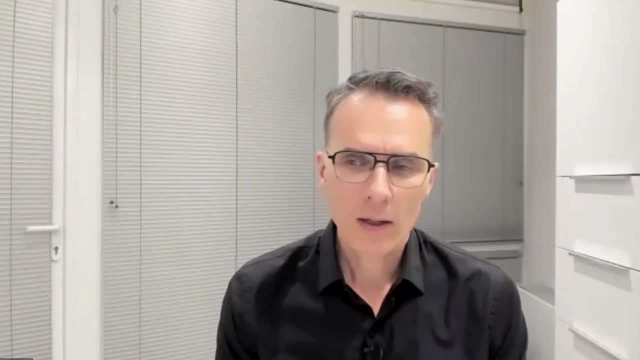 Martin can extend my shortlist. I think I recommend to Google ECSO syllabus. It's a great publication that lists all the standards out there at that point in time. It mentions three that I would highlight as my personal favorites. It's OWASP, SAM, of course. 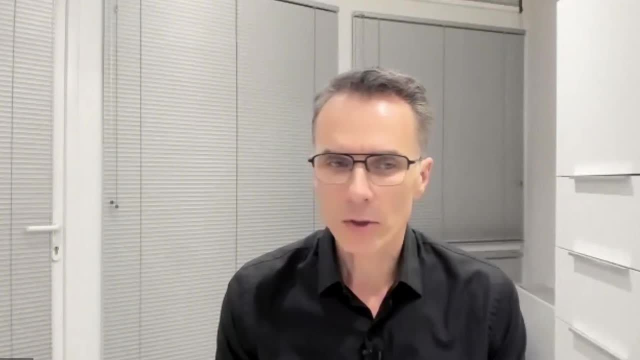 It's the BSIM by Gary McCraw Synopsis nowadays, which is more data driven, And there's IEC 62443. Which is for industrial applications, But it's actually quite good in describing a generic software development lifecycle for security, If I may add to that. 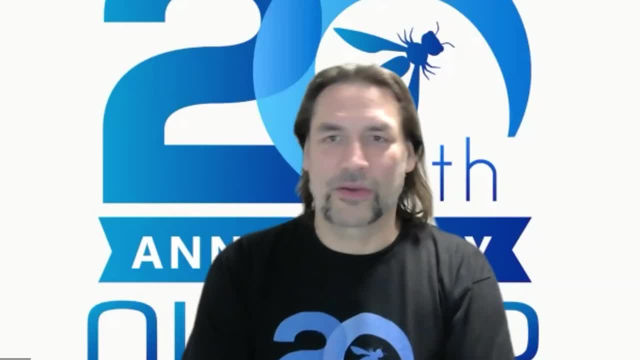 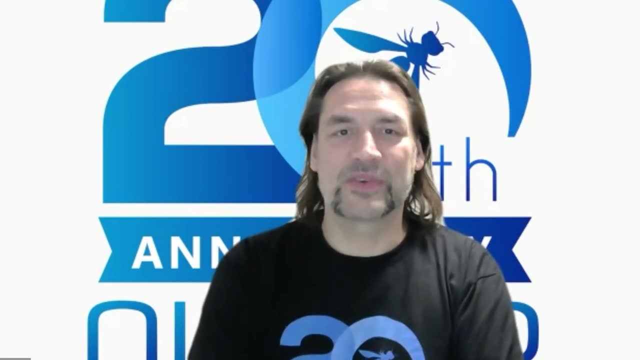 So the thing is a standard of guideline And that makes it kind of awkward. For example, we have the OWASP SAM That has been the open SAM. OWASP is not a standard body, So we have no standardization body. So standard being as a best practice. 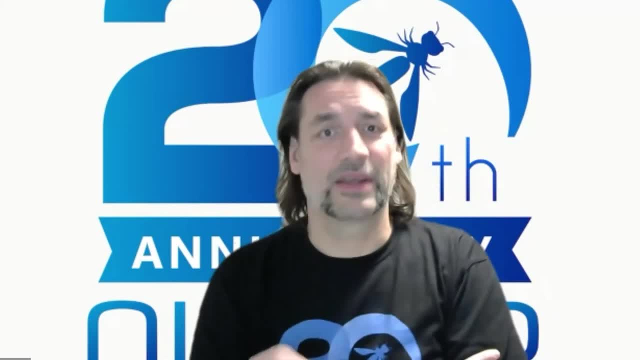 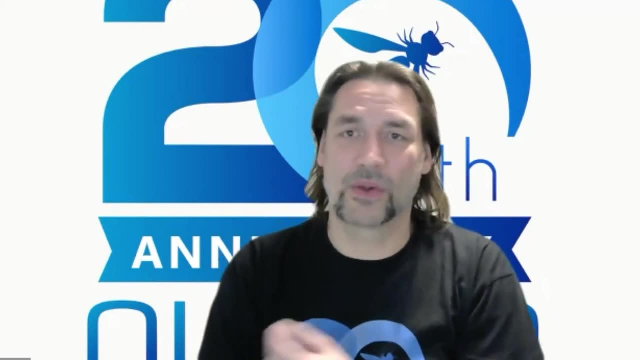 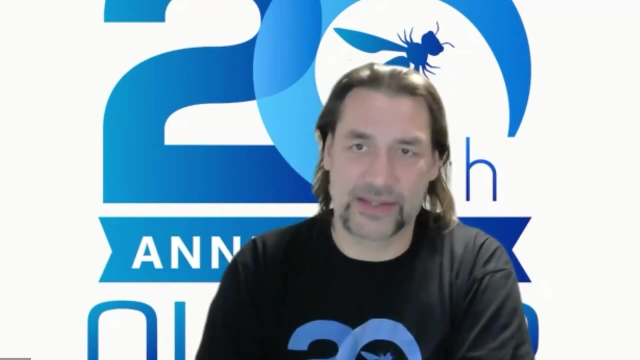 Is something else than a standard being a standard body. OWASP is not a standardization body, So the PCI DSS is actually a standardization body. When you are part of this whole digital payment system, Then you have to be verified against PCI DSS. 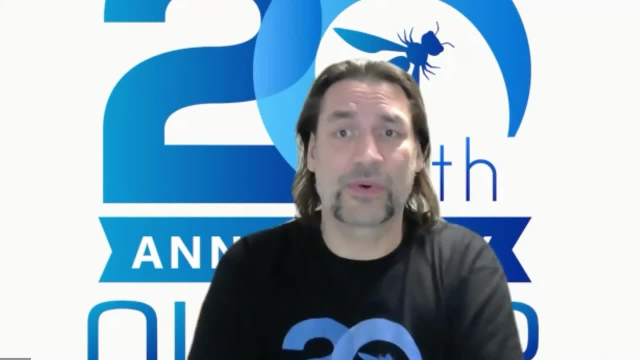 I think the new standard is a different name now And I think it's really good, But it did for us as OWASP PCI DSS. the first version said: your application should be scanned against the OWASP 10.. Great, isn't it. 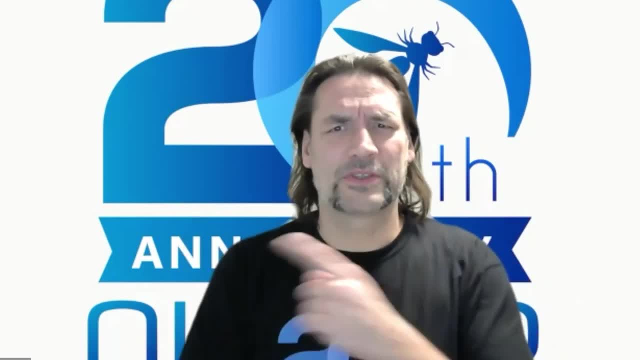 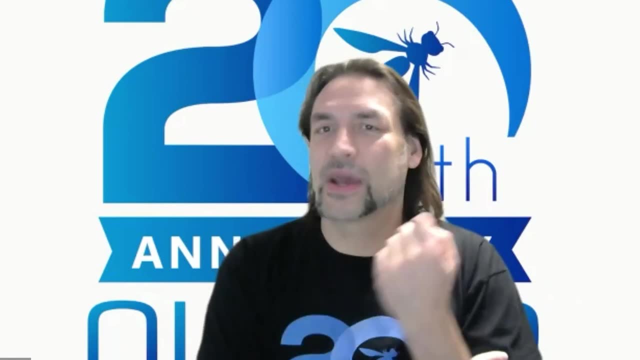 Maybe should I have this in there, or not something in there, And do I have to fix it? Oh, I don't have to fix it, It's also cool. So the standard don't rely on a standard. Yes, you have to do them for requirements. 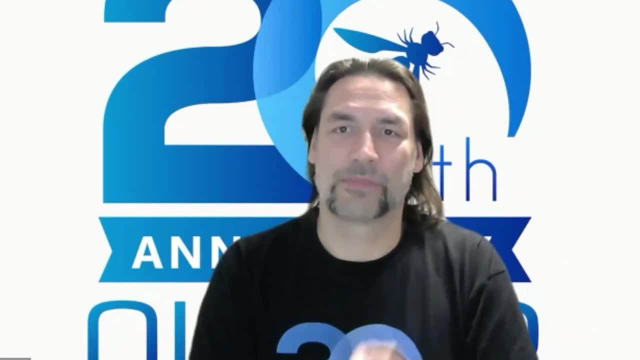 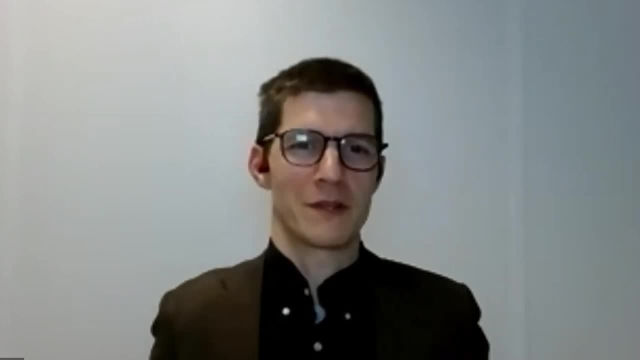 But I don't care which standards you have, As long as you have a practice on where you approach. Yeah, true, Yeah, I think that was also one of the remarks. There are so many. There is not one, just one golden rule. 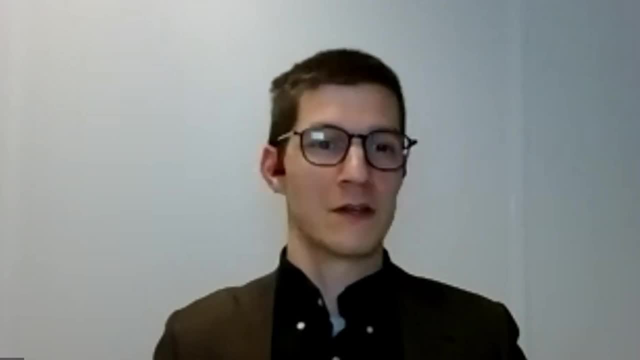 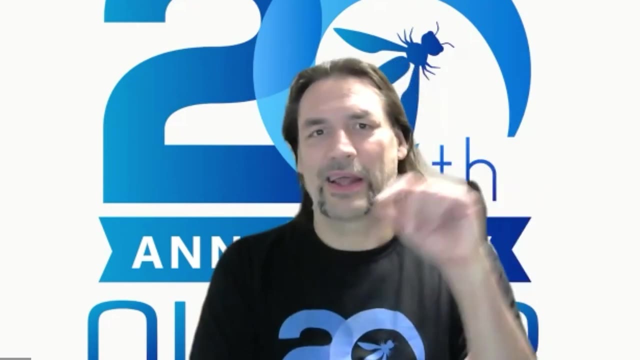 As long as you adopt one of them and stick to it. stick to it. i think, yeah, and a lot of them come from the same inheritance. i know that uh, as far as i know, uh patrick stillman, he had uh like uh- how to call it? uh istanbul, an inheritance tree. 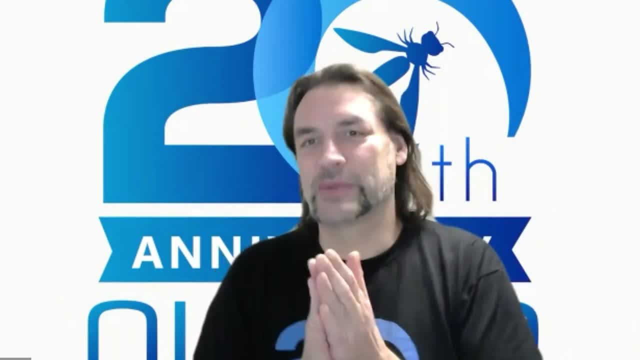 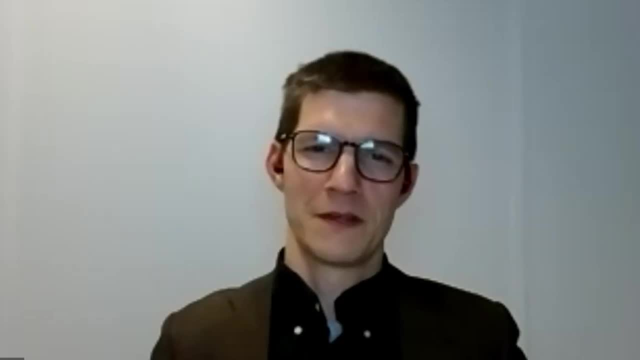 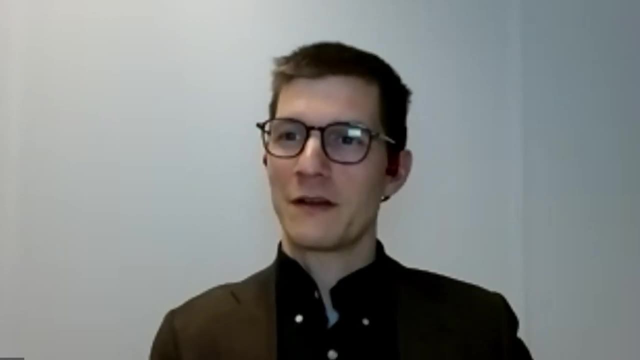 of standards because they try to fix the same and they are specialized for this one on that one. so you have the inheritance tree of standards was really good. uh, project, yeah, yeah, yeah, it's. i think it's the same, as i heard the anisha and and nist pass by a couple of times. i think they 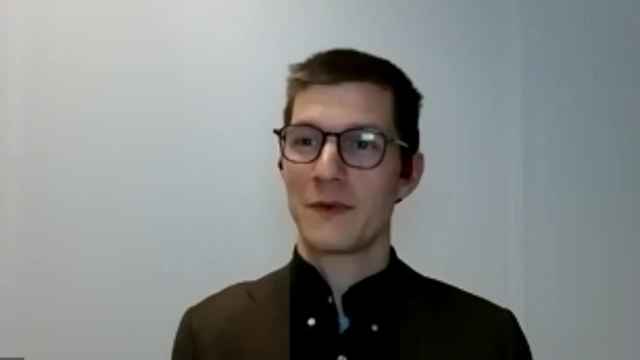 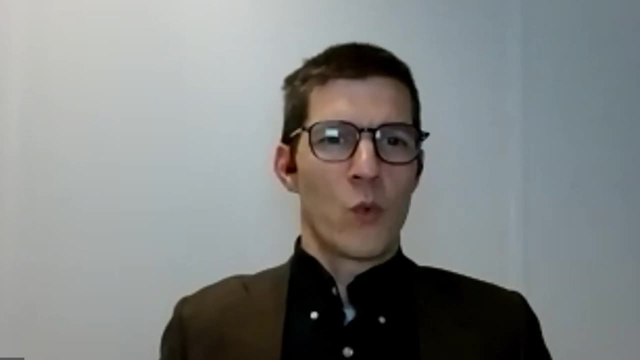 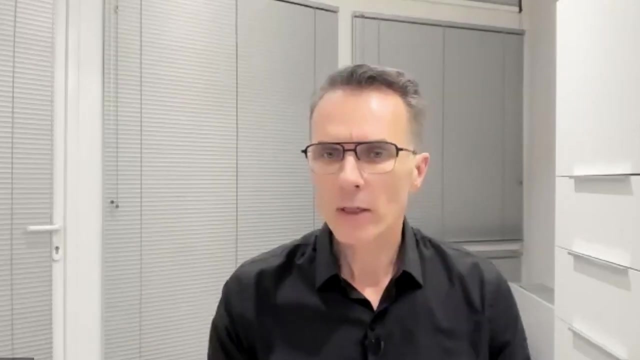 tried to do the same thing, although they come from different uh platforms or backgrounds and regions. what is the difference between hygiene and security requirements? that's a question from hans to rob, because i believe the question was answered in uh in in chat, but i can definitely give it a. 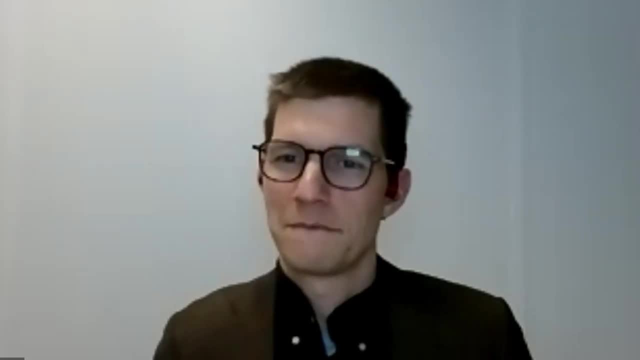 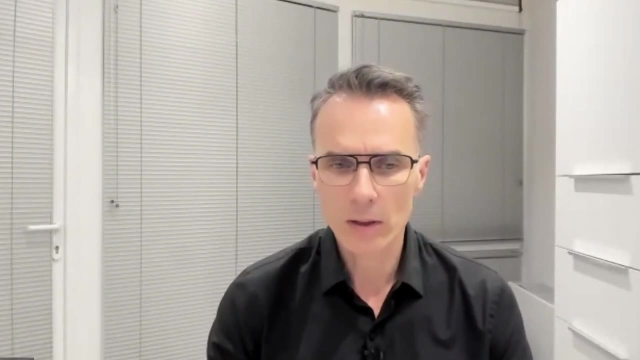 call go very quickly. uh, it's. it's meant to be the same in my narrative. so the idea is: hygiene means things that you do, uh like wash your hands before you go, uh, have dinner. security requirements are like: if you're gonna build, if you're gonna work with xml files, you 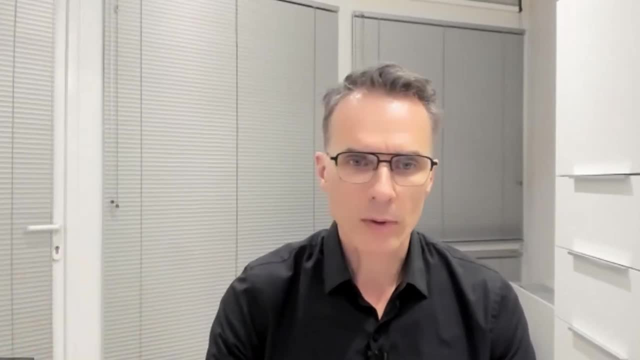 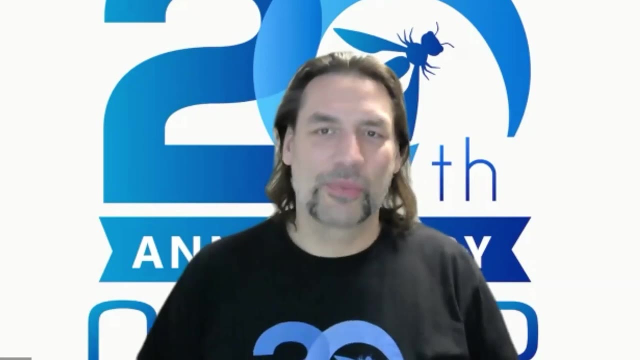 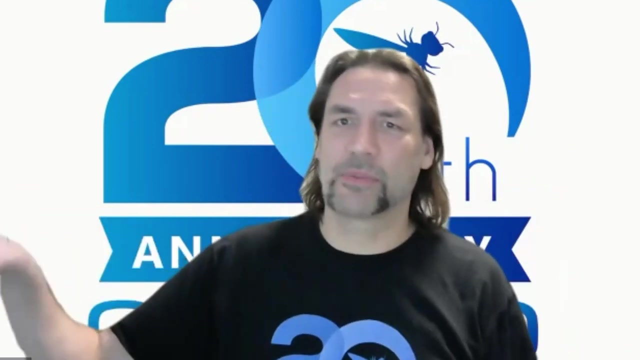 need to have these parser versions and these configurations there. okay, yeah, thank you, that's, yeah, this. what i made is how many times they say: security check. yeah, we have this high important application. there's most tests. uh, that we test. and this is other application we write. 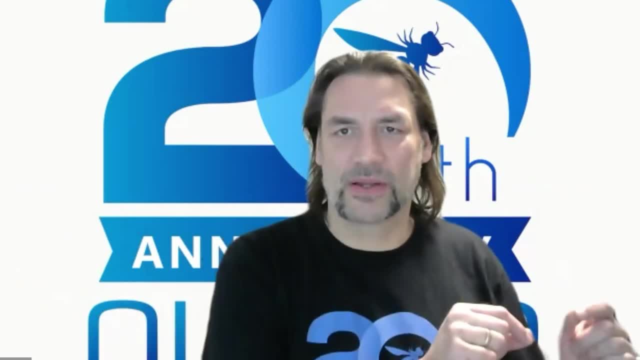 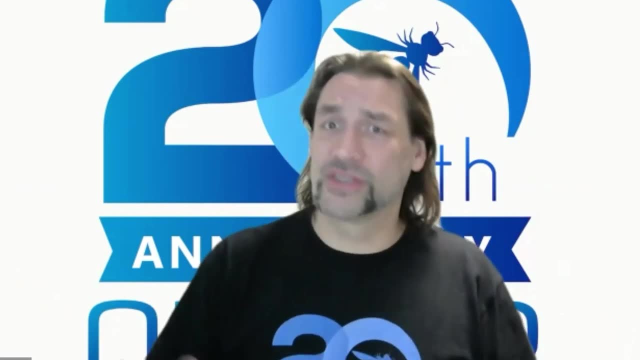 code as we want. there must be a way how we write code right. and they say: secure development doesn't take more time. if it's the way how you just do things and rob says: if you have, if you go to table, i have to send you back to wash your hands, then it costs time but it's in second nature to. 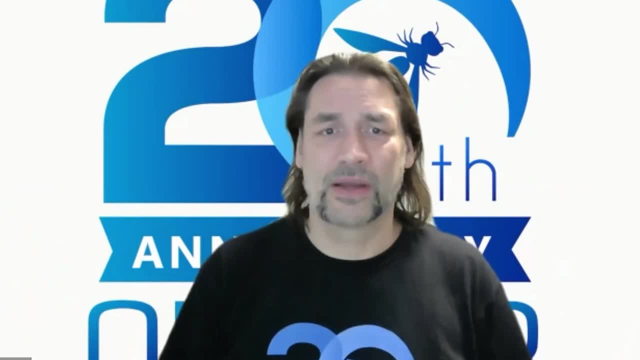 wash your hands before you go to the table. you lose no time, right? so it's not difficult to do that at all, but it's important to do that, and it's not so much about the- uh, the cost of the application and how you do your coding. it's you do it right in the fabrication differs. yeah, and i think that also. 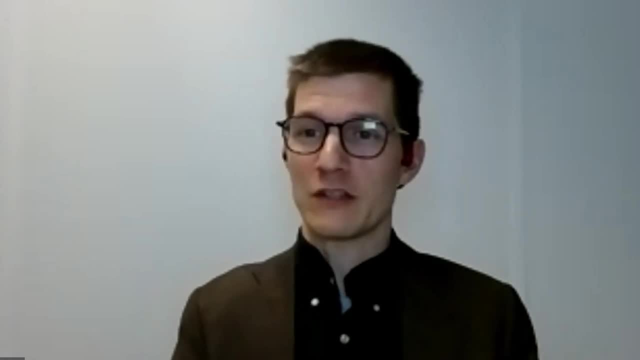 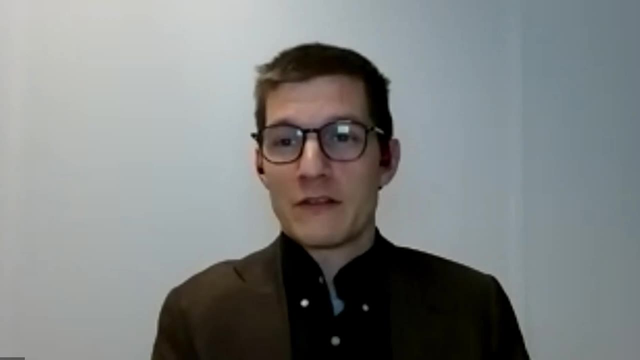 ties back to what you said earlier, martin, the fact that most developers want to develop in a secure way or at least try to fix things, because in the end they want to be proud of what they do as well. and if it is more secure, that's fine, but it doesn't change the fact that you need to develop it in that. 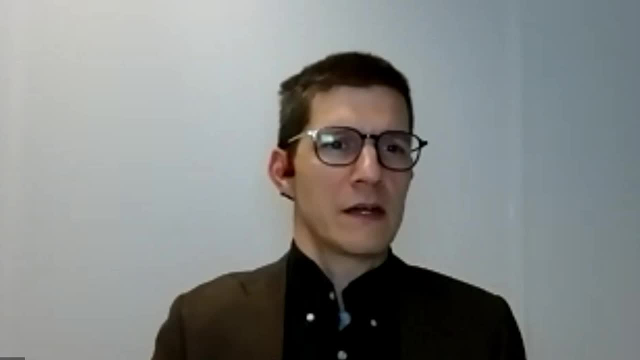 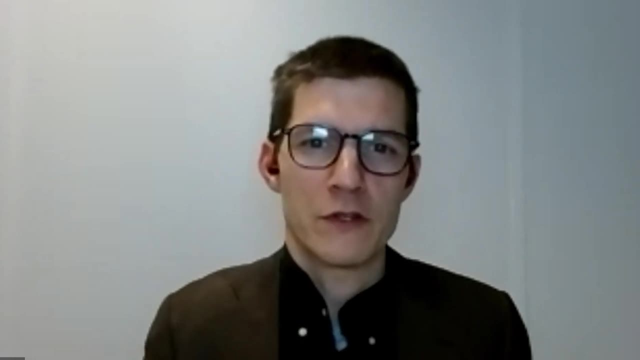 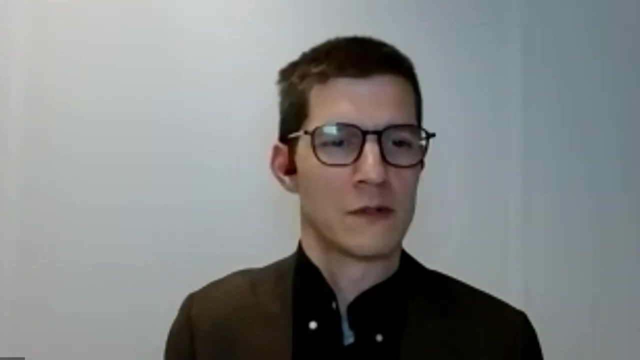 um, uh. i see one question for rob. from your knowledge, what is more efficient and, uh, efficient and efficient: to have one dedicated security expert per team, a secure champion, or make security expertise part of everyone's role? that's a good question, i would say, if you have. 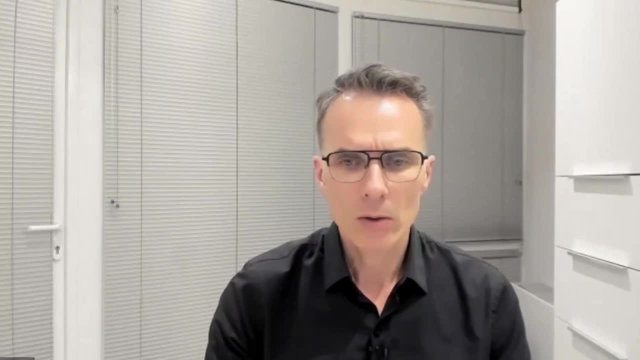 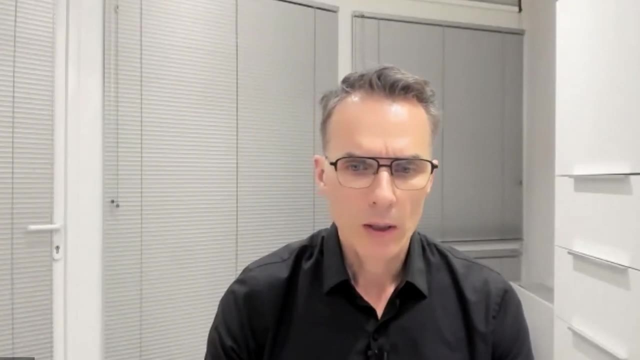 a good security expert. don't make him or her part of a development team, but let let him or her help multiple teams. if you have a security champion, ideally this is not a security expert, because you don't want to put responsibility for security into the hands of one person. you. 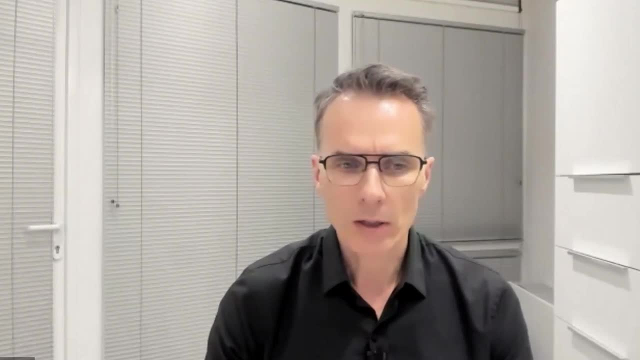 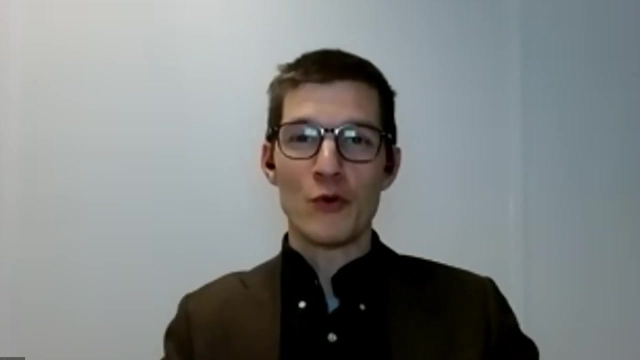 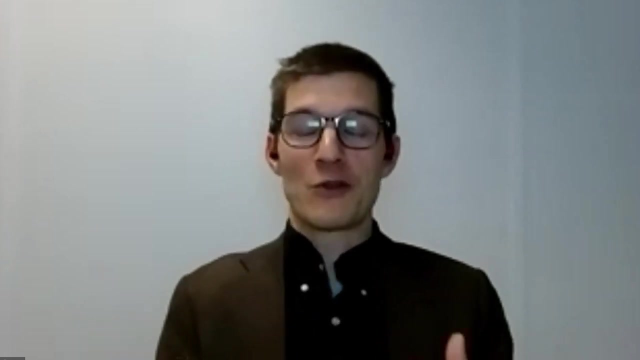 can make a security champion, a liaison or task this person with, uh, with knowledge exchange, but never, ever let that person take the sole responsibility for security. uh, i think you're. it's the same thing as you have people who do the work like programming or developing software, and you have managers, and they typically don't. they are not the same kind, and 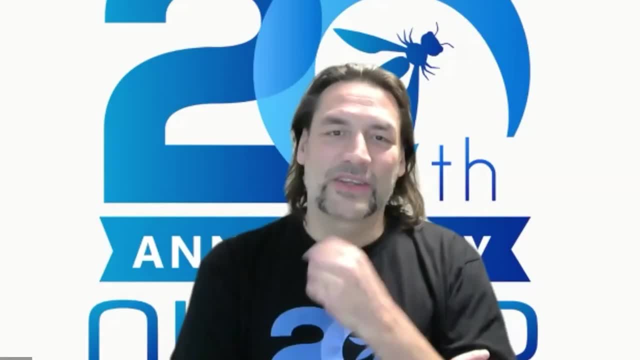 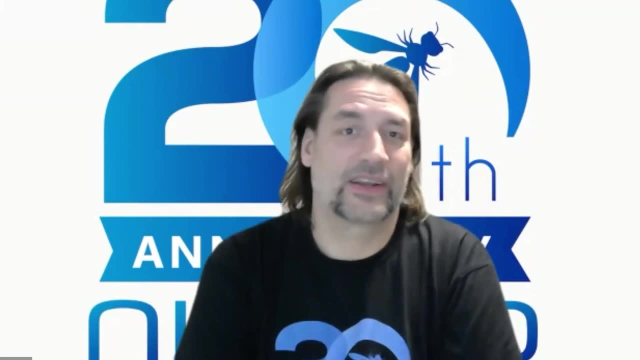 breed of people. in all honesty, i think the question is: what do you think make responsible security? they are not those who put the name on the blood science. there is no vulnerability in this release, right, but so it's everybody's responsibility, right, as you use postbones. that's what i tried in my talk to. 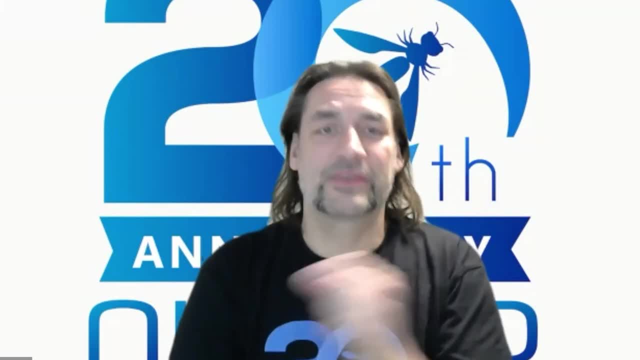 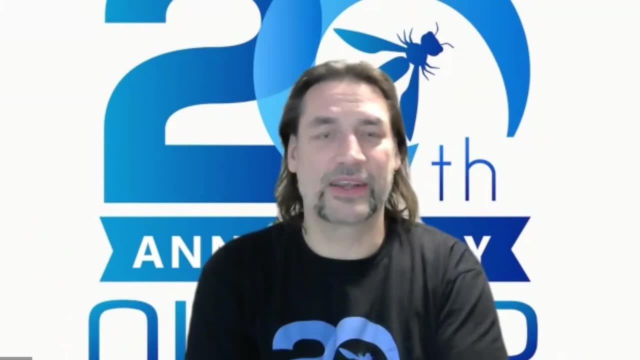 say it's shared responsibility, but you're different parts of the chain, right, it's like in our society: we all have a responsibility towards our society and actually here in europe and the netherlands we have some requirements, expectations, and as everybody does his bit, we are more secure. 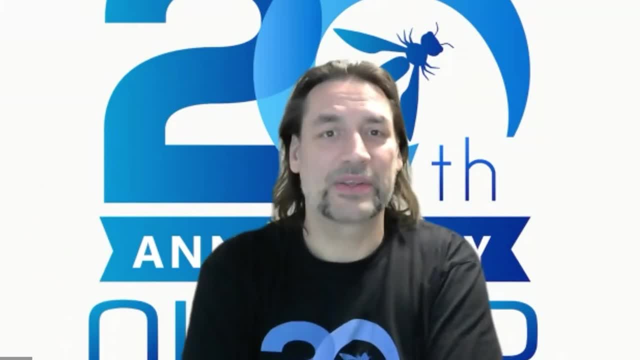 we could take it out even to the kobe discussion if you want. but yeah, there will always be people who are slacking and people do more the best. and yeah, if you're doing that, then you have to make a Yeah, as long as more people do the best. 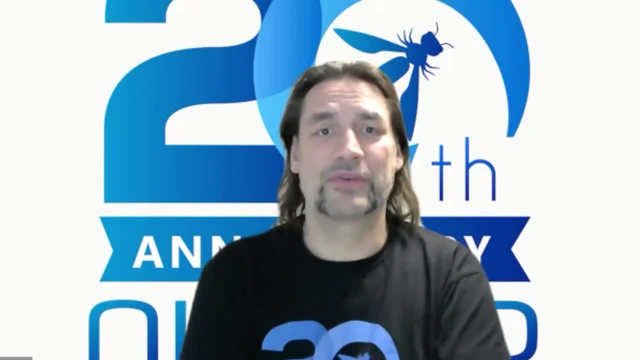 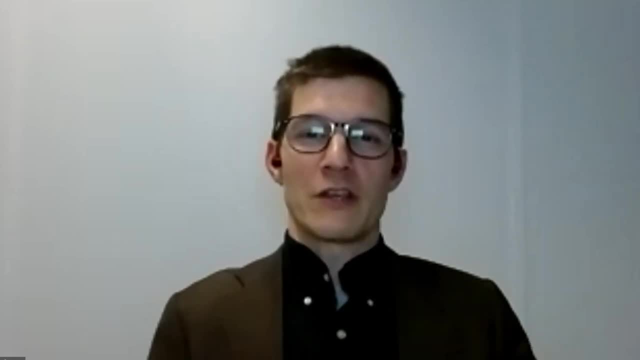 you will have better results, And to make them do the best better, you have to understand why it's better and how to do it. Yeah, so you can actually read that question in two ways. Is everyone a security expert? Now, everyone should have security as a mindset. 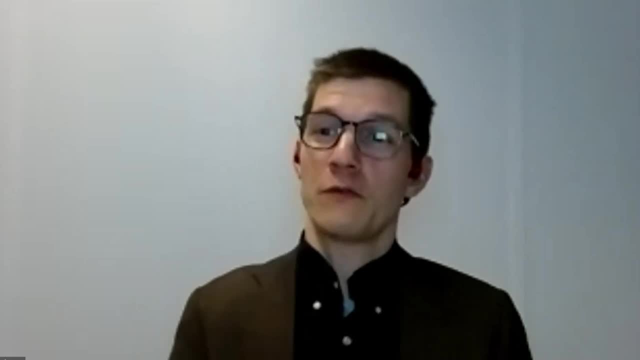 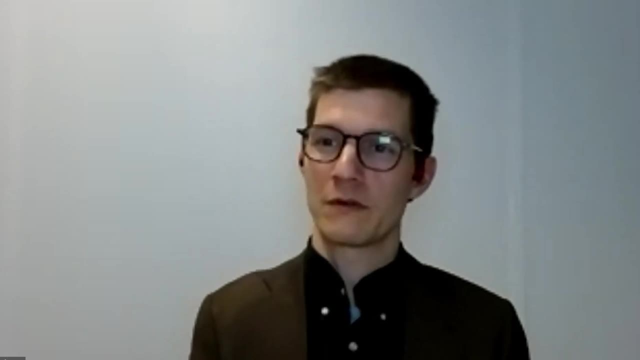 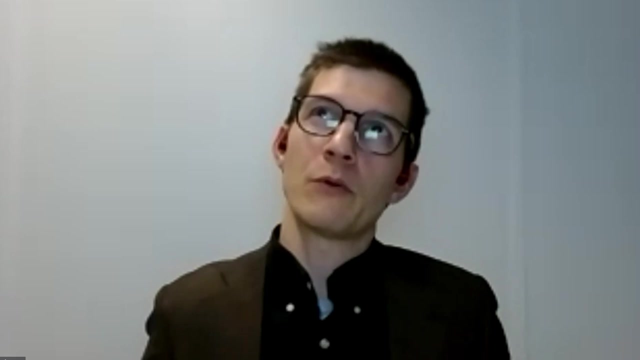 or secure development as a mindset. Is there one person who signs off? Yes, probably. or a group that is not developing itself? probably. is what I get from Rob correct: Signing off, what do you mean? Well, the people who are developing. 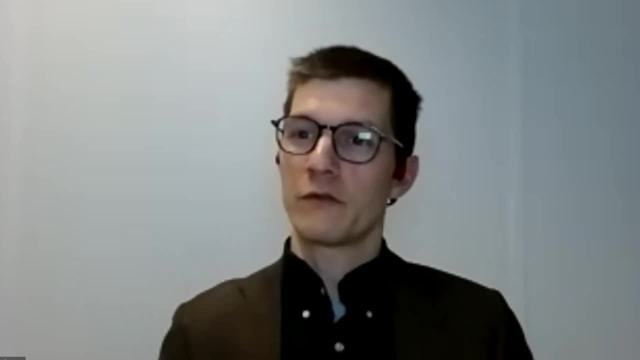 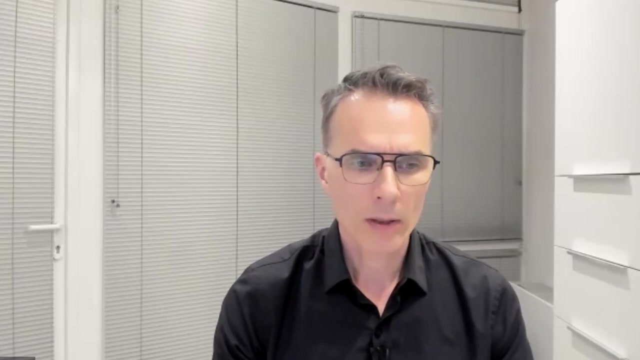 are not the same people who are reviewing codes and signing off that everything is secure and is the ultimate security sign-off platform body. Okay, so to me that has a sense of a quality gate situation where there's a security team. that is a quality gate. 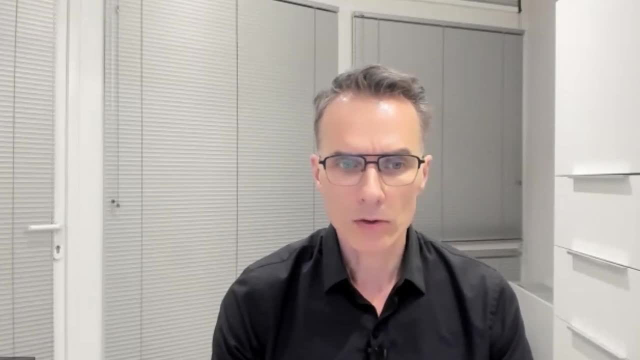 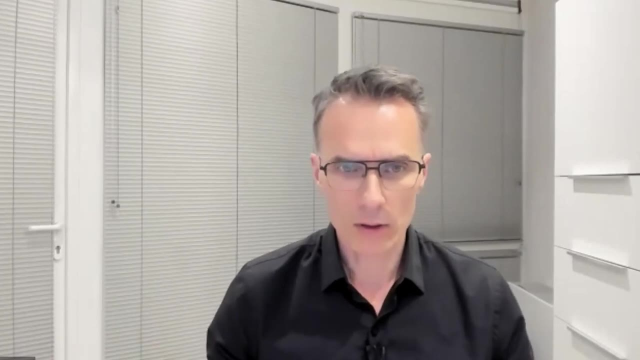 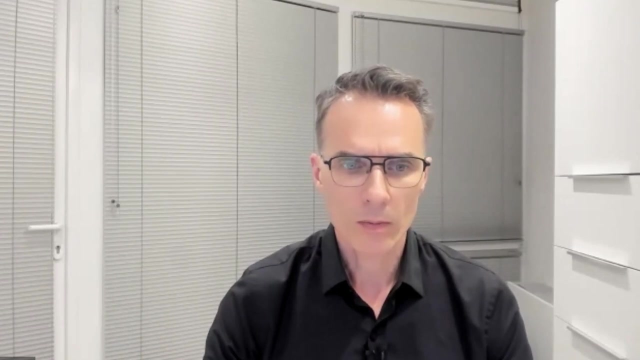 and needs to sign off. Of course, this is still part of many maturity stages, but in the end, you want to sign off to be by the collaborative, which is development team, supported by the security professionals. Okay, Yes, okay. 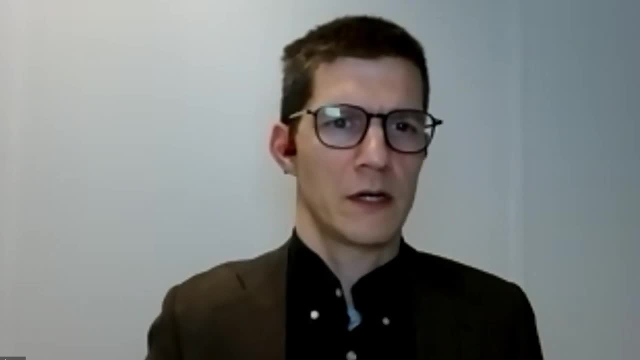 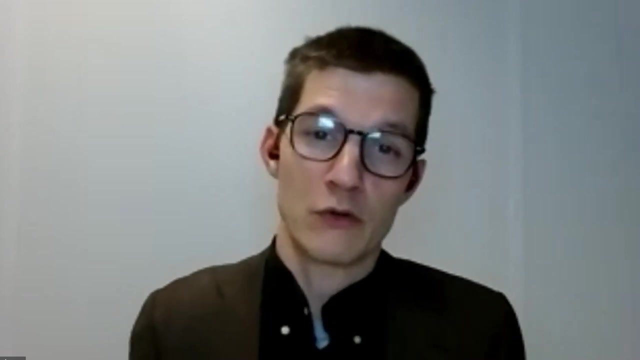 Let me see if I see some other questions. How to magically transform? I see one question: threats from supply chain and third-party software Are increasing. reviewing every external code and tool from suppliers is also not realistic. Any advice for achieving reasonable trade-offs. 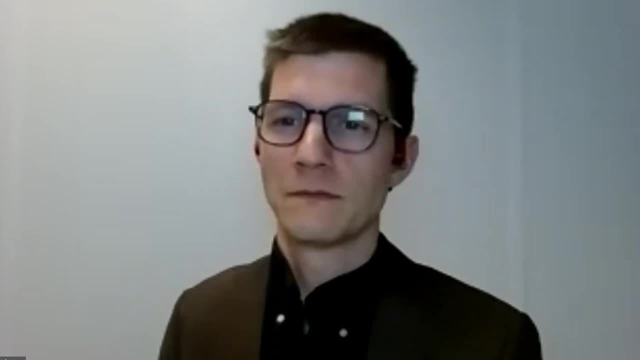 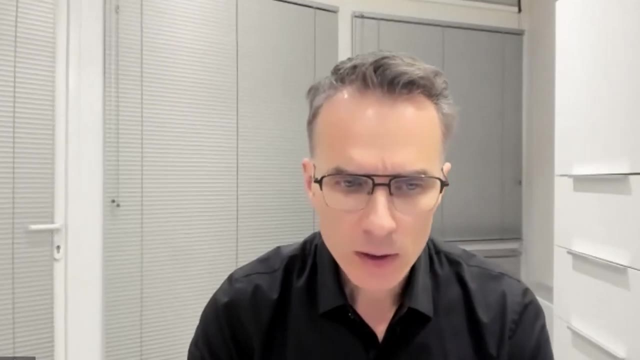 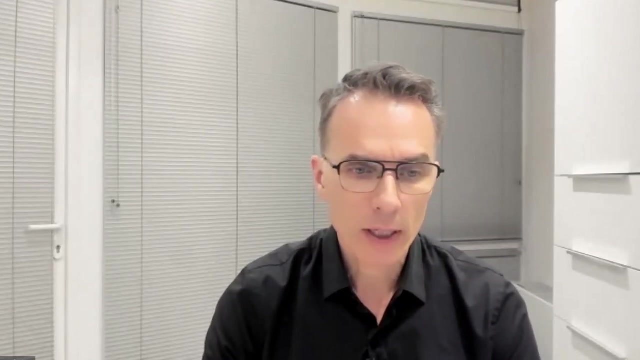 This was in Rob's session but I can start the answer and Martin can pick up. The question mentions the need to review external code. I would advise against that, although I would applaud more initiatives to do that as a community effort. but the key is: as a regular software development organization. you better rely on the documentation of known vulnerabilities in these external dependencies, and there are public databases for this, such as VonDB. Use a package manager and dependency checker. Have a quick response process for new vulnerabilities that arise. 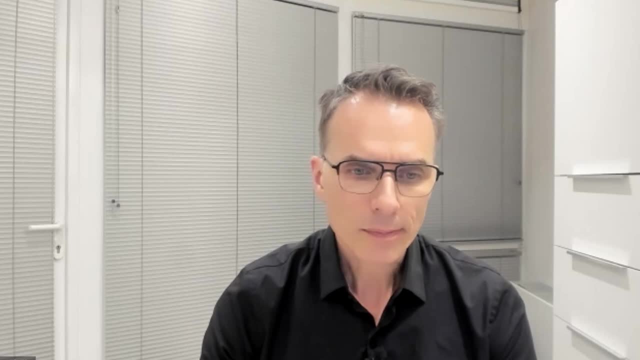 such as log4j, log4shell. Do some due diligence on reputation when you add a dependency and try to let the number of dependencies not grow too big. Those would be my takeaways. Yeah, I think we see it what I call always. 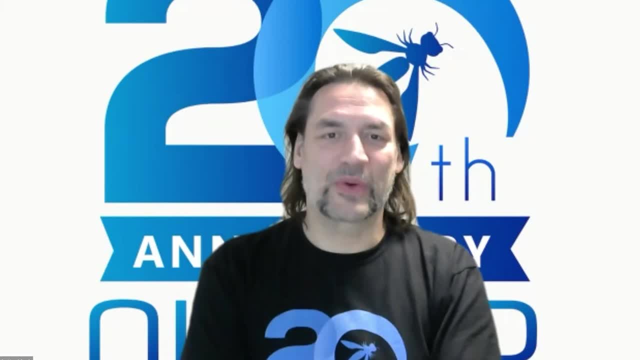 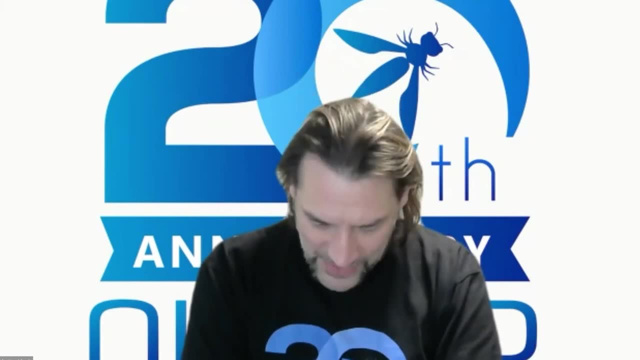 that the DevOps Wild West, it says, say, oh, developer responsibility, so we can choose what we want. and there's a very nice anecdote from- I'll just call him a name- the guy from Amazon, Bezos, Bezos, Yeah. 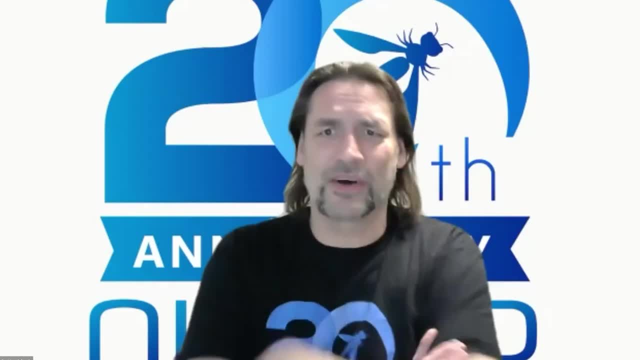 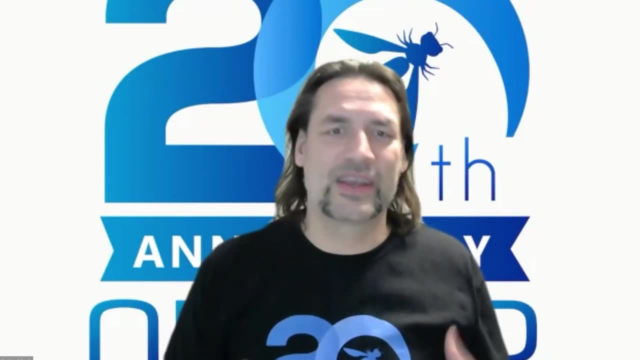 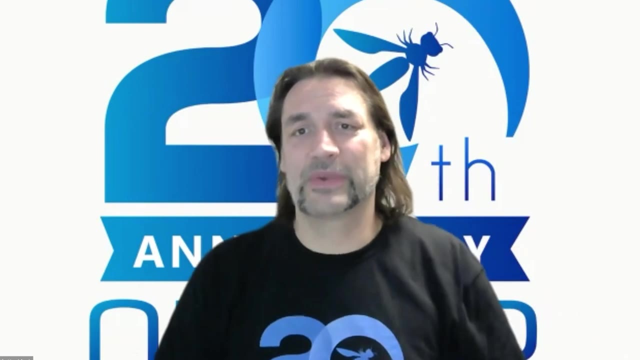 Jeff Bezos, Yeah, Jeff Bezos, Jeff Bezos, and say, yes, you can choose betweennet or java, two choices, not hundred choices. right, you have to stick somewhere so you cannot do everything every library. no, there is a, a subset, uh, a requirement, and it's what i try to say is a responsibility, so you have to development. 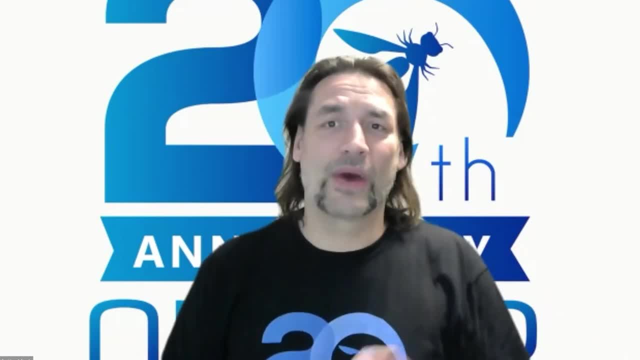 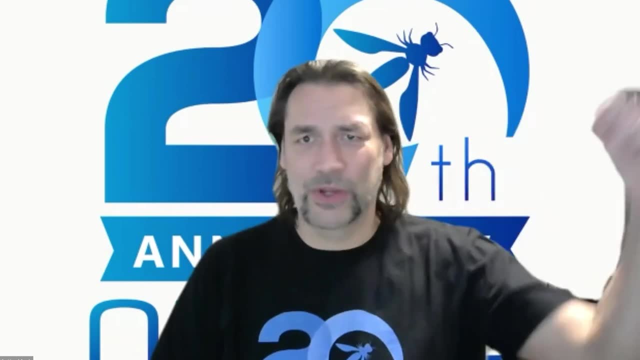 have to understand you have a responsibility, that you now write enterprise software and therefore you have a more mature approach, that you're not 25 years old. yes, we need the people say we conquer the world, we jump off the cliff. then we need all the people saying maybe not all at. 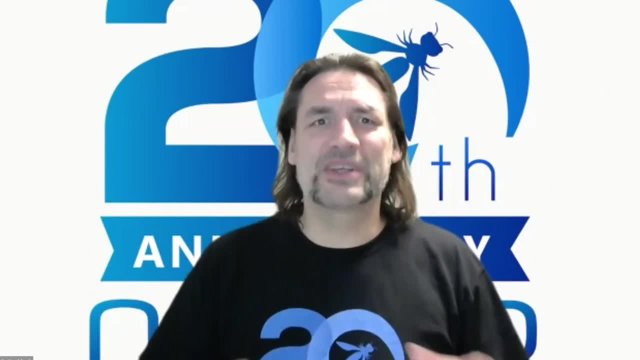 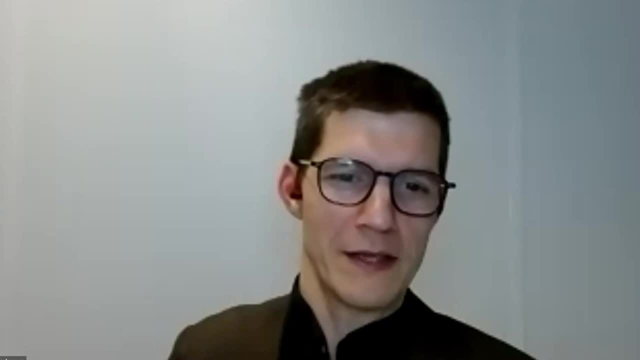 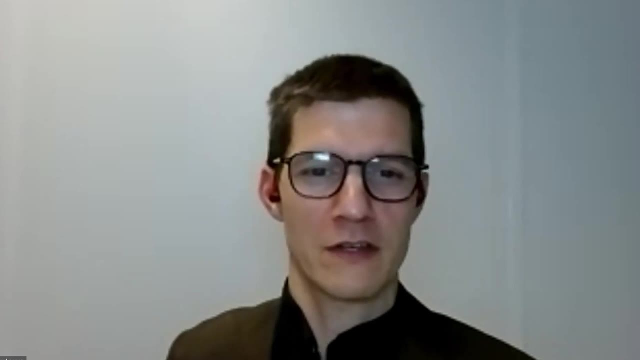 once you go first right, try to be sensible and mature in your choice of software development. that was also a question, although i think you answered it already, martin: what are good sast and dest tools in the market? i'm kind of based. i work for micro focus fortified. 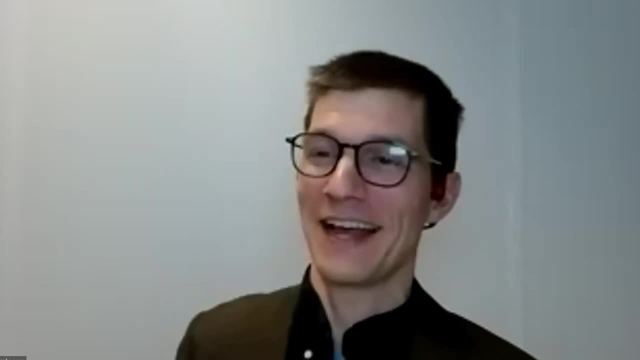 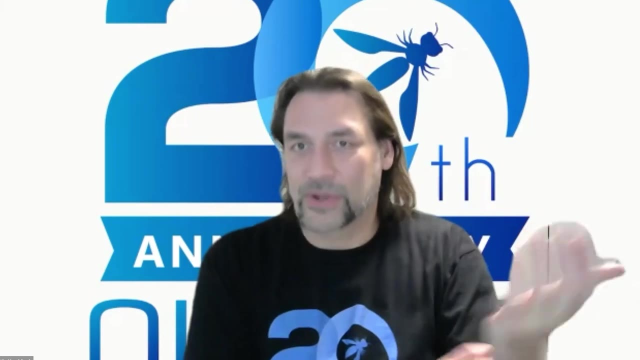 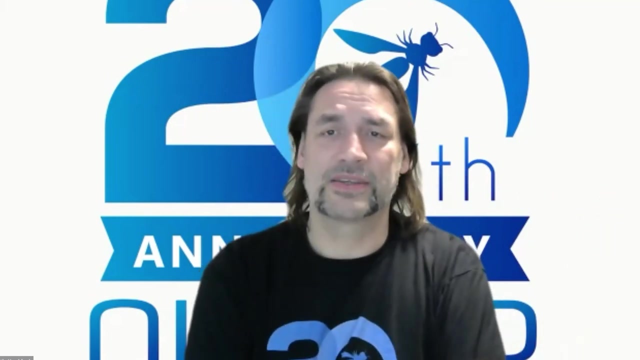 but uh, yeah, you have to mention at least two others. no, yeah, so that's what we're going to do. so when you look in january, there's fair code. they have own check marks. there is open source tools from owasp for uh dynamic scanning. we have semgrep for uh other things. we have now a sneak. 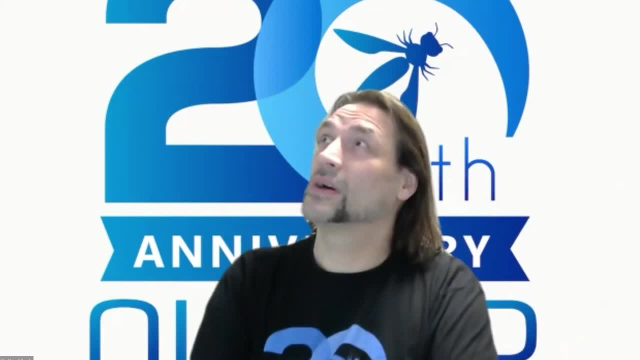 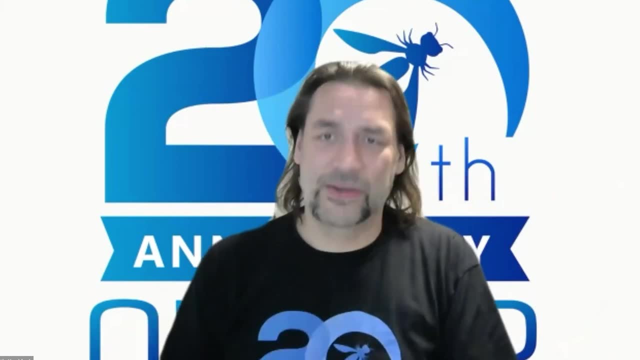 uh, github has their own tools. uh, with snow, um, solar type is getting better, so you have all kind of stuff. yeah, the thing is you have to choose the right one. i don't care which one you use. yeah, you know i have my salary has to be paid, but of course, yeah, 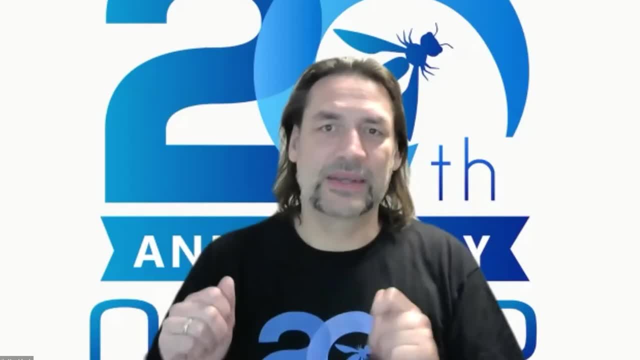 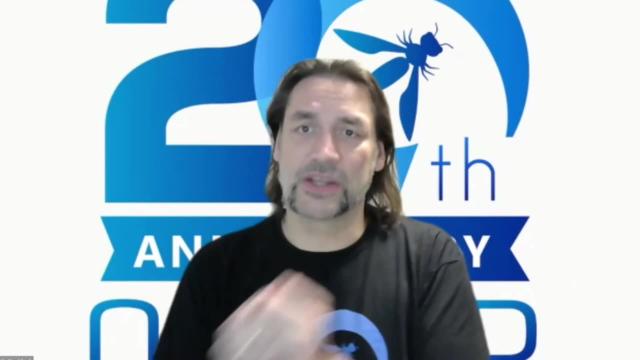 as long as you use something, if you do it by hand, the thing is not which tool you use. you have a tool, you have a technology stack right, you have a development process. find the right tool in your context and the thing is: you should actually a bigger company, should not? 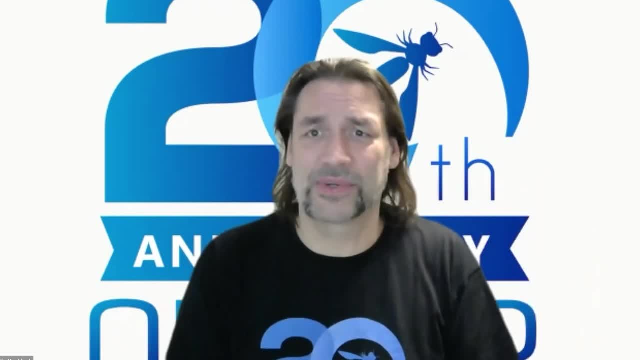 have one tool, they have two or three. it's like, uh, you said something about carpenter, they don't have one hammer, they have four different hammers. the problem is, a hammer is much cheaper than a software. security, uh. uh to analysis tool. that's the thing, yeah, but uh, the one is better in java. 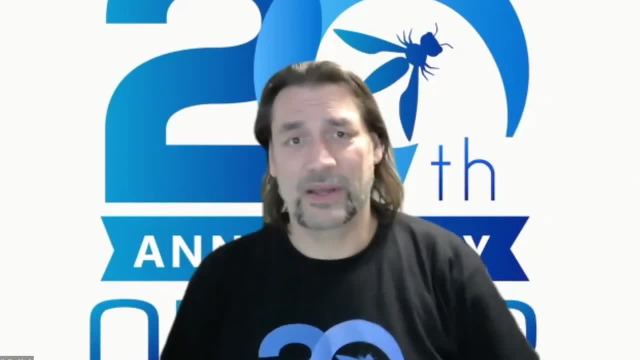 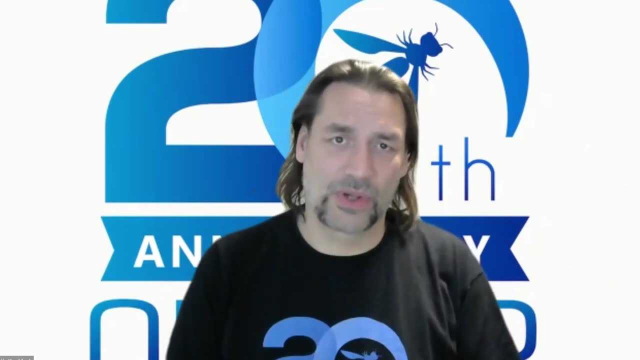 the net. the other one is better in the scene. oh yeah, i missed the synopsis also tool. so yes, there's so many that what is your context? what is the languages you support, what is your development? do you have an onboard? you have external, internal development. there's so many things, and do you? 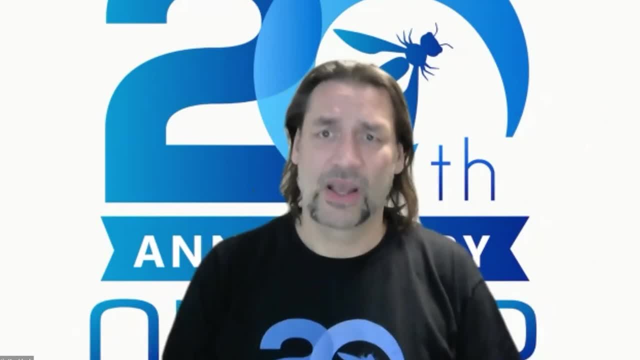 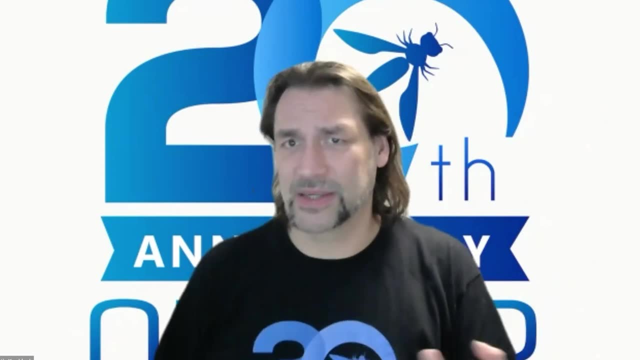 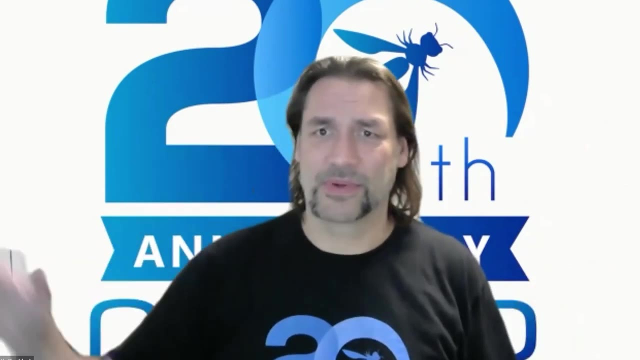 proof concept and as long as you use something it's most and you start not with the security tool, start with a software quality tool. cyclical complexity, coding standards: have the base of quality right. don't try to run first or high jump, try to send up a walk first. software quality is. 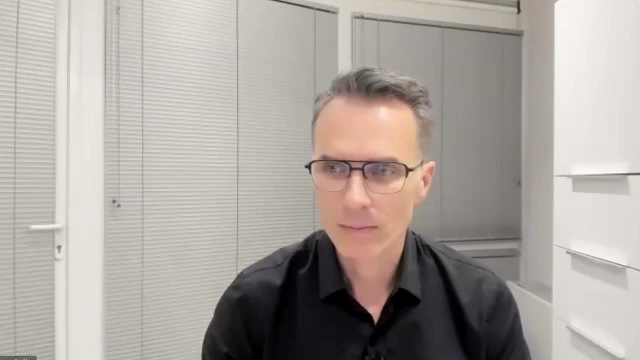 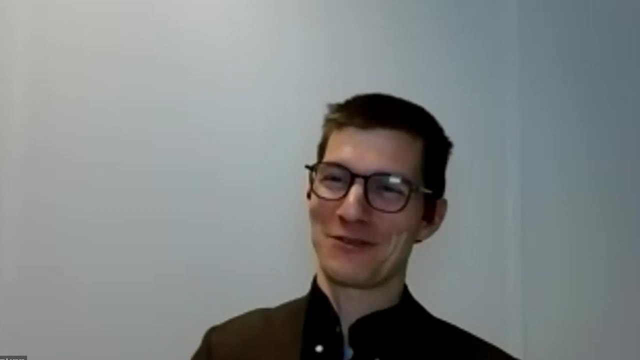 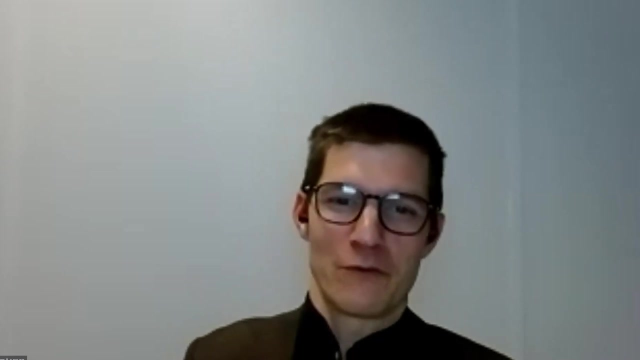 the first step. amen, yeah, wow, definitely almost a nice quote for the end of the evening, but we still have a couple of questions to go through. sorry, um one for for martin, security can be seen as a non-functional requirement, but you could also make user stories about security. i read different opinions about it. what's your take on this? 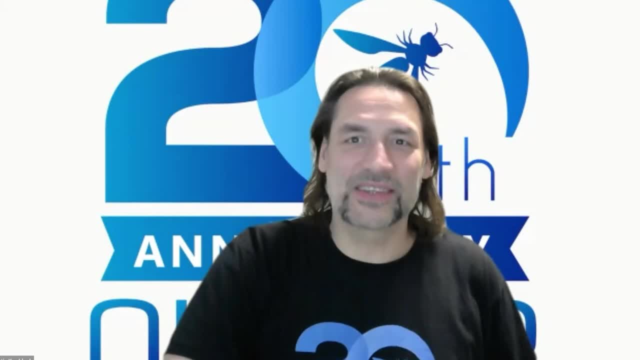 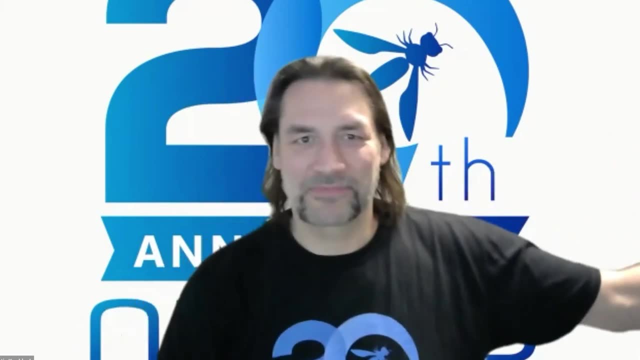 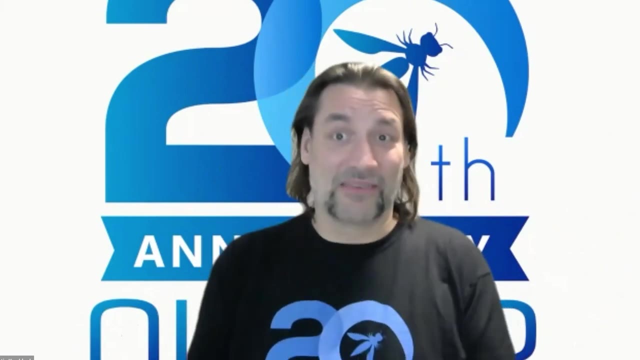 this is a discussion i never understand fully, ever since i'm in security. a lot of people try to push off to non-functionals because no functions are great, it's for the architect, right. but login- if i have a login query and have a spell injection in my login, then it's a function required, why i have 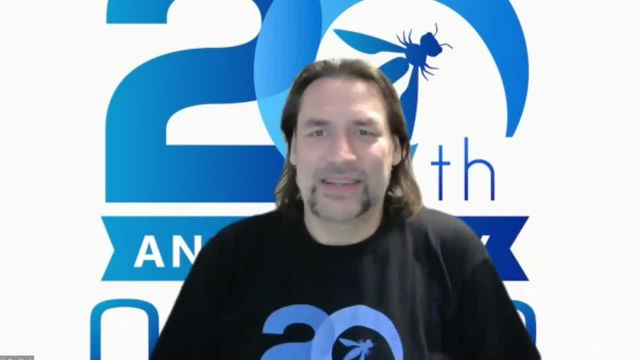 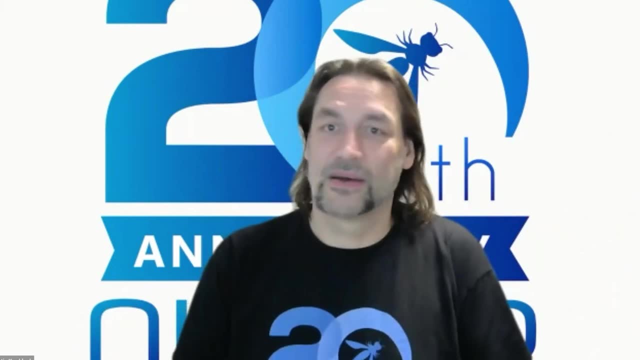 the three logins, i cannot log in anymore. it's an insecurity? no, it's not a function non-functional as a security, it's a functionality we develop. we develop a technology and you see, is this uh, actually it's more say it's a bug or floor, it's a technical form or is a functional insecurity? 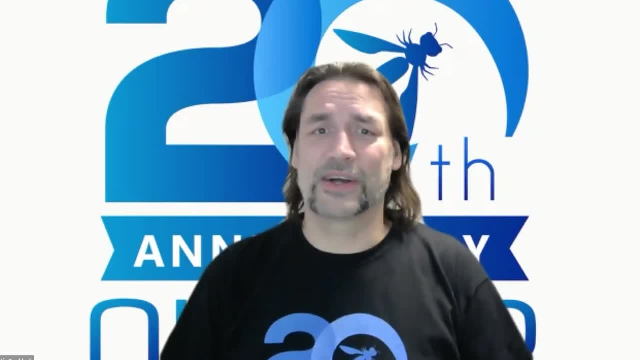 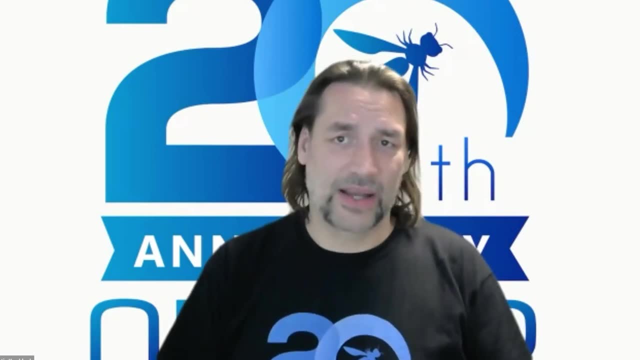 and what's our risk? right, so i don't care if it's a function non-functional. if there is something risk or vulnerability or a flaw or bug, what is the impact? what is the likelihood you have to fix it now. can i avoid it easy? who hasn't thought about it? and they have just said modeling what i hope. 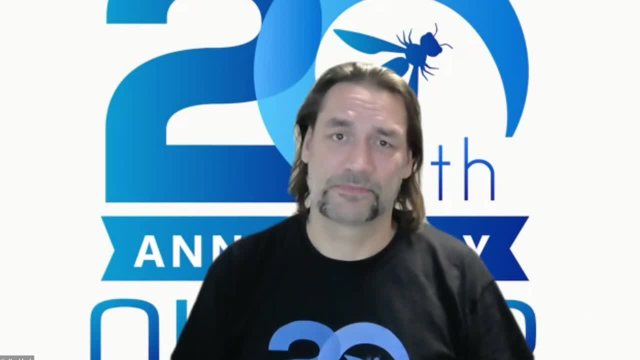 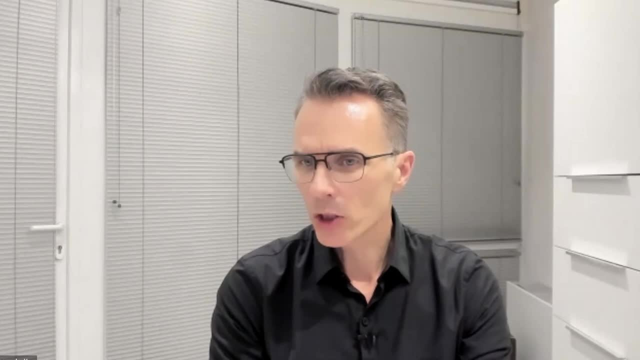 for you about it up front at the north front. thank you, maybe i can after that. sometimes you see abuse cases on backlogs. they are useful as a sort of a reminder what can go wrong, but in my opinion they should not be treated as things that you can plan and that you can have in your 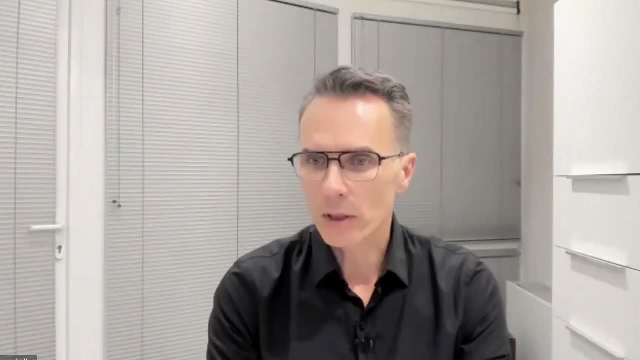 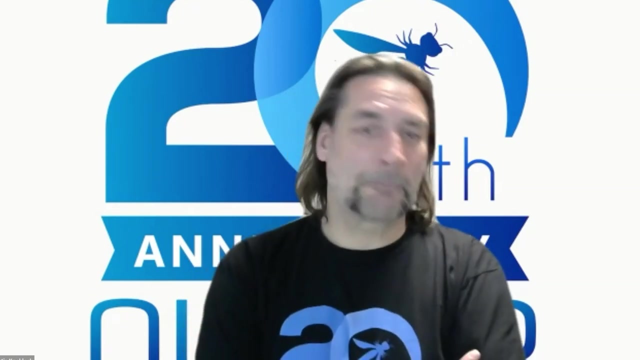 in your, your, your, your sprint, because they don't represent a specific change. they can be helpful for threat modeling, but not to plan in your, in your, in your sprint. okay, what's that modeling hope? did you talk about conicopia? i didn't talk about it, but so, when you're the same morning, there's also a good thing to. 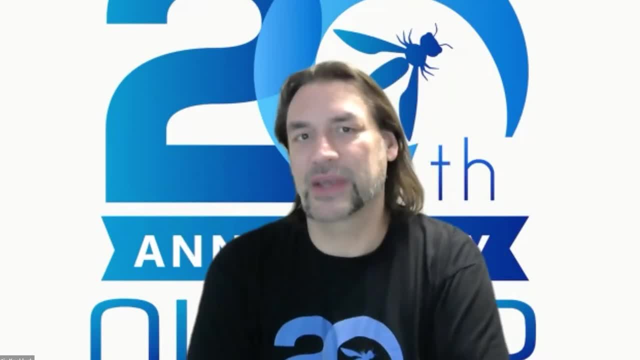 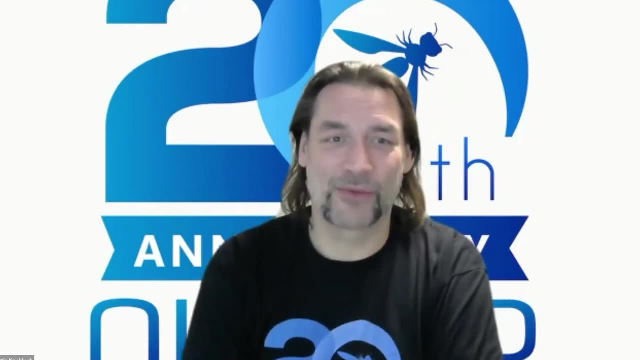 ask you why it was exercise threat modeling. but there's also a good way to gamification, where, for example, the over conicopia and it's very strange. but but look in the application security wayfinder, what mentioned uh, where you have a like off keyboard and all uh do the security threat modeling as a card game. 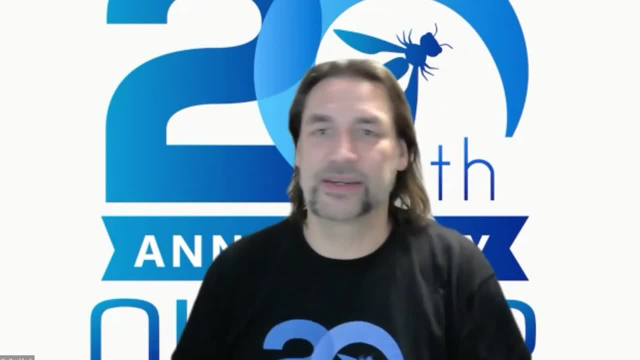 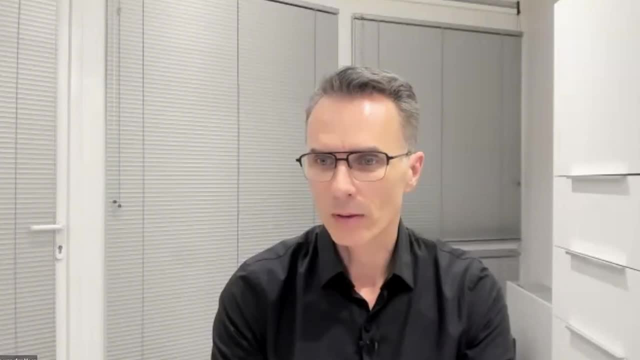 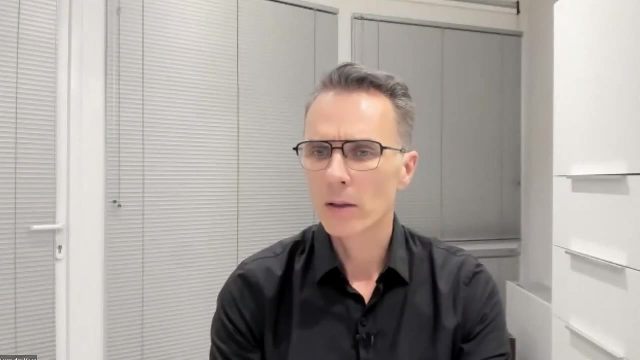 so you're not diverted by your keyboard or with other ideas, and i did it several times with customers and friends and for previous hours, and it's always helpful, it's cool, yeah, and it's it's a nice gift as well. i don't know if they're still available through osr day martin, but 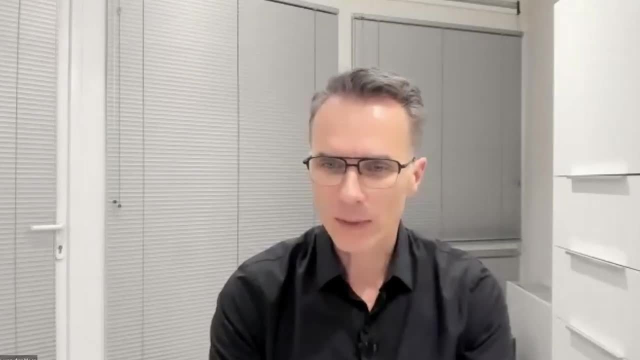 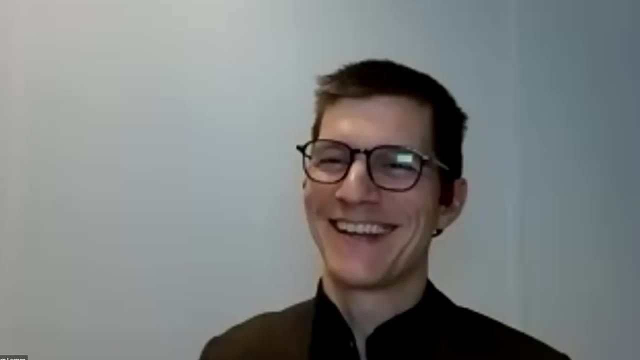 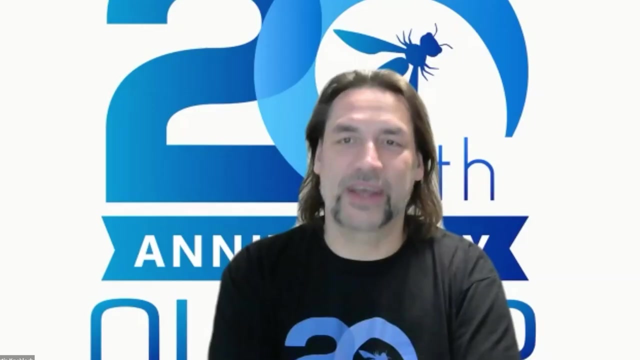 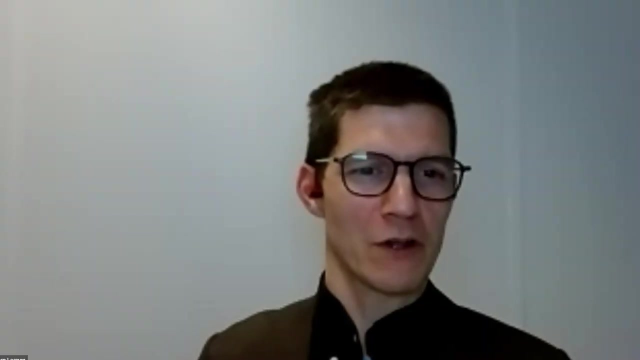 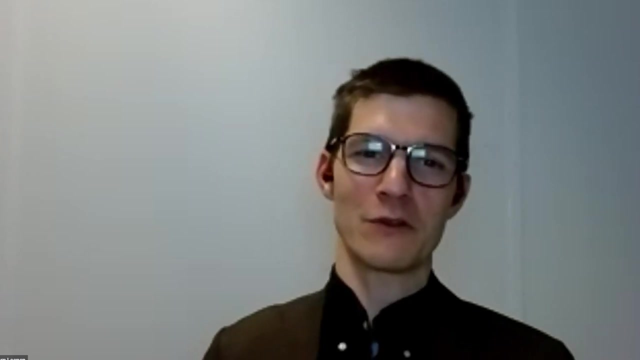 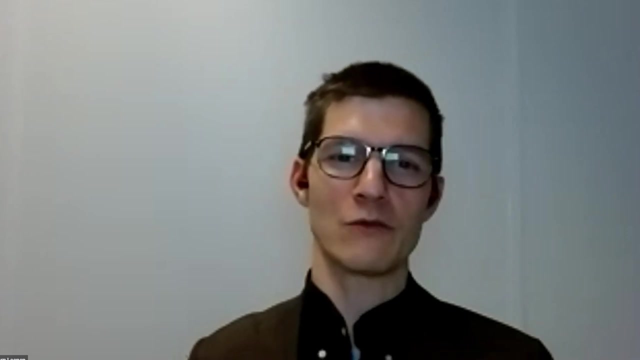 the ideas. talk about it card game. yeah, and it contains uh typical threats or patterns that help you think about how your system can be compromised. it's based on the asvs. Johannes asked: how can we create a bridge between the it development world and this ideas about building security in uh and the ot, uh eos development world? in the ot world, we need to. 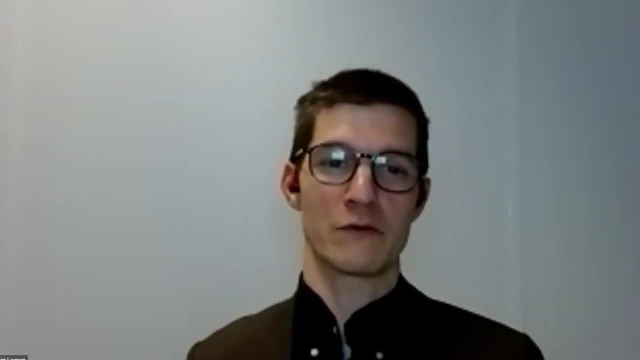 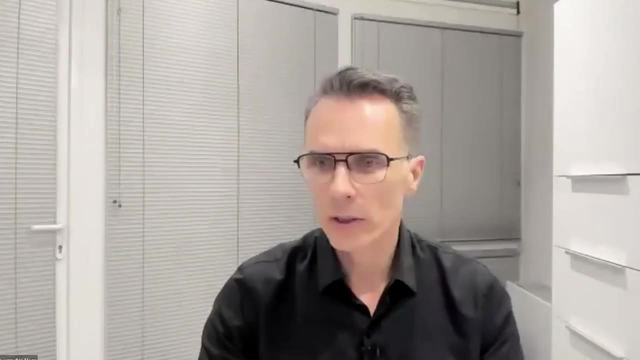 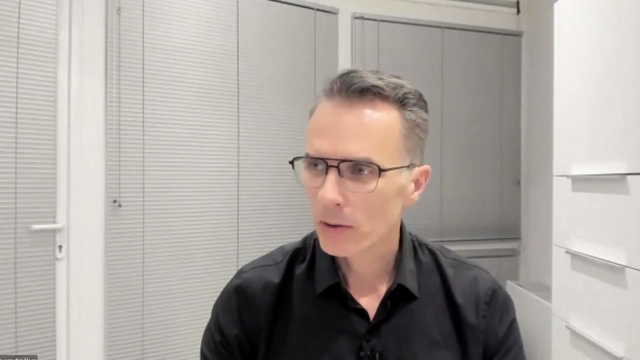 shift left as well, not only because of security but also because of safety. one question interesting: yes, i once was as at an industrial control system conference and i felt a bit out of place because i had a very large room and i asked: does anybody know of the oasp, asvs? and nobody, nobody did. 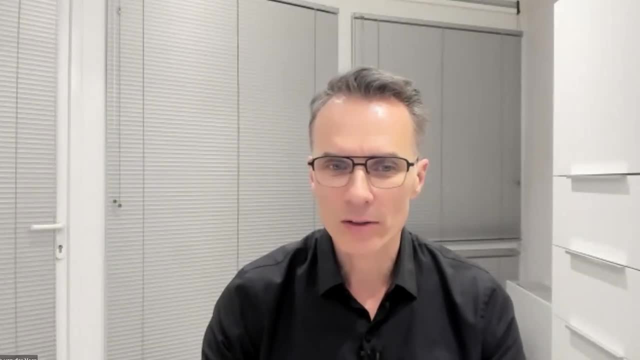 it's still a mystery to me. and still, the the 6243 standard is is is quite amazing. so there is a drive there. but uh, maybe martin, you have some insights. yeah, i think it's the same as we had in scott on the past. right, they come from the industry and i myself come from the. 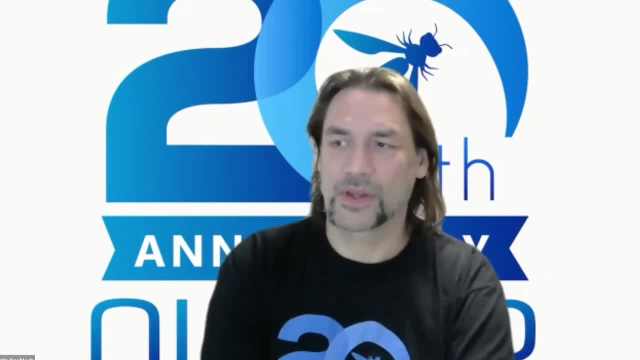 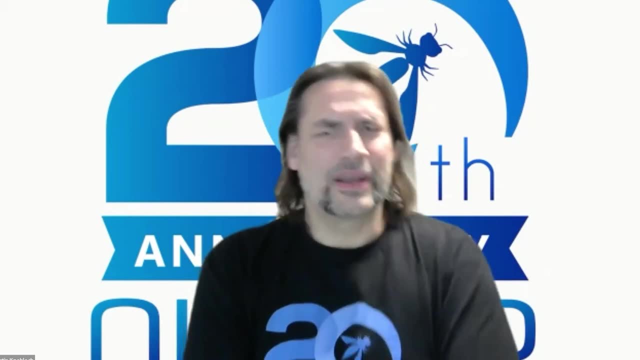 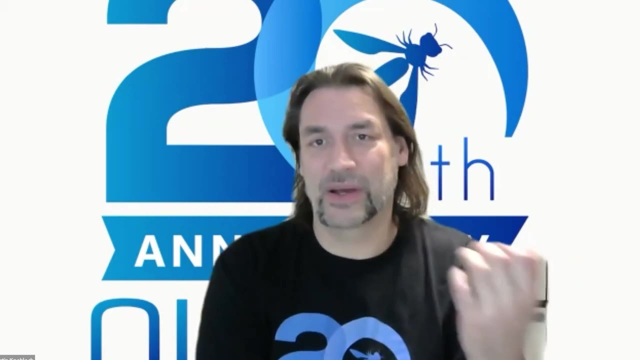 industry and i did the talk for uh, always for uh, somebody who does plc programming. i don't want to fail me. uh, who was it? and uh, i looked and said hey, i didn't say programming when i was a developer mechanic, and it's totally different these days, so they come from a different area, they're just. 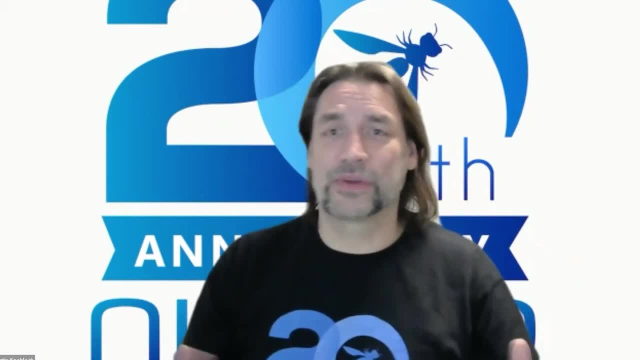 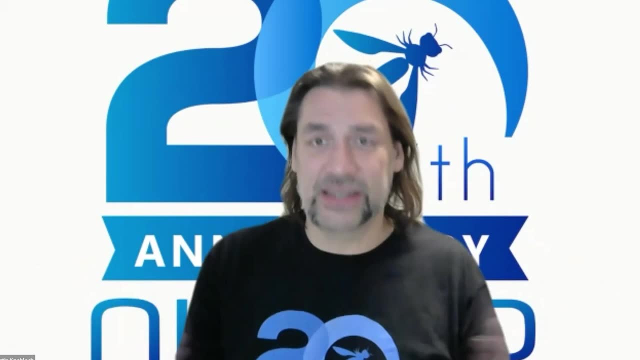 looking over the edge from this, our current age, on software development and all that could go wrong. but they are now opening up to this bad outside world because it's their previously closed systems. but it's very scary for them. but they say, definitely when you look in the automotive or the 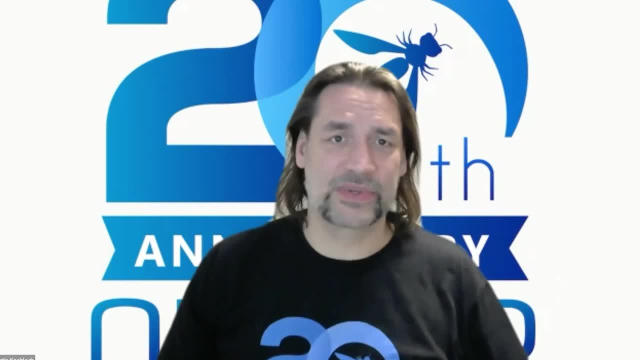 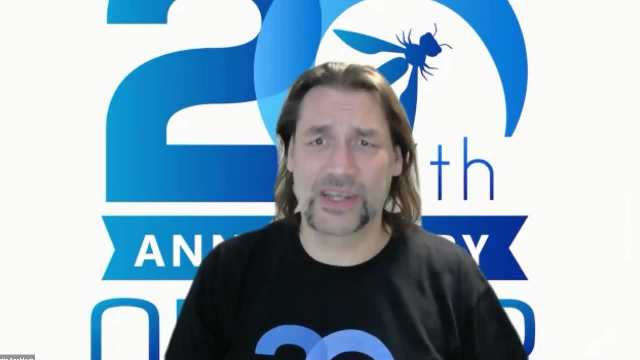 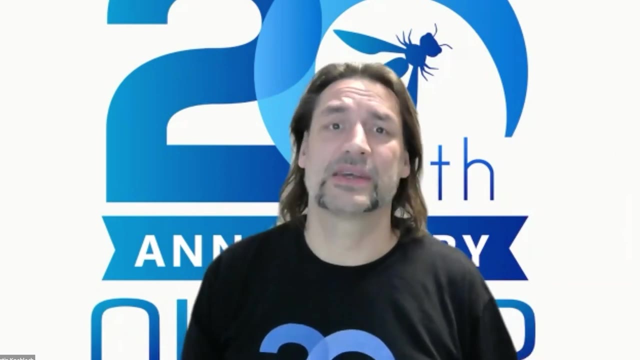 t. they have so limited other specs. you know, these days with uh, all the cloud abilities, more rams, more space, no problem. try that in the ot environment, on the iot environment, and there's actually good european regulations for iot. these days it's the certified, not a product, but also the process to. 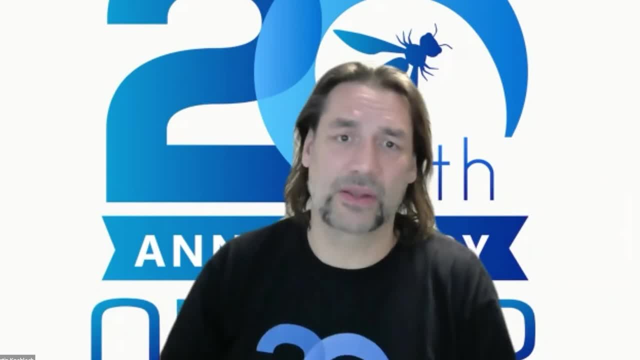 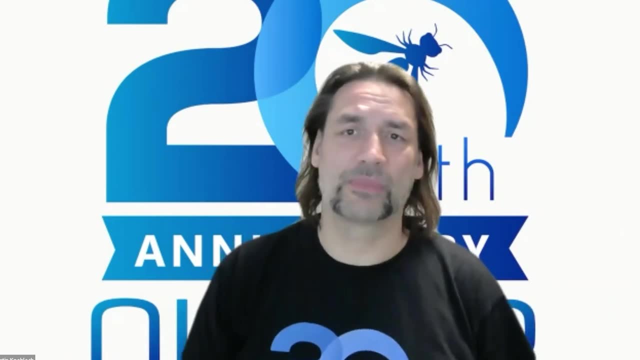 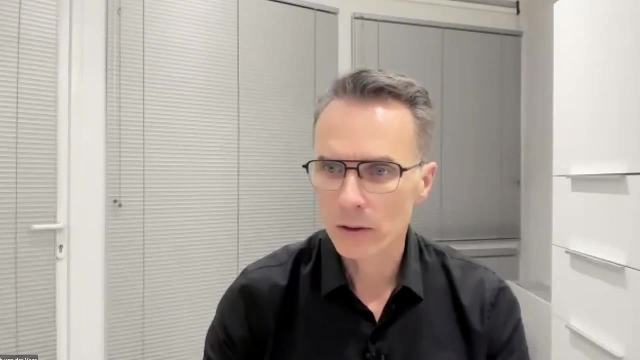 create a product right, you have to prove that you are able to update and improve and fix, for example, but it's very different from the origins where they come from, from software or web development. maybe a direction to answer johanna's question additionally is to have more knowledge exchange. 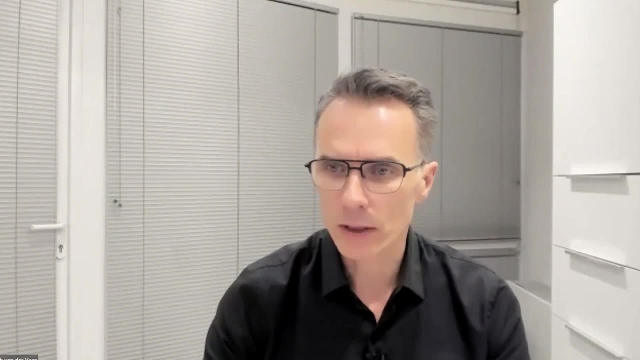 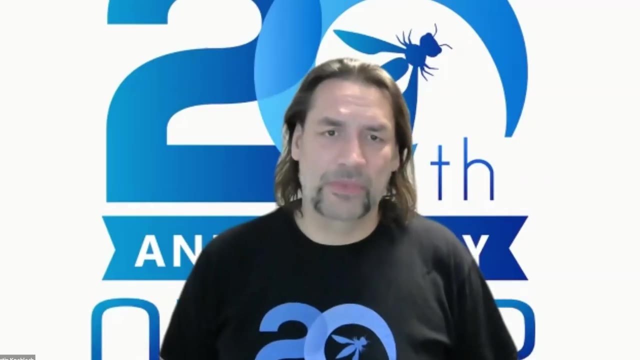 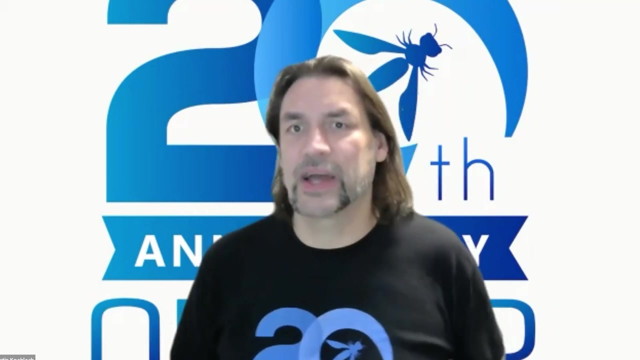 and more mingling between the people involved in that area and the people in in in it to share. i've been there for uh- i'm the cavalry also outsource community uh with the european community. uh talked about certification of iot development and things like that and um it's. it's a bit like i didn't come here because i was. i was. 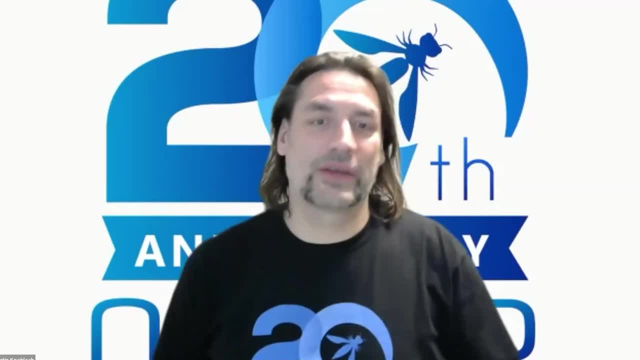 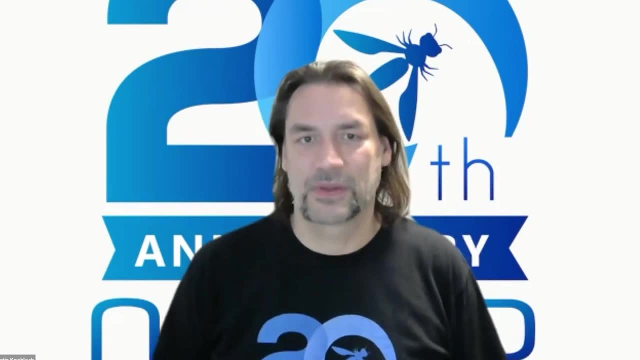 a bit, like you know, i'm a ně. i don't know what you don't know what you want. i mean it's i think we have um a lot of problems with the modern system, but, um, as it's sort of hard to get the right kind of solutions, and, yeah, i can tell you that we're not just trying to develop it. 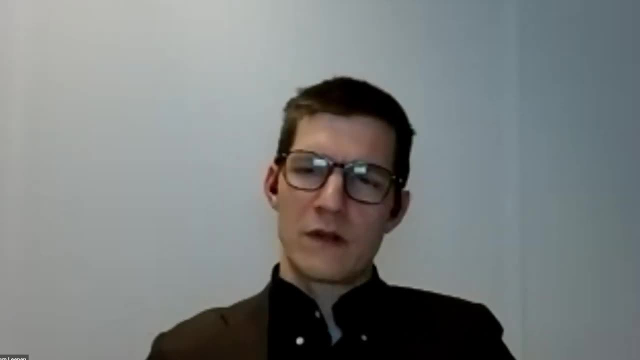 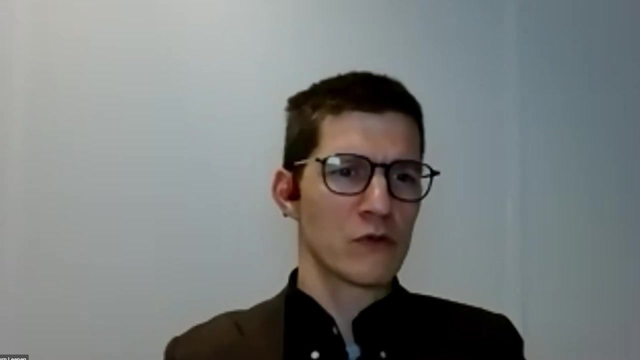 but and and it's, it's, it's the very basic principle. we have to get the right thing and in many cases, so that's why i uh in a way, like i think this- the expert i i would recommend to uh- is that you follow that really well, because i think that it's a really easy uh method, you know. 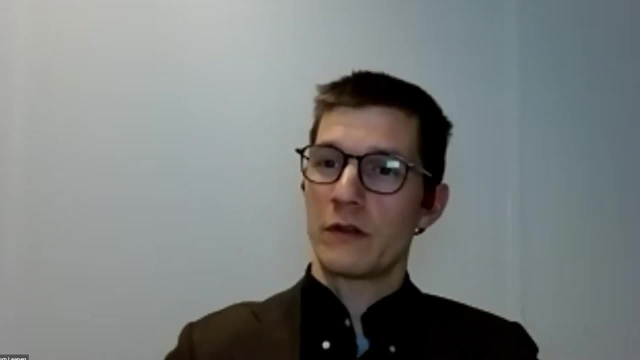 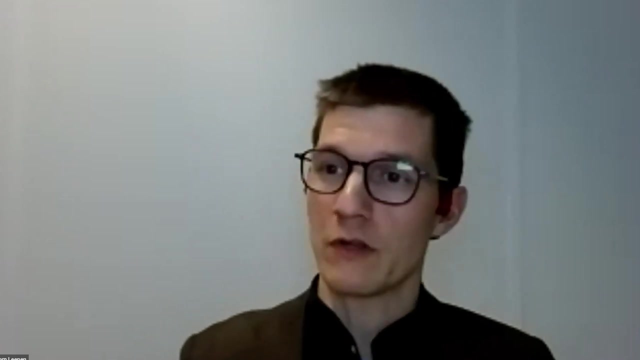 to go there with the device or not, here requirements. so it's they go there and they look at you like a moment ago because with the quality, well, take quality in uh now built from a quality platform and then built in security, i think, or i would add, that having a good process um comply or explain. 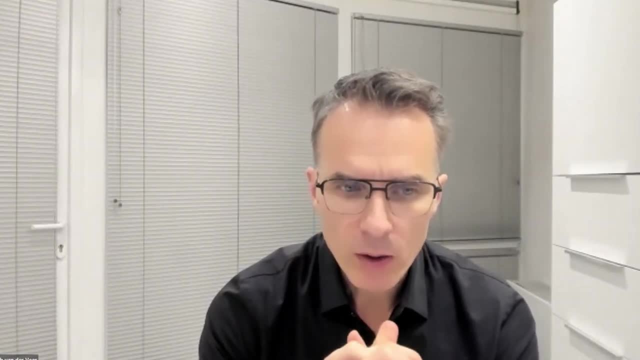 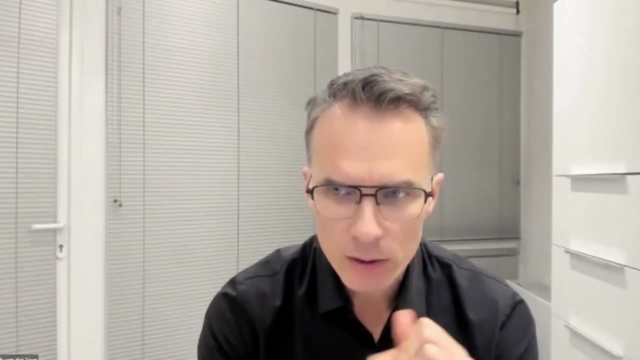 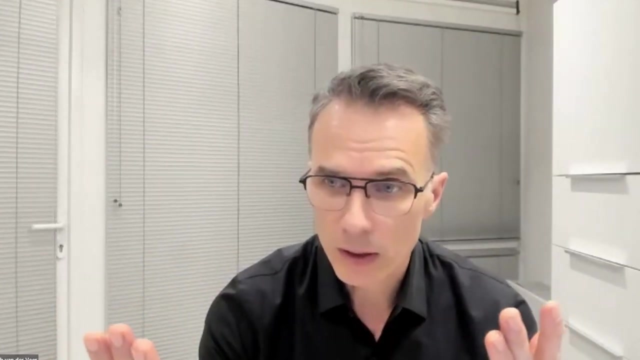 will allow you to make trade-offs consciously and openly, document them. so i'm not just saying thou shall apply two-factor authentication, but say you need to apply it, but if you don't come, come with your uh exception and explain to us why, and then perhaps you can deviate, being open to 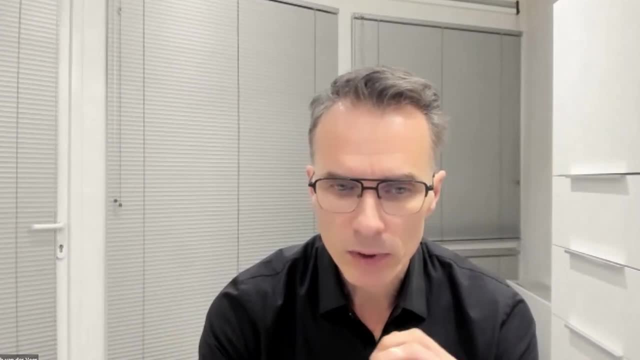 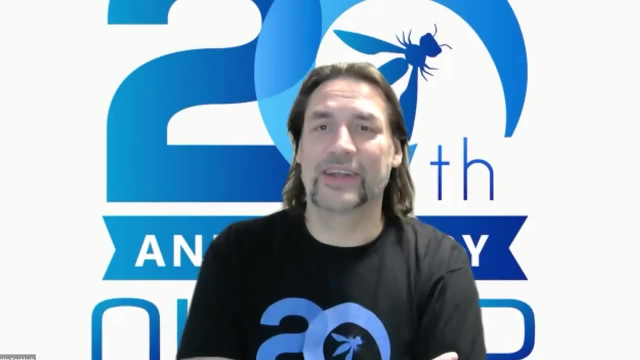 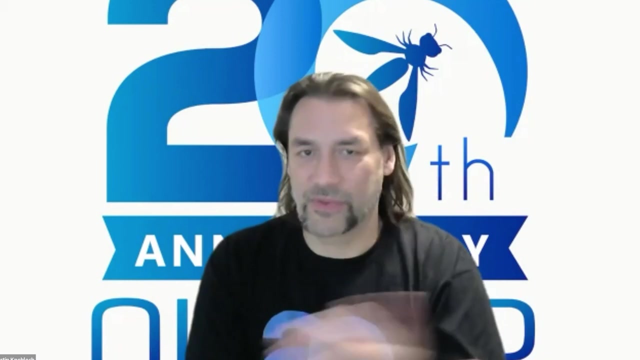 such discussions is an important part of culture and and processes. that helps here, yeah, and of course, as we uh what called hygiene. if you have to basic right, if you write quality software, do you have enemy a lot. but that's also what i said, the the box and the flaws. and then we quoted gary mcgraw. 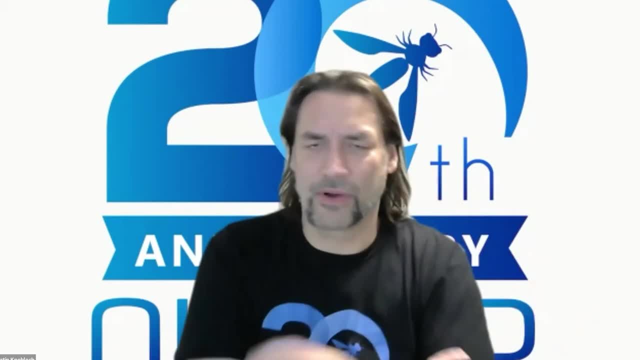 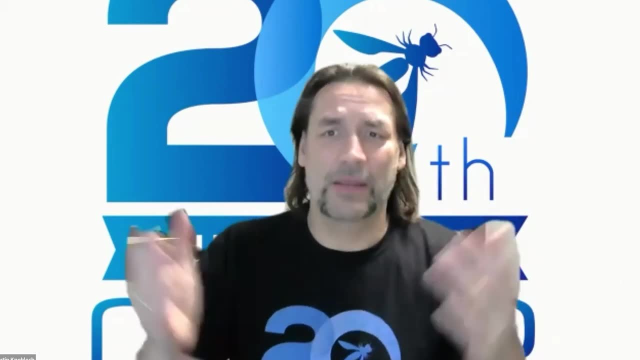 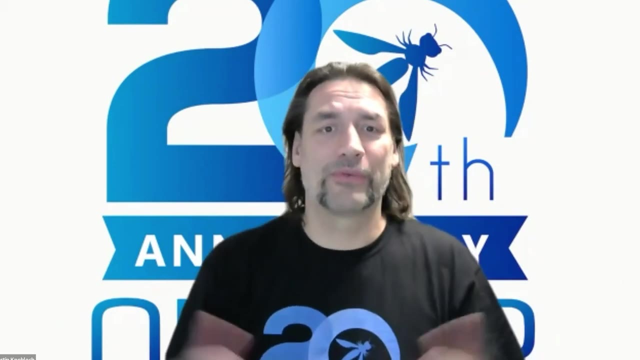 before and he said: what is the bug is a technical form and a flaw is a functional flaw. so when you do, for example, you forget some security. uh, an example is: i know that, uh, in the past, when we had mobile phones not being able to do anything, then call a mobile phone number in the bank. when you 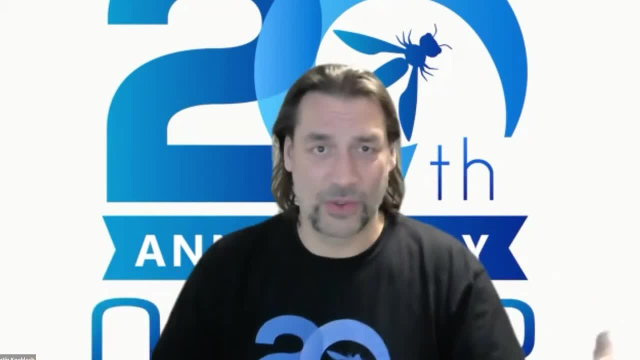 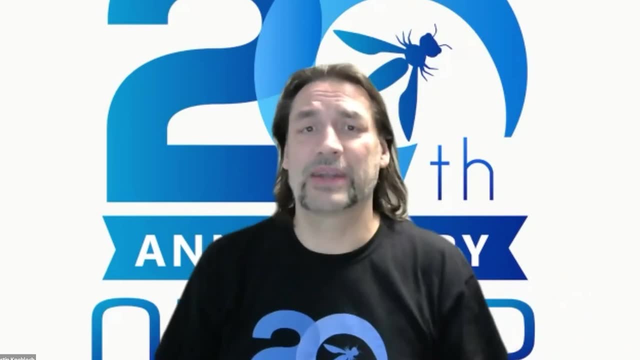 gave it to them, they were happy because then they could call you and sell you banking products. but these days, with mobile apps, the mobile phone number actually is this verification token right and i know a bang. they had no problems with the app itself, but the process of changing. 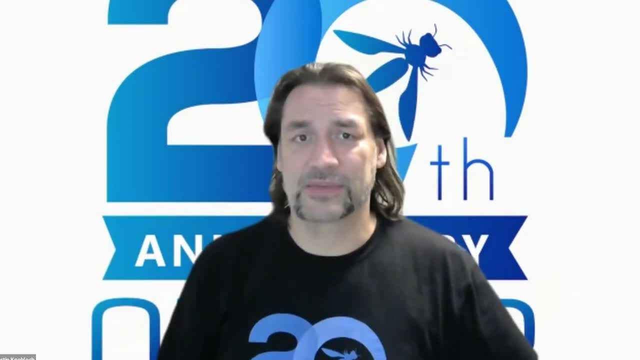 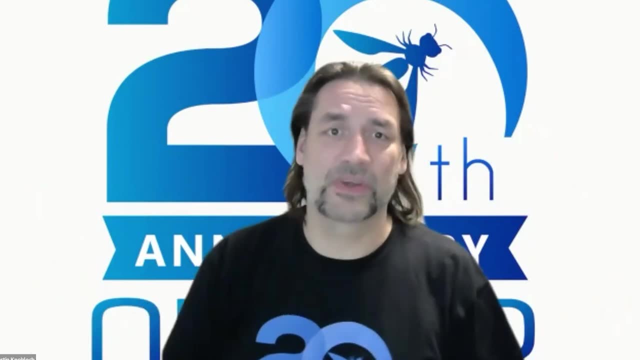 your mobile phone number was so easy because it was a very old process, so i can't call up and hey bang, i'm rock with the fair. they were heavy. hey, we can the phone number, forgetting that this day's, a phone number is more than that and that's the flaw. and you can find flaws only. 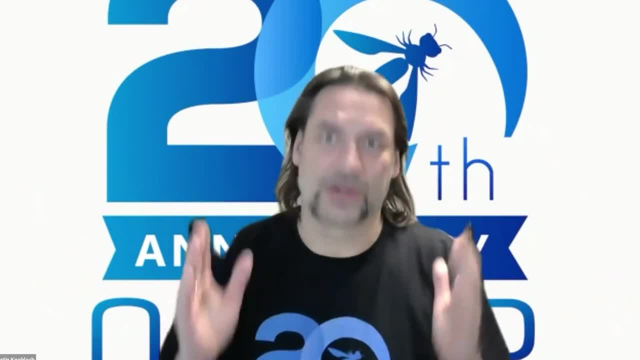 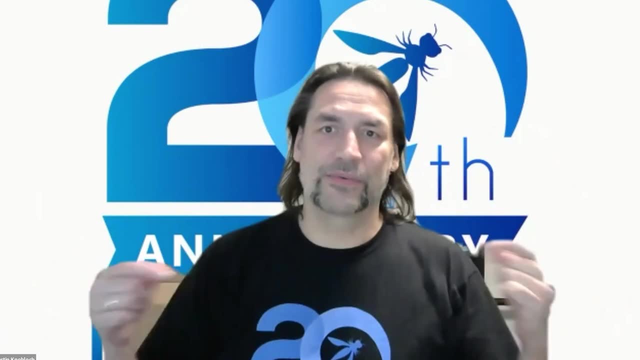 when you look at the same thing with the, security goggles on that's what you think. the same with the also say it's not more secure, less secure than a proprietary software. because we all, as software developers, look at a code in the same context, so you have to look differently in the code and this. 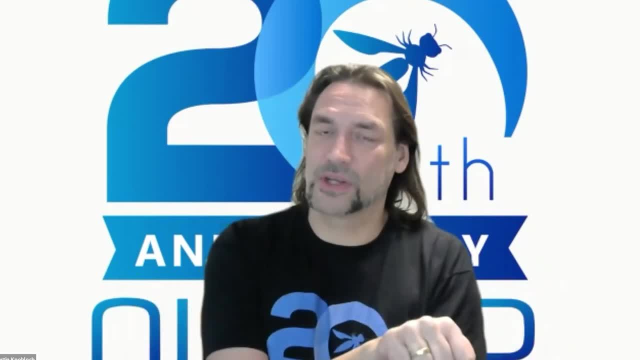 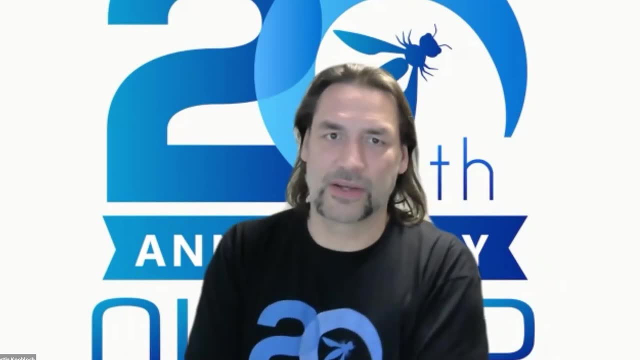 is what i say. whatever you write when you look for security issues on the technical floor, that is, you're creating the writing software right here how you write uh sql statements. i don't do string coordination, for example, when you look at flaws, it's much more complex because now you have to. 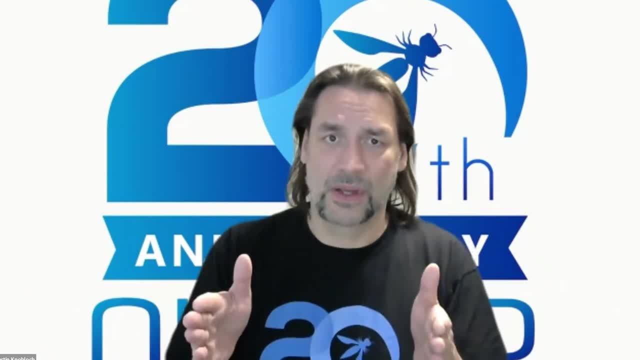 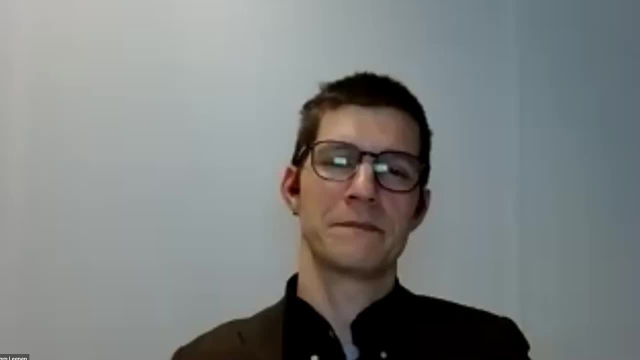 see is the process as i, as a devops team, have over the company process, the data that i have, is it relevant or has a different specification? on the other end of the application there's a difference. so security is not left or right or here. there it's on, yeah, on match magnitude you. 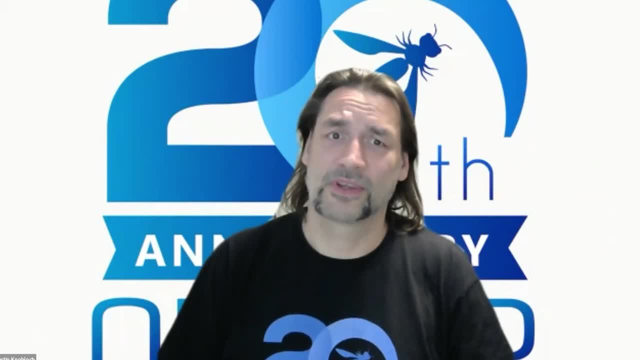 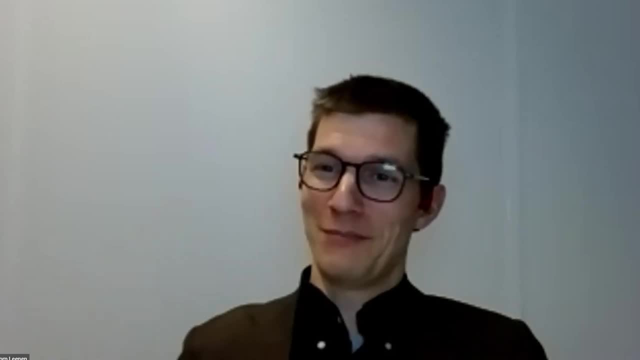 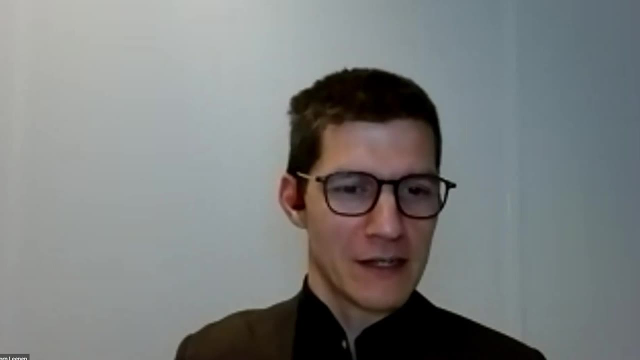 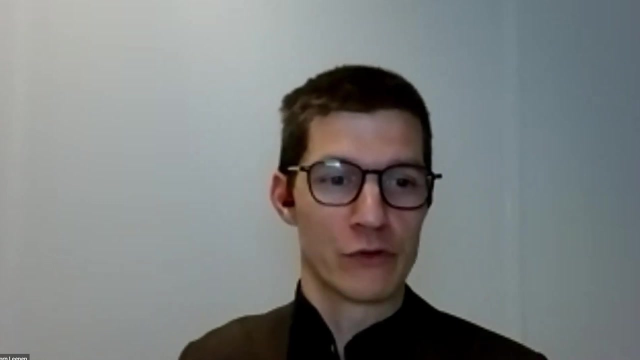 look at it. thank you, no, no, not at all. i have to process this. i have a lot to process by the end of this webinar. um, um, there are a couple of questions about uh, where were they about recommendations about unified dashboards or vulnerability dashboards? uh, are there any tools that people can take a look at? 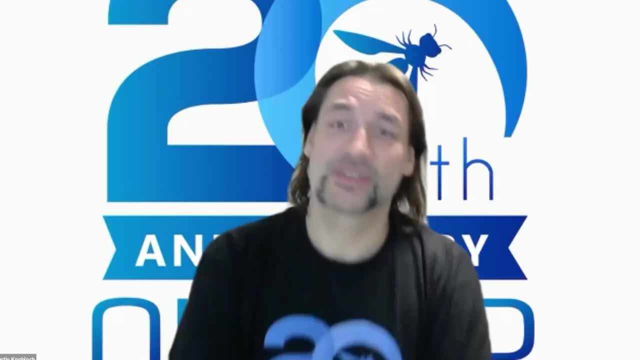 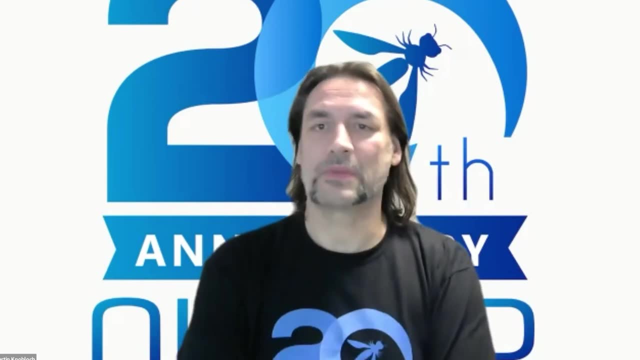 the effect we have. yes, that's what i want to say. it's a different touch, it's a good one. so always open source tool, but actually, um, it's also again depending on what you do. if you have internal development, you want something there. some tools have providers. 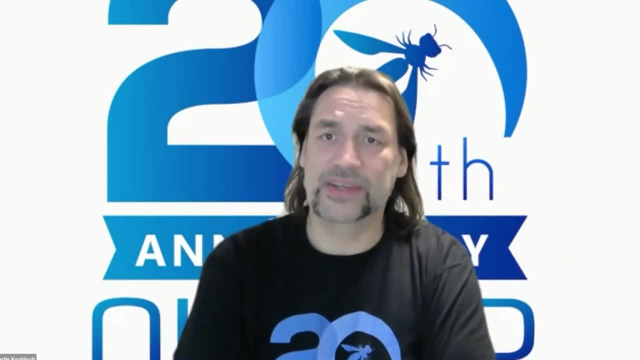 have dashboards. there are also integratable, where there's always had threat tricks with still open source version, but it's not maintained anymore. we always have defect dojo, whereby defect dojo is more intense. to have the security verification schedule, a bad team, right, you have this security assignment: security team. 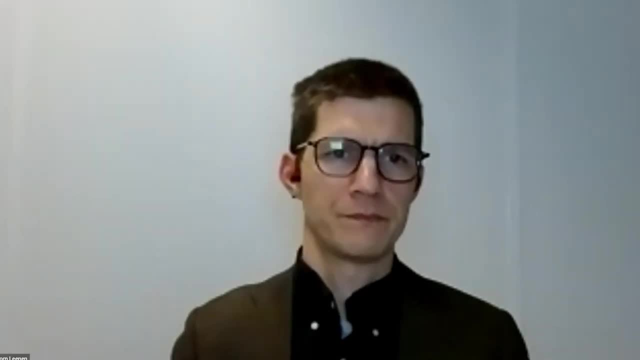 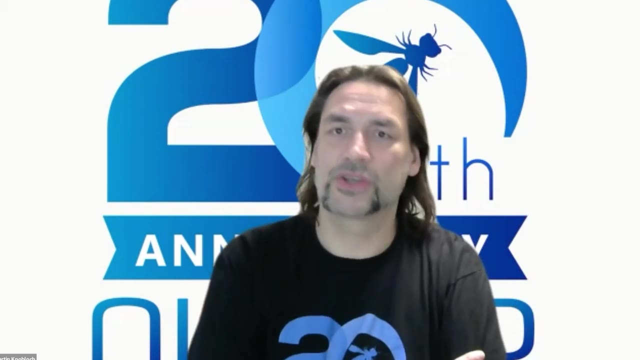 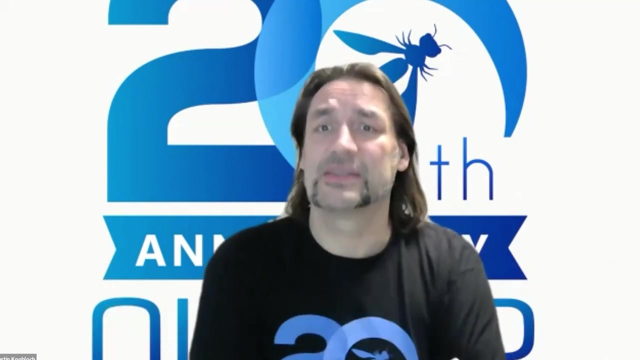 assignment against software development assignments to measure points, but still you can use it definitely on a wider space and uh, they can fit in um different security tools results. because the same problem: when you have different security tools they have different reports so you have to manually see what's all there. different dojo, for example, does that and you can. 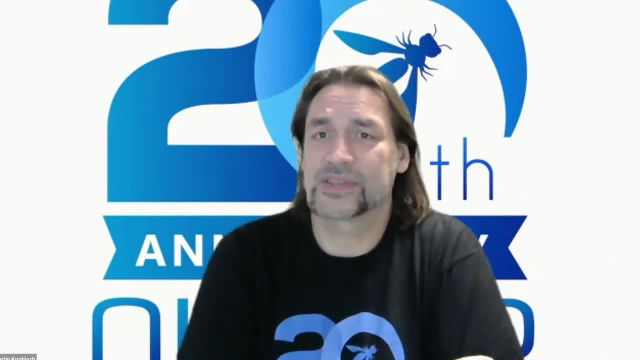 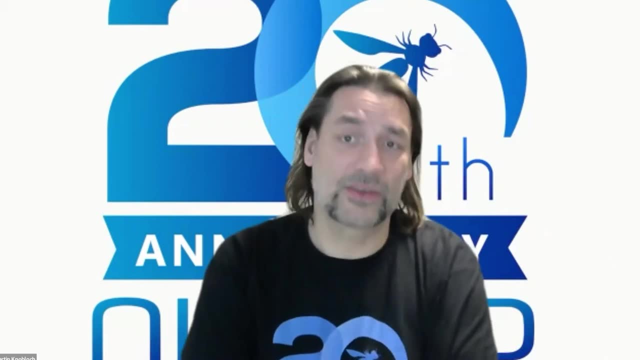 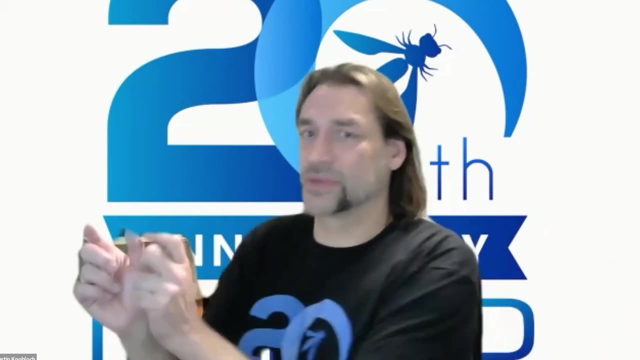 make a commercial about if dojo, because it's an owas tool and everything else is for free. so they understand different tools, uh reporting- and they even can to certain extents correlate the findings from comparable tools. i mean there's two sas tools. they can find two tasks which can. 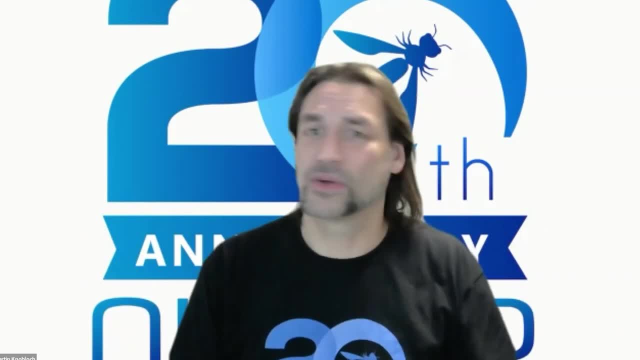 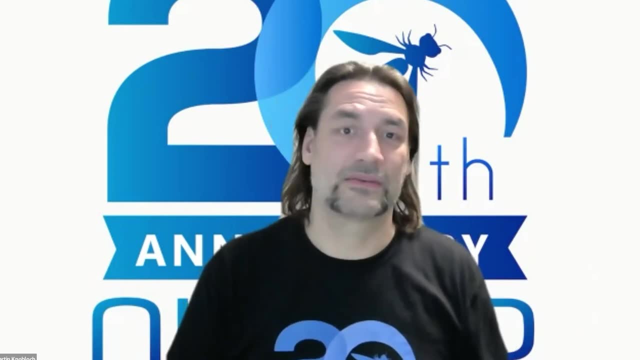 compare it: sas and dash, you can easily compare it. so if you don't come to closest, i would like to see more uh risk component and i know a fender, and so it's depending on what you want and can start with something that you have more than one. 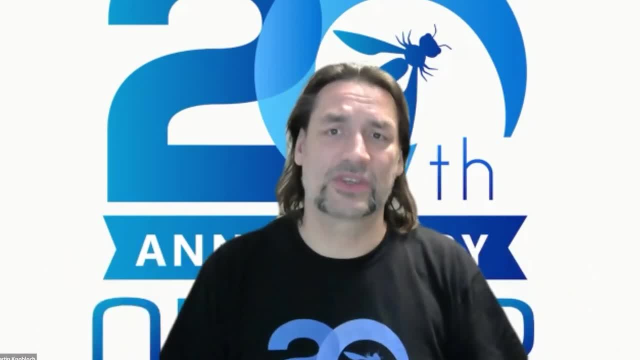 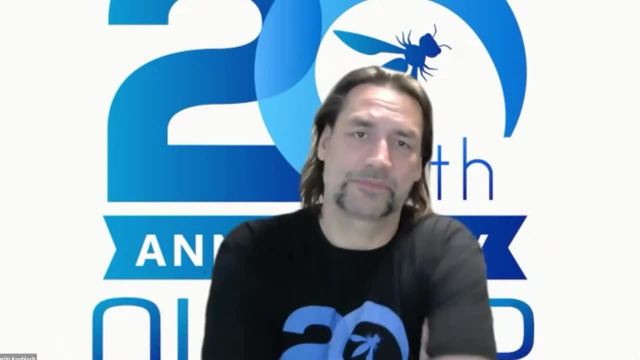 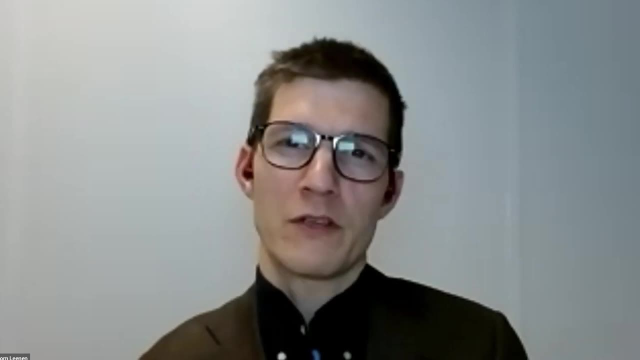 a view on your software and not just sticking to this while i have this tool on this dashboard. try to get a maximum from your dashboard so that every people can use it. no, but i i think how i see people use dashboards is a visualization of where you stand at that point. 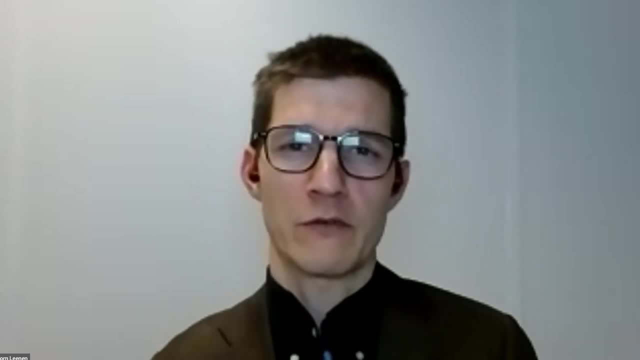 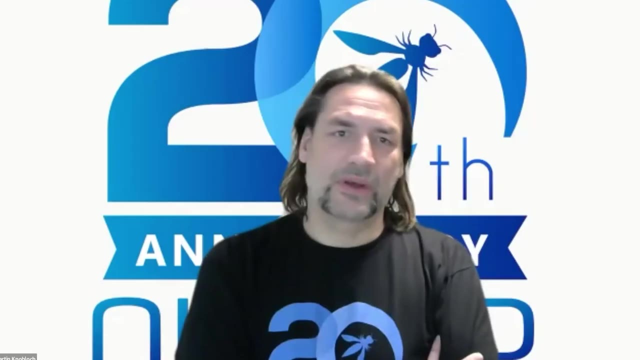 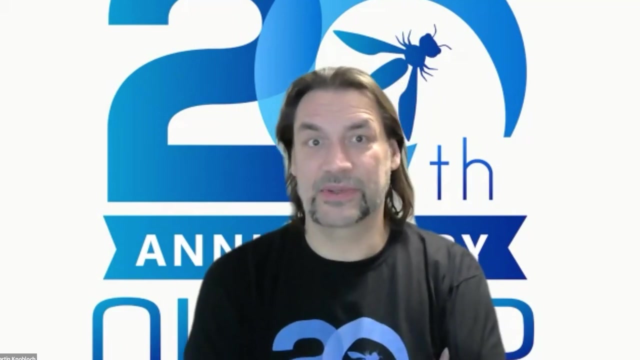 are real time. some of them are more on the scheduled uh interval. um, people aren't quite visual and it's easier to work with dashboards, so that's a bit uh intriguing. you can also see trends right. i said i don't care if i have five SQL injection or six, so the team is six. 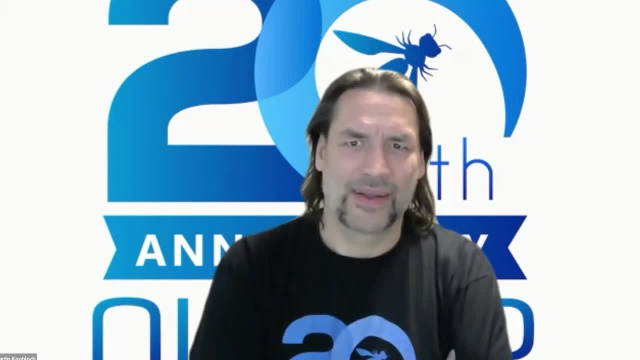 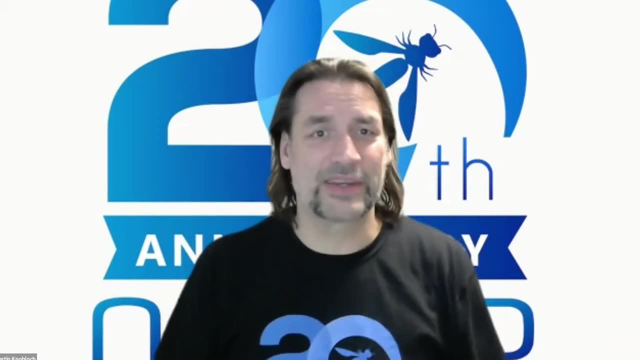 SQL injection is not as good as the one is five. no, it's both bad. so i want to see a trend. do i have? like it's it's going down, it's good, it's going up, it's bad, it's for security, right, it's the other way around. normally you say business is up is good and down is bad. we say everything. 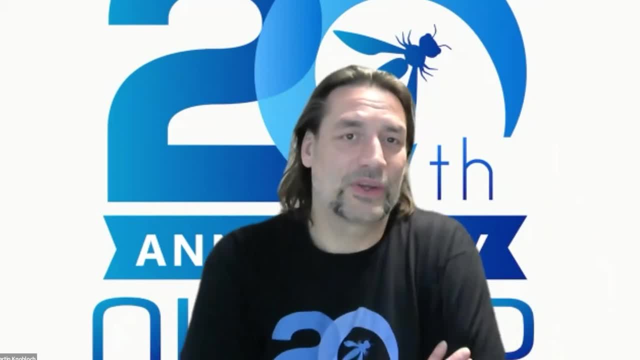 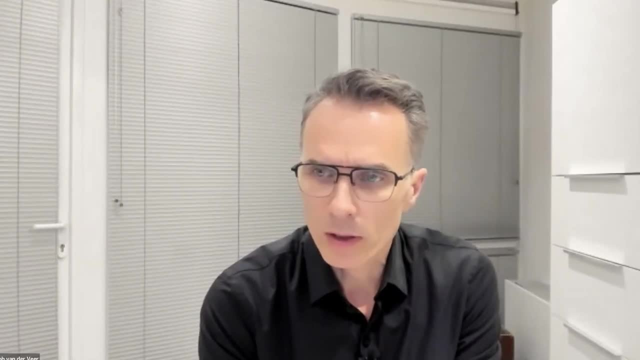 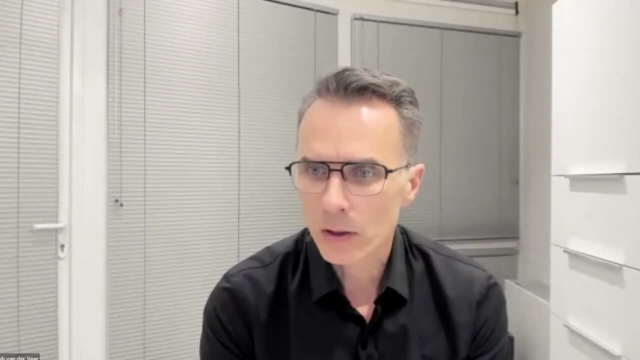 is more is bad, less is better. uh, it's good and you need to find a way to turn this. sorry. so good dashboard provides, you could say, three things: it's visualization and analysis, including the trends, it's integration from multiple sources and it's traceability- uh, tracing, uh, the risk acceptance. 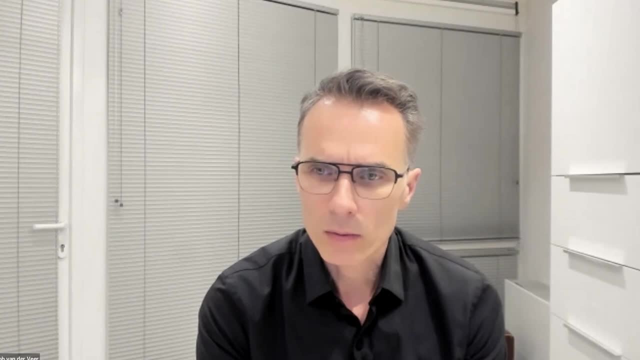 etc. and i know that code dx uh was and perhaps still is positioned as a system that does. this is now part of uh, part of uh synopsis, and we at srg uh cigarette is our platform- we also have such correlation dashboards and uh tool integration in place. we have one, so 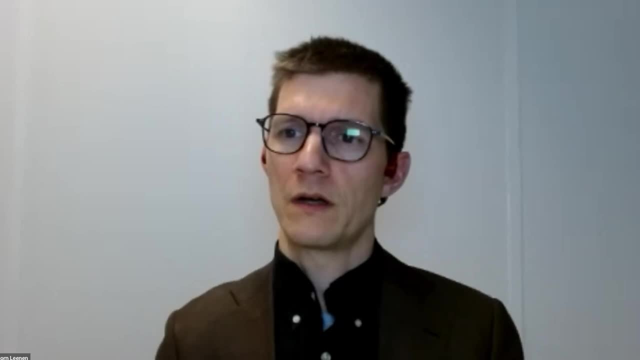 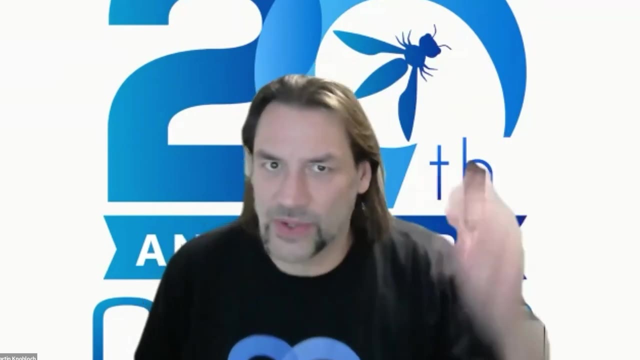 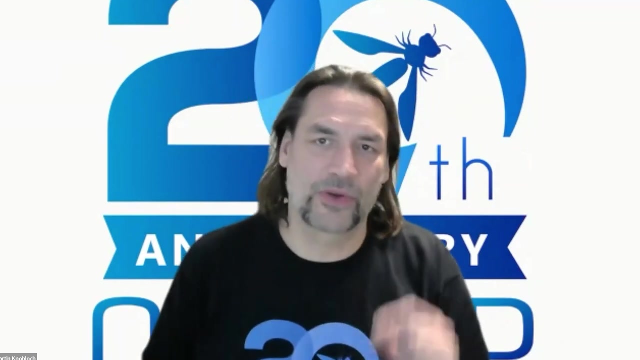 you have one single pane of glass with the whole overview in one. yeah, that's the idea for all these vulnerability tools. yeah, but again, i think that's a different, because when we build tools, we have a lot of things that we don't have in there. it's not just listing your number of vulnerabilities. 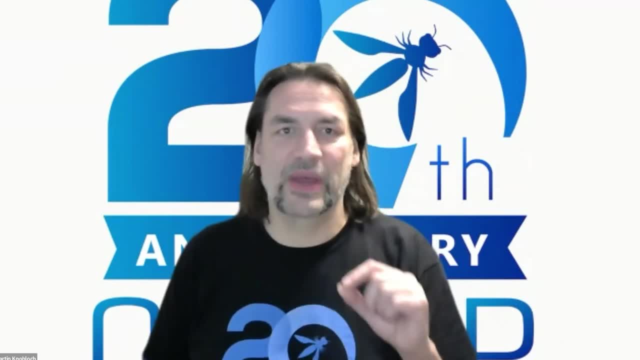 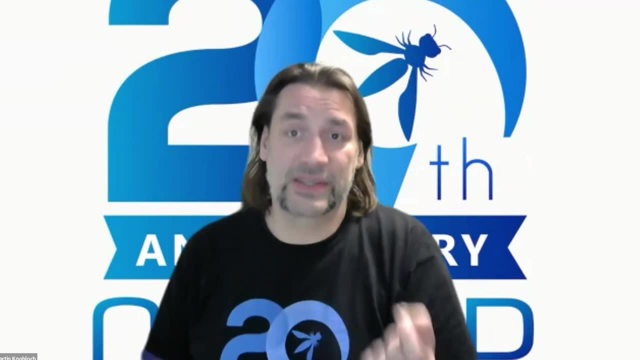 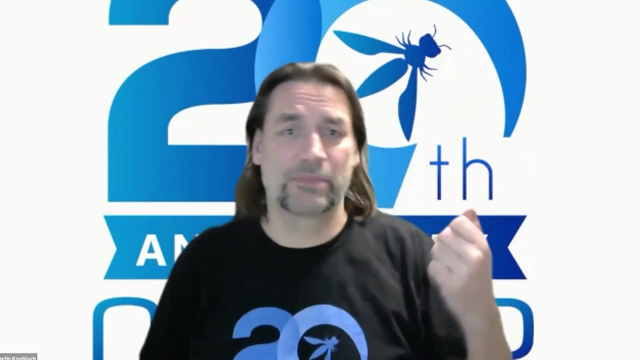 per project or scan. what you really want to have is something where i see that technology to have a racing trend or this trend goes down and not, and i'll see my risk, because when i have the risk I can always integrate in this dashboard. then i don't have to discuss: for example, why do I have 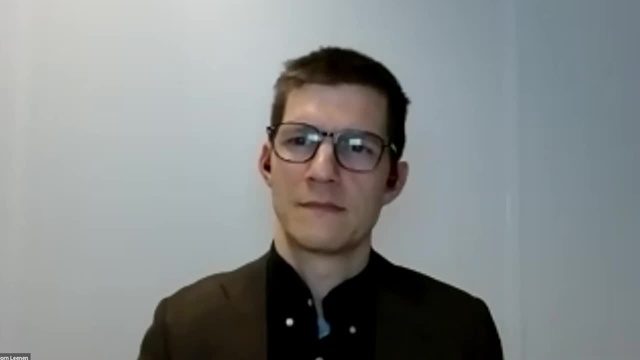 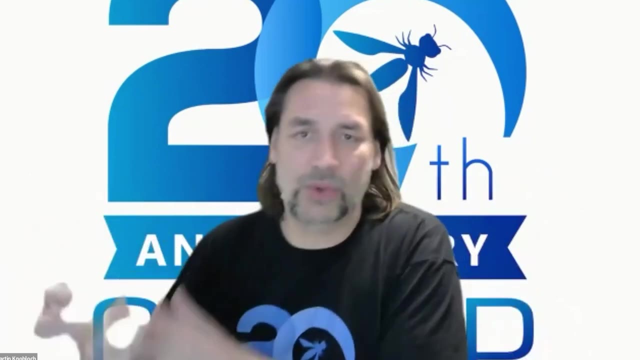 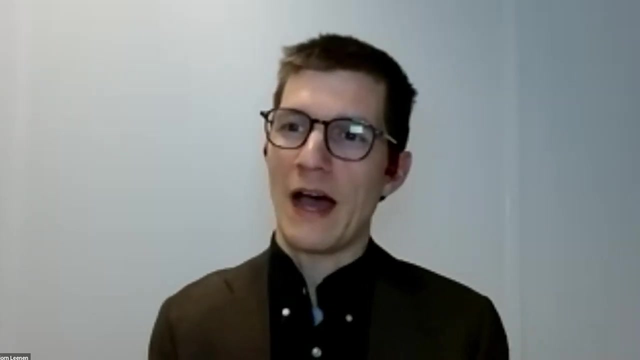 to pay for the renewal certificate. i know that i have a certificate and it's required to this security requirement there, right? so the correlation from security measures to the security requirements to your application is also important. yeah, but is that not part of your impact analysis on what the 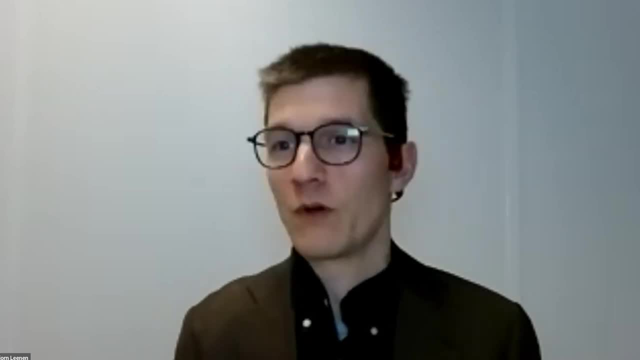 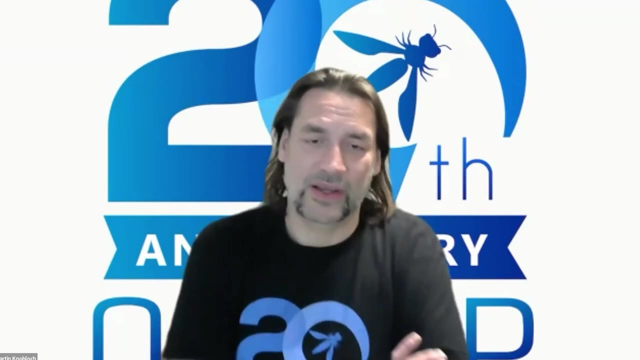 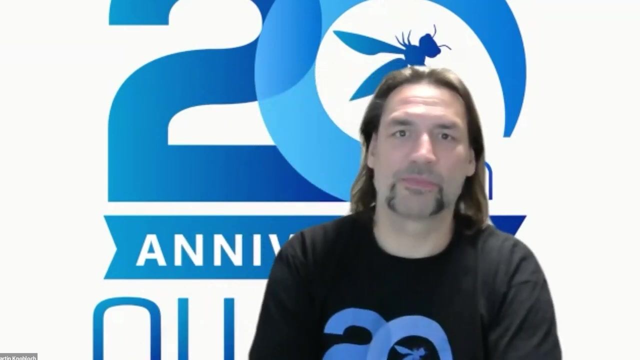 risk is. I mean it can be small, but, uh, if it has a wider use, yeah, so it's, yeah, the thing I envisioned with my talk. it's not there yet. I have seen different tools and I try to do find people, uh, to build this is more than one purpose. yeah, but I, I think 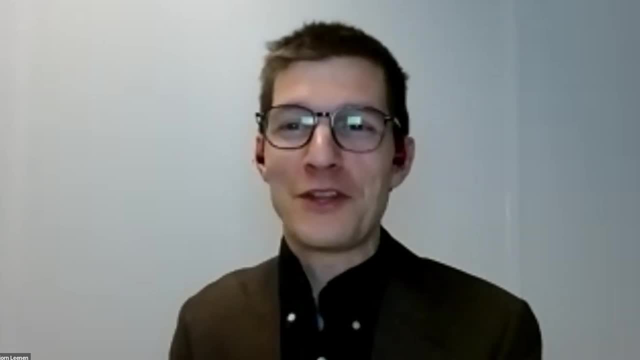 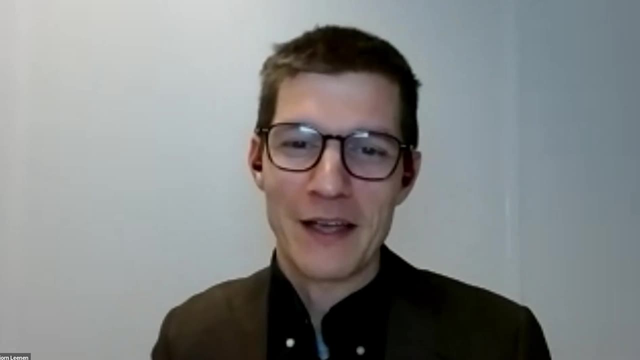 the whole audience here is in in an industry that will never die, I guess, because security is something that will never stop being a thing on the agenda. I think I also see here that Sander Meyer says you can use over secure code box and over dependency check as the SCA dashboard in in. 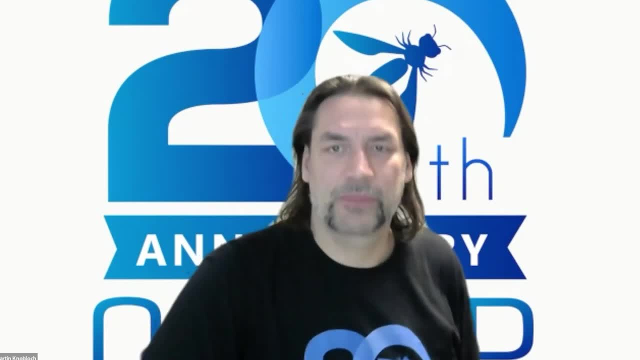 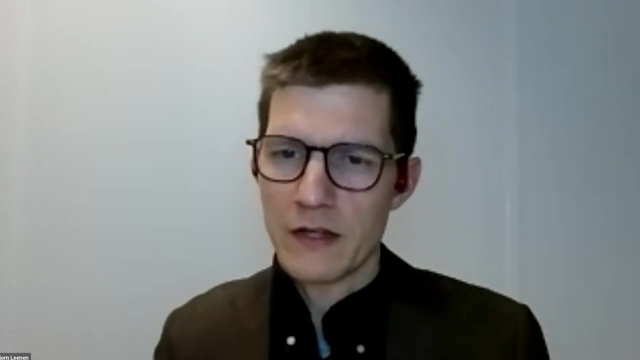 chat. um, yeah, that's what? yes, dependency check looks as an SCA tool, so dependency check by itself. that looks in the normalized for the National vulnerability database about normal, and so for the libraries it does have its own dashboard. yeah, that's a dependency track, but is it again? it's a dashboard for one purpose, okay? um, I just saw one one extra question pop-up after. 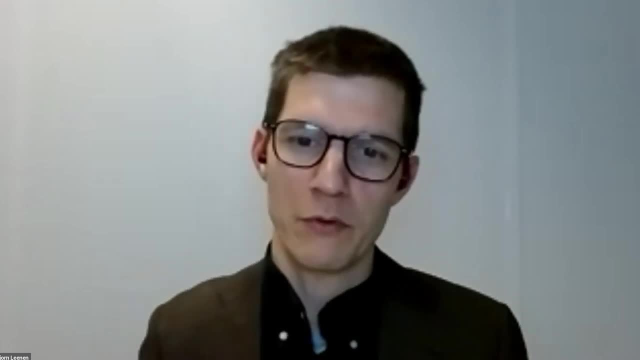 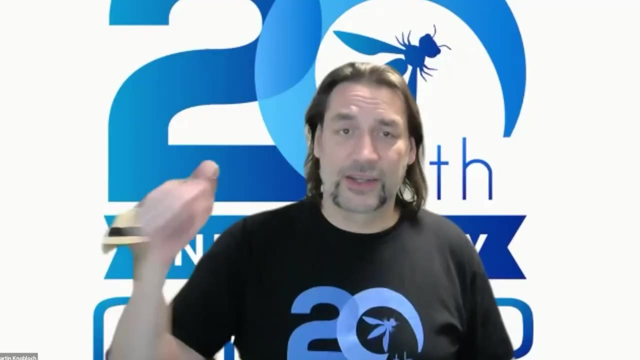 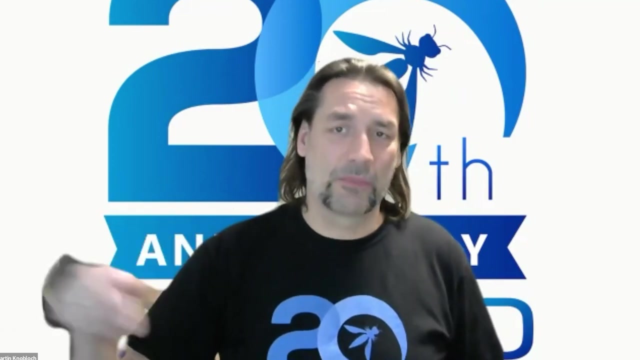 that: how do you set up a security Champion learning path? a tribe around it and how to make people enthusiastic for it? well, gamification, I think. yeah. talk to HR, yeah, because people forget. you think, oh, we have to fix it. no, it needs to have a way for them because they are part of. 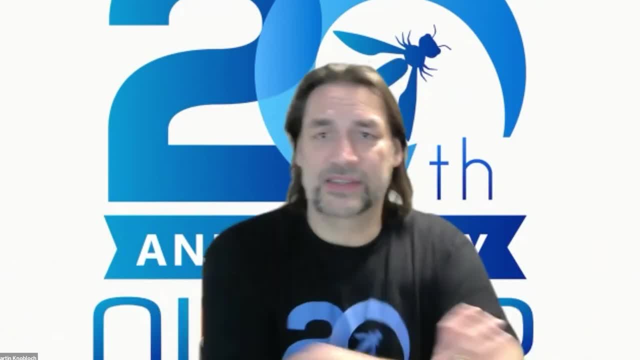 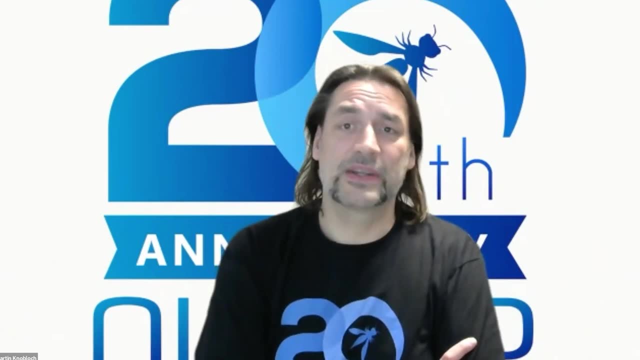 development. so they're not getting paid for being a or they're going to get the bonus as a developer being a security champion. so you have to make it a role in your development environment. yeah and um, different initiatives, even on the OWASP about security champions, and in the Netherlands we're. 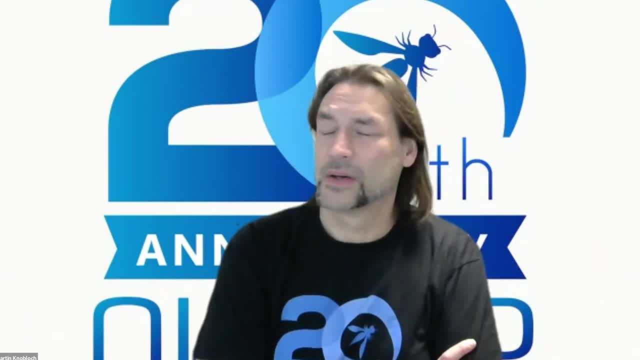 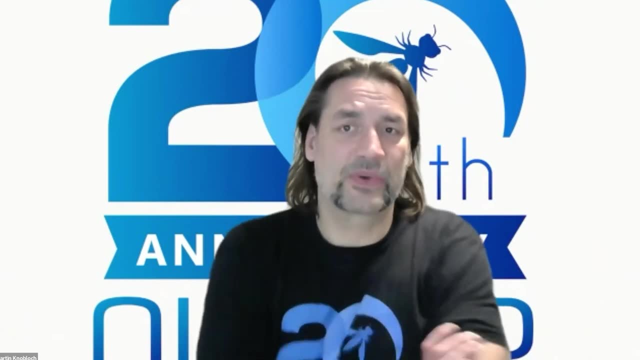 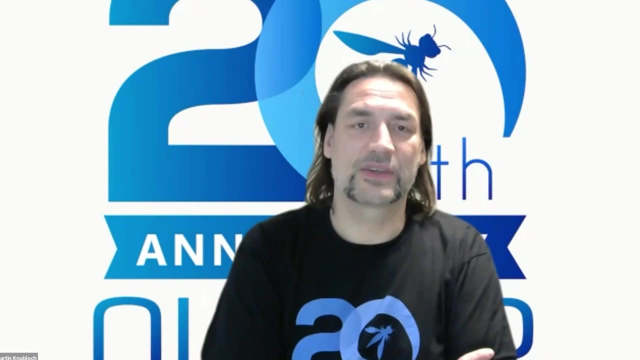 looking also that for a Dutch project. but there's also the OWASP. it's not called security champions or button project anymore. but how to do incentivize those security champions? because it's like an architect and a software architect in the one company. it's not the same as the software, I think, the other company. so what is a security champion differs? I said my 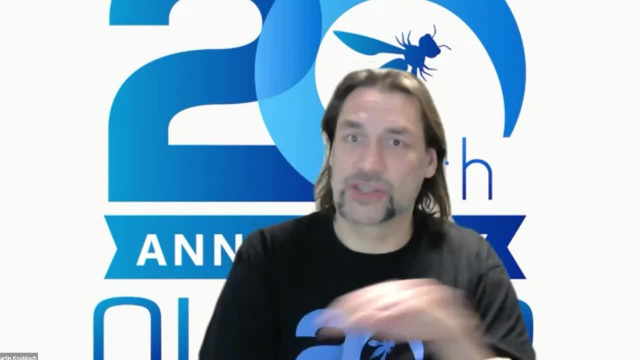 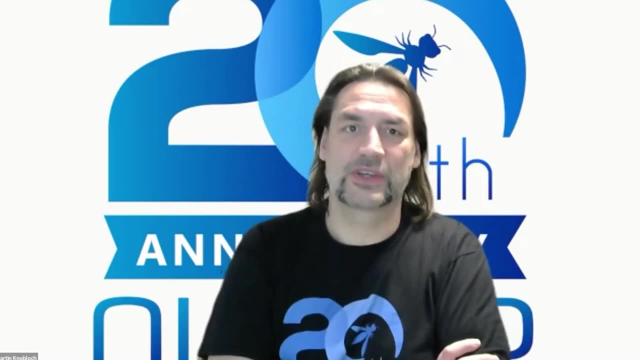 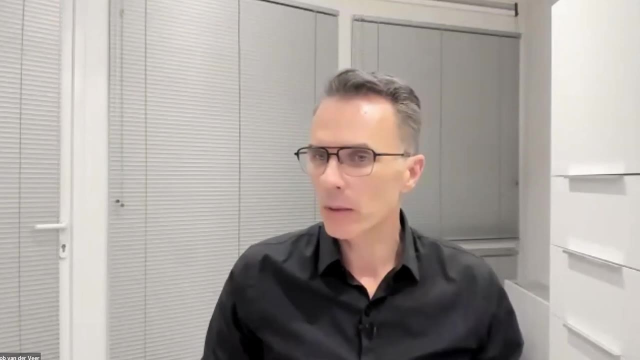 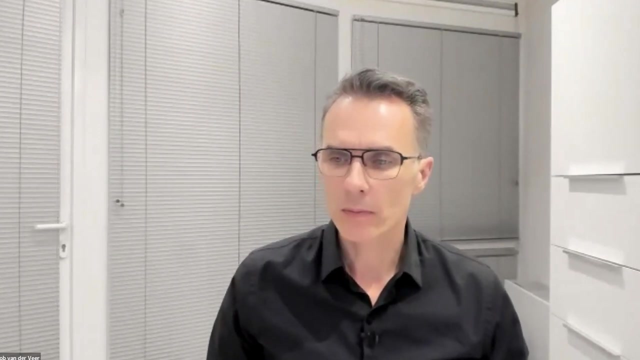 opinion, it should be those who, not being shifted off, left the security requirements, not doing the best stuff, but should be like that: the alliance song for security to development, right, yeah, yeah. so the, the enthusiasm is preferably intrinsic, but then people also require, as Martin says, the enthusiasm for actually having the mandate, uh, to spend time on this, true, yeah, yeah. 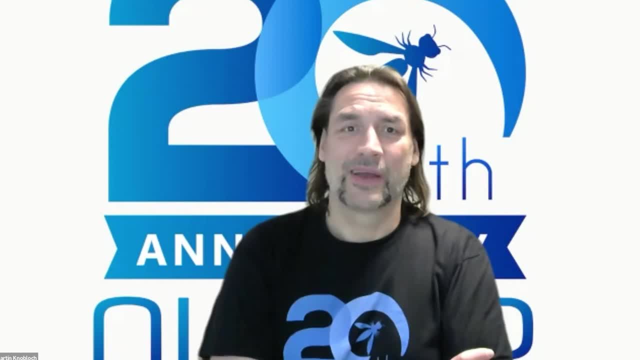 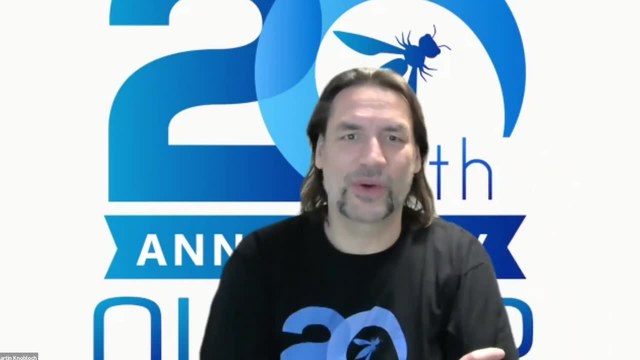 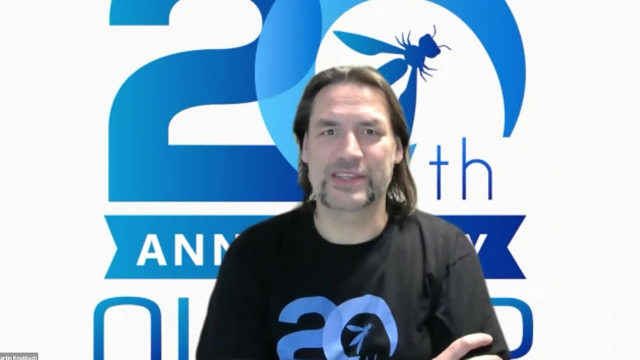 and when you want to create one, talk to us the developers. right, we can think about. oh, we need a security chairman and uh developers who is a private volunteer? no, you have to make them enter us first and whatever initiative you do, you need some uh William Wallace who goes in front of. 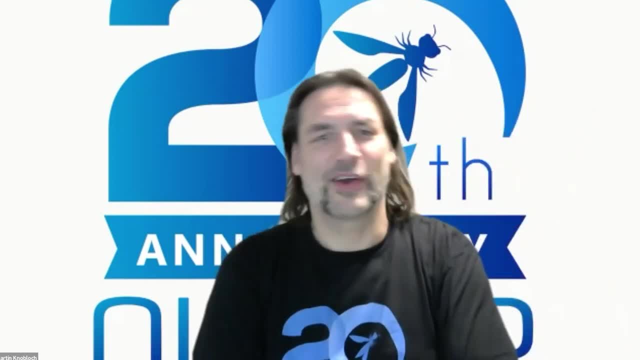 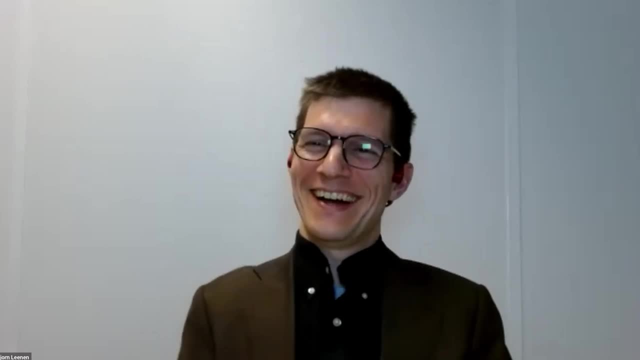 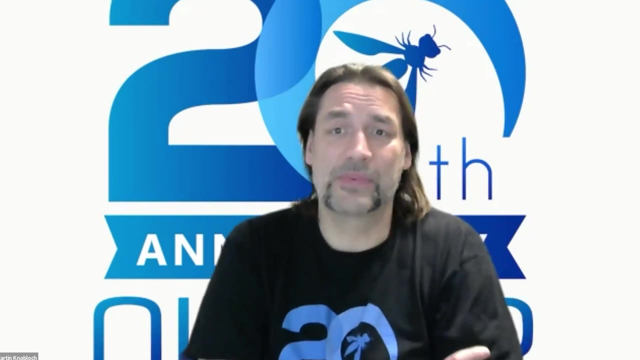 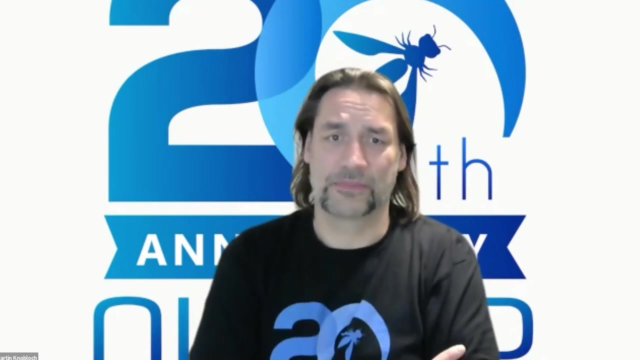 the league says: free Scotland, down the health right and then you have developers who care. you will have somebody who actually wants to lead them and help them. let the developers find the security. it's not a security plan. you don't. you have to mentor them, not to create it. 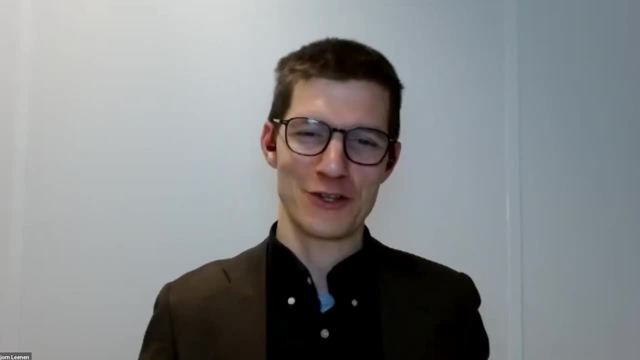 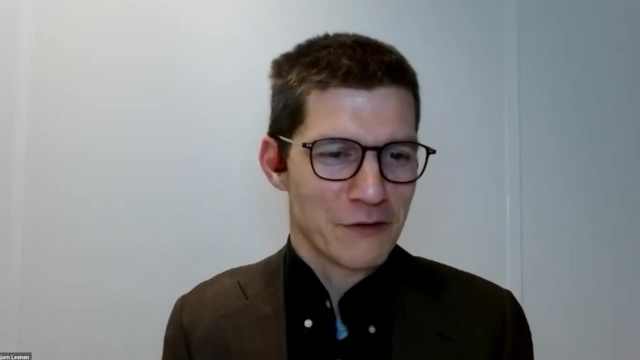 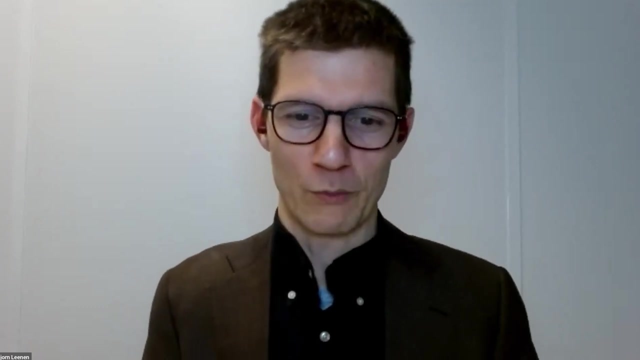 cool, I think you get just got a thumbs up from town the the question and the the person who. who posed the question. so, um, there is a longer question for martin from mark uh chang singh pang, if i pronounce the name correctly for martin at slight dev sec ops who makes the architecture? 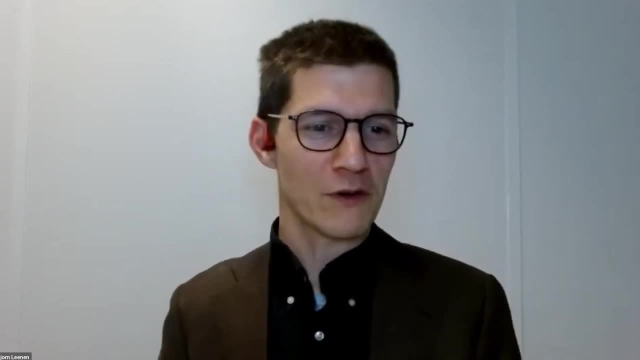 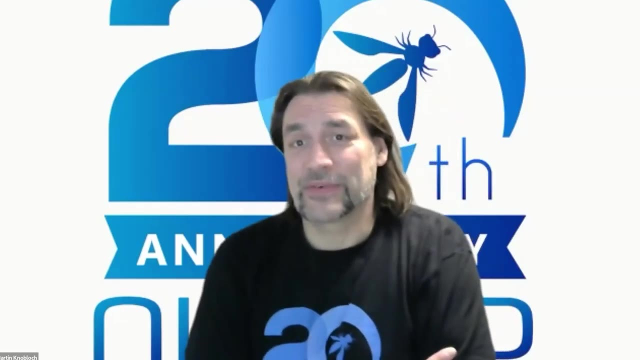 of the system. you say in dev, you start coding. who defines the application architecture and the overall system? architecture, again, when you talk about internal development, is different than we have. portrait teams, so we talk now devops team, so we talk internal development, so you have to have 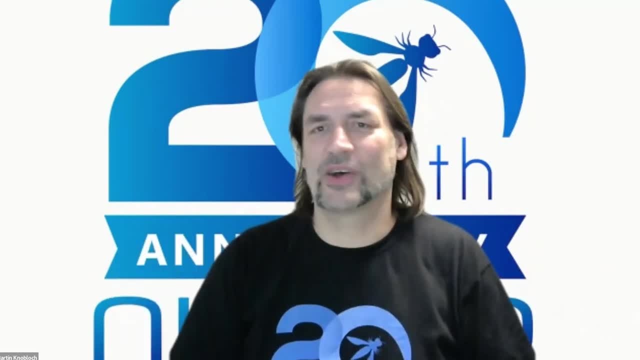 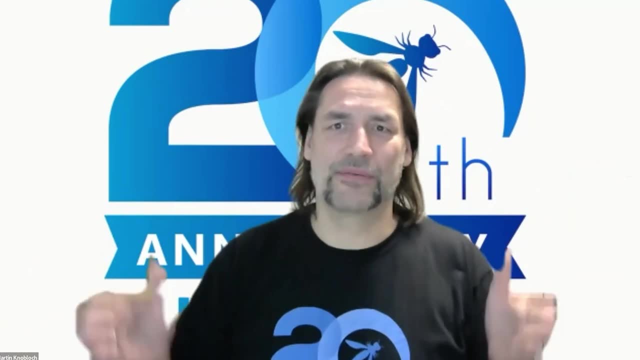 your outlines. i remember that when i was once in the customer i said: oh, it's agile, it can be everything. you say, no, even in agile, your bicycle shop will not be a bakery tomorrow. right, you have to have your fundament right, and the same with technology choices. and you do it, yes, as i think. 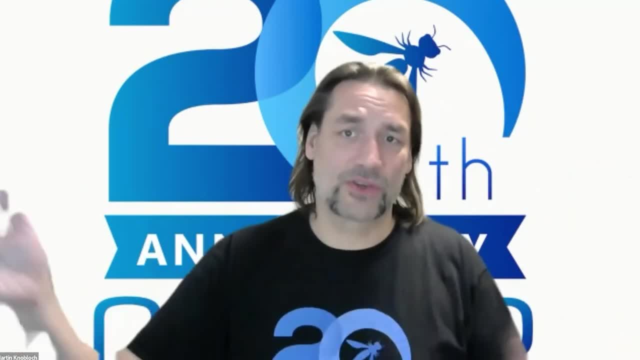 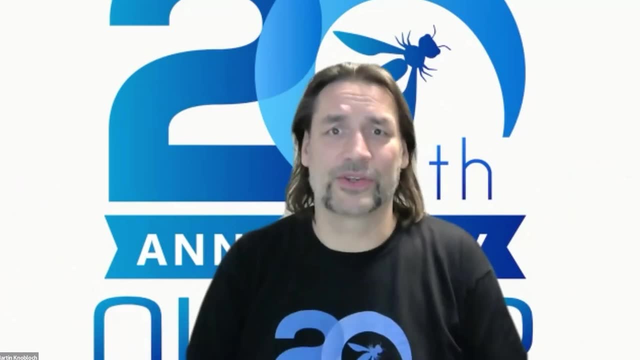 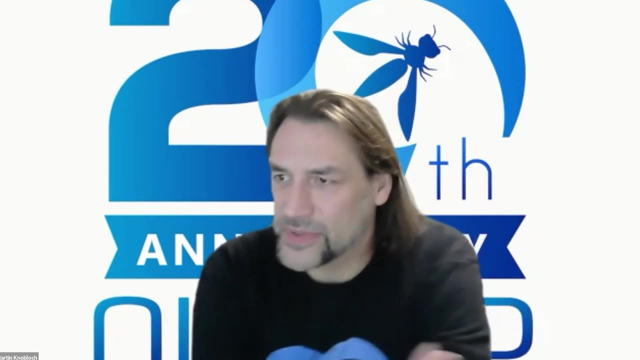 normally those say: which is my target environment? so you have to talk to the operations. guys, if you go for azure, i don't start uh um, using um aws technology, right, so you have your outline, your context. so it's, it's a natural ingredients. you actually have to limit it with some applications. yeah, you have still have to. 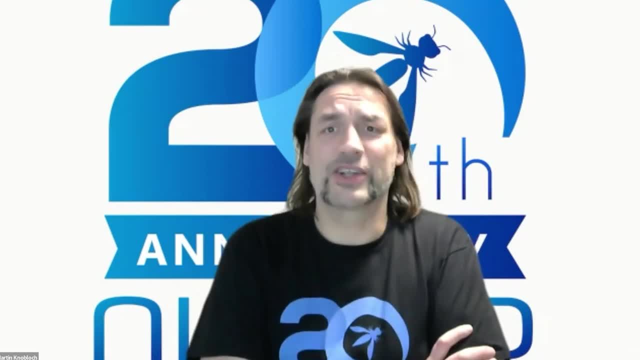 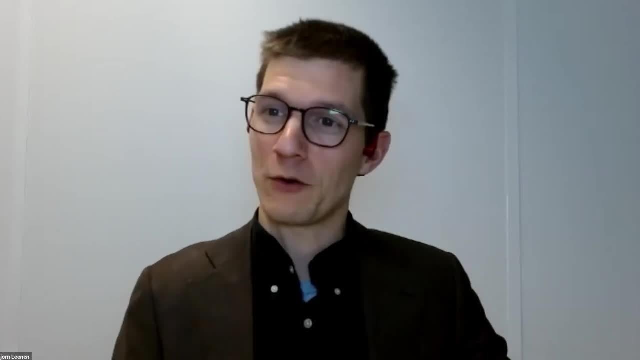 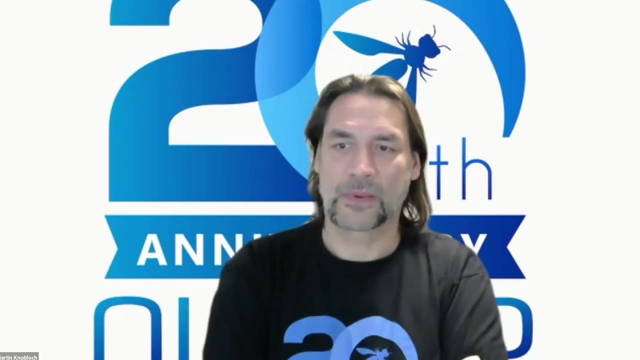 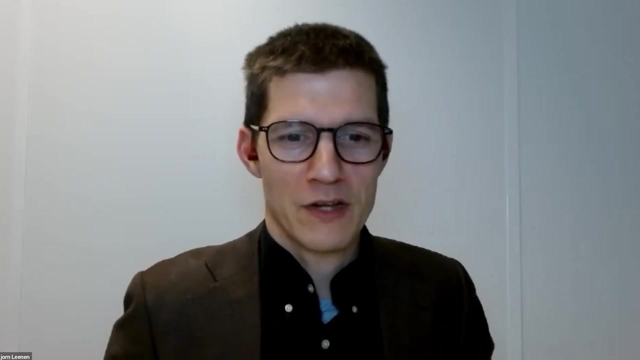 as you have to make choices. as i said, with bezos you can choose, yes, freely choose between the one or the other and not between, yeah, or even, if we go further back, you can choose black or black with ford. yeah, yeah, yeah, yeah, um, uh, oh, this is an interesting one. i think it ties into the question that tone asked: uh, how to. 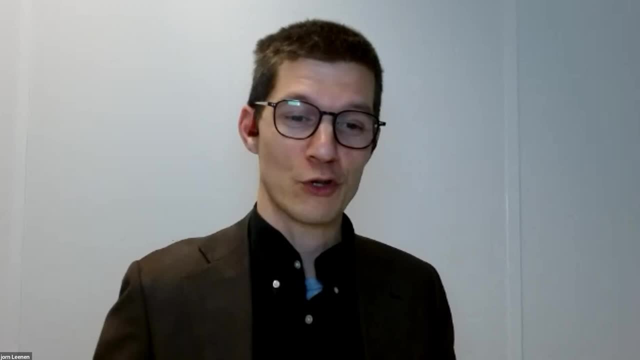 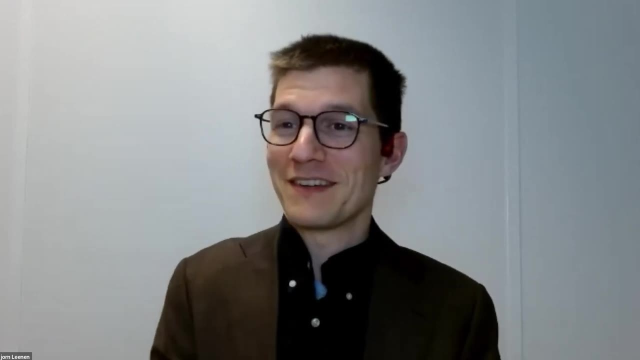 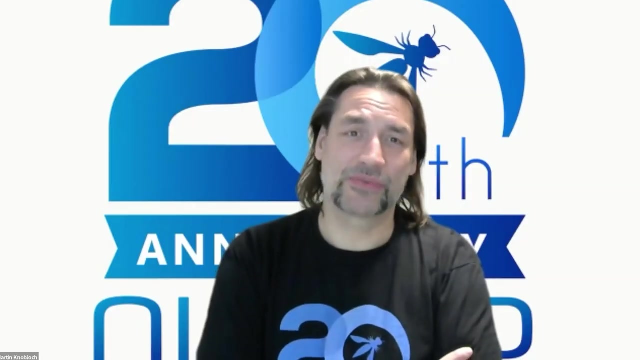 magically transform functional testers to test automators or security testers. actually, a lot can be covered with normal testing, though there is a lot of ground to win. it's more like a remark, but yeah, how do you transform people? well, a tester to secure test. automation is different because 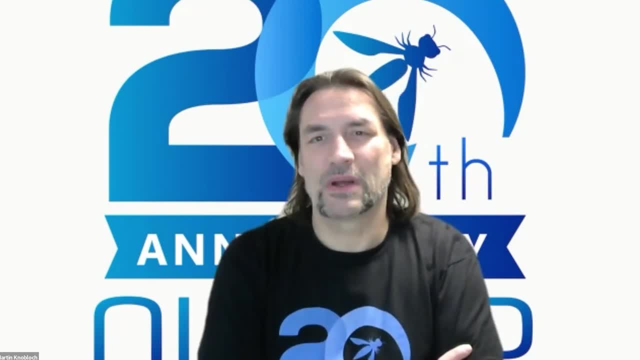 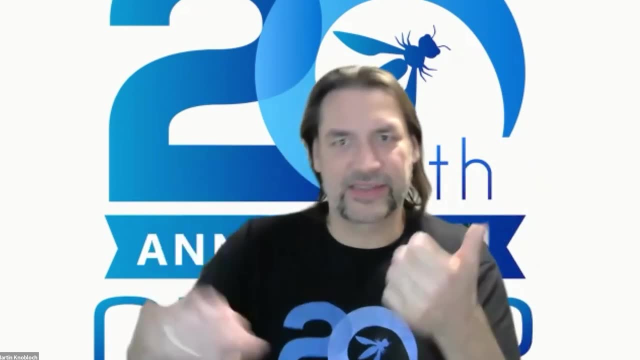 i think that's, i almost would say, the new type of test, right, the the really test of the system and test the time out with the stopwatch, hits the button and does 30 seconds and teach us again. no, it's not these days anymore, so we will. 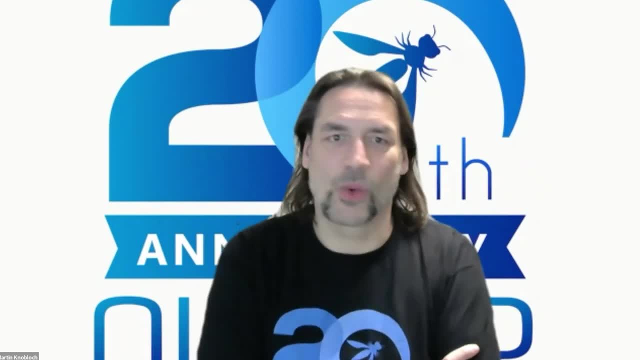 all more mobile. uh, test automation. that that's the way to go, otherwise you can't handle and be flexible and do the the velocity of teams right, true, um, i think i, if i would have to choose, i rather have a security aware developer than a software development, a real security guy, because 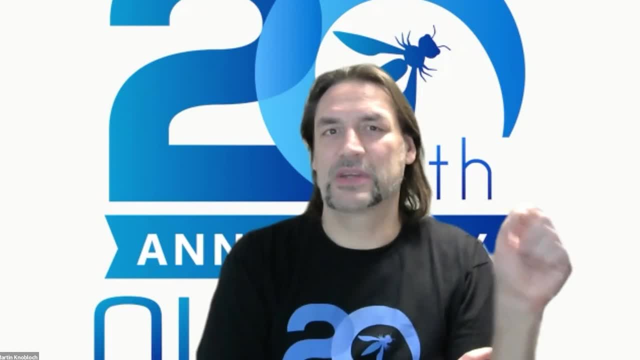 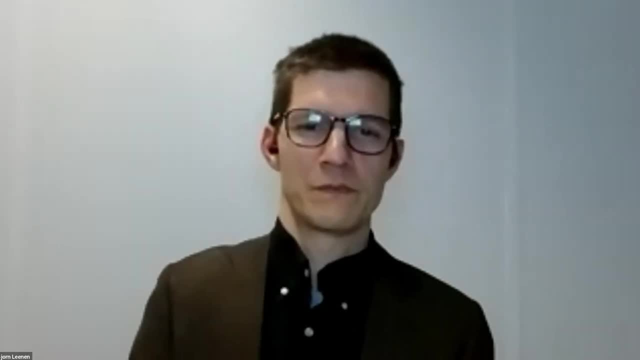 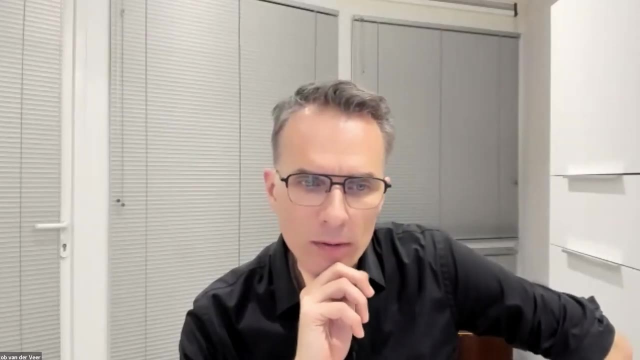 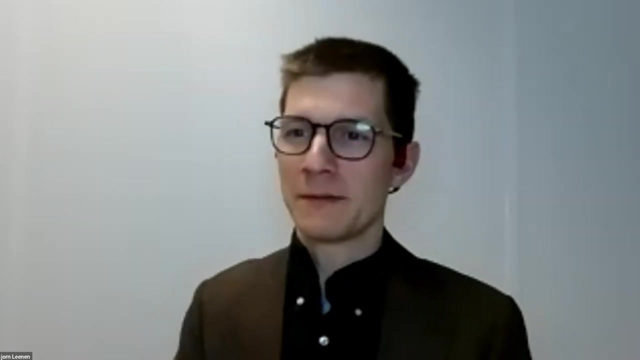 i can't teach and develop a security, but i cannot teach as develop the security guy's developer. no, no, true, true. you think the same way, rob. or when we look at the typical tester, uh, if there is one, but let's say uh, the, the, yeah, let's call her tina the tester. you know tina tester, um, tina can present. 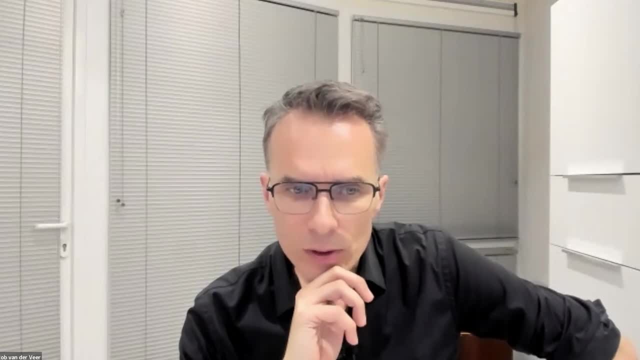 the system with prepared abuse cases. um, you know, i think we can truly see that we can really build on that. i think that's key, because i can't teach and develop a security, but i can't teach as a devel. uh, security cases, of course, uh, and, and you can also learn how to automate them by scripting these cases. 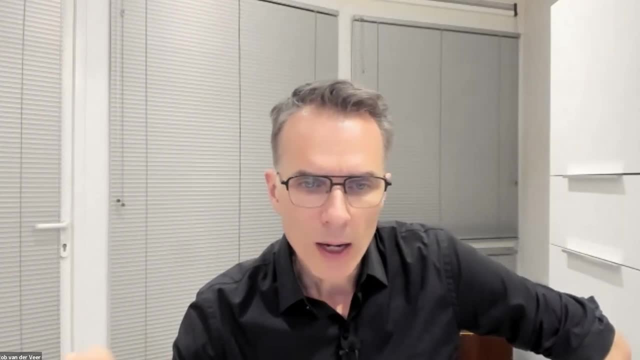 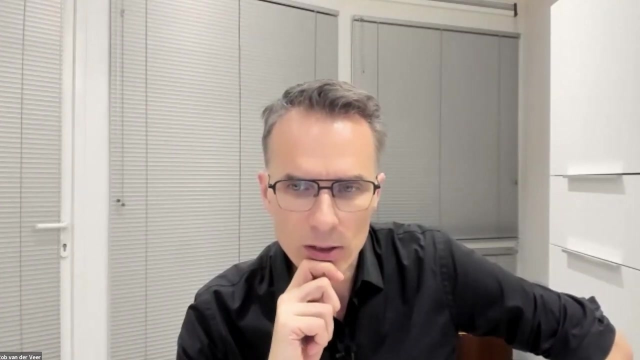 but at the other end of the spectrum is the really creative application of tricks and tools, actually manual penetration, testing. that that requires vast experience and knowledge, and it depends on the affinity and the experience of the tester whether he or she can learn this, and one of the key talents that are necessary is what i call the attacker mindset. so it's the it's. 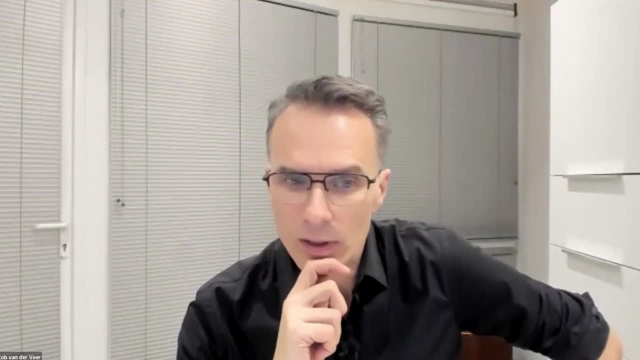 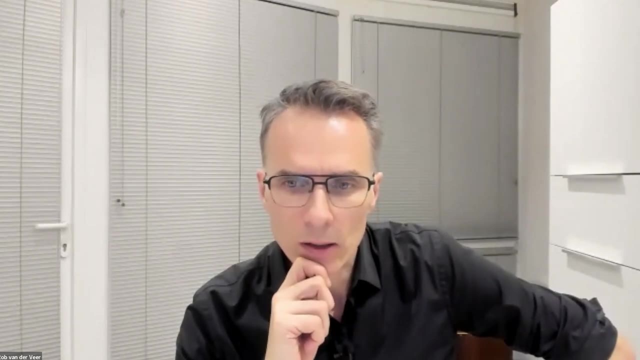 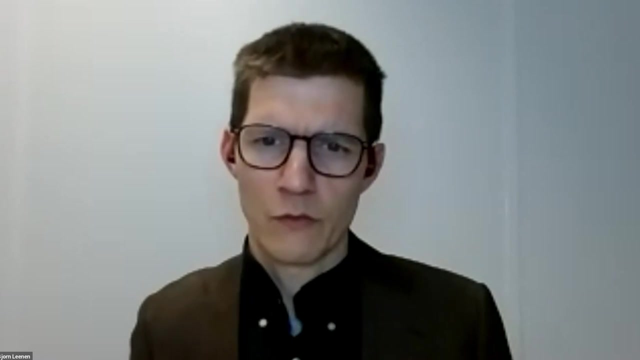 the talent to be an attacker, and definitely there are um many typical testers out there that that can learn this, but it requires a lot of time. yeah, okay, so i can only imagine, um, rob, do you know good tools to manage this library of acceptance criteria? there are requirements, engineering, 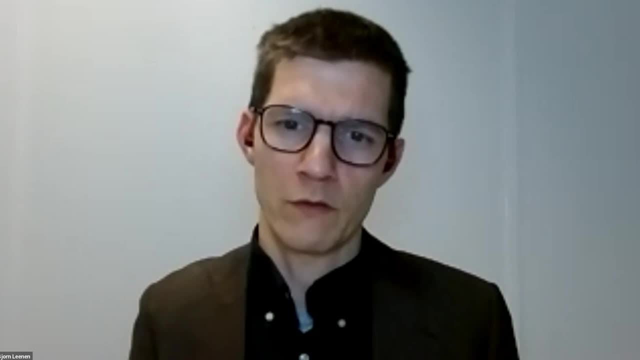 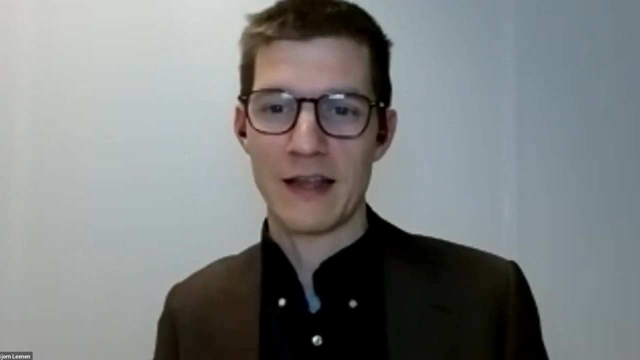 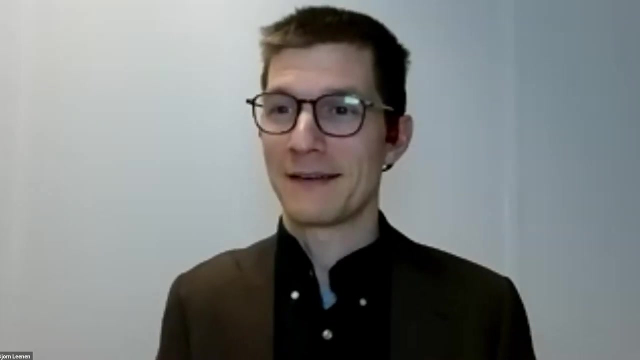 tools, of course, but many are very dated. but what for acceptance? uh, what for acceptance criteria? also consider integrations with popular devops teams like gitlab, azure devops and github. yeah, by the way, github is down. um, what it said here? yeah, i don't know if it's already back up online. 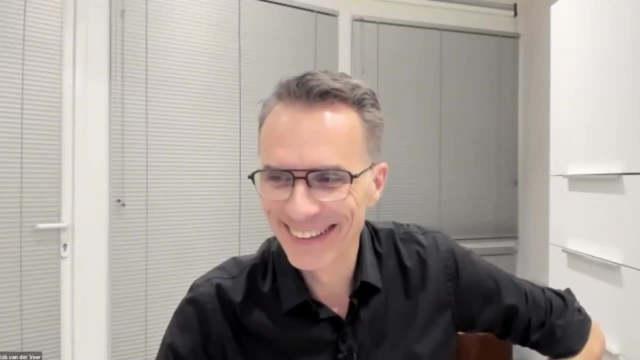 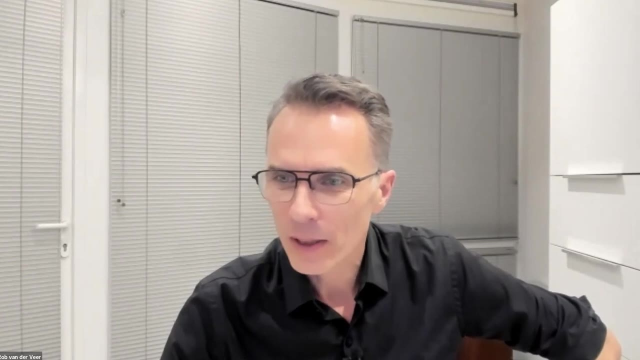 but i need to make some calls. people were chatting about it, all right. um, now i'm a bit, uh, distracted by the question, so, there, this is bleeding edge, uh, which makes it really cool. the way we solve it generally is we map the, the triggers and the requirements, uh, on a tool that organizations. 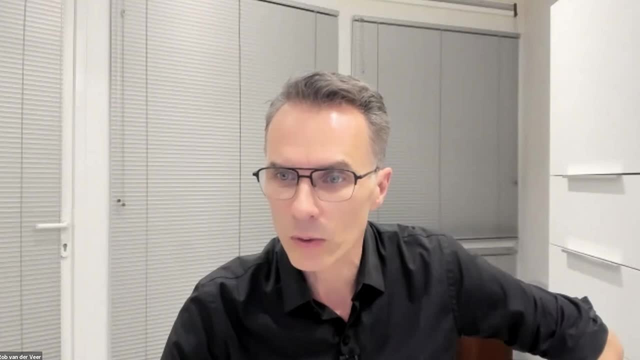 typically use for uh accessing knowledge, which is mostly wiki. yeah, they use the wiki to get access to the triggers, to the right uh instructions and tests and they basically copy paste it to their their tickets in the in jira, for example. that's uh a way if you don't have a tool, but it. 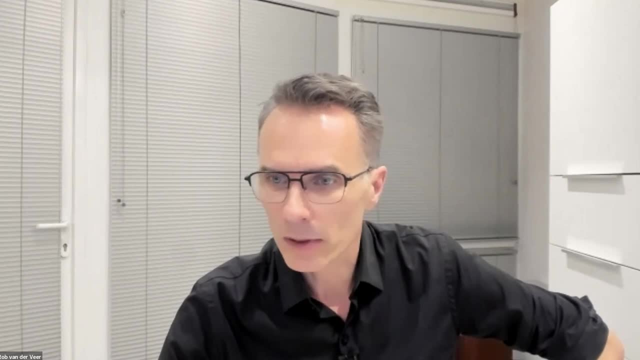 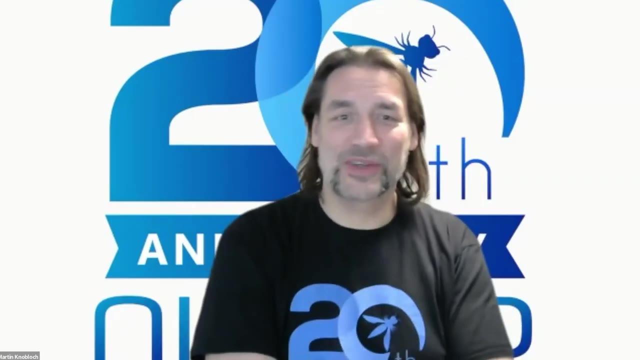 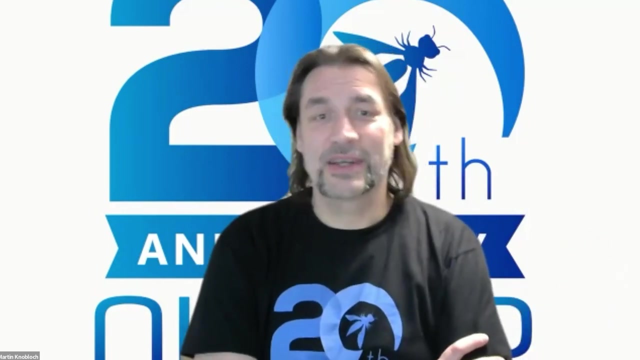 nicely integrates in the existing infrastructure, but it definitely is. uh, this is a, this is a blue ocean. i would say yeah. what about security reps? the over security requirements automation tool- and we have always skf, but actually it's developed by two dutch brothers that actually has a checklist where you can. 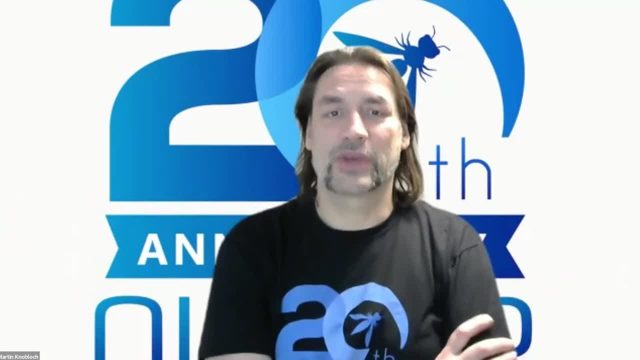 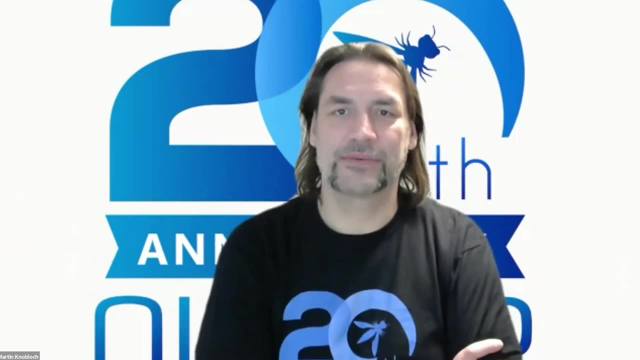 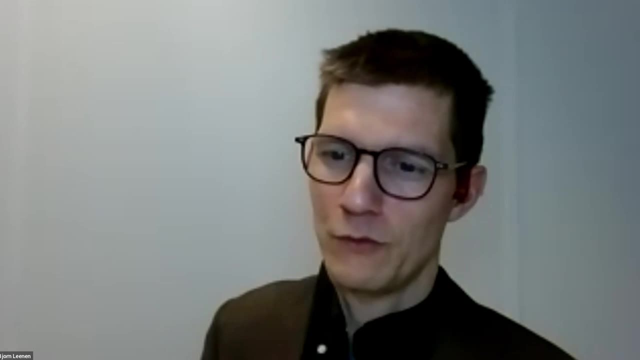 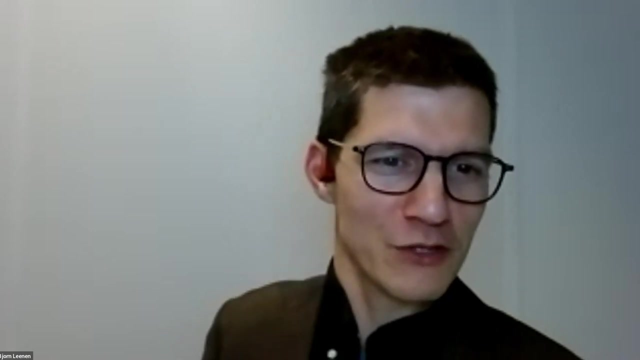 always asps or another one if you want, and you can do requirements there. your sprints by functionality. they have the always security knowledge framework, skf. very cool um tool to implement. yes, thank you. um. i'm trying to catch up with some of the questions, if we still have a few open, because we are also nearing the end of the webinar. um. 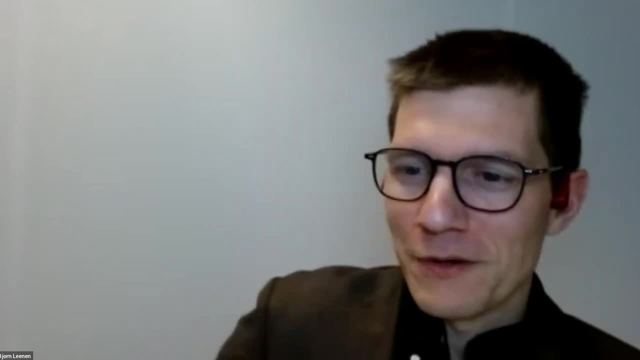 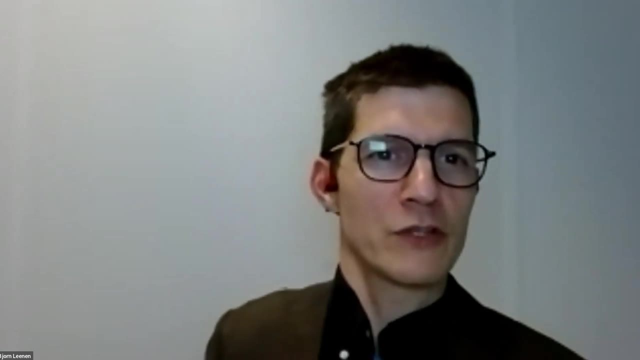 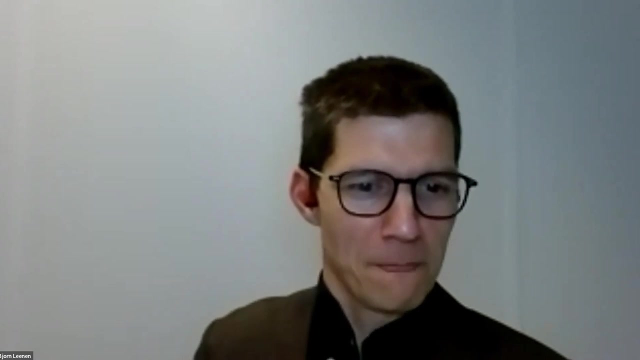 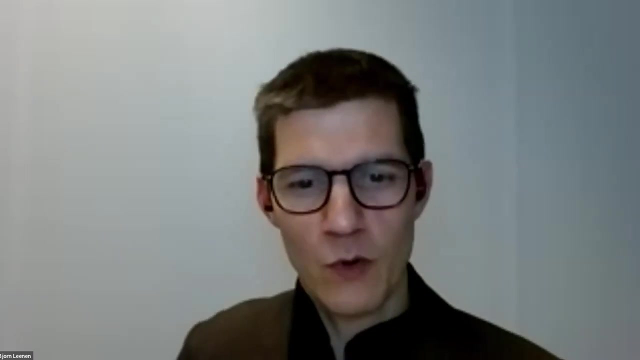 and if you see any support, please let us know. ask any questions, okay. yes, elchien, i saw your remarks. um, let me see. uh, oh, we still have a couple. oh, no, no, that's my old deck, sorry, so many questions. um, we have to come back. 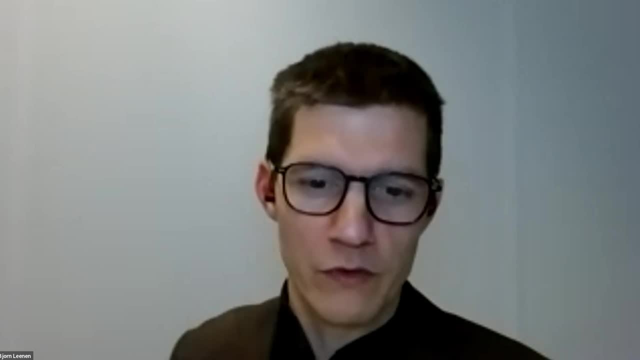 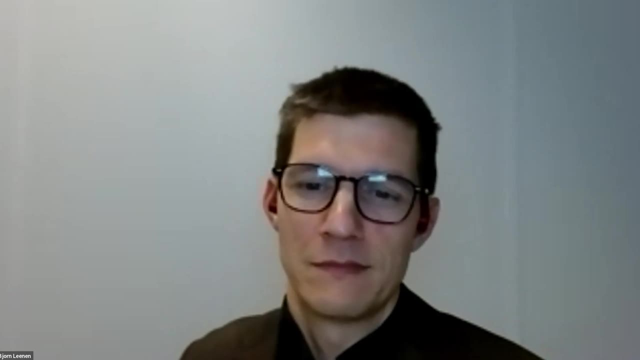 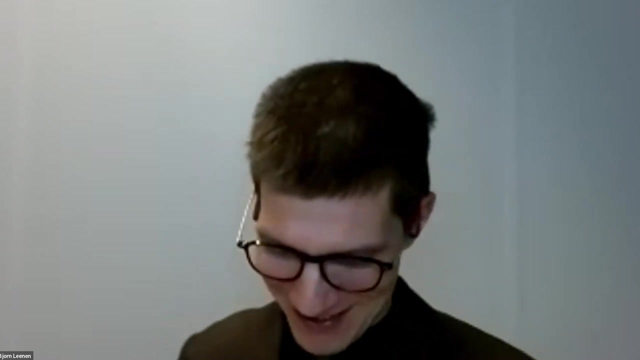 which are tools, i guess. what's your view on this? uh, uh, to the tool gap, um to rob, yes, and you must come back, martin. thank you, hank, rob too, by the way, i think this is a chapter that, uh, that uh, or a subject that is not covered yet. 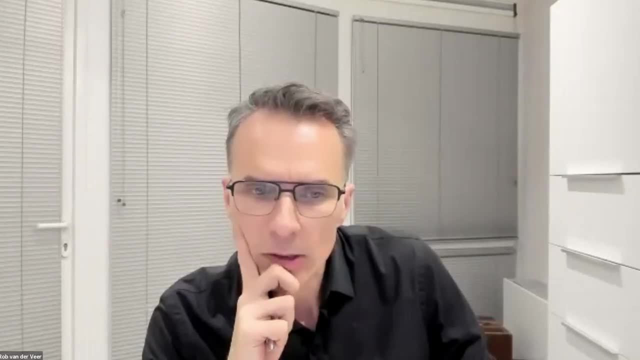 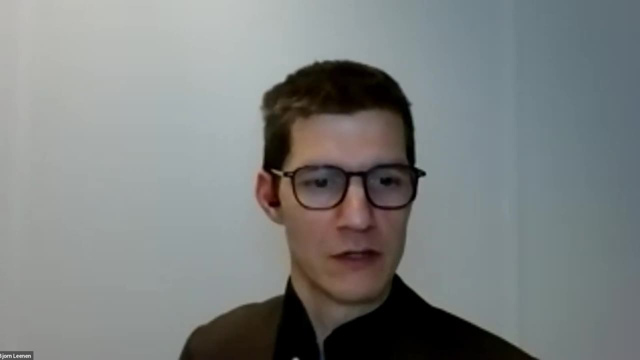 completely, so i need to parse, parse this question. can you repeat it? yeah, uh, you hear developers say that they want all the controls in code. so automation, um, which are tools? i guess. what is your view view on this? uh, to the tool gap. i don't understand the question. maybe martin does. 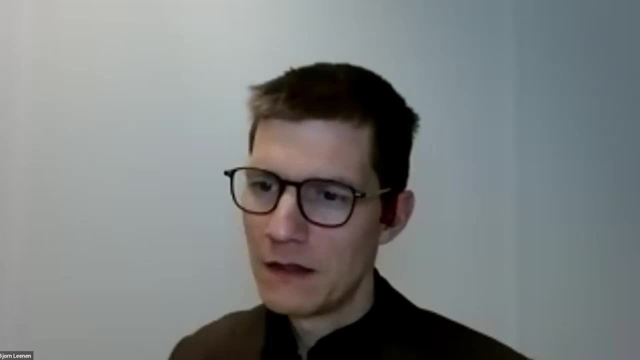 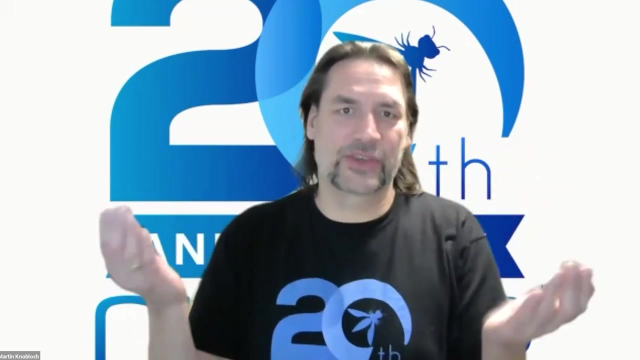 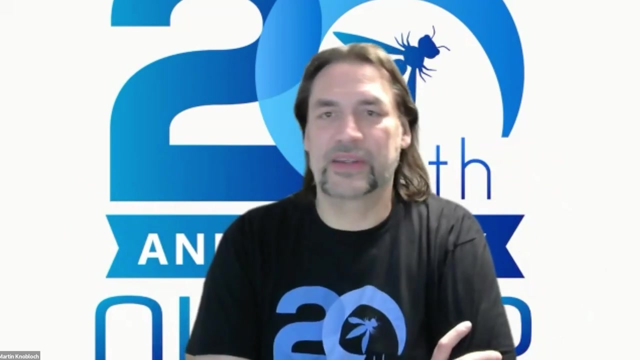 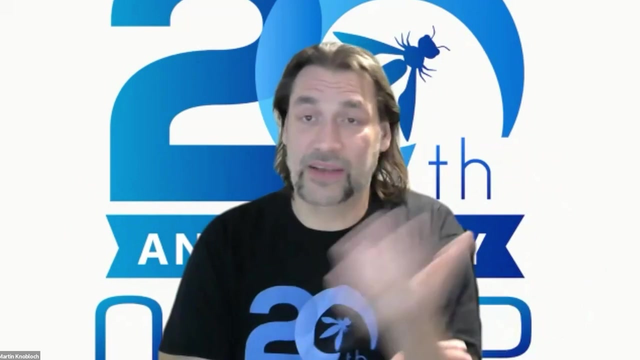 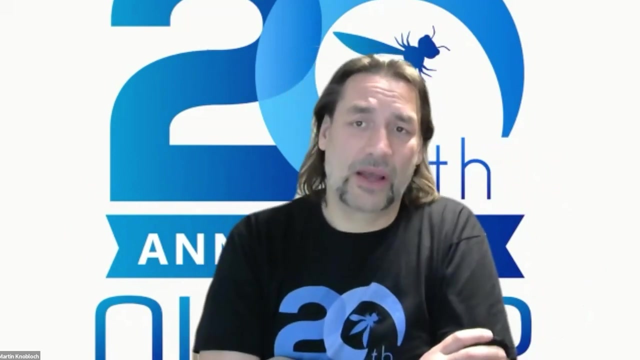 um, i think that, yeah, you cannot solve everything with the tool. i think the tool gap can be either the gap between two tools when you secure them, it's like the overlap, the correlation between the sars and dars tool, for example, and, uh, yeah, i I think the manual thing. I think that's, every tool you use, you have to. you will still, as I said, you want to have all of them, but they cost money, but they're also free. like OWASP has OWASP subproxy, there's a very highly automatable dynamic application security testing tool. 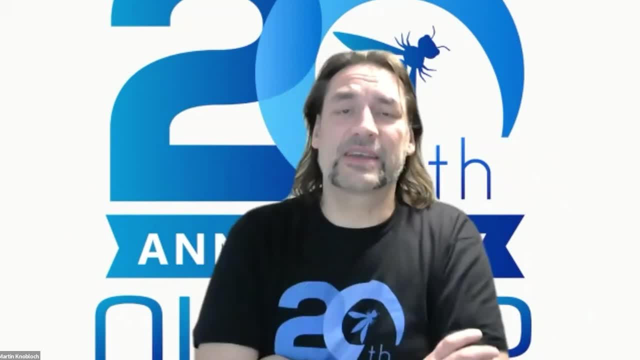 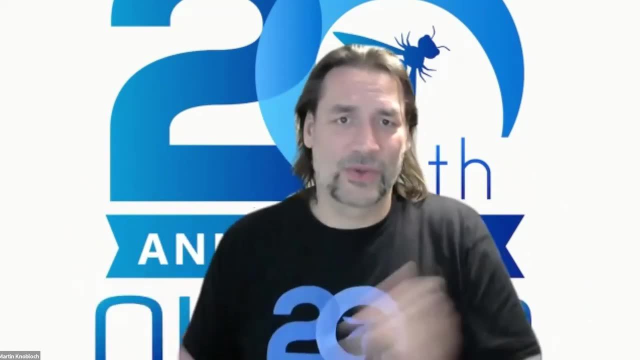 Tools solve everything you need. Yeah, I think that's the thing. so, yes, but you cannot solely rely on tools, right? A fool with a tool is still a fool, and a tool with a fool is still a tool. so, yes, they can only find technical problems, but they will never find everything. 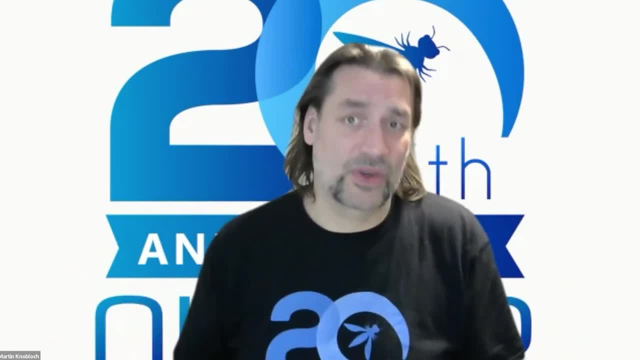 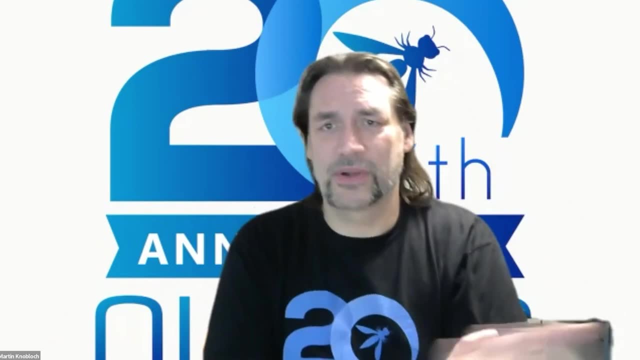 So you need more tools to find more to cover more, and I think Gary McGraw said it again about his flaws and bugs and he said: when you have 100% of the tools you use, you can only find technical problems. 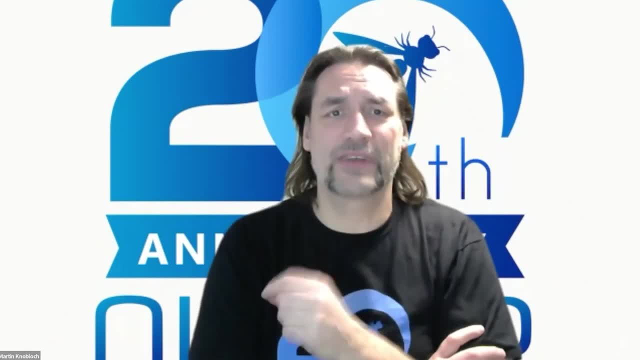 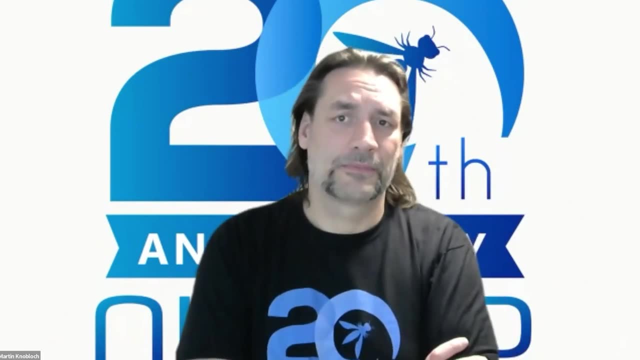 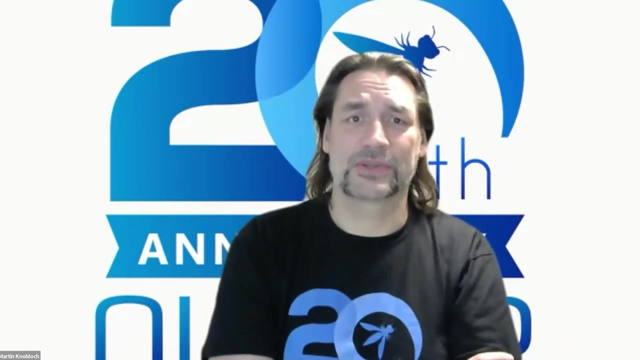 You can only find about 50% from all the security issues because you cannot find vulnerabilities. that are flaws, so functional flaws. so you will find by tool, And then you don't have all the tools, so you go down, you have like one or two tools and then you will find maybe 20% of all security issues. That's what I meant by the tools are there to find the low-hanging fruit. 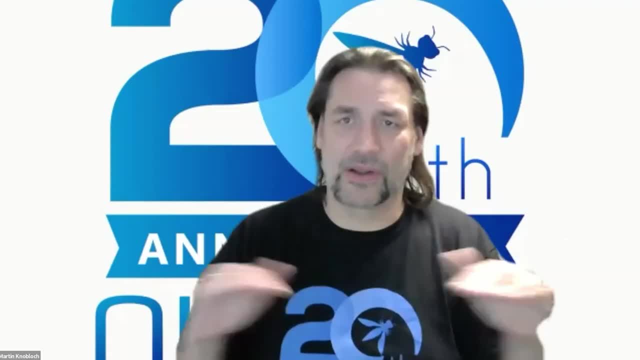 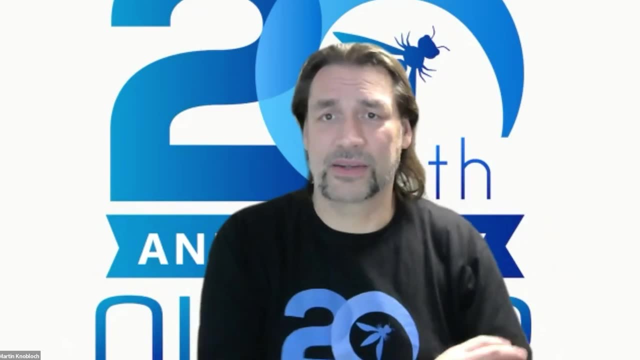 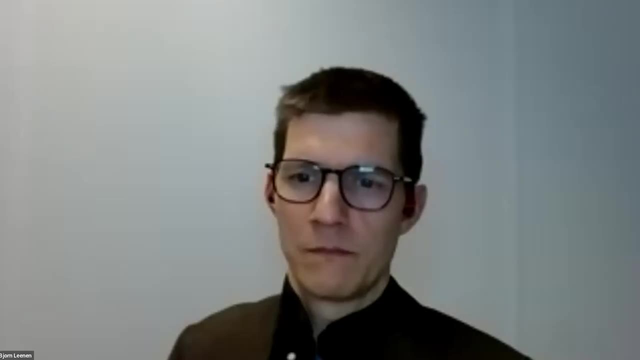 The tools are there. you have mandatory- It's a minimum level of quality And then you need you have to feed Human resources. you have to find the more out of the multi-stage security issues right? Short question: is DevSecOps a thing or is it? Is it just DevOps done the proper way? 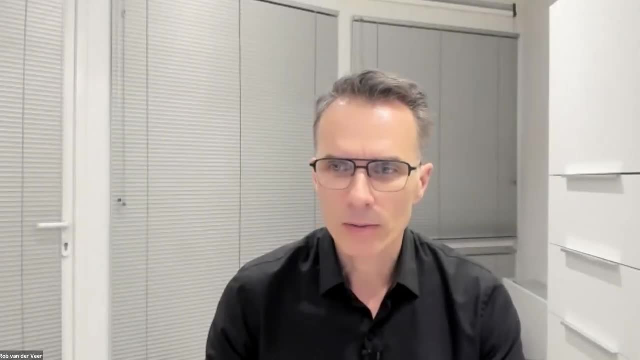 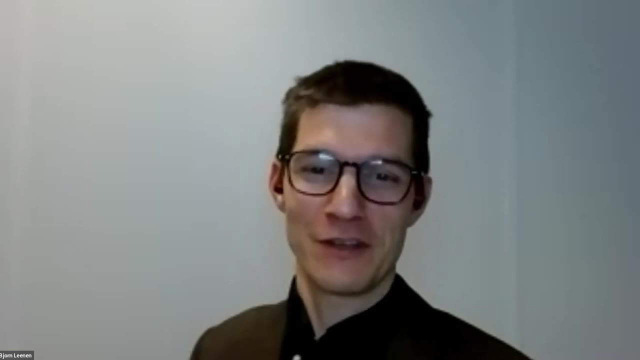 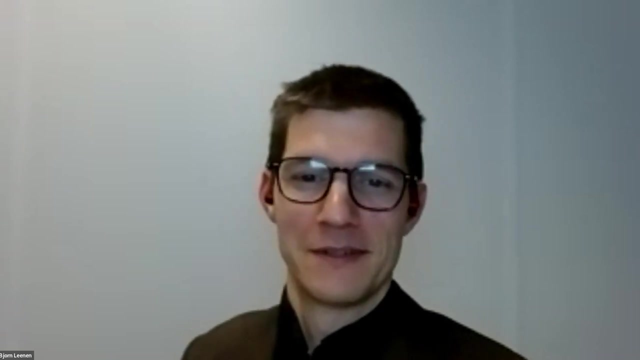 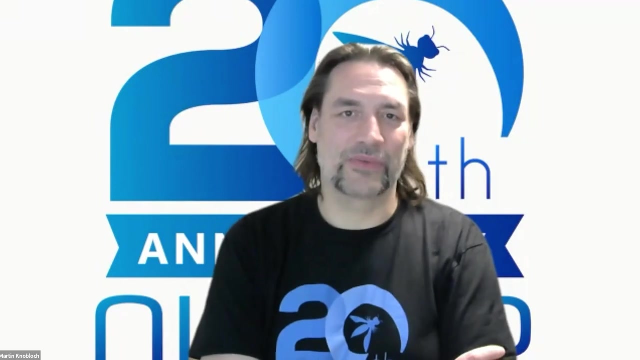 That's nice. I would say that the S in DevOps stands for security. Yeah, DevSecOps. Yeah, DevSecOps, the development security operation. Is the development operations a thing, or is development operations done properly? Wow, yeah. well, yeah, it's. I said I put it like this: the SEC should be there to put emphasis on so you develop source code and when you put emphasis on you, you have to name it. 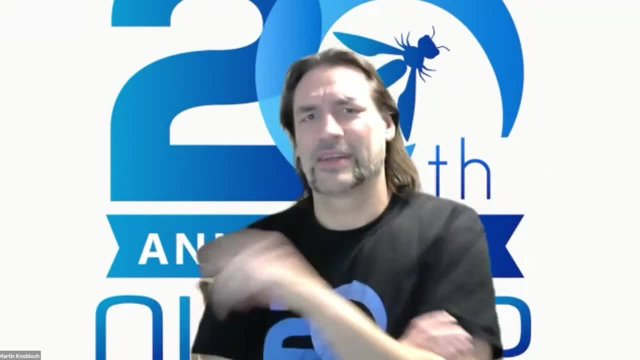 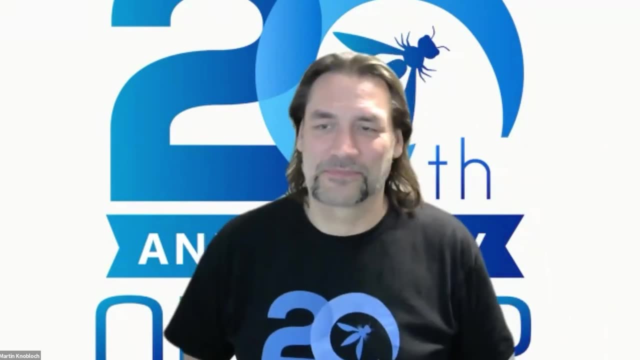 It was also the question SEC, DevOps, DevSecOps. I don't care, as long as you do why? secure code: right, Yeah, true, Yeah, okay, so it is, Let's do it in the proper way. 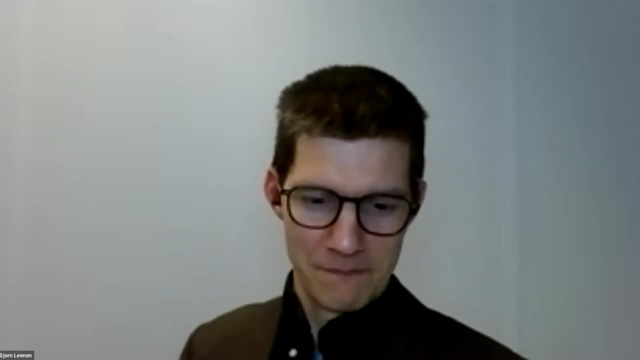 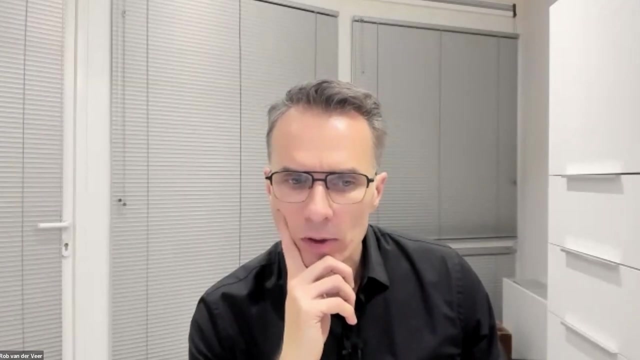 And then it is both the same thing, If I may. I noticed the question: Do your recommendations also apply in low code applications such as Mendix, IBM, FSB? Yeah, And that was indeed one. My answer would be: yes, they do. 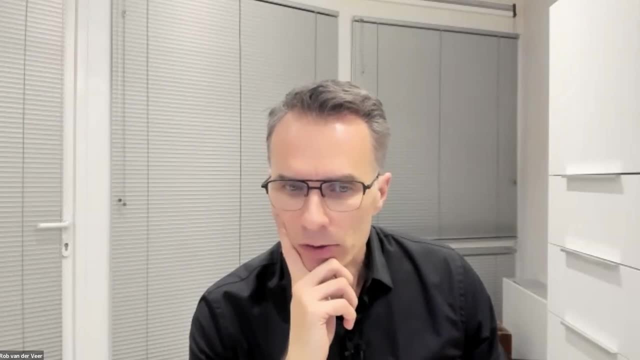 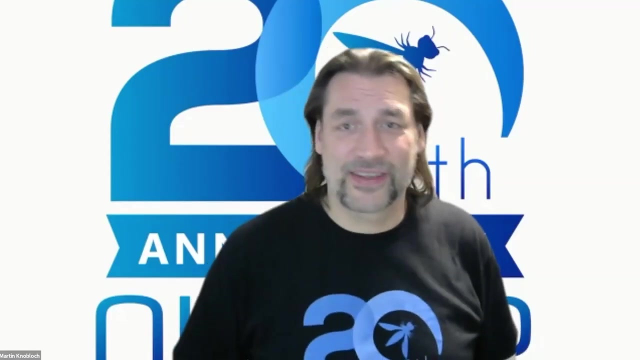 It is programming. either way. We help many organizations Doing a low code with software quality, including security. even many low-code systems also have open source dependencies. for example, It's forced by humans, Still humans, Yeah. so yes, you will not make the new mistakes, maybe because there's one with this. 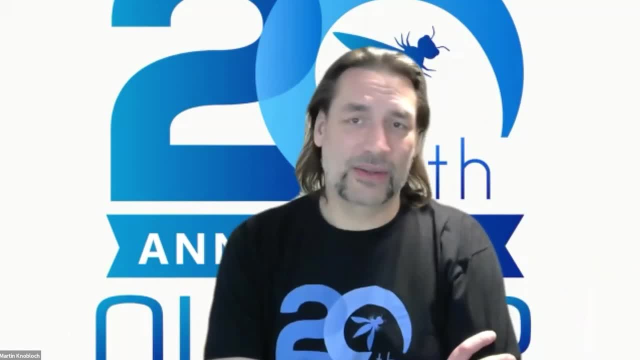 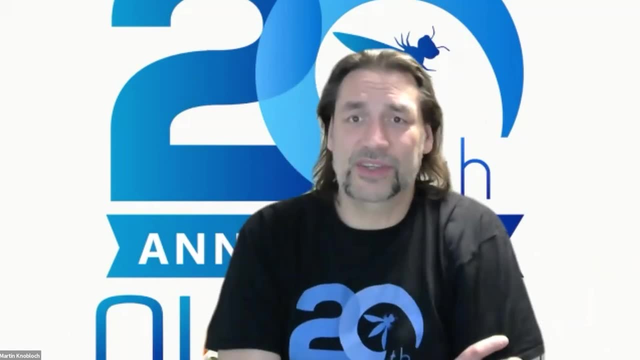 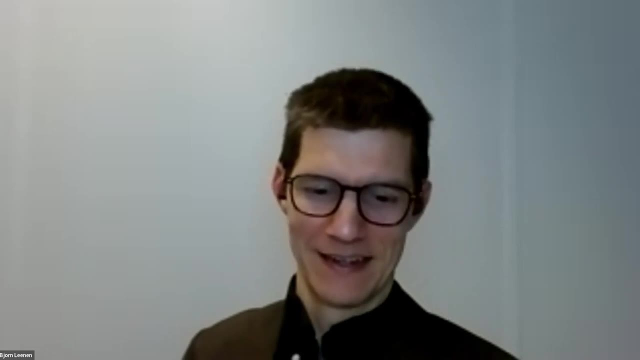 Yeah, it's the components thing that I have more people looked into it, the more we had the same with what is it called WordPress. Well, everybody was starting to despair. Yeah, WordPress by itself is secure, but it's the plugins you have, so you have low code. it's perfect, maybe, but then you have this: oh, I want to be able to change that as well. and then you introduce a new area where I can make mistakes, right. 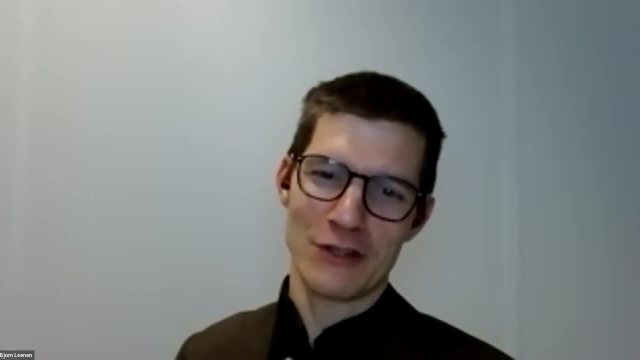 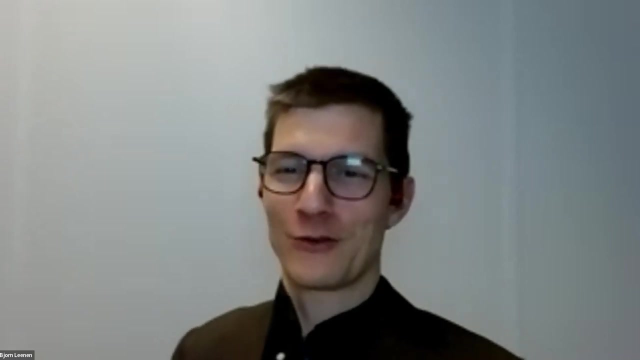 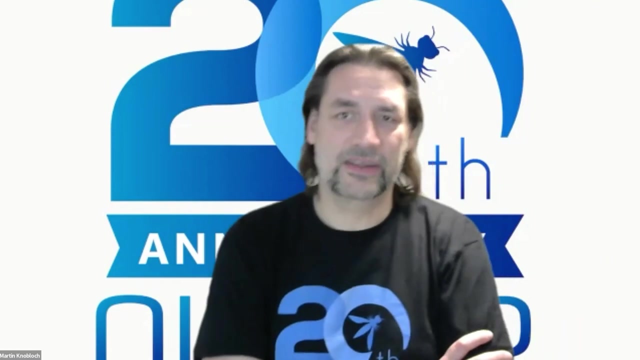 Yeah, I, like Hank says here, security is like the LGBT thing. It should go without saying. but as it does not, we need positive discrimination until it goes without saying. Well, it's also a way of yeah. Yeah, You have to make it clear. yeah, everyone has the same rights, so sometimes you have to. 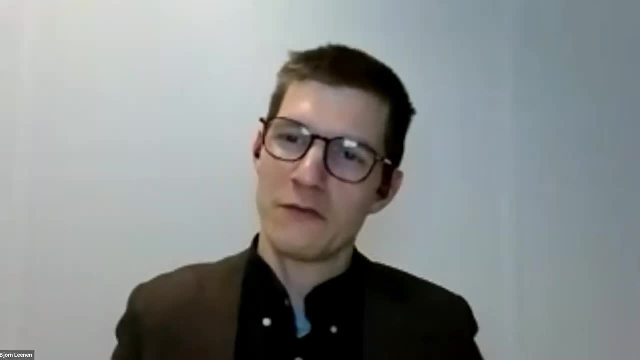 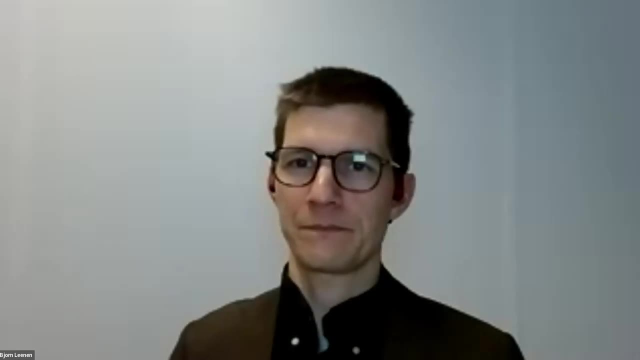 Yeah, so first it needs to be dealt with as something exclusive, and then it will be inclusive, or it should then be treated as inclusive? Yeah, it should be put an emphasis on it. Yeah, You have to make aware by being out loud about it. 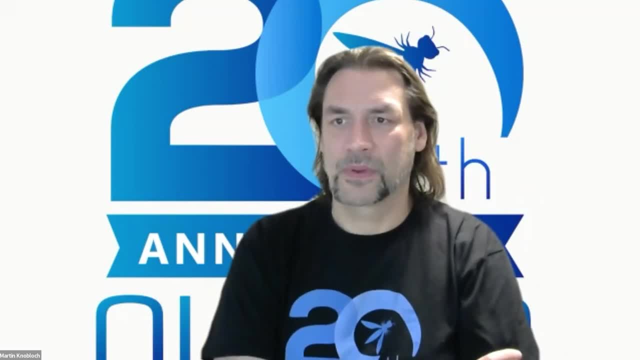 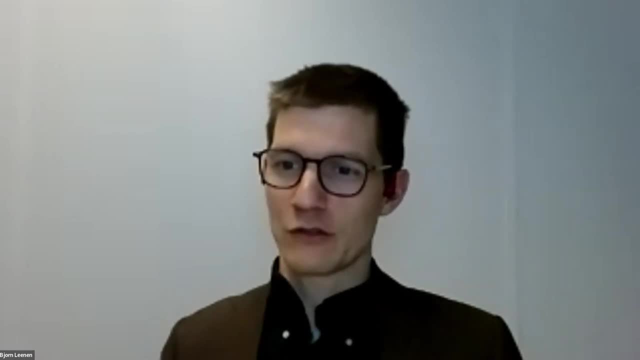 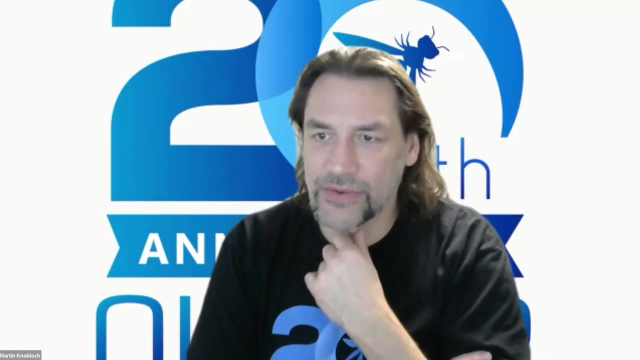 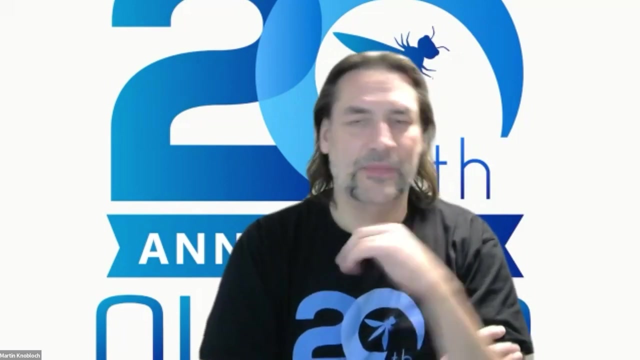 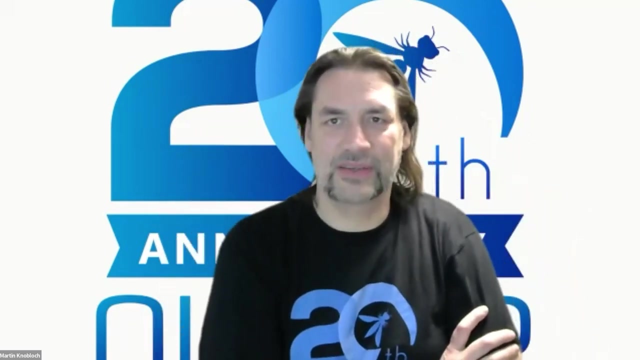 Okay, It becomes normal. yeah Yeah, I'm trying to go through everything that I copied and pasted from chat. Yeah Yeah, Q&A and so much. There's one about the ASVS and they asked if ASVS level 1 is still fully testable by tools. a good way to start- and I said as again, ASVS is when you have four levels of 0 to 3 security gradation. it's not a standard body. 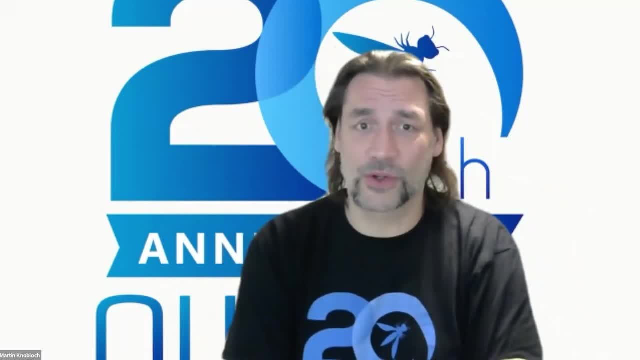 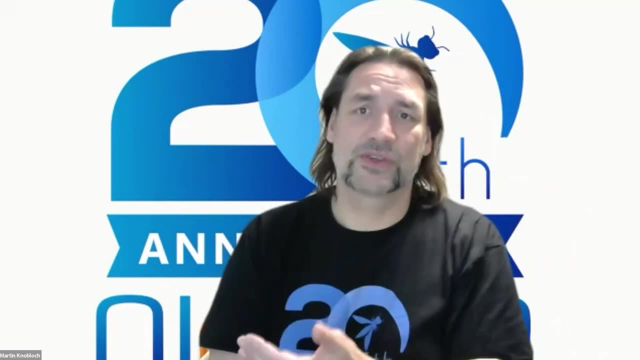 You cannot be always top 10 certified, not always some certified and not always ASVS certified, But it's about the first thing you do is to have quality tools in place. so the first thing you start with is quality and quality verification, because you have a proven quality. 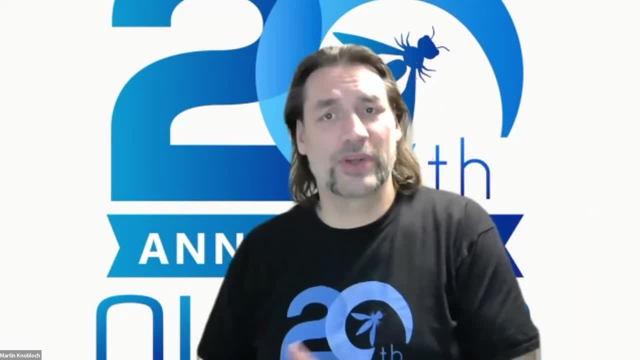 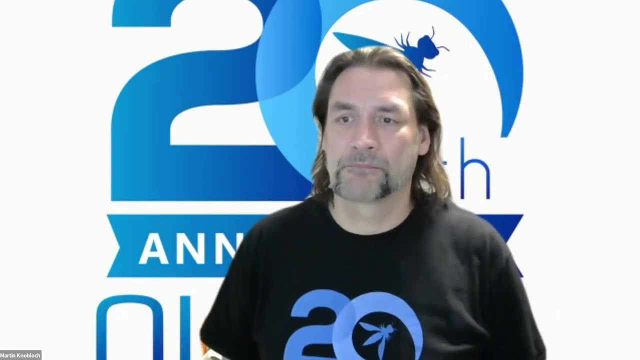 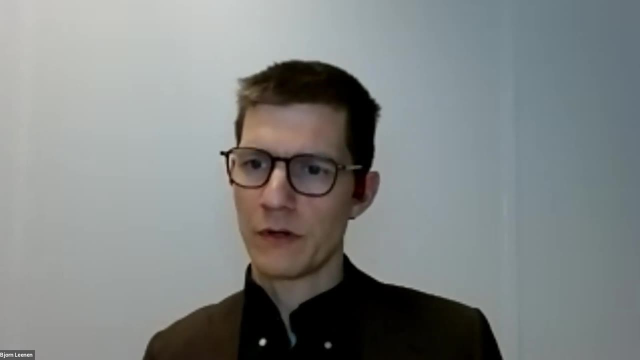 But ASVS 0, you do nothing right. So for ASVS 1, at least you have some basic tools. that's it, yeah. Okay, Let me see still things open Um any recommendation. No, that is already answered. 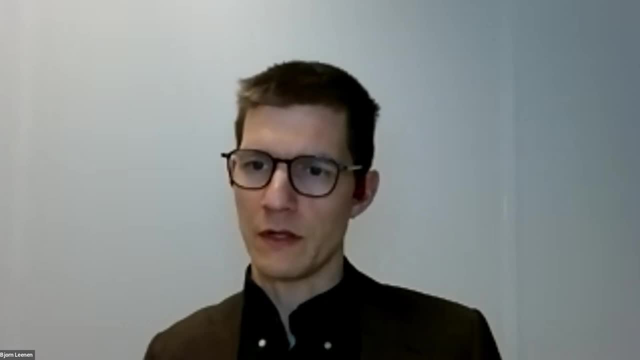 How do you balance securing software with keeping it usable The that one, two supply chain, third party. yes, I think you got the mold, Jor. Yeah, I you know what I think or what I find right now. 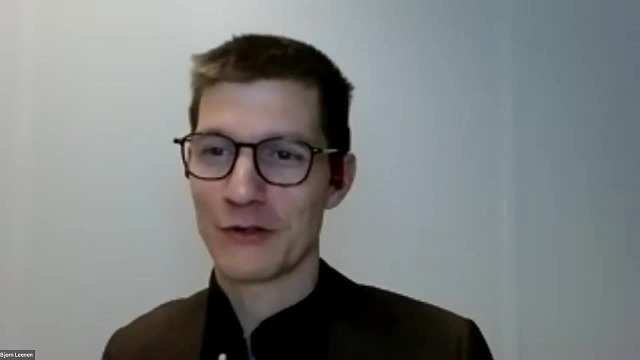 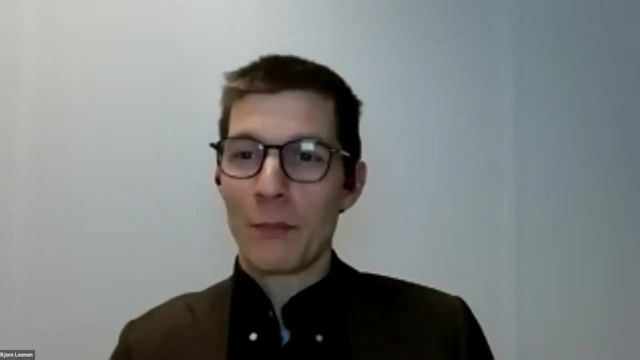 Normally it's quite difficult to get people to ask questions because most, in most situations where we either have webinars or events, you need a couple of questions to get them to ask questions. You need a couple of questions to get them to ask questions. 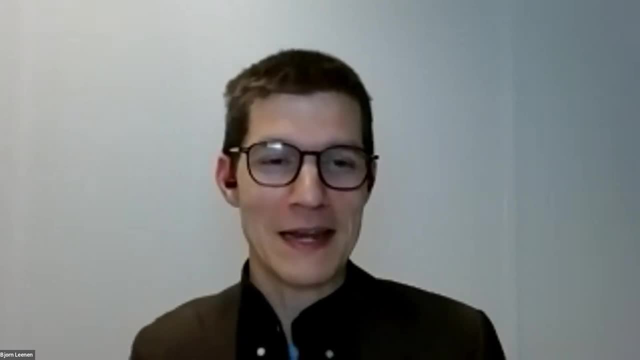 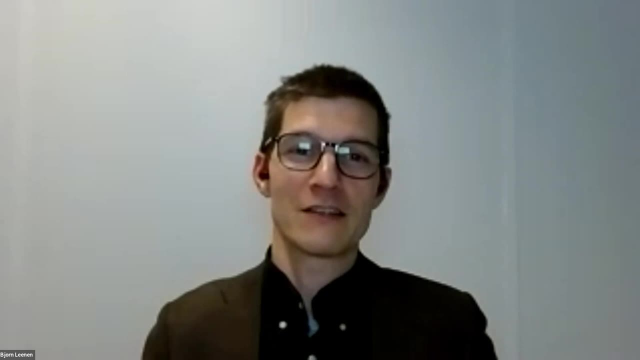 You need a couple of questions to get them to ask questions And um, but right now we had already a huge list of people posting questions, so I'm really happy about that. It that that it goes without saying that this makes it an interactive webinar. 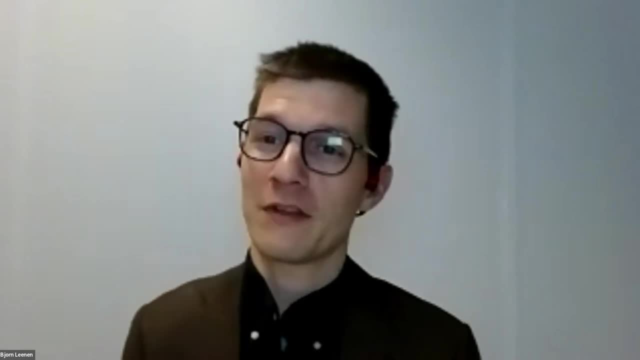 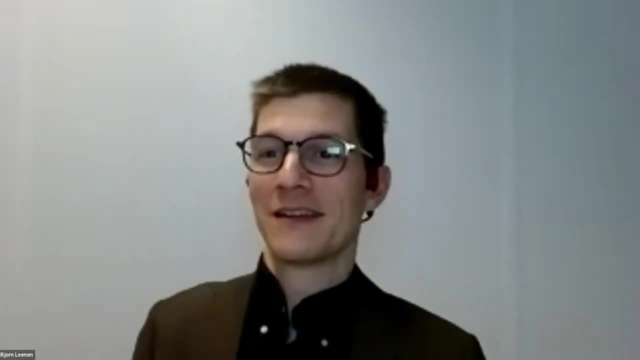 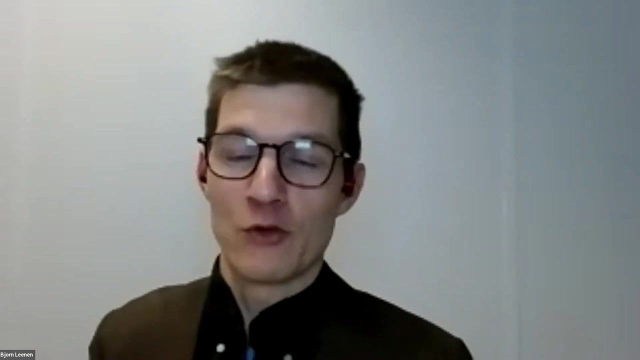 Um, so not only Martin and Rob, thank you for participating, uh, but also the audience in participating in the discussion, because otherwise it would be presentation and that's it. Um, with that. With that we can stretch it many minutes, oh sorry. yes, Martin. 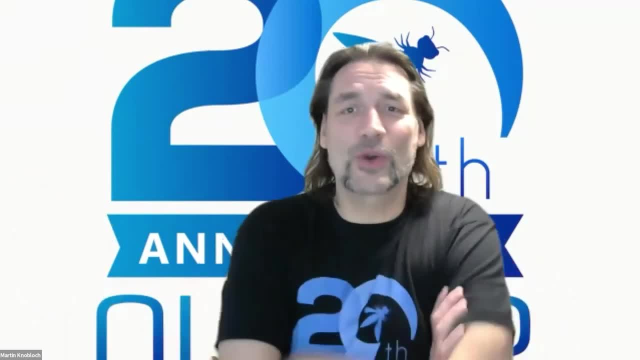 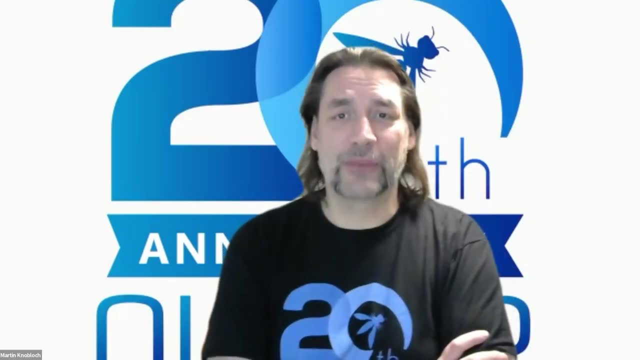 One thing in the own, the thing OWASP is free. we have a local event, the OWASP Benelux Day, and it will be the 31st of March for the training day and the 1st of April for the joke in Kottrijk in Belgium. 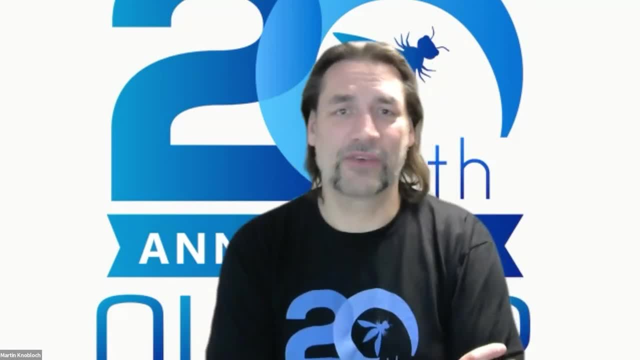 So OWASP Benelux Day, so be welcome. it's a free event. Belgium is: can we? can we reach it without being held back at the border? or, Uh, it's in April, so we don't know what the measures might be. 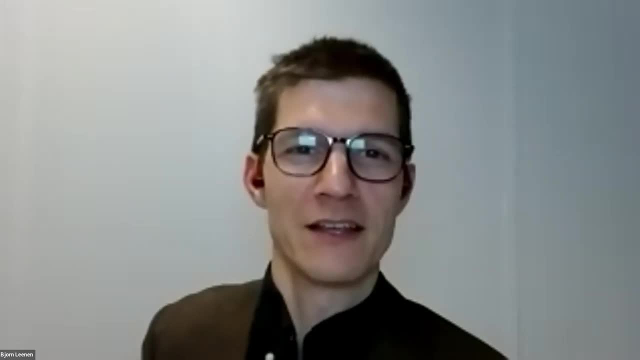 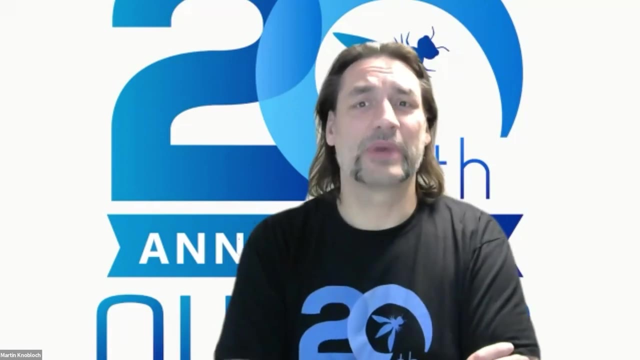 Uh, it's in April, so we don't know what the measures might be. Uh, it's in April, so we don't know what the measures might be. But but then the Benelux Day is an annual event and the last Thursday and Friday of November- from my head is the 26th and 27th, I'm not sure it will be in the Netherlands. 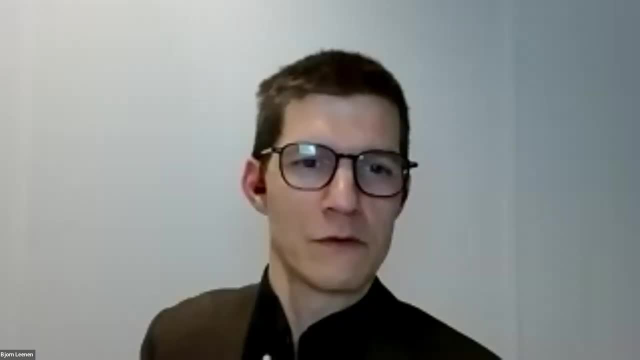 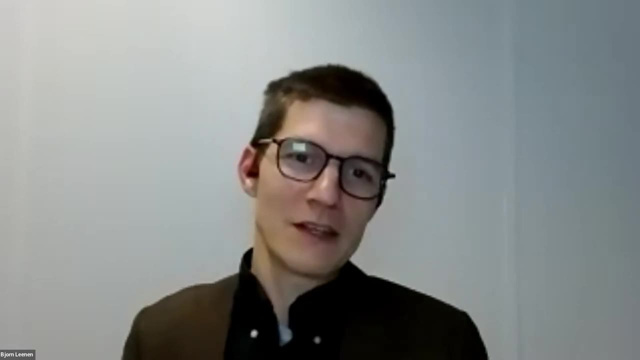 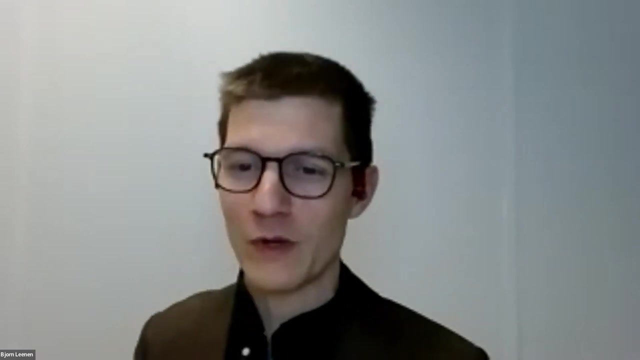 Cool, Awesome. Thank you for sharing that because I think, given by the number of questions that we got, really this is an interesting subject to talk about And people were interested, because we started with a little over 200 participants and we ended with 172.. 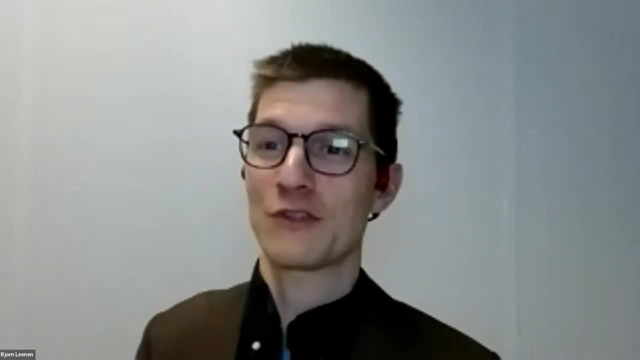 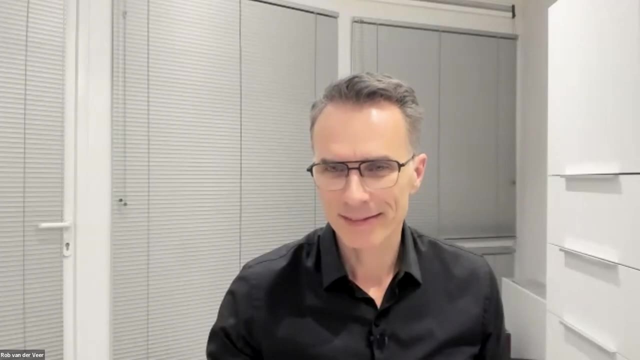 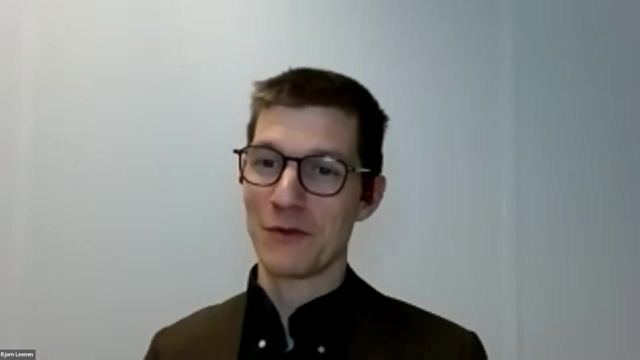 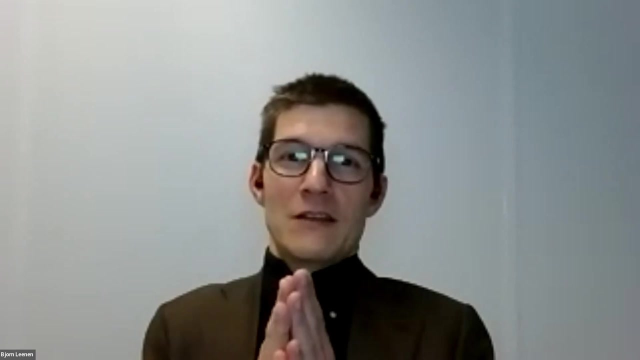 right now, and some of them excuse themselves because dinner was shouting. so, um with that, yeah, um, and it is barely over nine o'clock, so, um, yeah, thank you very much for your time, your effort, your input and sharing the knowledge with this, uh, wider audience. again, the slides will be: 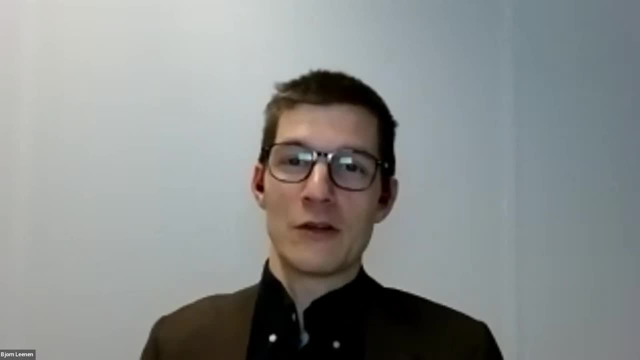 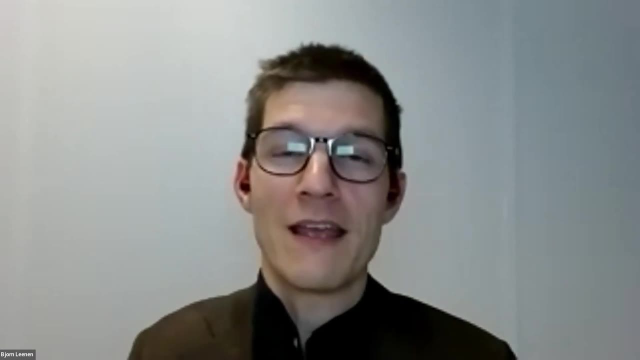 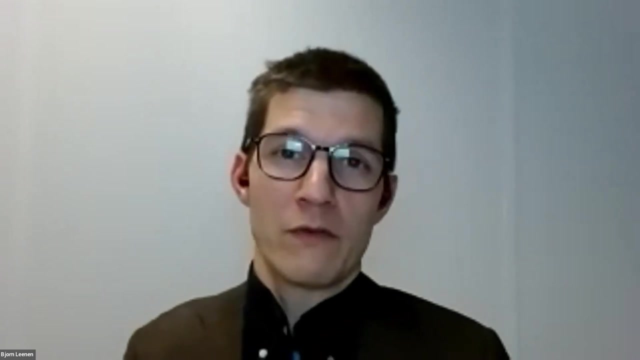 shared on the website. the recording, after it's done, will be downloaded, edited, clipped, pasted, polished- what have you? and uploaded to youtube, and i think we will update everyone through email on this, or at least it's on the website. um, for those who registered with their ic square number: 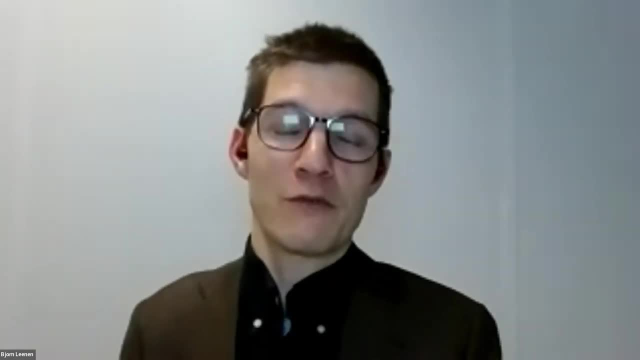 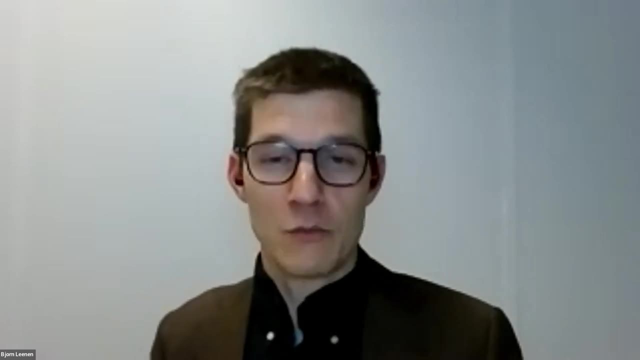 that's one very big, important question remark that i forgot to mention. you will be handed a couple of cps for this. we will do the uh, the assignment of the these points. so we will do that. it will take a couple of weeks, though, um, not because we are slow.